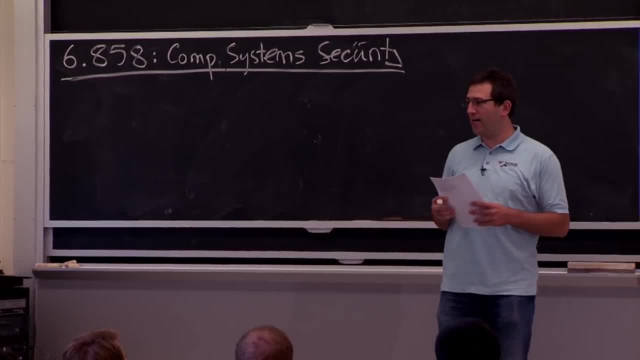 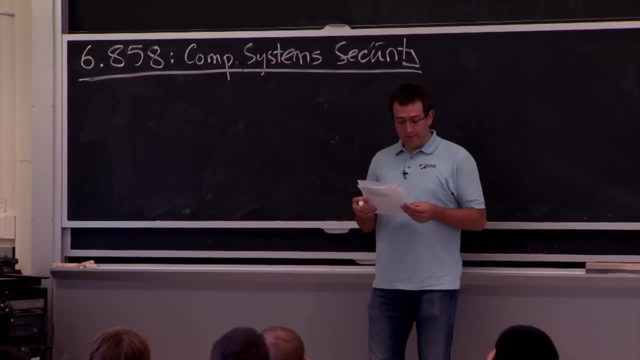 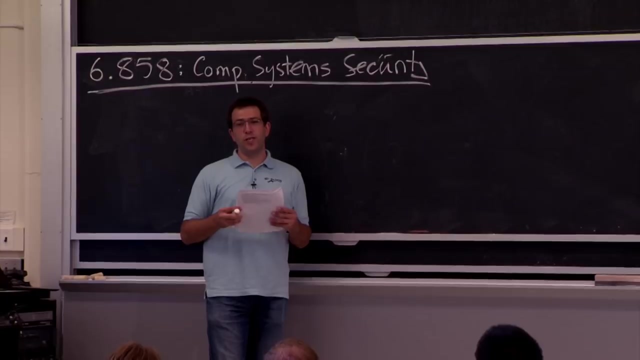 in terms of lecture split up. We also have four TAs this year- Steven Webb, Haogang and James- And hopefully you'll meet them in office hours over the year if you need help. So the plan for this class is to understand. 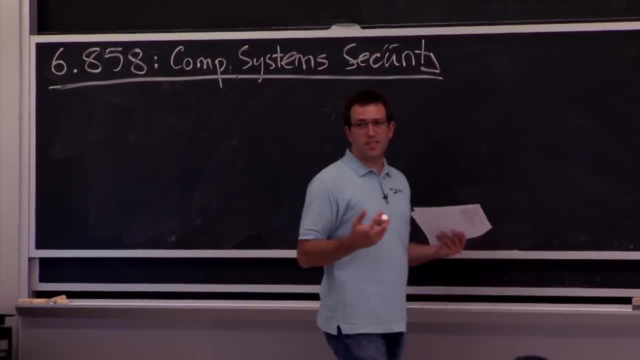 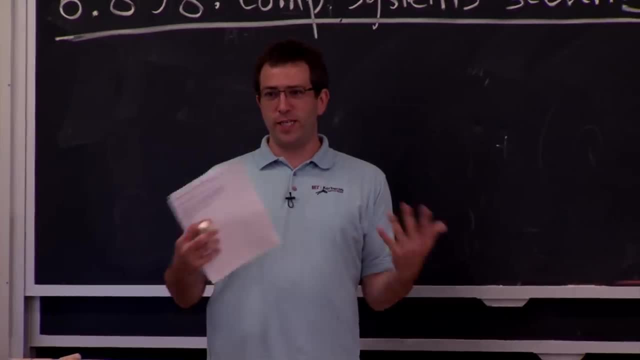 how to build secure systems, Why computer systems sometimes are insecure and how we can make them better, and what goes wrong. And in order to do this, there's not really a great textbook about this topic, So instead, what we're going to do is each lecture. 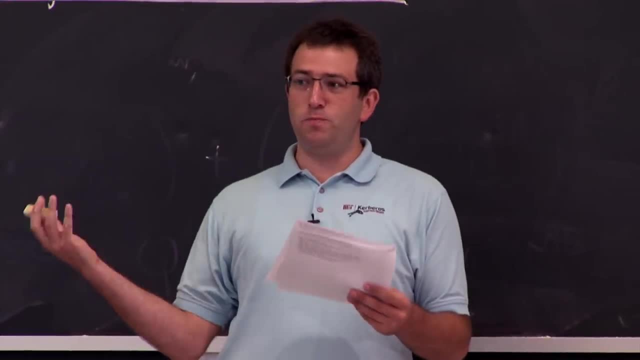 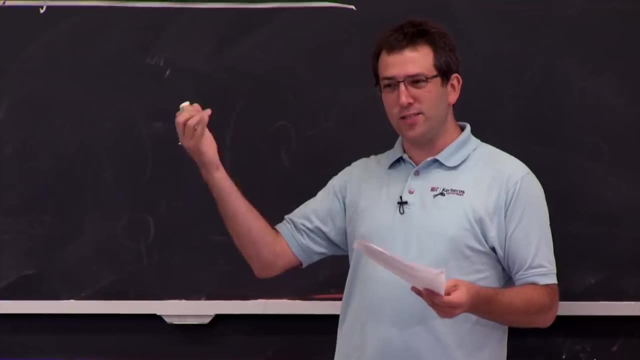 other than this. one is going to be focused around some research, typically paper that we'll assign on the website And you guys should read ahead of time And there are some questions that you should answer in the submission system about the paper and submit your own question by 10 PM before the lecture day. 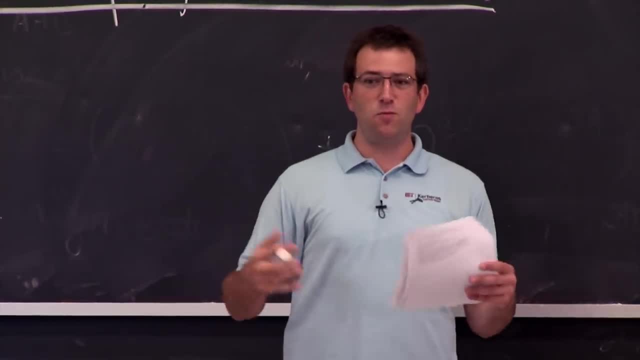 And then, when you come to lecture, we'll actually discuss the paper. figure out what is the system, what problem does it solve, when does it work, when does it not work? are these ideas any good in other cases, et cetera. 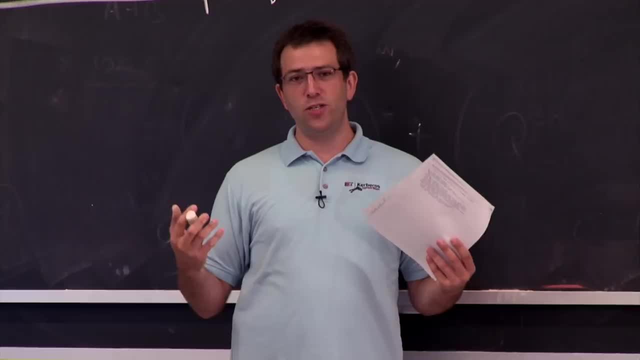 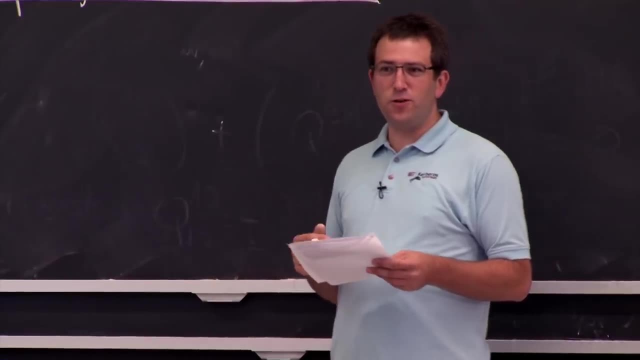 And hopefully through these case studies we'll get some appreciation of how do we actually build systems that are secure And we have some preliminary schedule up on the website If there's other topics you guys are particularly interested in or if there's particular papers you're excited about. 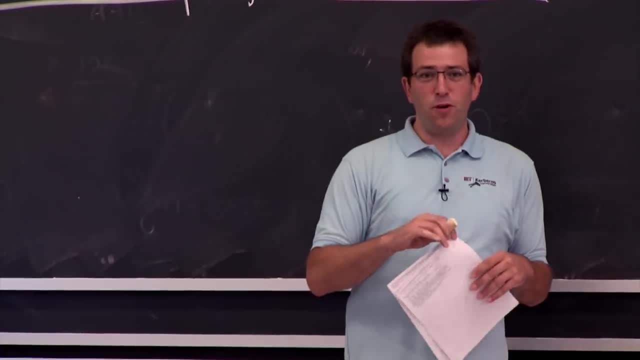 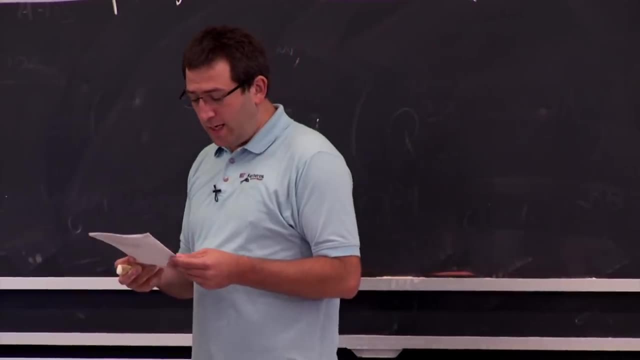 just send us email and we'll see if we can fit them in or do something. We're pretty flexible, So if there's anything that you'd like to hear more about, just let us know. And, in a similar vein, if you ever have a question. 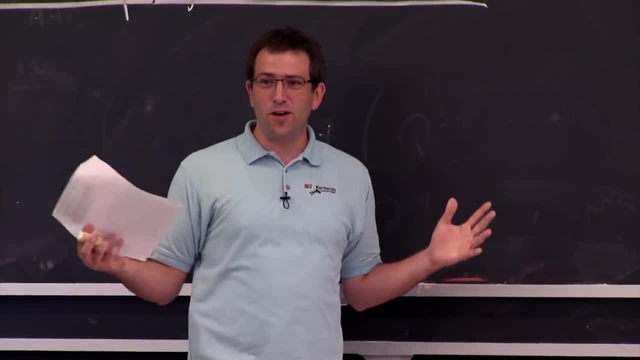 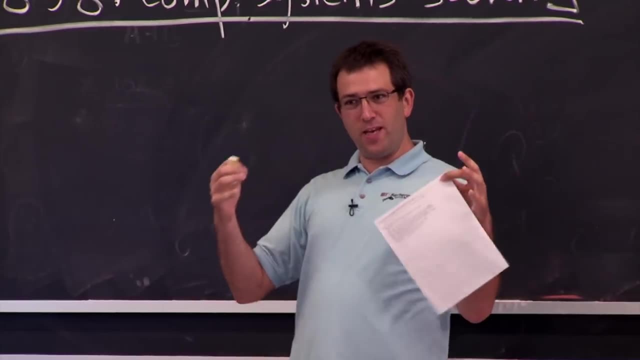 or, if there's some mistake, just interrupt and ask us What's going on in lecture any time. Security is, in many ways, all about the details and getting everything right, And I will inevitably make mistakes, So if something doesn't seem right, 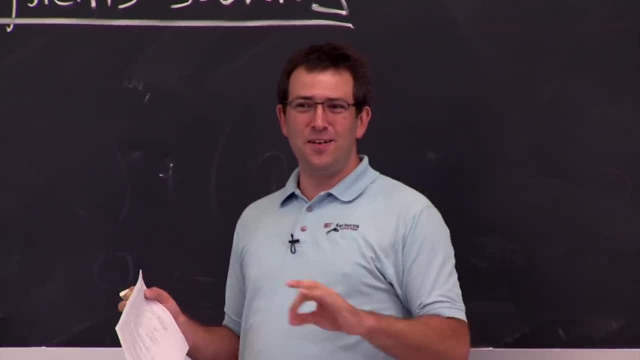 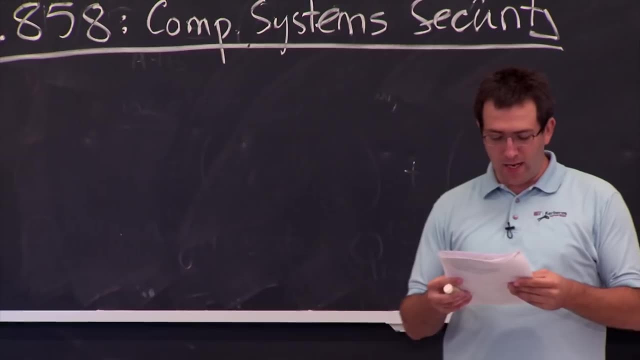 there's a good chance, it's not, And you should just interrupt and ask And we'll figure out what's going on and what's the right way to do things. And I guess, in terms of the class organization, the other large part of the class, 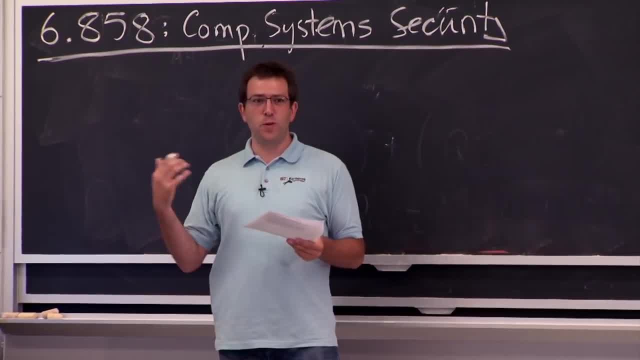 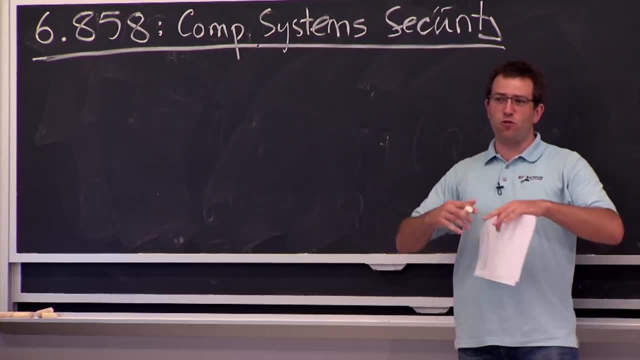 in addition to the lectures is going to be a series of lab assignments. The first one is already posted on the website And these lab assignments will help you go through understanding a different range of security problems and how do you prevent them in a simple web server. 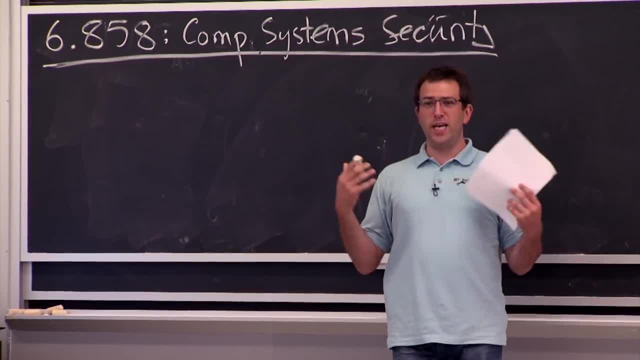 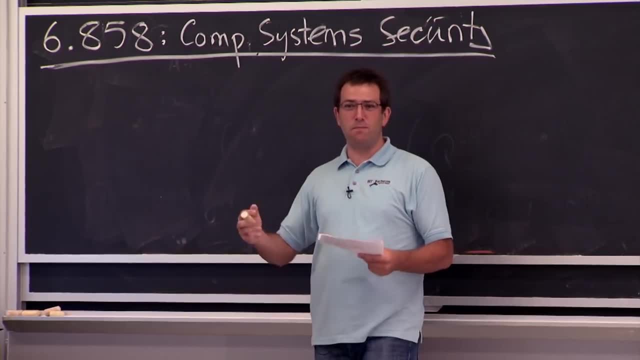 So in lab one which is out right now, you'll actually take a web server that we give you and find ways to exploit buffer overflow vulnerabilities, And you'll take control of this website by just sending it carefully crafted requests and packets. And in other labs you'll look at ways. 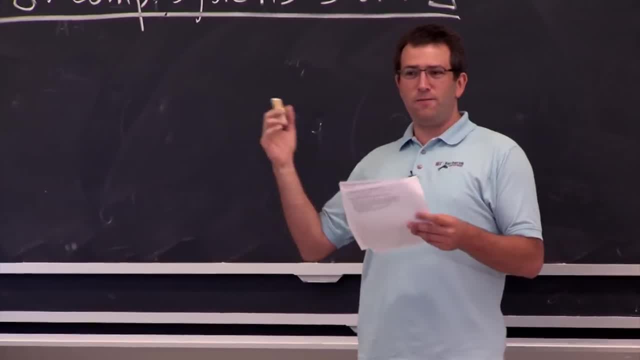 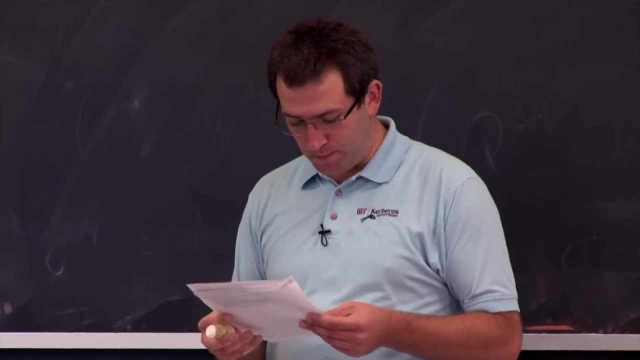 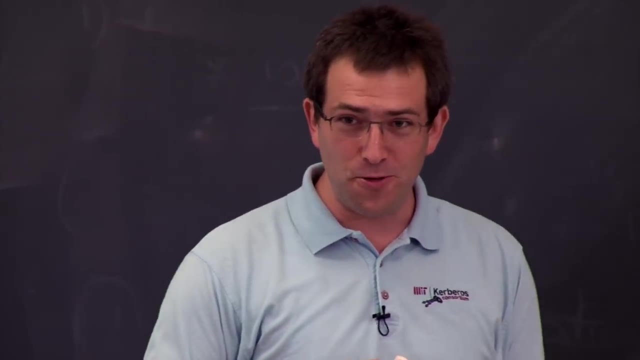 to defend the web server, to find bugs in the code, to write worms that run in the user's browser and other kinds of interesting security problems. One thing that surprises many students is that every lab uses a different language. So lab one is all about C and assembly. 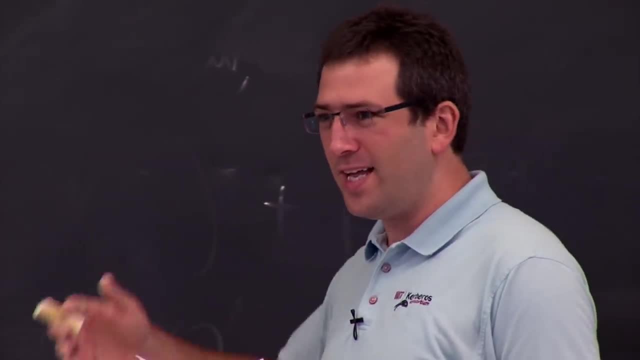 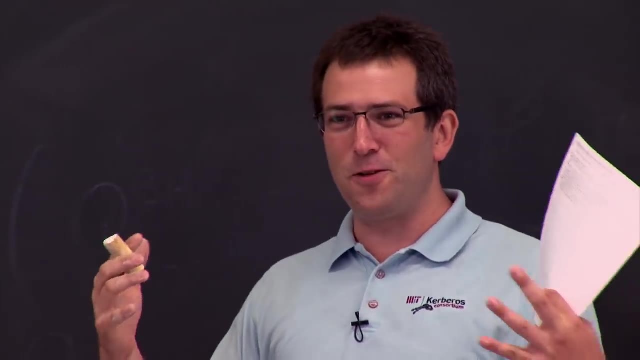 Lab two involves a lot of Python coding. Lab three will be something else. Lab five will be JavaScript and so on. This is sort of inevitable And I sort of apologize ahead of time that you're going to have to learn all these languages. 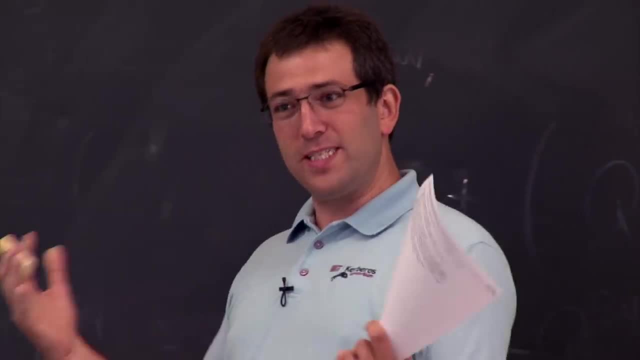 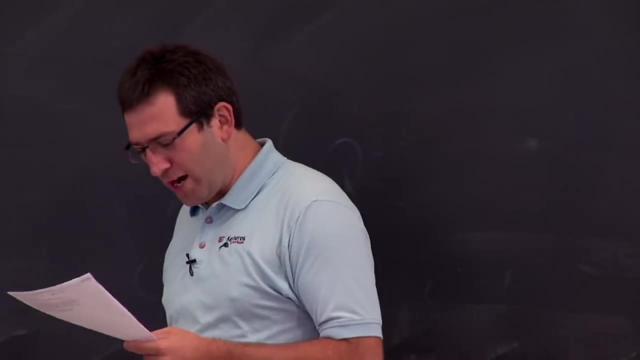 if you haven't seen them already. In some ways it's useful, because the real world is like this: All the systems are complicated and composed of different parts, And in the long run, it'll be useful for you to, for your moral character or something like that. 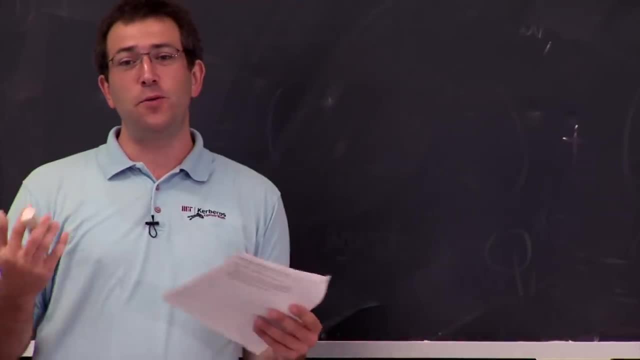 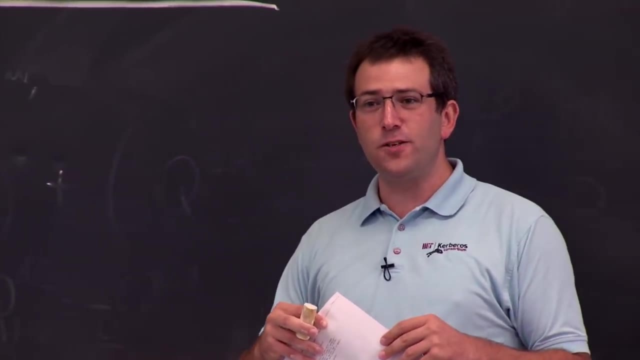 to learn this stuff, But it will take some preparation. especially if you haven't seen these languages before, It might be helpful to start early In a particular lab. we're going to rely on a lot of subtle details of C and assembly code. 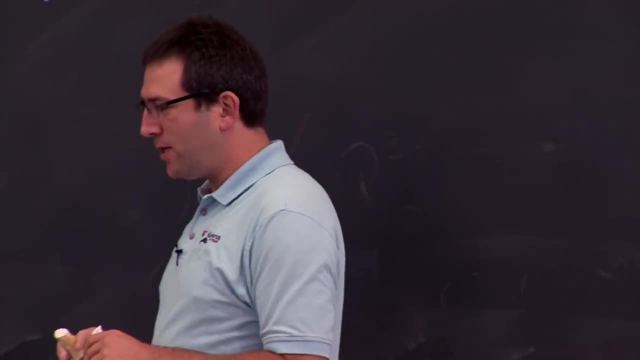 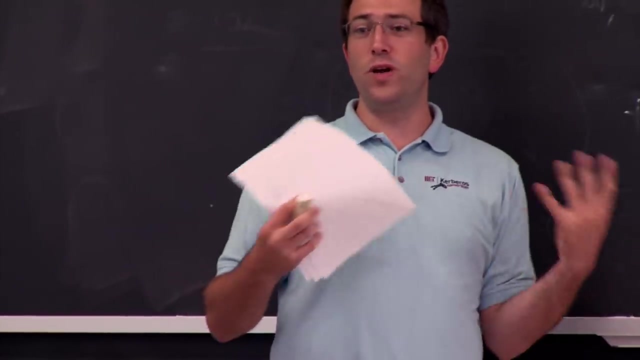 that we don't really teach in other classes here in as much detail. So it's probably a good idea to start early And we'll try to get the TAs to hold office hours next week where we'll do some sort of a tutorial session where 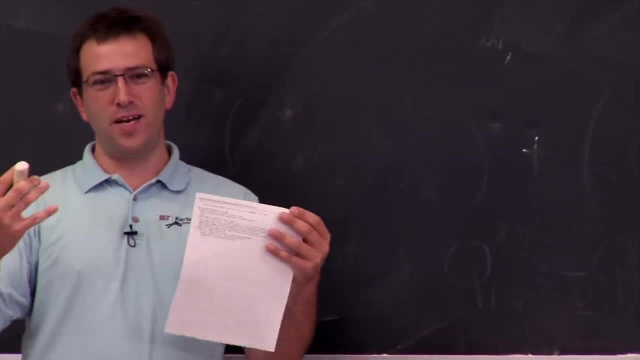 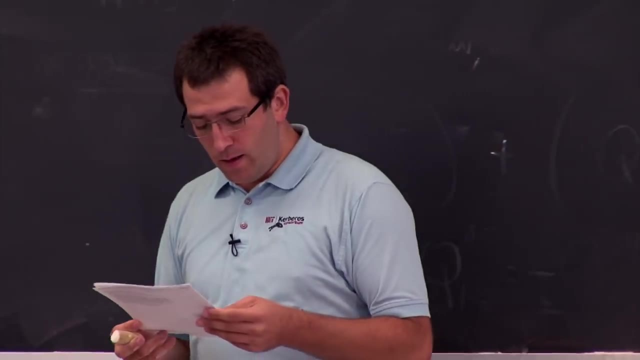 we can help you get started with understanding what a binary program looks like, how to disassemble it, how to figure out what's on the stack and so on. All right, And I guess the one We're actually videotaping lectures this year. 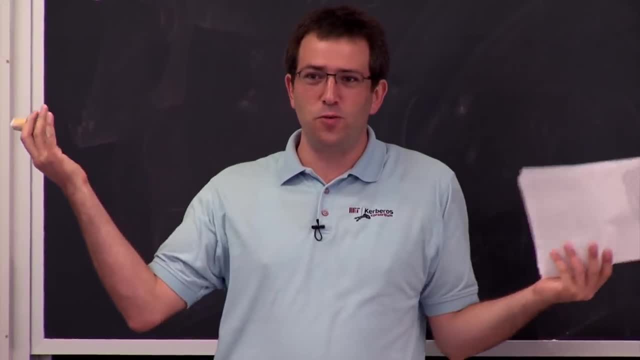 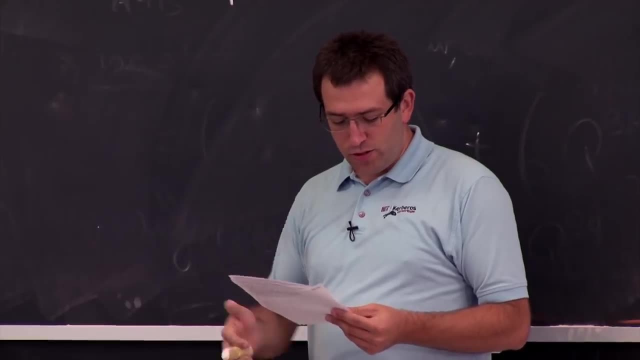 So you might be able to watch these online. We'll post them as soon as we get them ourselves from the video people. And the last bit of administrivia is if you have questions online. we're using Piazza, So I'm sure you've used this in other classes. 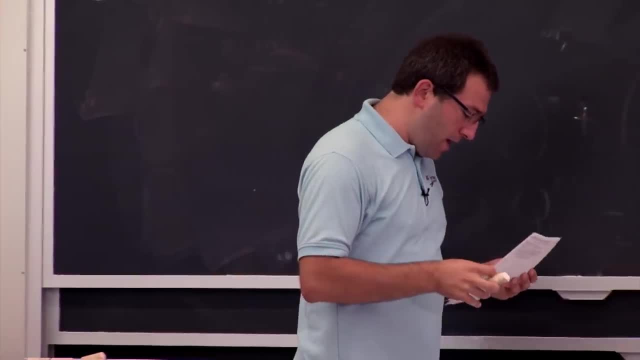 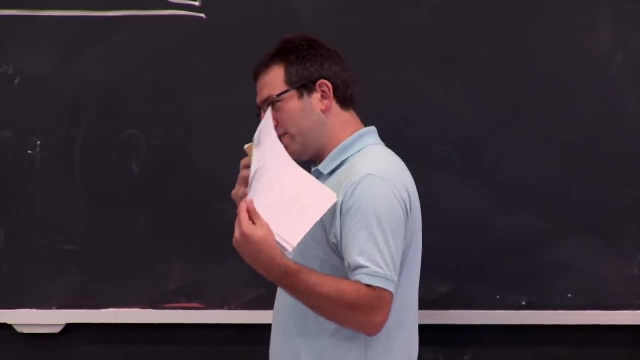 All right. So before we dive into security, I need to tell you one thing: There's a set of rules that MIT has for accessing MIT's network, And when you're especially doing security research or playing with security problems, you should be aware that not everything you can technically 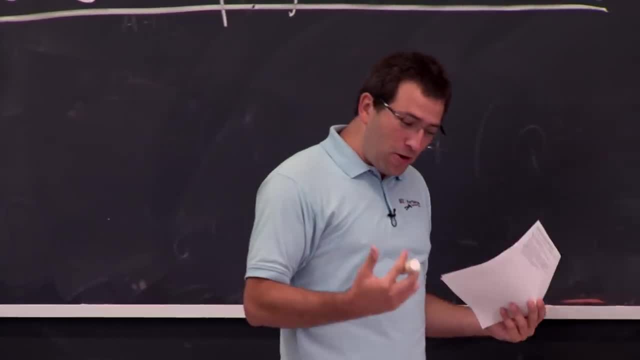 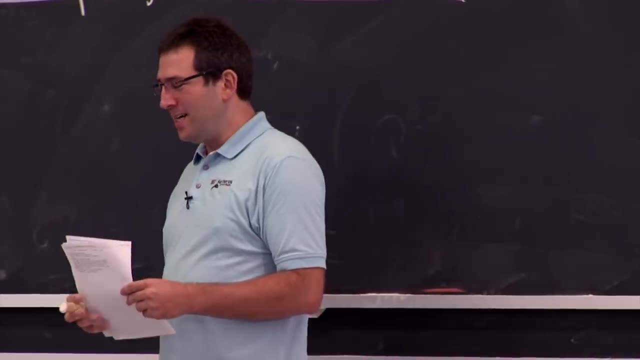 do is legal, And there's many things that you'll learn in this class that are technically possible. We'll understand how systems can be broken or compromised. Doesn't mean you should go out and do this everywhere, And there's a link in the lecture notes. 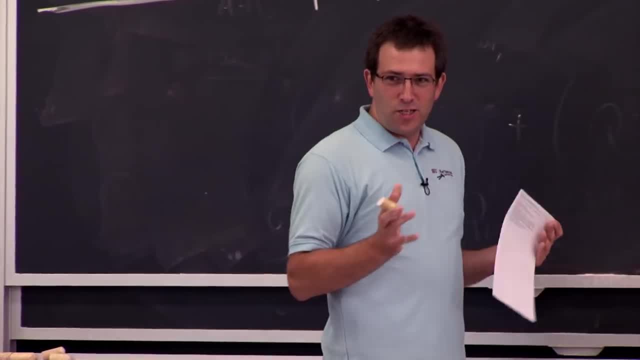 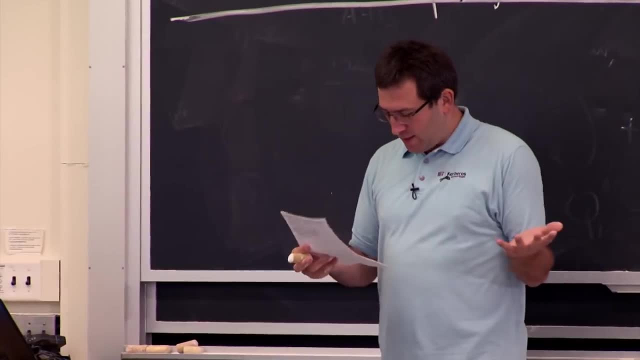 we'll post. that has some rules that are good guidelines, But in general, if you're in doubt, ask one of the lecturers or a TA as to what you should do. All right, And hopefully it's not too puzzling what's going on. 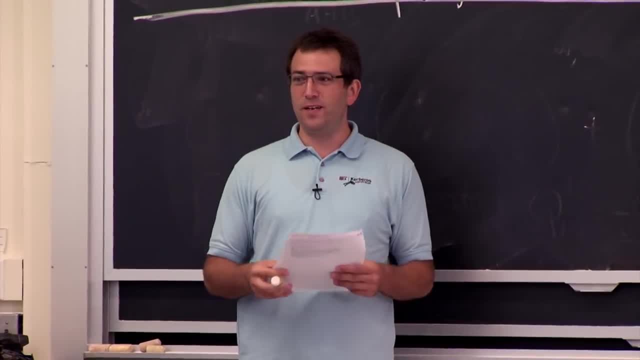 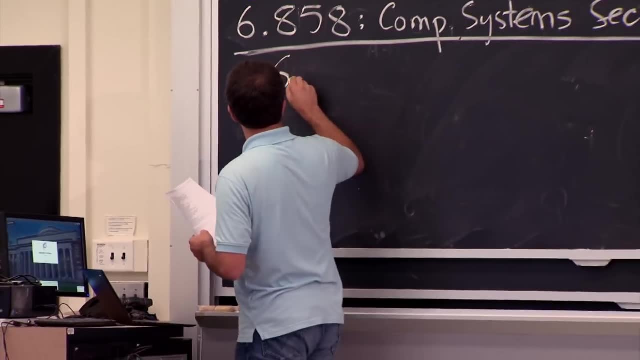 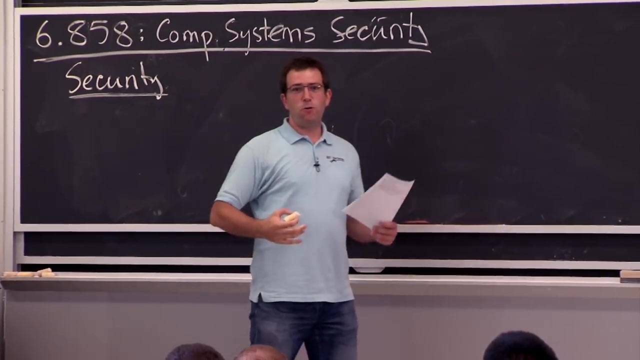 All right. So any questions about all this administrivia before we dive in? Feel free to ask questions. OK, So what is security? So we'll start with some basic stuff today And we'll look at just some general examples of why security is hard and what it means. 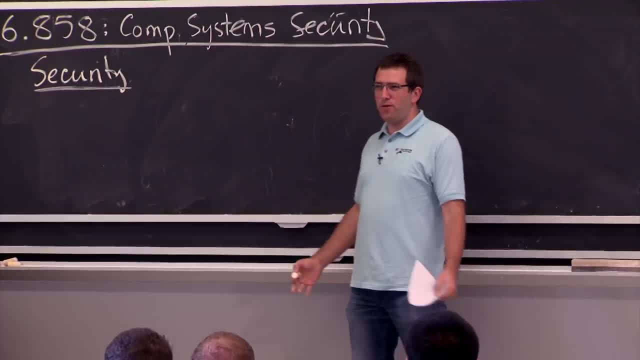 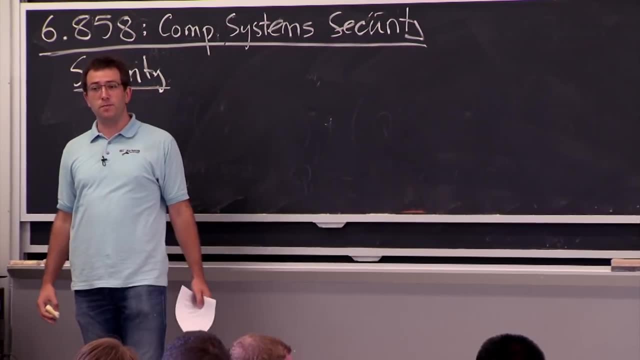 to try to build a secure system, Because there's not really a paper. this will not have sort of deep intellectual content maybe, but it will give you some background and context for how to think about secure systems. So security in general is all about achieving some goal. 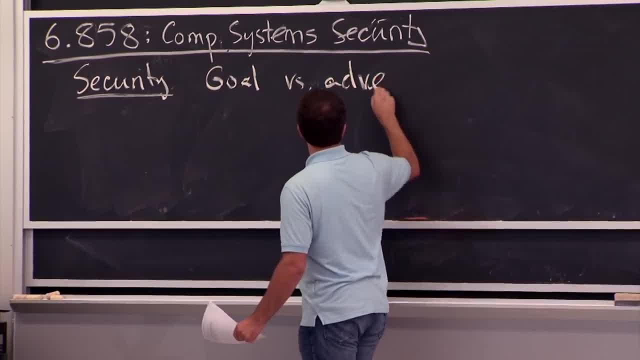 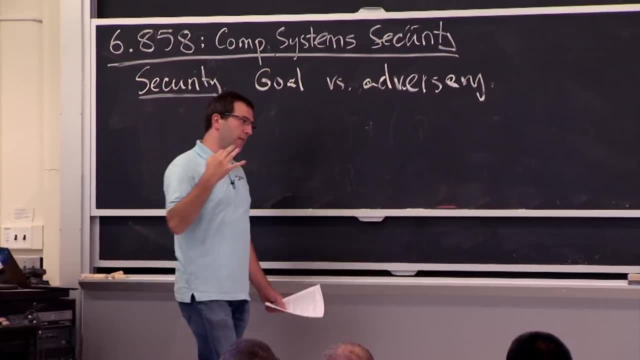 when there's an adversary present. So think of it as there's some bad guy out there that wants to make sure you don't succeed. Like they want to steal your files, they want to delete your entire hard drive contents. they want to make sure nothing works. 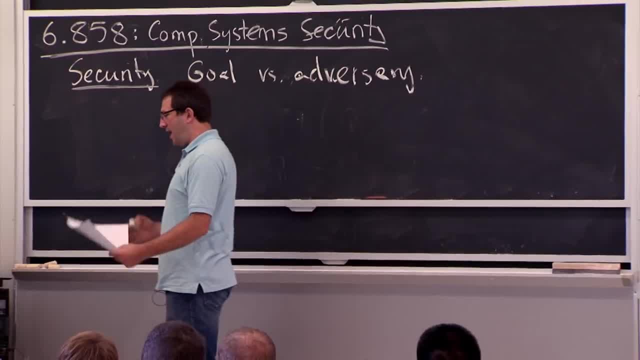 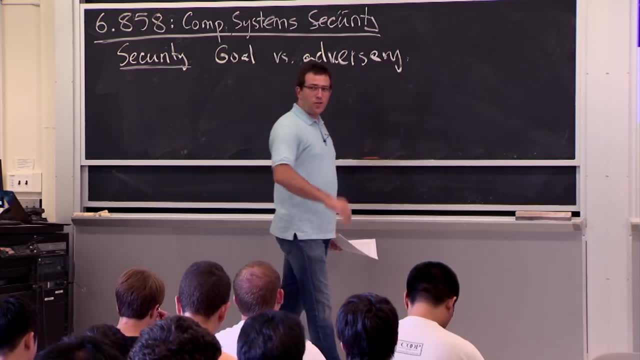 and your phone doesn't connect all these things, Right, Right, And a secure system is one that can actually do something regardless of what the bad guy is trying to do to you. So it's kind of cool that we can actually potentially build. 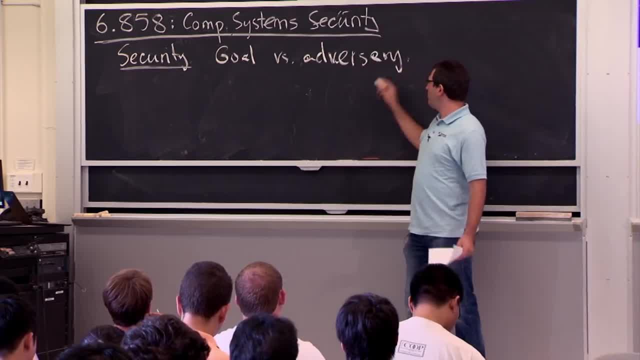 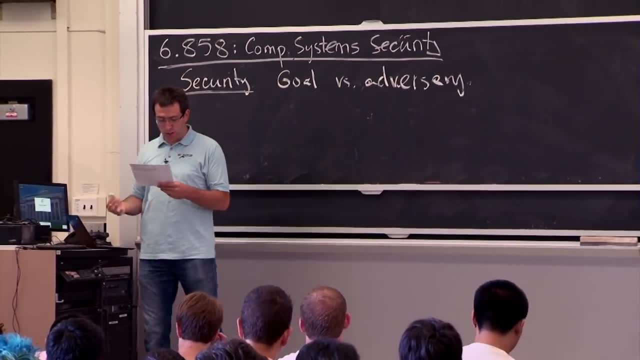 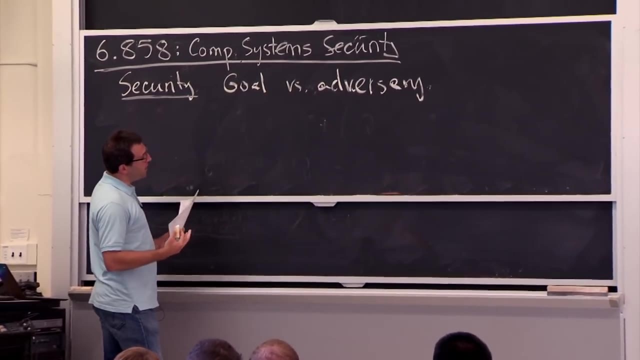 systems that are resilient to a whole range of bad guys- adversaries, attackers, whatever you want to call them- And we can still build computer systems that allow us to get our work done. And the general way to think about security is sort of break it up into three parts. 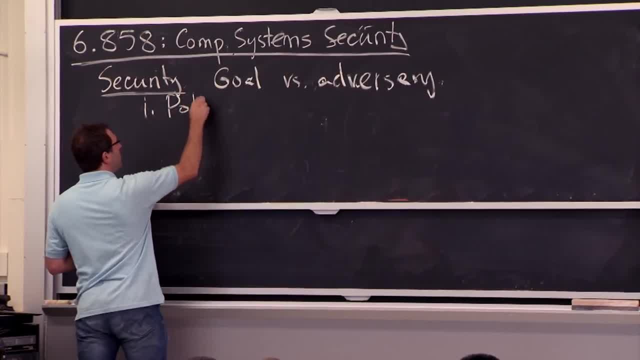 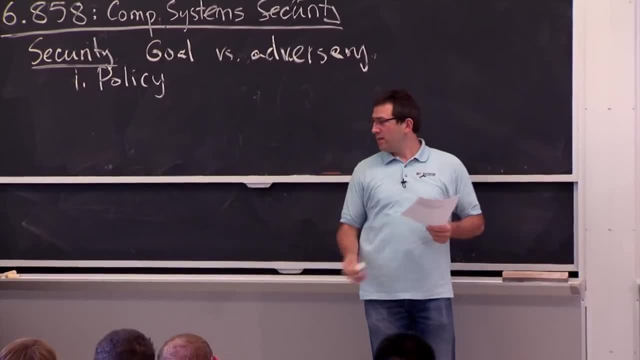 One part is roughly OK. This is roughly the policy that you want your system to enforce. This is roughly the goal that you want to achieve, Like well, maybe only I should be able to read the grades file for 6858.. 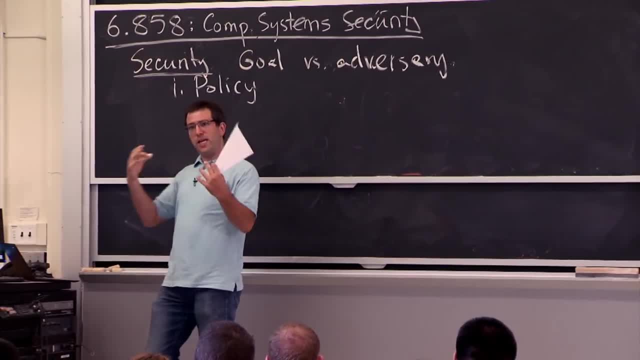 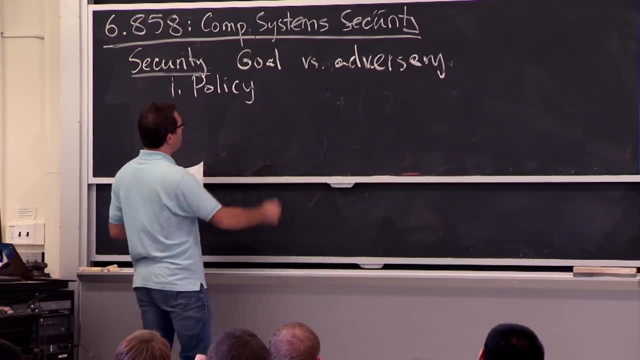 Or maybe the TAs as well, and all the co-lectors, et cetera. But there's some statement about what I want my system to be able to do And then, if we want to sort of think about what kinds of policies you might write- typical ones- 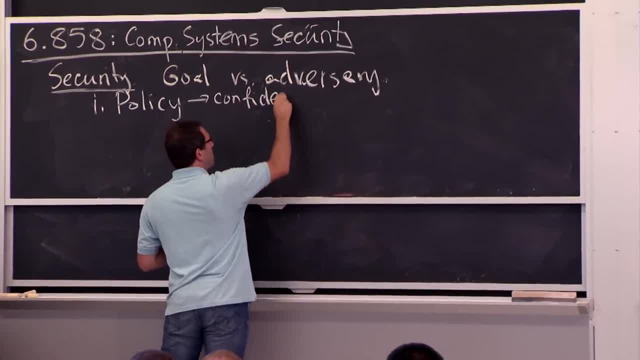 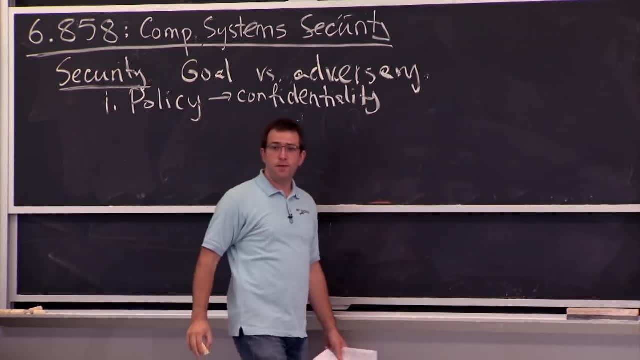 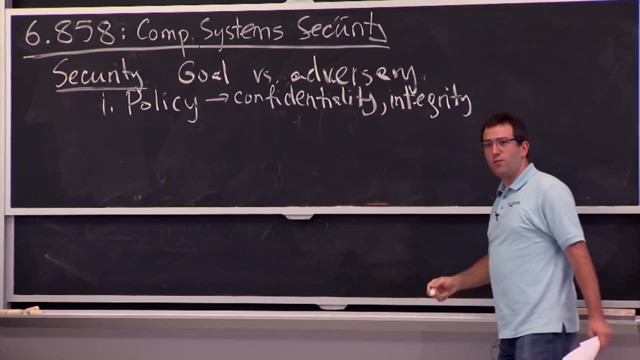 have to do with either confidentiality of data. The grades file is only accessible to the 6858 core staff. Another example of a security policy has something to do with integrity. For example, only the core staff can also modify the grades file, Or only the core staff can upload the final grades. 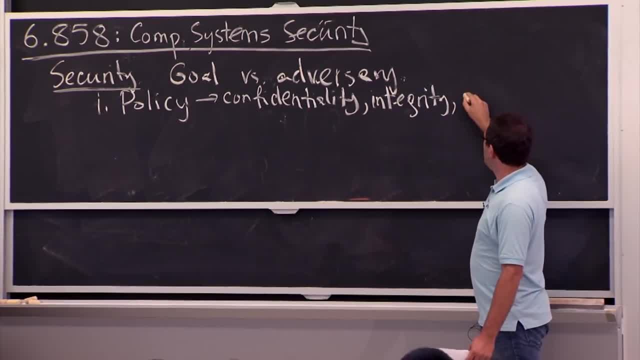 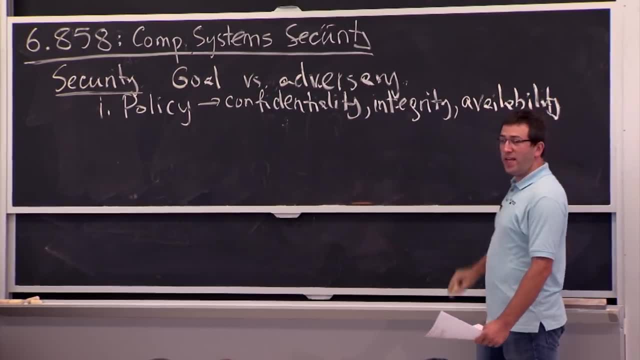 to the registrar's office. That would be great. And you can also think about things like availability. So, for example, a website should be available even if the bad guys try to take it down and mount some sort of a DOS denial of service attack on it. 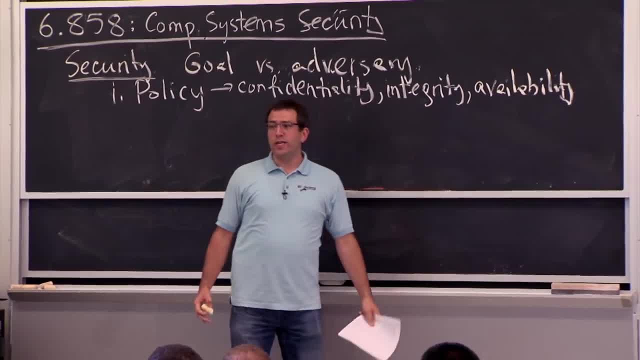 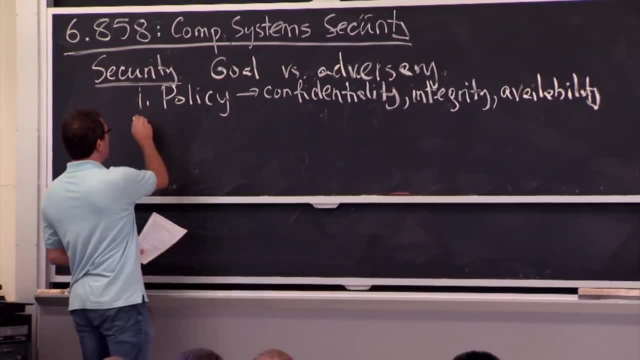 So this is all well and good. So these are the policies that we might actually care about from a system, But because of security, there's a bad guy involved. We need to understand what are we thinking the bad guy is going to do? 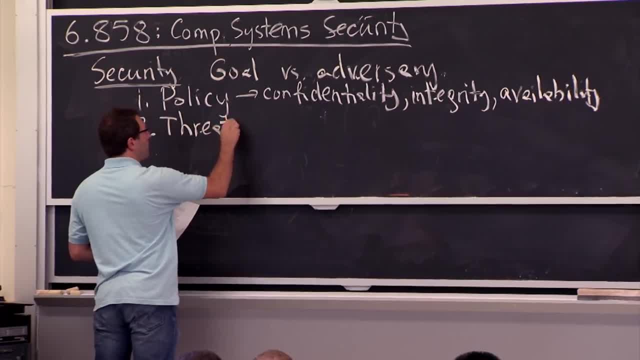 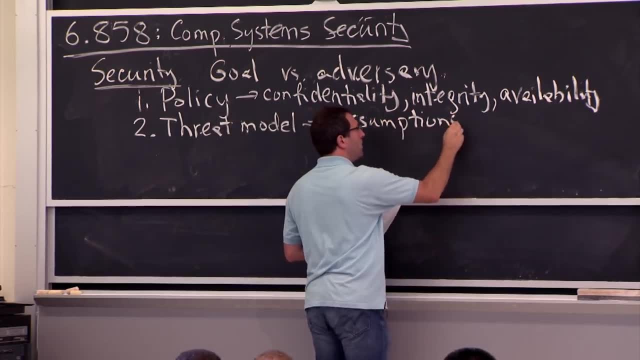 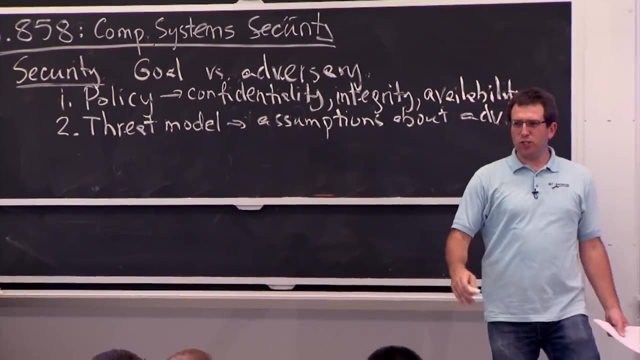 And this is typically what we call a threat model, And this is basically just a set of assumptions about the bad guy, about our adversary. And it's important to have some sort of assumptions about the bad guy, Because if the bad guy is omnipresent, 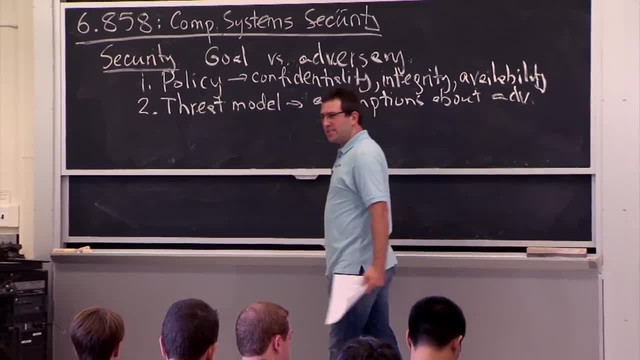 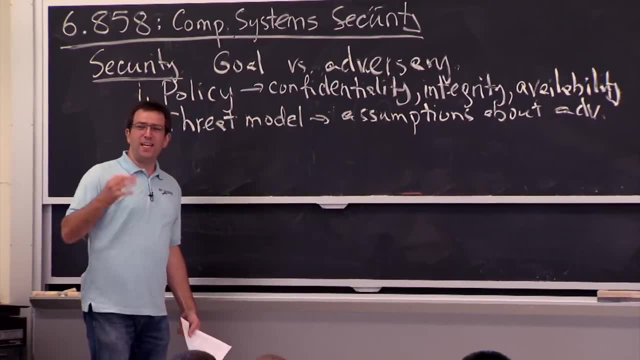 and is everywhere at once and can do anything they want. it's going to be hard to achieve some semblance of security. So, for example, you probably want to assume the bad guy doesn't exactly know your password, Or they don't actually have physical access to your phone. 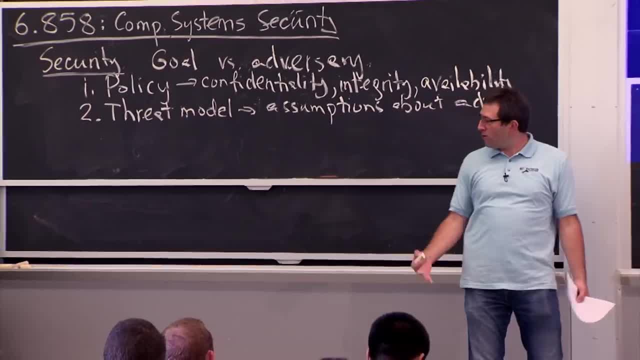 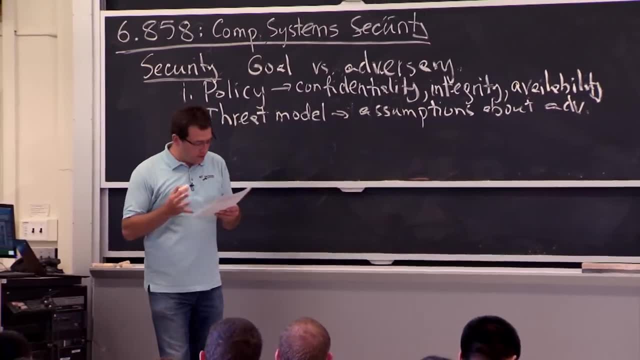 and your keys and your laptop. Otherwise, it's going to be hard to make some sort of progress in this game, And it turns out that, well, this is actually quite tricky to come up with, but I guess one general rule is. 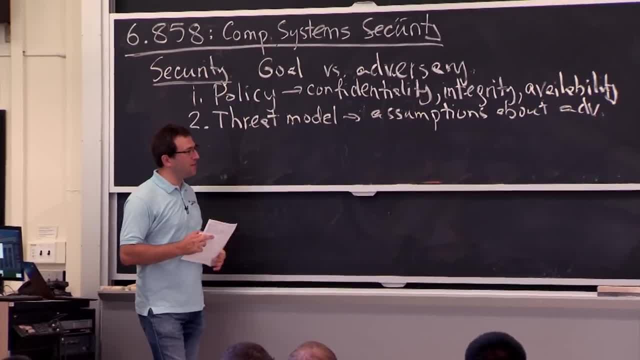 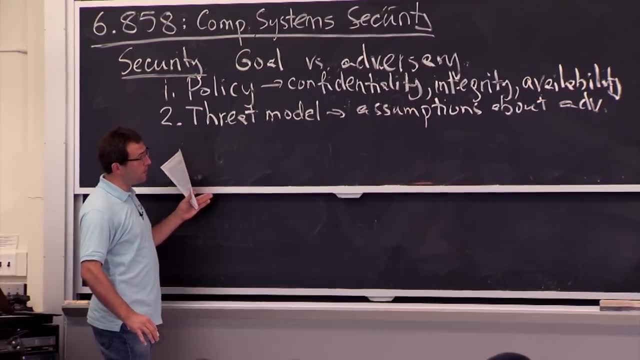 it's much better to err on the side of caution and being conservative in picking your threat model, Because the bad guy might always surprise you in terms of what they might be able to do in practice. And finally, in order to achieve security, in order to achieve our goal under these set of assumptions, 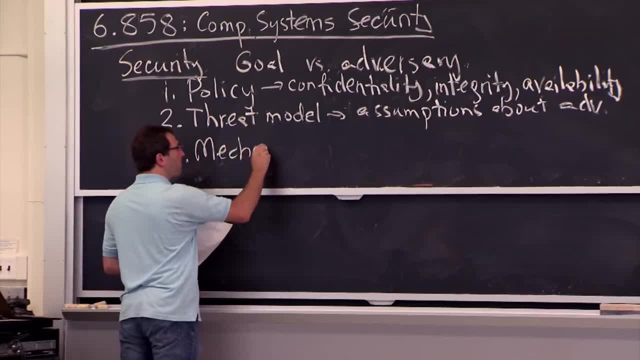 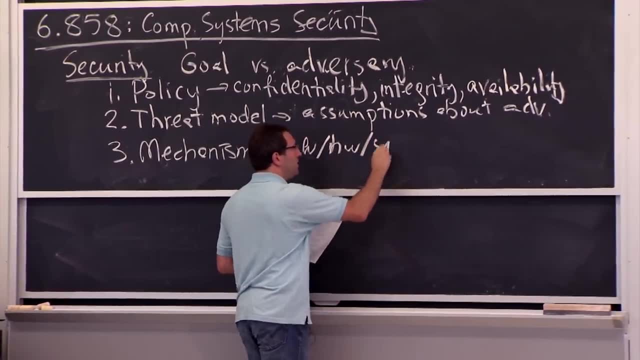 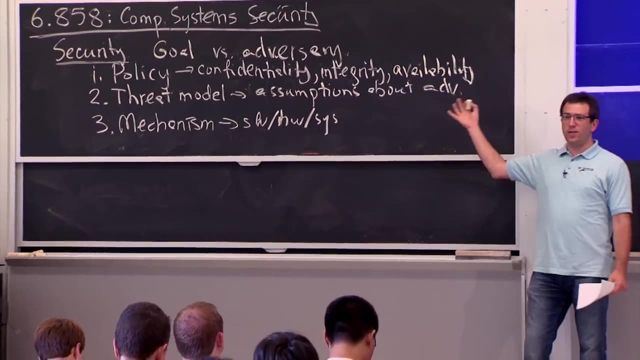 we're going to look at some mechanism, And this is basically software or hardware or whatever part of system: design, implementation et cetera. That's going to try to make sure our policy is followed, as long as the bad guy follows the threat model. 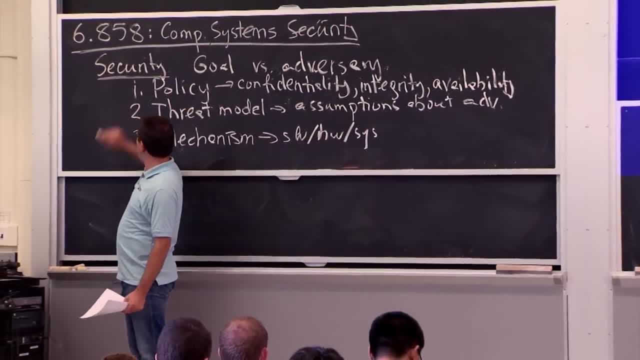 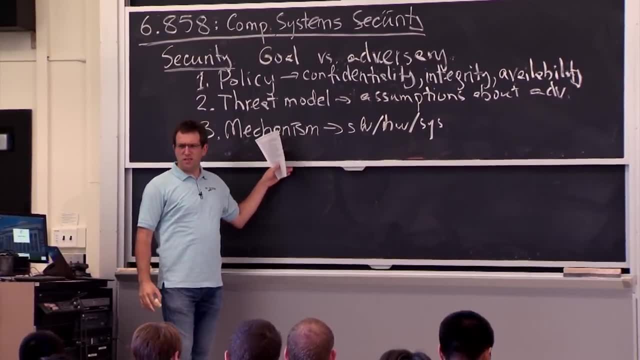 So the end result is that, as long as our threat model was correct, hopefully it will satisfy our policy- And it has to be the case that the mechanism doesn't screw up Make sense. Fairly high level story about how to think about this kind of stuff. 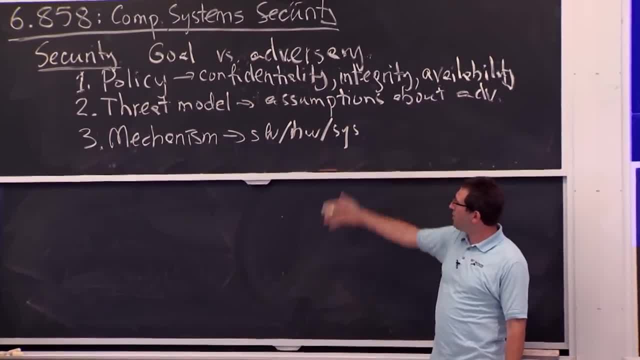 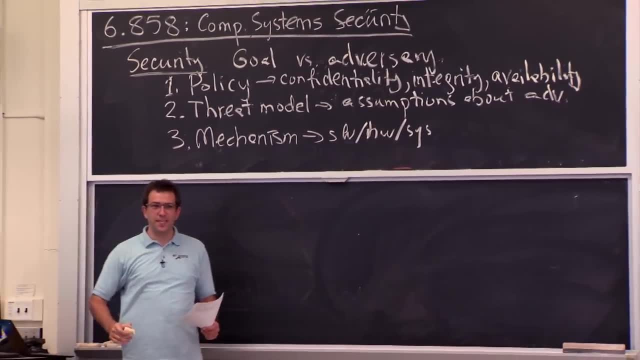 So why is this so hard? It seems like a simple plan, like you write down these three things And you're off and running. But in practice, as you I'm sure have seen in the world, computer systems are almost always compromised in some way or another. 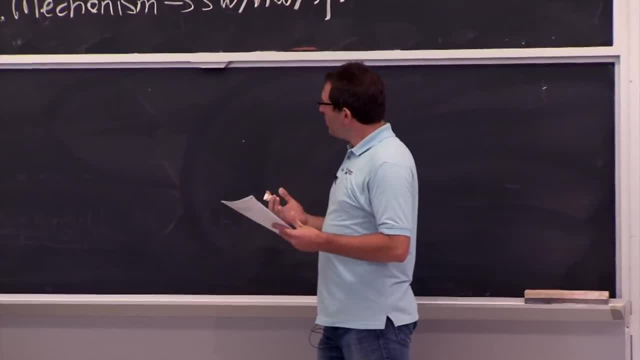 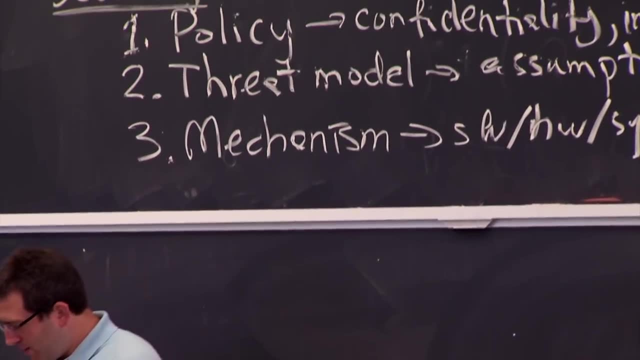 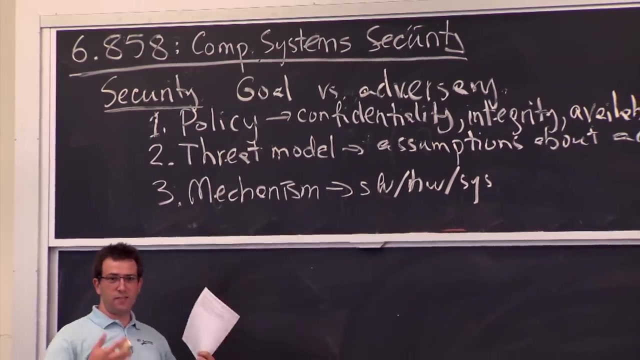 And break-ins are pretty commonplace, And the big reason why security tends to be a difficult problem is because what we have here is sort of: this will be familiar to those of you who do 6033,. this is a negative goal, Meaning that we have to make sure our security policy is. 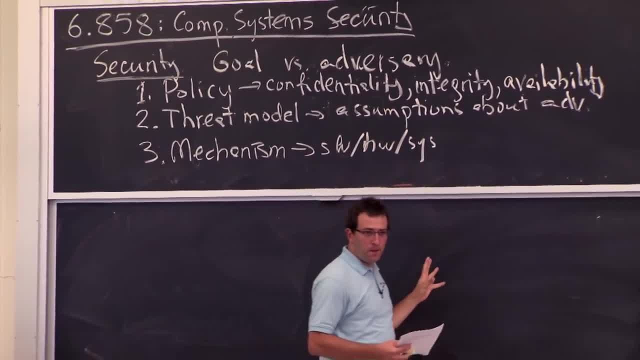 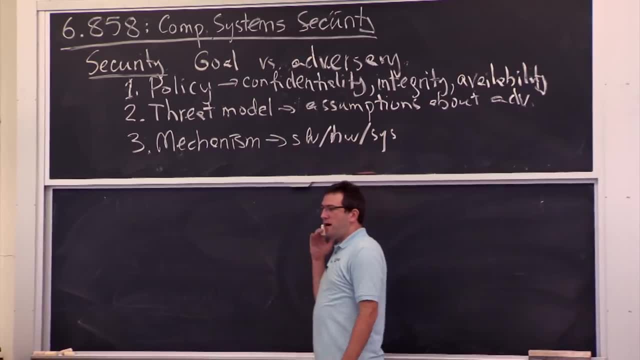 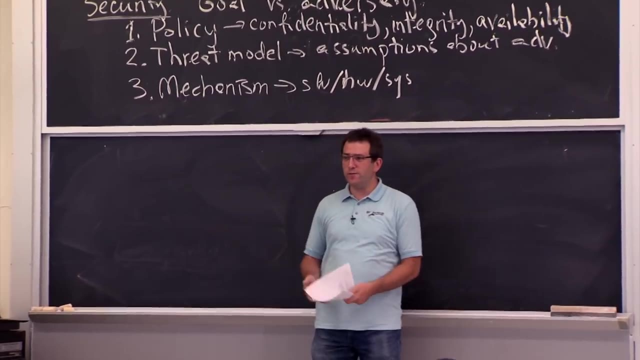 followed, regardless of what that has to do with what the hacker can do. So just by contrast, if you want to build a file system and you want to make sure that my TAs can access the grades file, that's pretty easy. I just ask them: hey, can you guys test and see? 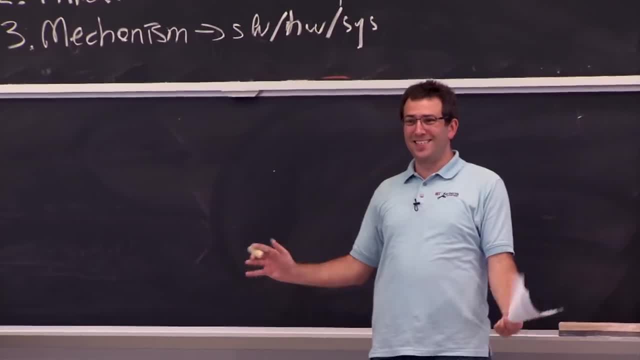 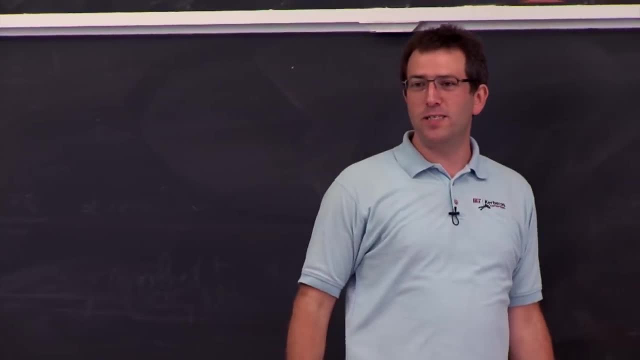 Can you access the grades file And if they all can access it, done, The system works. But if I want to say that no one other than the TAs can access the grades file, this is a much harder problem to solve, Because now I have to figure out what could all these non-TA 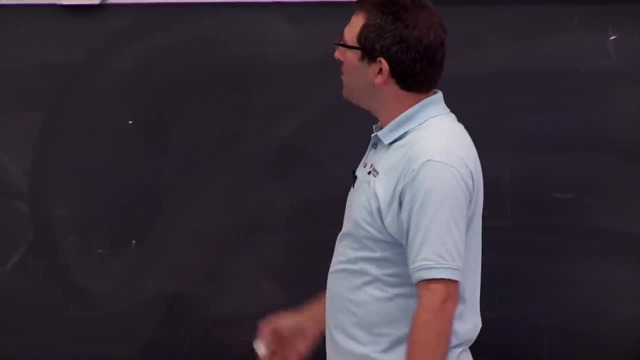 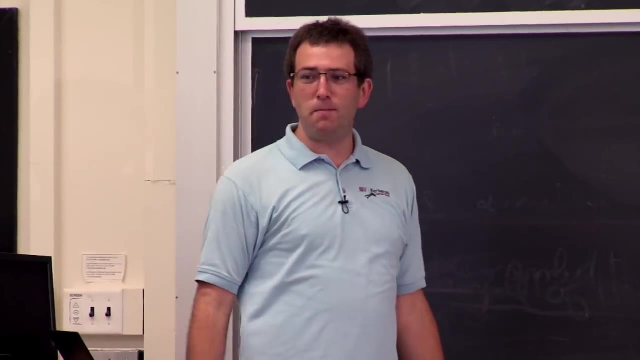 people in the world try to do to get my grades file. They could try to just open it and read it. Maybe my file system will disallow it. But they might try all kinds of other attacks, like guessing the password for the TAs. 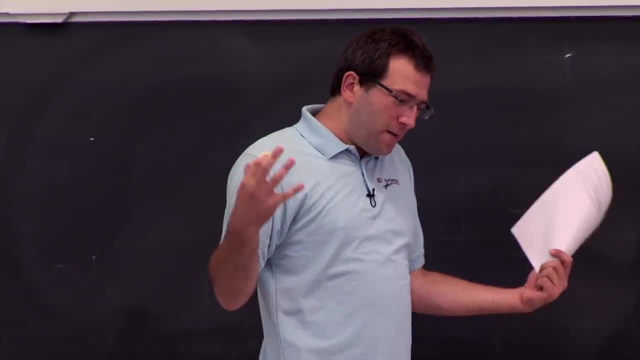 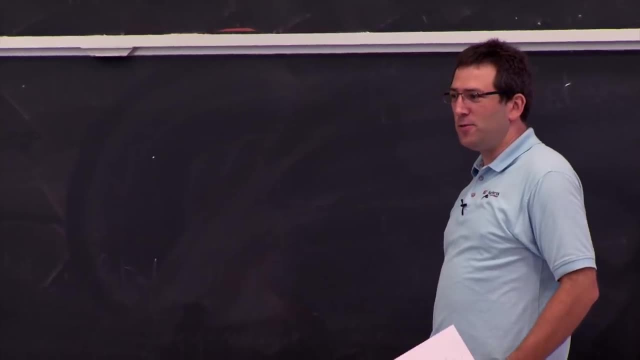 or stealing the TAs' laptops or breaking into their room or who knows. This is all stuff that we have to really put into our threat model, Probably for this class. I'm not that concerned about the grades file to worry about these guys' laptops being stolen. 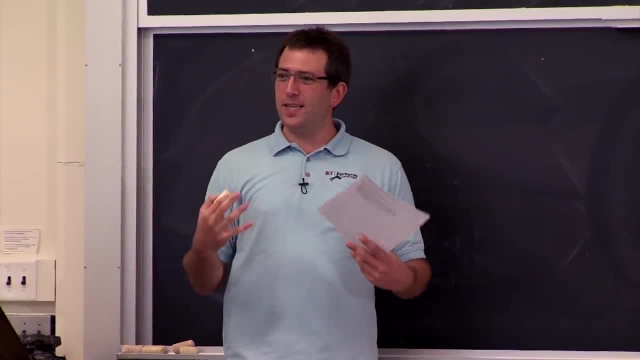 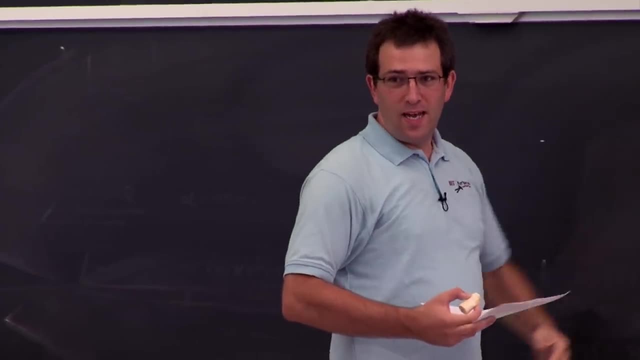 from their dorm room, Or maybe I should be, I don't know- And as a result, this security game is often not so clear cut as to what the right set of assumptions to make is, And it's only after the fact that you often realize. well, 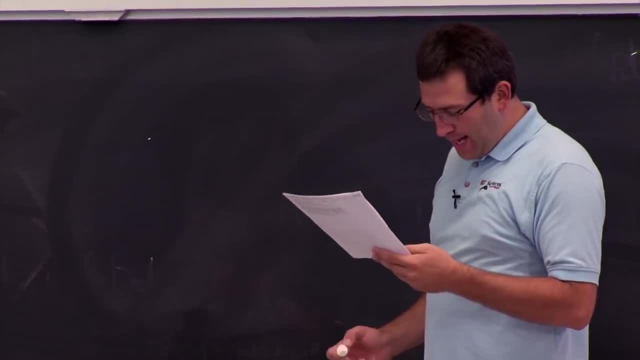 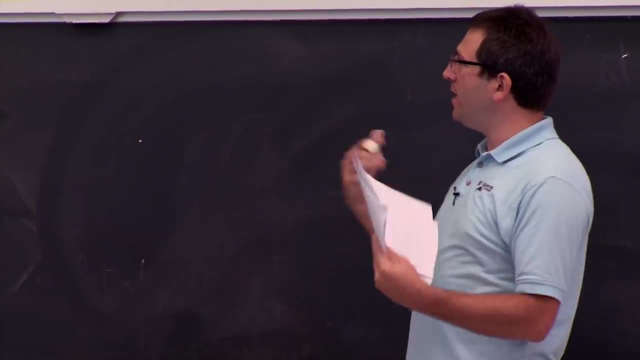 I should have thought of that All right And sort of. as a result, this is very much an iterative process, And the thing you end up realizing at every iteration is: well, here's the weakest link in my system. Maybe I got the threat model wrong. 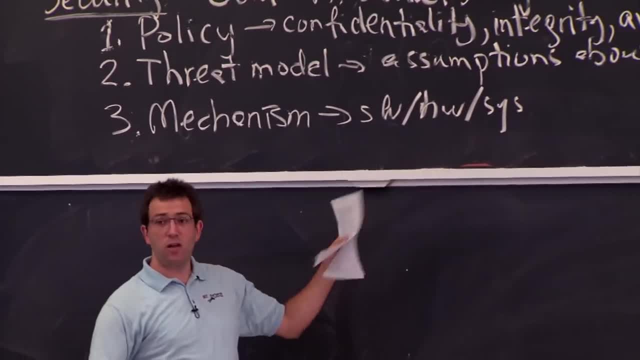 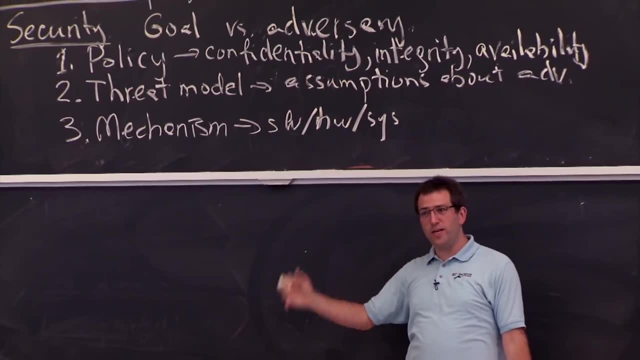 Maybe my mechanism had some bugs in it. because of software and it's going to be large systems, They'll have lots of bugs And you sort of fix them up. You change your threat model a bit And you iterate and try to design a new system. 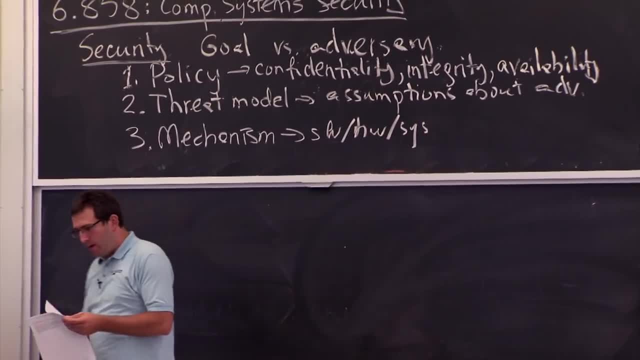 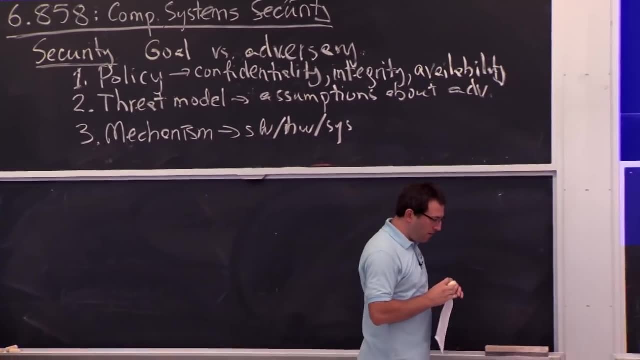 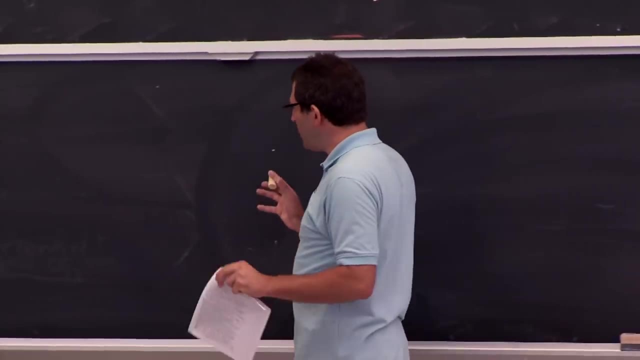 And hopefully make things better. So one possible interpretation of this class, or one danger, is that you come away thinking man, everything is just broken, Nothing works, We should just give up and stop using computers. And this is like one possible interpretation. 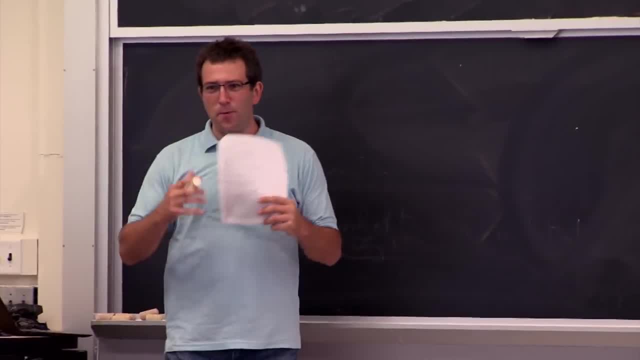 but it's probably not quite the right one. The reason this is going to happen, or you're going to think this way, is because throughout this class, we're going to look at all these different systems And we're going to sort of push them to the edge. 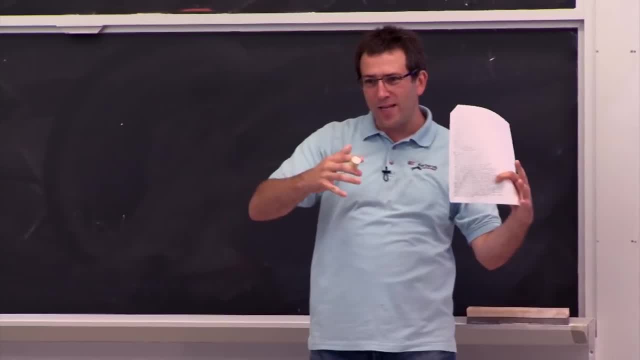 We're going to see: OK, well, what if we do this? Is it going to break? What if we do that? Is it going to break then? And inevitably, every system is going to have some sort of a breaking point. 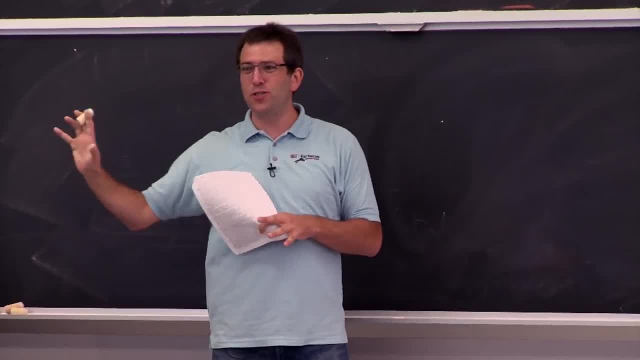 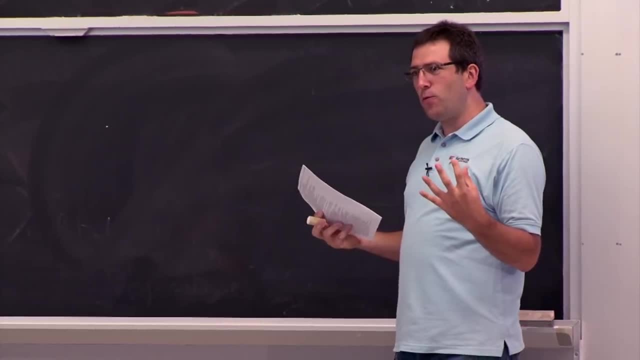 And we'll figure out: oh hey, this system, we can break it if we push this way And the system doesn't work under these set of assumptions. And it's inevitable that every system will have a breaking point. but that doesn't mean that every system is worthless. 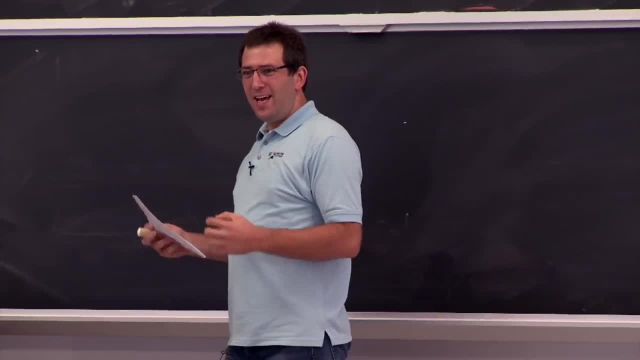 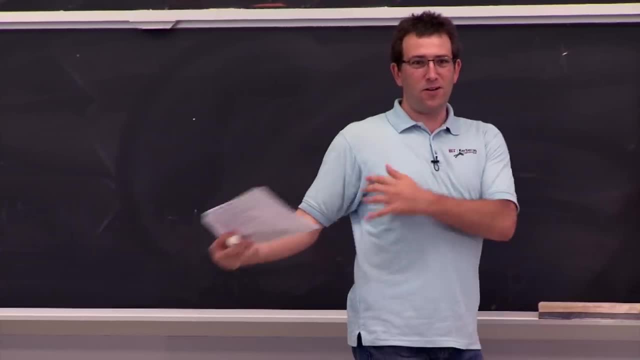 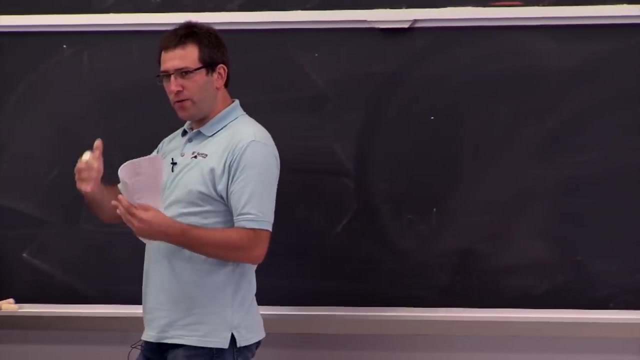 It just means you have to know when to use every system design, And it's sort of useful to do this pushing exercise to find the weaknesses, so that you know when certain ideas work, when certain ideas are not applicable. And in reality this is a little bit of a fuzzy boundary. The more secure you make your system, the less likely you'll have some embarrassing story on the front page of New York Times saying your startup company leaked a million people's social security numbers And then you pay less money to recover from that disaster. 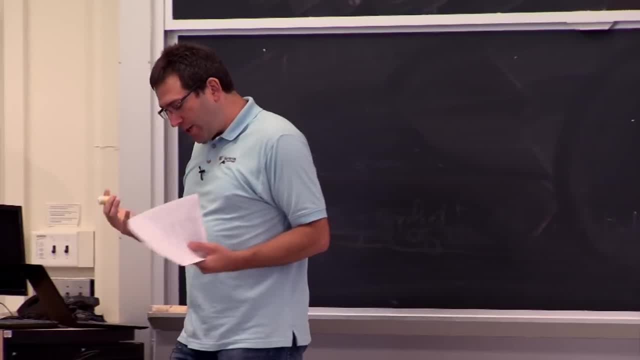 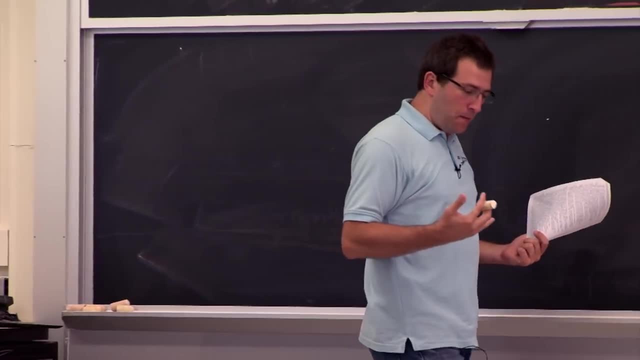 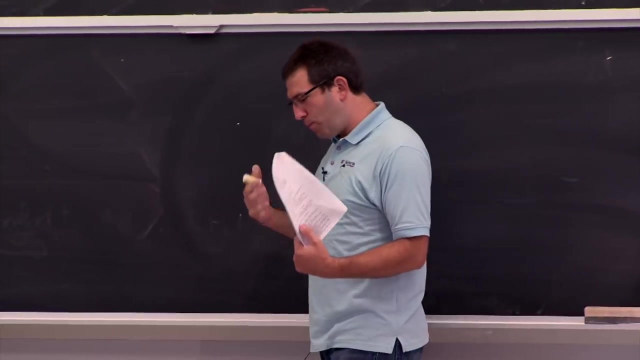 And I guess one sort of actually positive note on security is that in many ways security enables cool things that you couldn't do before, Because security, especially mechanisms that allow us to protect against certain classes of attacks, are pretty powerful. As one example, the browser used to be fairly boring in terms. 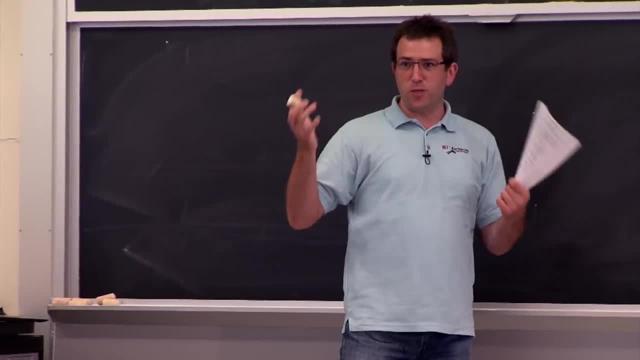 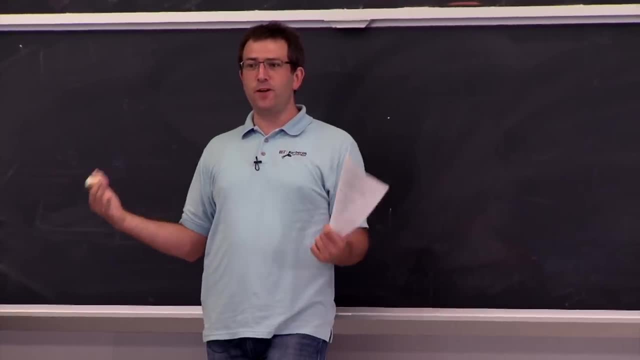 of what you could do with it. You could just view web pages, maybe run some JavaScript code in it, But now there's all these cool mechanisms- we'll learn about in a couple of weeks- that allow you to run arbitrary x86 native code in the web browser. 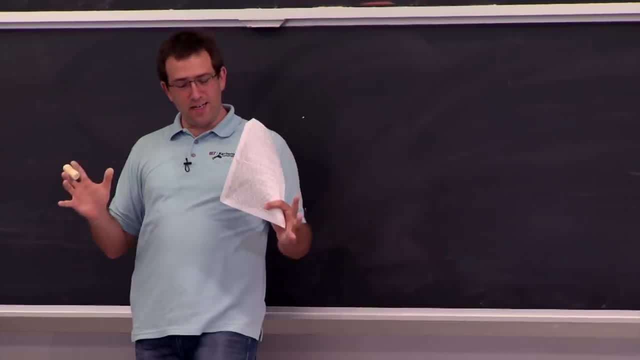 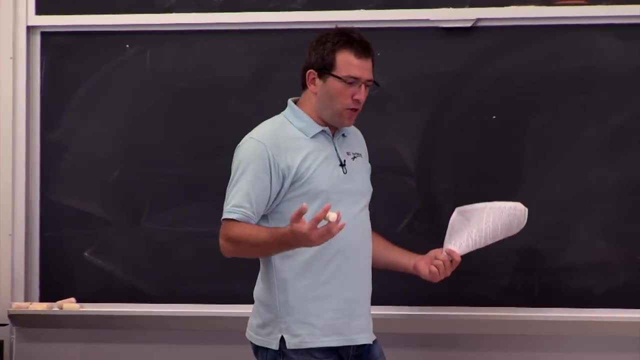 and make sure it doesn't do anything funny to your machine, And there's a technique or system called native client from Google that actually allows us to do this securely And before. in order to run some native game on your machine, you have to download and install it. click on lots of dialog. 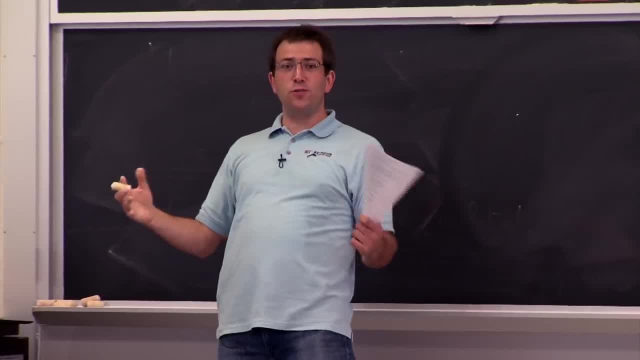 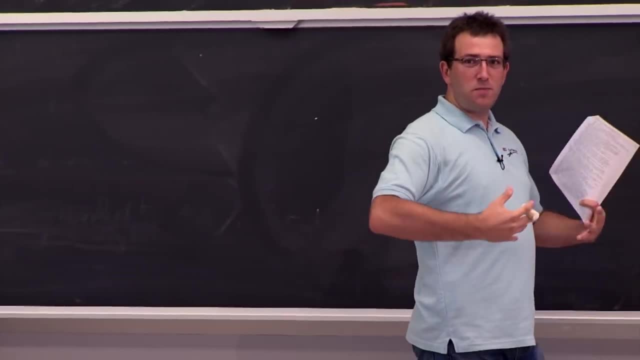 boxes say: yes, I allow this, But now you can just run it in a browser, No clicking required, It just runs, And the reason it's so easy and powerful is that our security mechanism. You can sandbox this program and not have to assume anything about the user choosing the right. 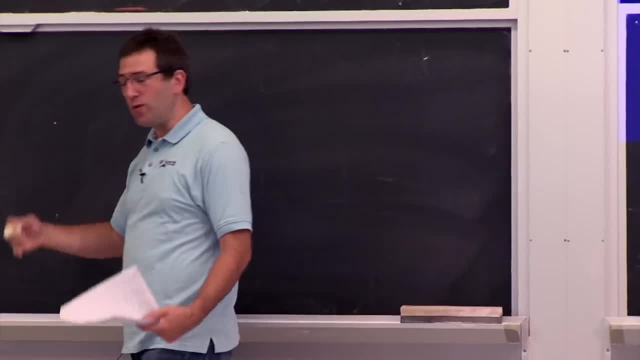 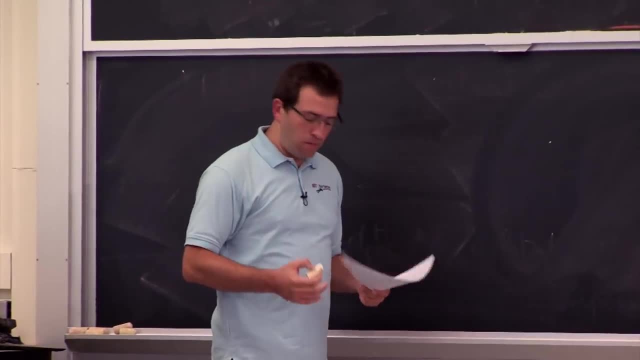 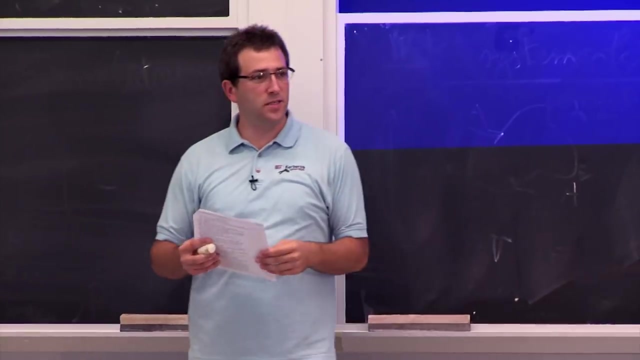 game and not some malicious game to play in their computer or some other program to run. So in many ways good security mechanisms are going to enable constructing cool new systems that weren't possible to construct before. All right, Make sense. Any questions about this story? 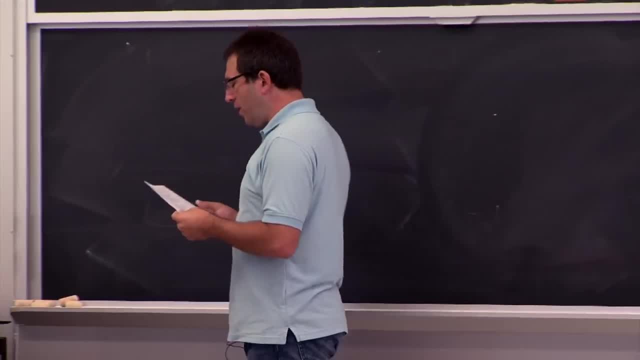 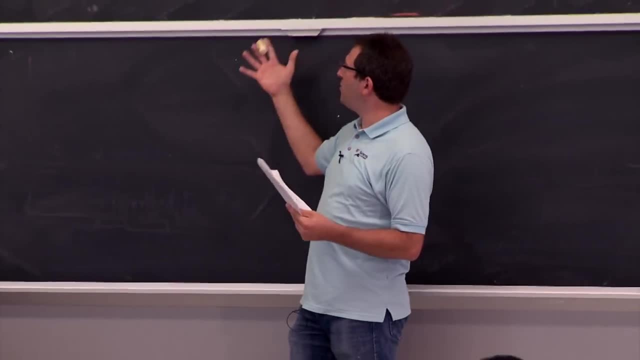 All right. So I guess in the rest of the lecture I want to go through a bunch of different examples of how security goes wrong. So so far we've seen how you can think of it, But inevitably it's useful to see examples of what not to do. 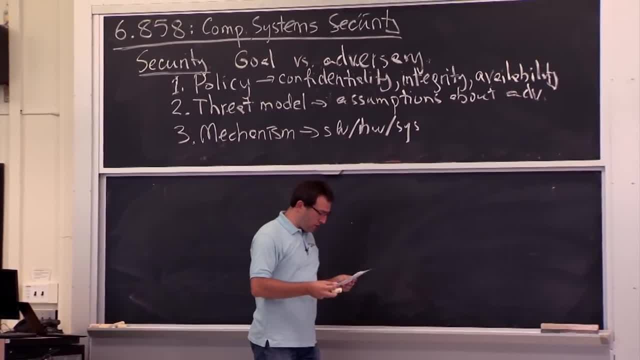 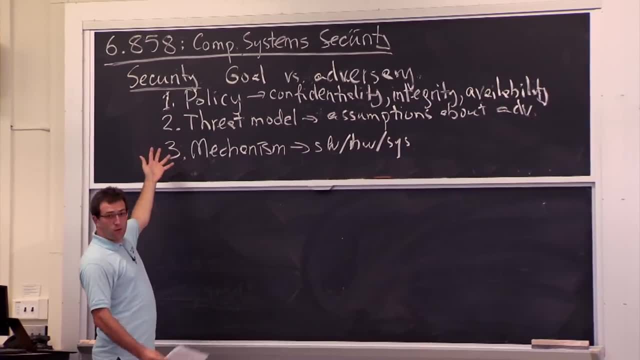 so that you can sort of have a better mindset when you're approaching security problems. And in this sort of breakdown of a security system pretty much every one of these three things goes wrong In practice. people get the policy wrong, People get the threat model wrong. 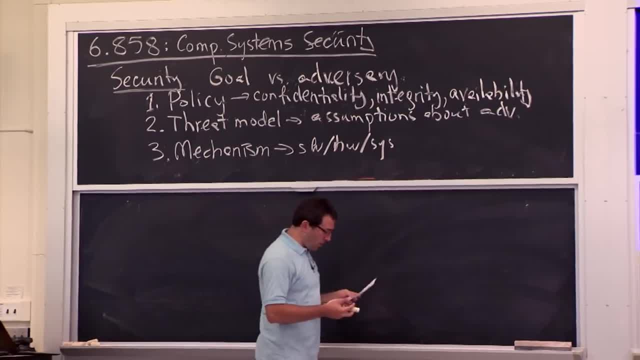 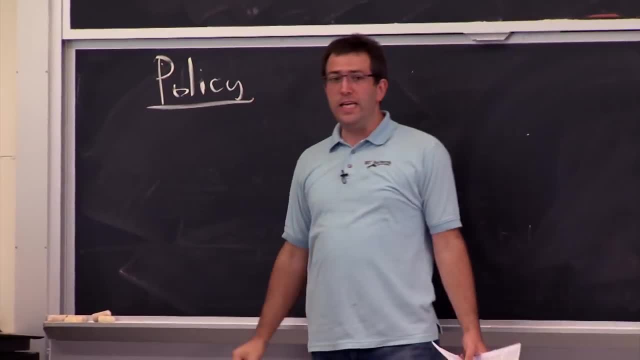 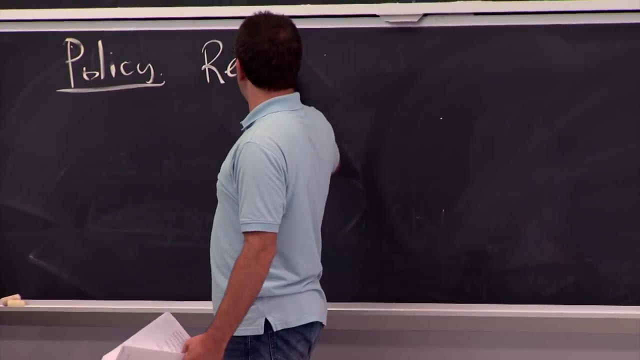 And people get the mechanism wrong. And let's, I guess, start with policies and examples of how you can screw up a system's policy. Maybe the cleanest or sort of simplest example of this are account sort of recovery questions. So typically when you sign into a website, 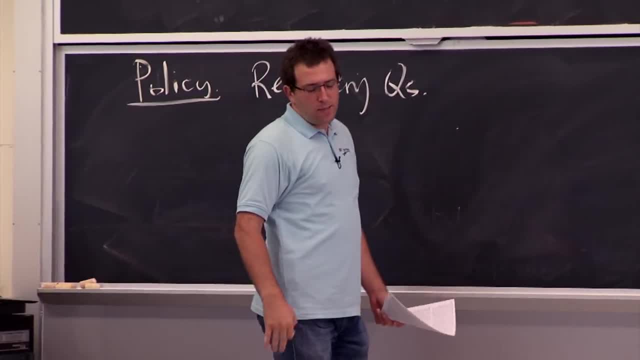 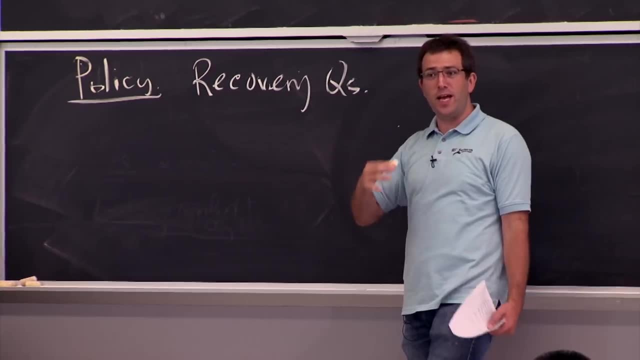 you provide a password, But what happens if you lose your password? Some sites will send you email. if you lose your password with a, you know a link to reset your password. So it's easy enough if you have another email address. 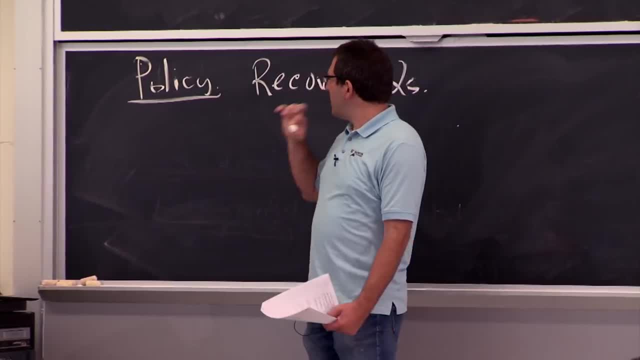 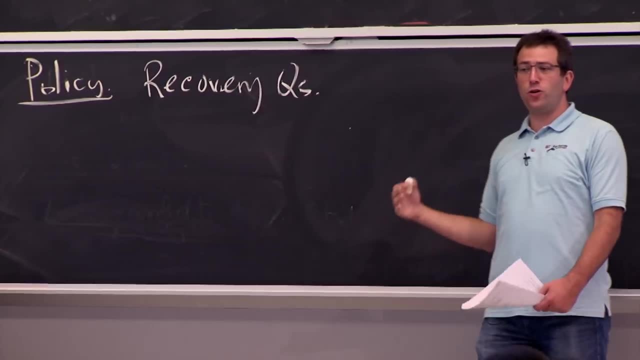 But what if this is your email provider, So companies? well, at least several years ago, Yahoo, you know, hosted email webmail for anyone on the internet, And when you forgot your Yahoo password, they couldn't really send you email. because you couldn't get it. So instead they had you register a couple of questions with them that hopefully only you know, And if you forget your password, you can click on a link and say: well, you know, here's the answers to my questions. 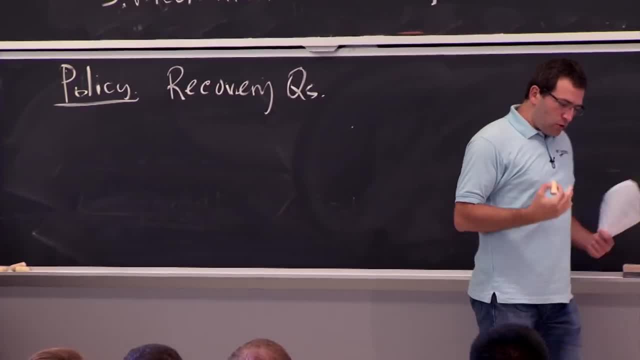 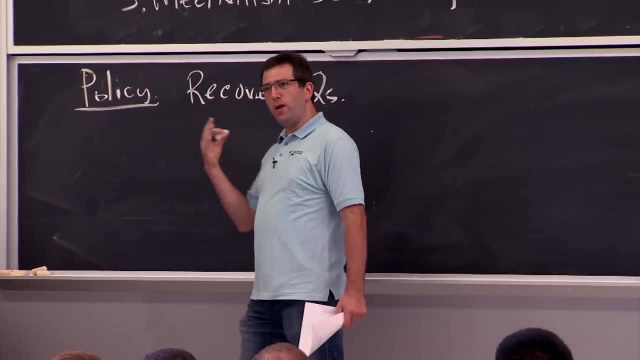 Let me have my password again, And what turns out to be the case is: well, some people fail to realize is that this changes your policy, Because before the policy of the system is people that can log in are the people that know the password. And when you introduce these recovery questions, the policy becomes: well, you can log in if you know either the password or those security questions. So it strictly weakens the security of your system And many people have actually taken advantage of this. One sort of well-known example is, I think: 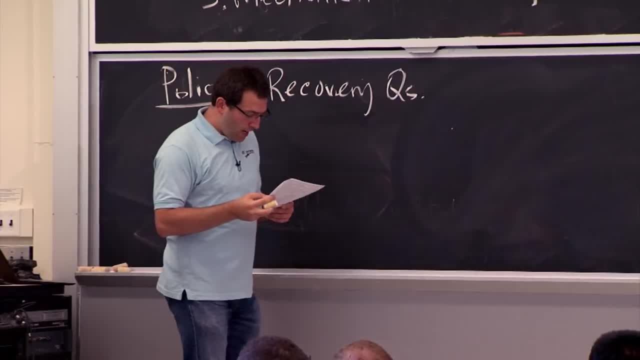 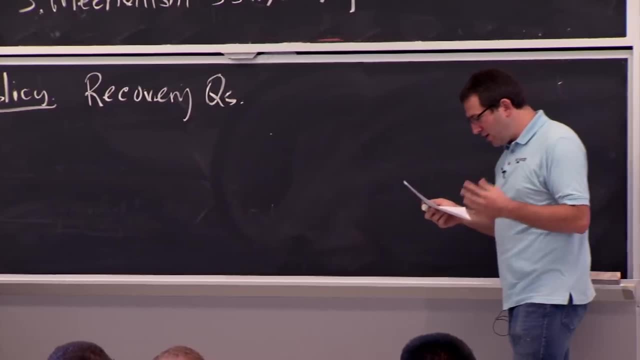 a couple of years ago, Sarah Palin had an email account at Yahoo And her recovery questions were things like: well, where did you go to school, What was your friend's name, What's your birthday, et cetera. These are all things written on her Wikipedia page. 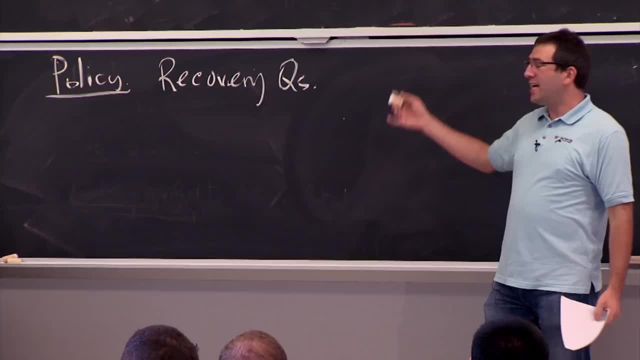 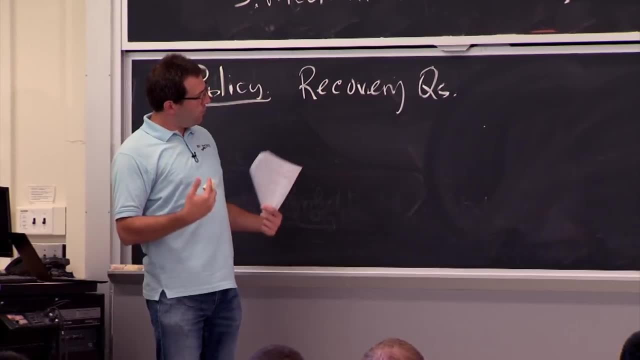 And, as a result, someone can quite easily- and someone did- actually get into her Yahoo email account just by looking up on Wikipedia what her high school was and what her birthday was. So you really have to think carefully about the implications of different security policies. 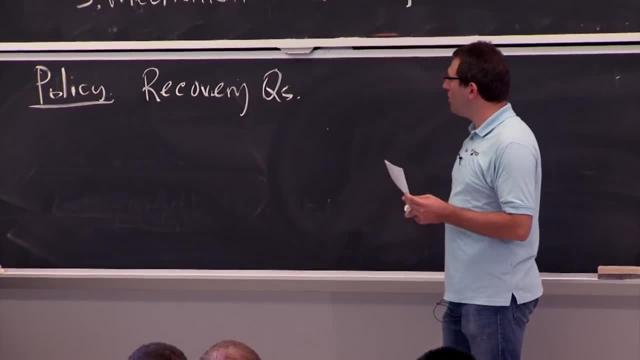 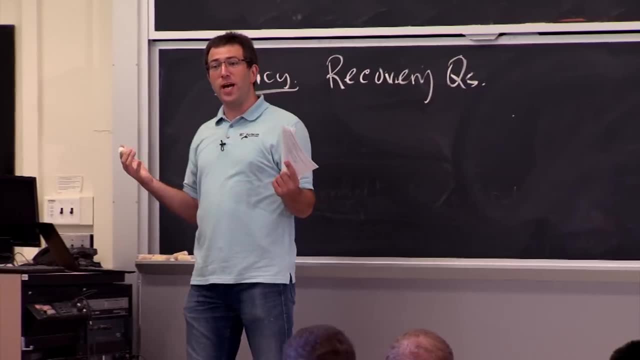 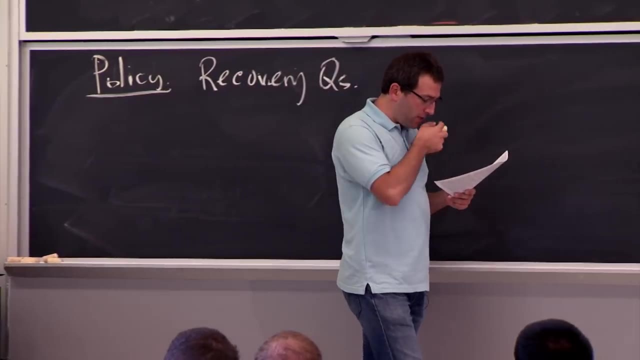 you're making Making here. Perhaps a more intricate and maybe interesting example is what happens when you have multiple systems that start interacting with one another. So there's this nice story about a guy called Matt Honan. Maybe you've read this story a year or two ago. 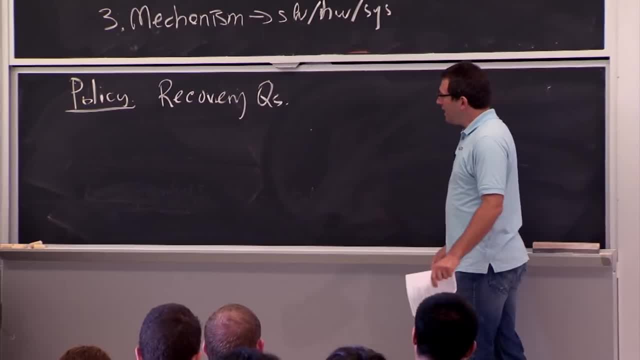 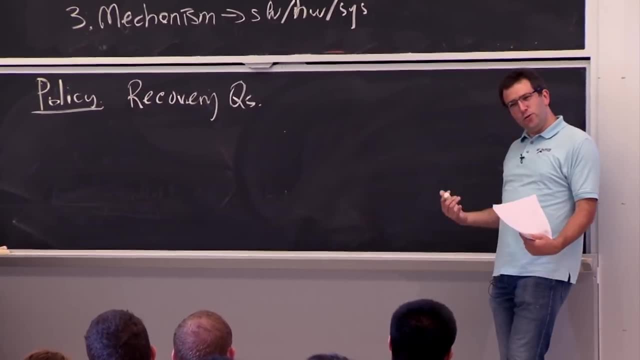 He's an editor at this wirecom magazine And he had a bit of a problem. Someone basically got into his Gmail account and did lots of bad things, But how did they do it? So it's kind of interesting. So all parties in this story seem. 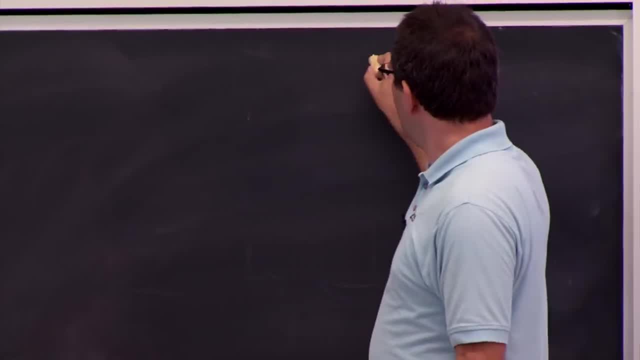 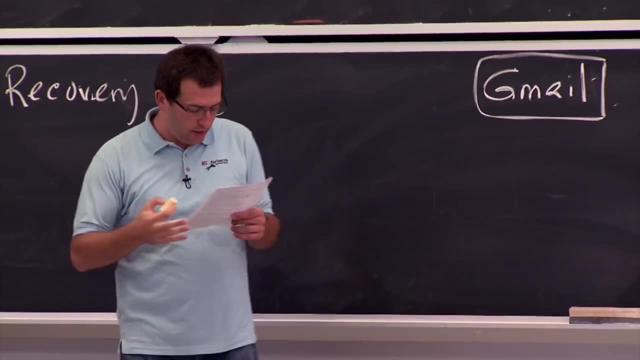 to be doing reasonable things, But we'll see how they add up to something unfortunate. So we have Gmail, And Gmail lets you reset your password if you forget, as do pretty much every other system, And the way you sort of do a reset at Gmail. 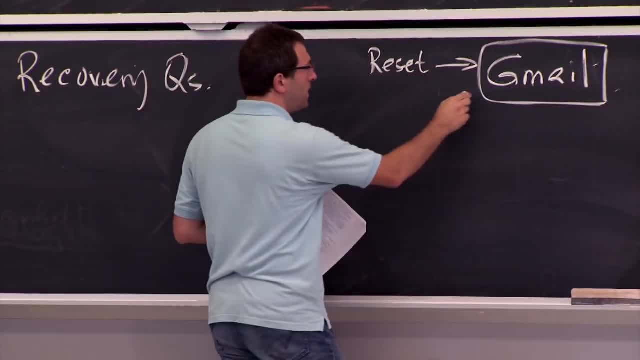 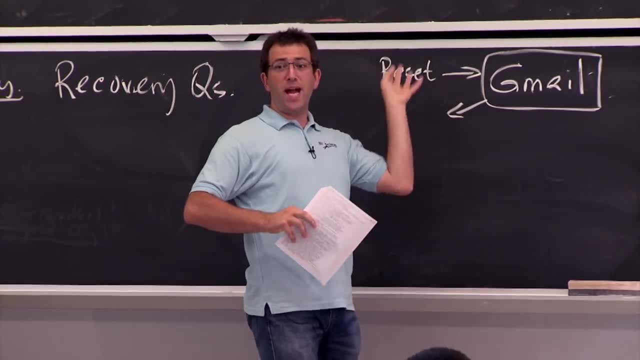 is you send them a reset request And what they say is: well, we're not going to do this recovery questions, at least not for this guy. What they do is they send you a recovery link to a backup email address, So some other email address that you have. 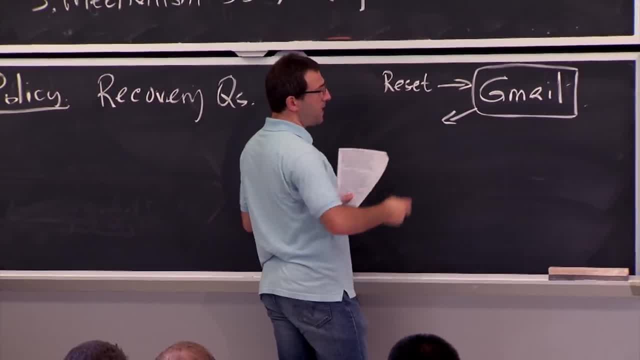 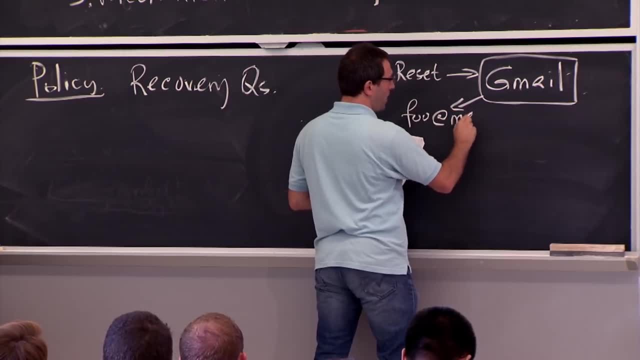 And helpful, they actually print the email address for you. So for this guy's account someone went and asked Gmail to reset the password And they said: well, yeah sure, We just sent the recovery link to this email foo at mecom. 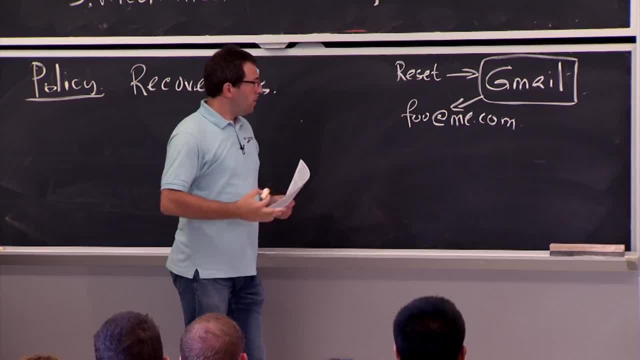 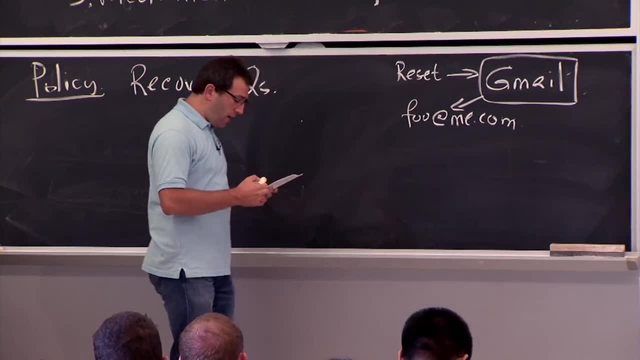 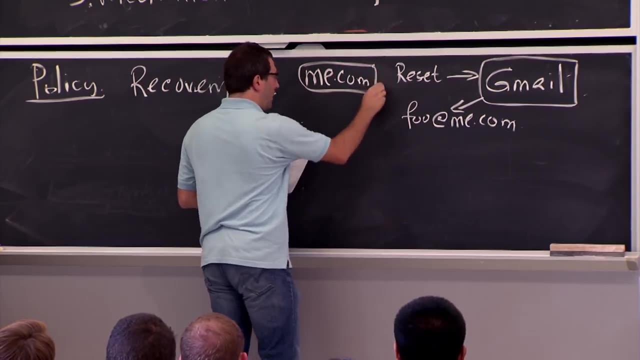 which was some Apple email service. OK, But the bad guy doesn't have access to mecom either. But they want to get this password reset link to get access to Gmail. Well, the way things worked was that, in Apple's case, this mecom site allowed you to actually reset your password. 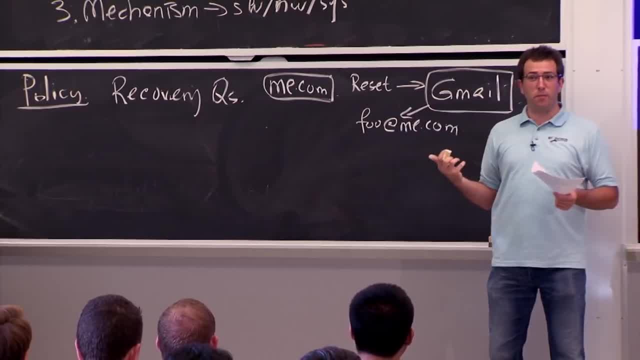 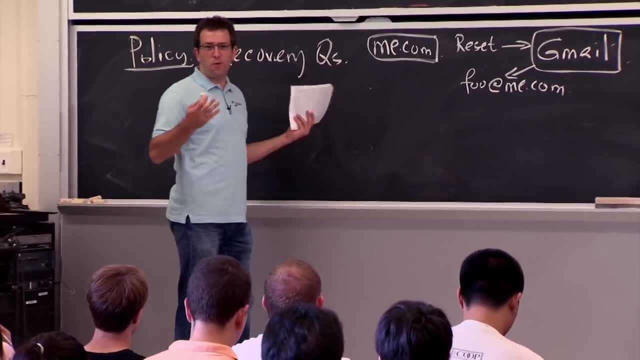 if you know your billing address and the last four digits of your credit card number. So it's still not clear how you're going to get this guy's home address. Maybe you can look it up somewhere. This guy's a well-known person at the time. 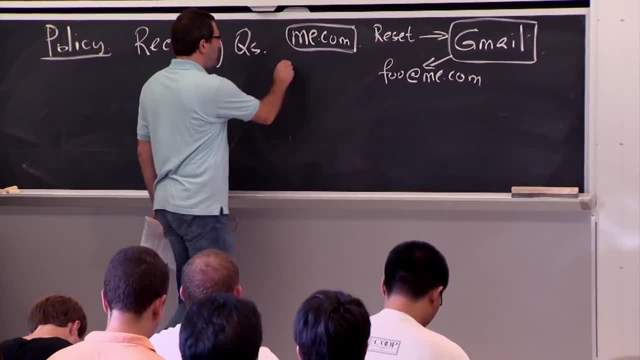 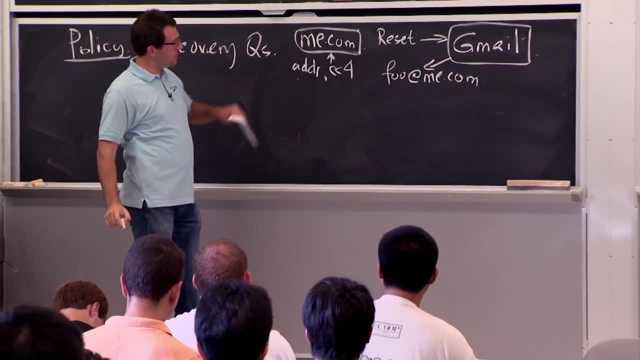 But where do you get the last four digits of his credit card number? Well, not clear, But let's keep going further. So you need to send these things. You need to send these to mecom to get access to his email account there. 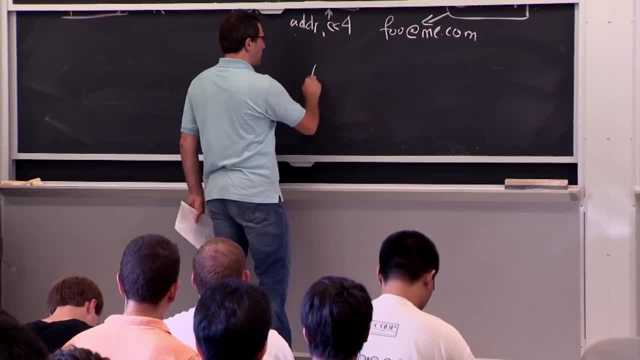 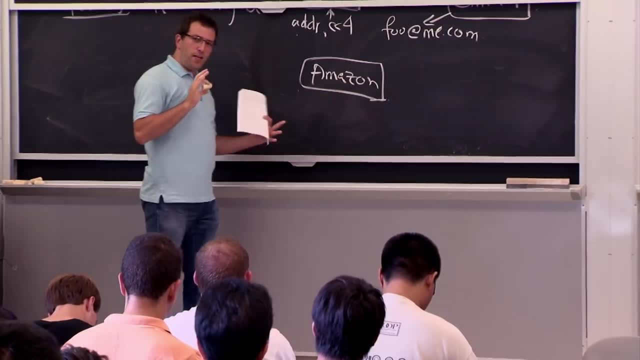 Well, it turns out, this guy had an account at Amazon, which was another party in this story. Amazon really wants you to buy things And, as a result, they actually have a fairly elaborate account management system, And in particular, because they really want you to buy stuff. 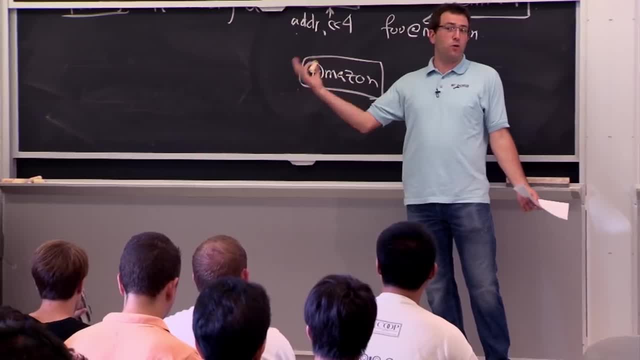 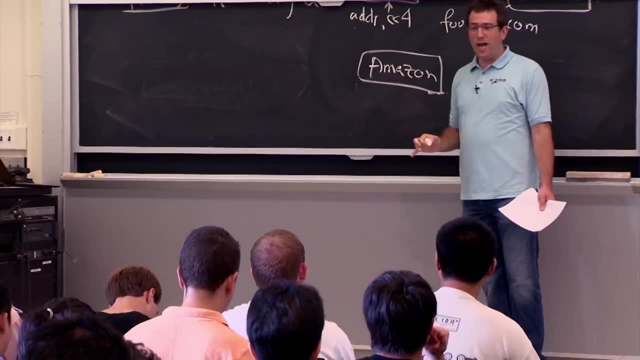 they don't require you to sign in in order to purchase some item with a credit card, So I can actually go on Amazon, or at least at the time I was able to go on Amazon and say, well, I'm this user. 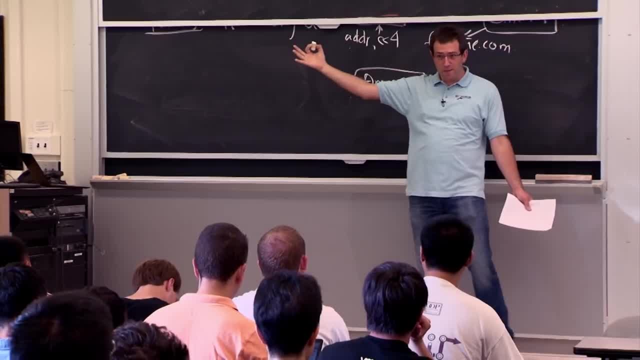 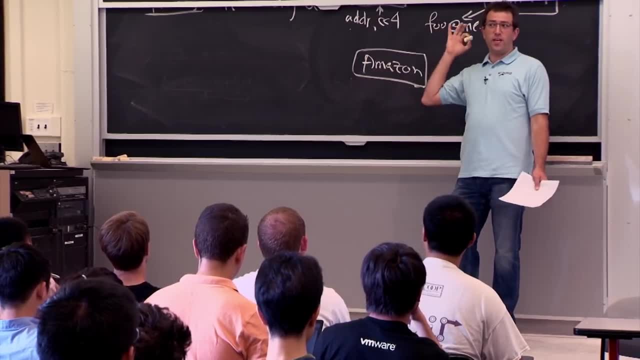 And I want to buy this pack of toothbrushes, And if I wanted to use the saved credit card number in the guy's account, I shouldn't be able to do this. But if I just provide a new credit card, what Amazon would do is they can actually add a new credit. 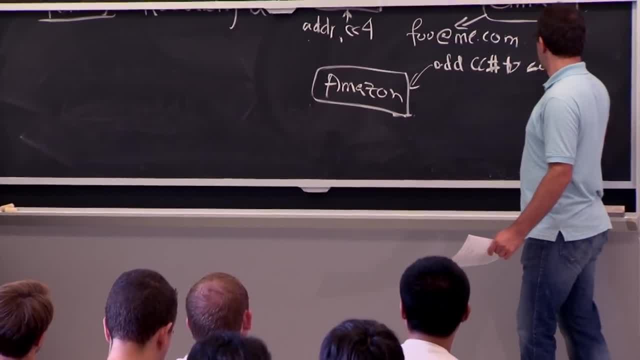 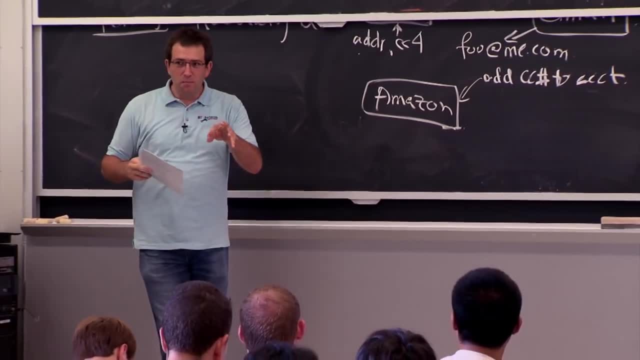 card to some guy's account, So that seems not too bad, right, Like? I'm basically ordering toothbrushes through one of your Amazon accounts, But it's not your credit card anyway, It's just my credit card number being used, So it's not clear how things go wrong yet. But Amazon had another interface. Like all, these are complicated systems And Amazon had an interface for password reset, And in order to reset a password in Amazon, what you had to provide is just one of the user's credit card numbers, So I can order stuff and add a credit card number. 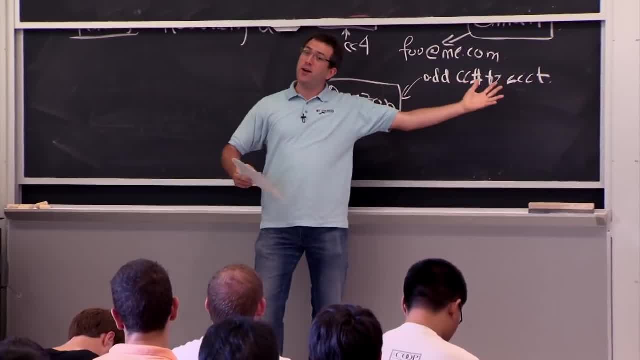 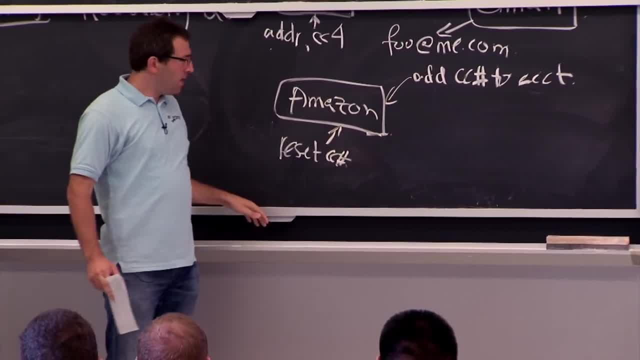 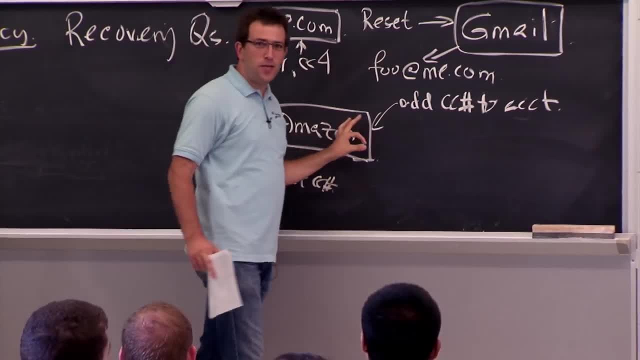 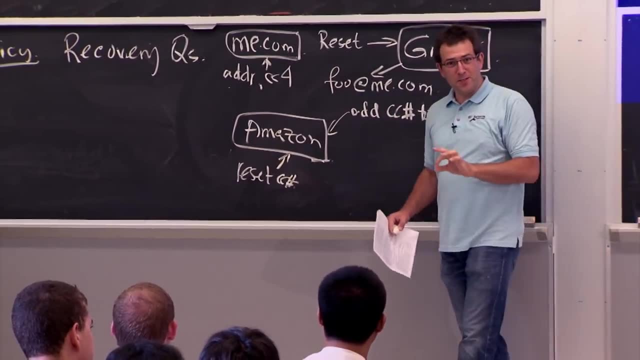 Well, Amazon was actually very careful. Even if you break into someone's Amazon account, it will not print you the saved credit card numbers from that person, But it will show the last four digits, just so you know which credit card you're talking about. 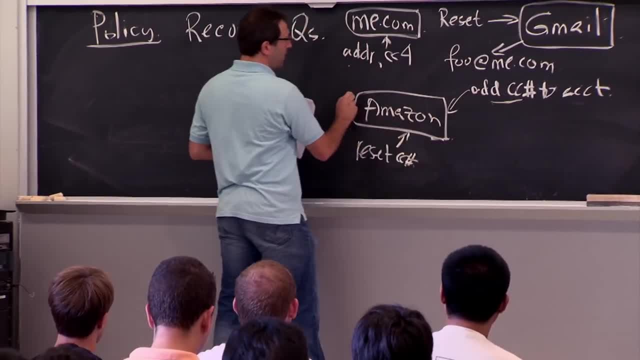 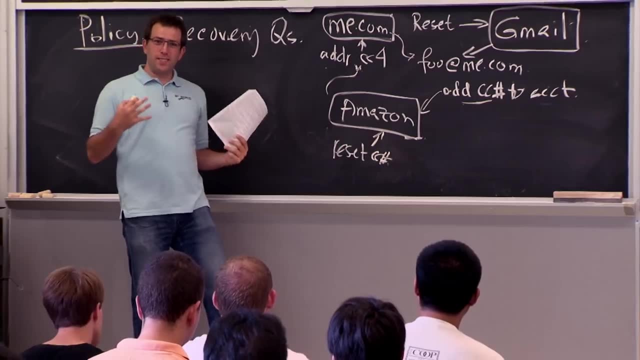 So you can list all the credit cards other than the one you added. You can then go and break into mecom. You can click on this link and get access to the guy's Gmail account. It's all very subtle stuff, stuff, And in isolation each system seems. 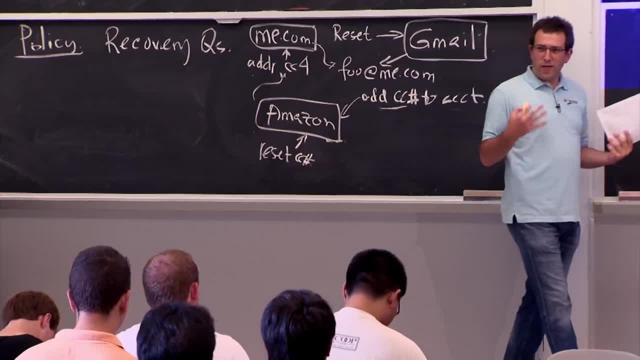 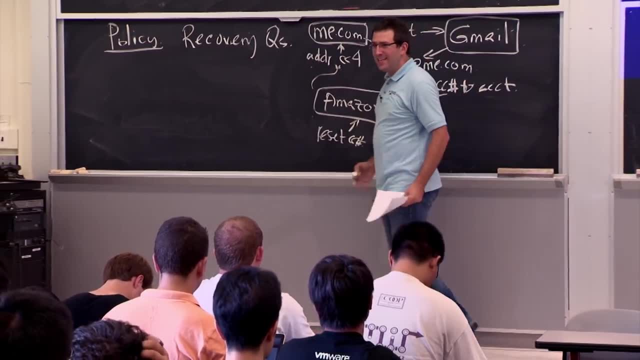 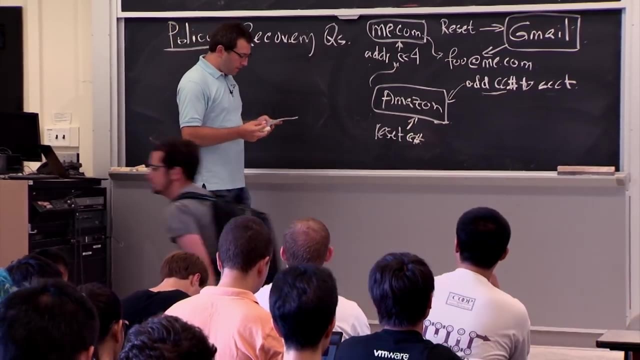 to be doing somewhat sensible things, But it's actually quite hard to reason about these vulnerabilities and weaknesses unless you have this whole picture explained to you and you put all the pieces together. So this is actually fairly tricky stuff And, unfortunately, much like for every one of these three. 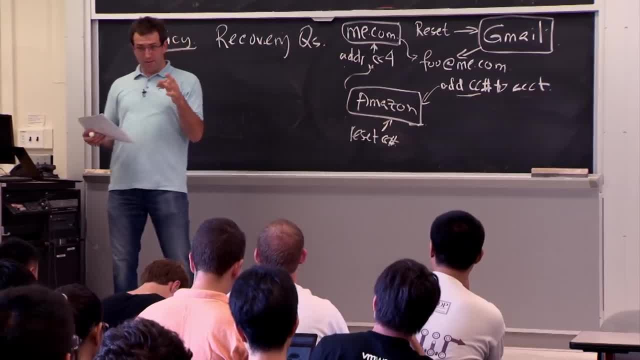 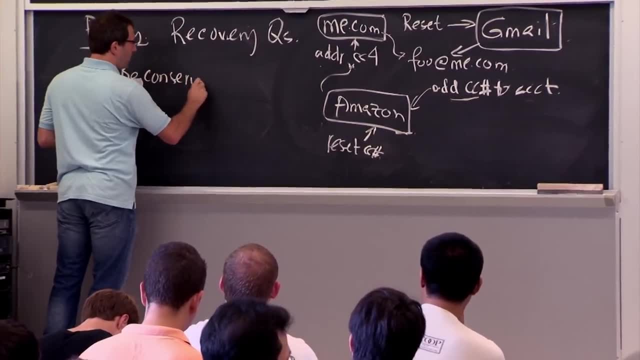 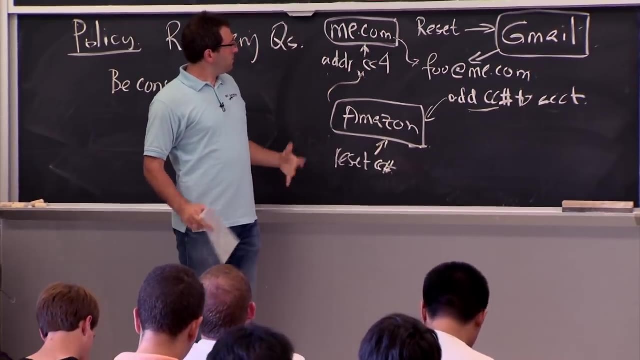 categories. the answer for how to avoid this is often think hard and be careful. I guess the one general plan is: be conservative in terms of what you set your policy to be, to maybe not depend on things other sites might reveal So well. I'm not sure if any really great advice. 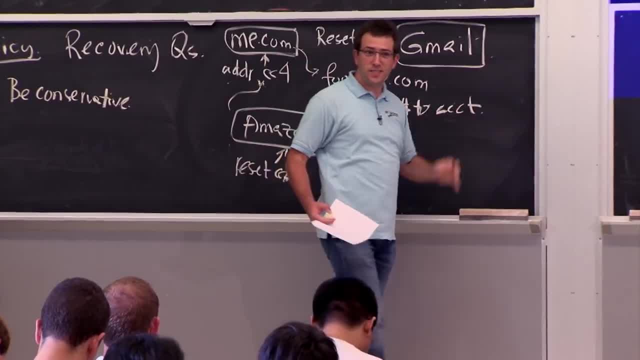 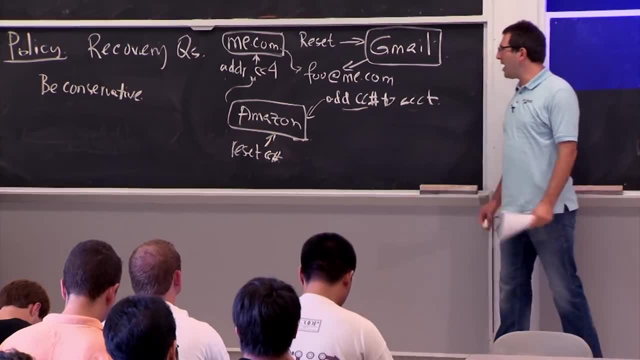 would have prevented this problem. But now you know, and now you'll make other mistakes. There are sort of many other examples of policies going wrong and allowing a system to be compromised. That's interesting enough, but let's look at how Some people might screw up threat models. 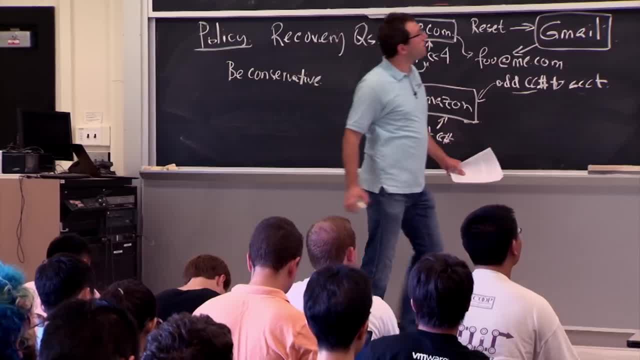 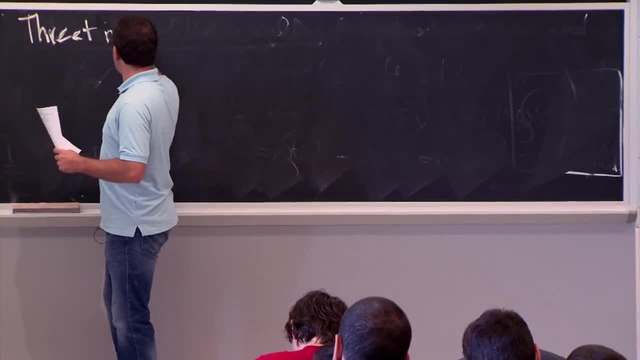 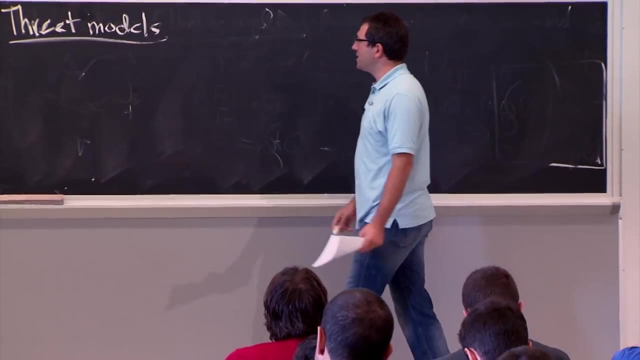 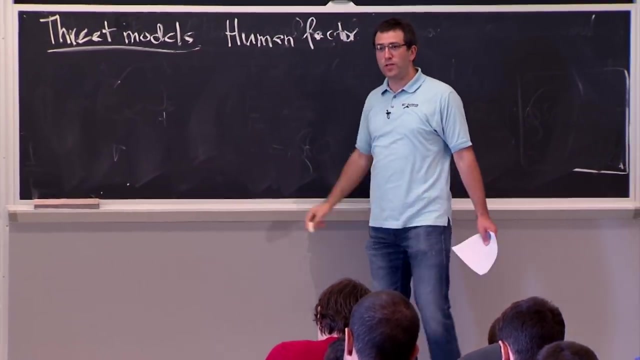 So let me maybe turn off this blue square. So what are examples of threat models that go wrong? Well, probably a big one in practice is human factors. So we often make assumptions about what people will do in a system, Like they will pick a good, strong password. 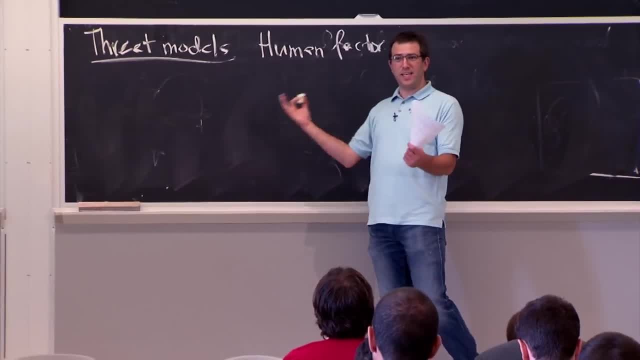 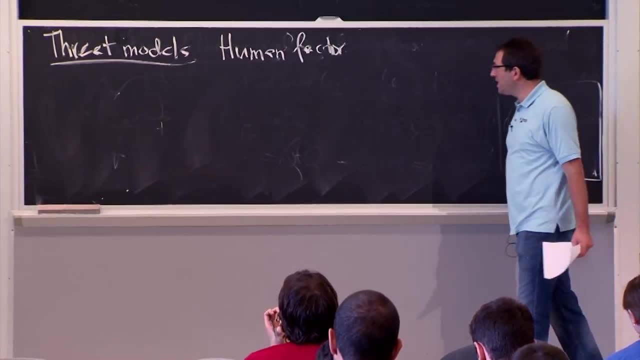 Or they will not click on random websites that they get through email and enter their password there. So these are well, as you probably suspect, and in practice happens to be the case, these are not good assumptions in all cases And people pick bad passwords. 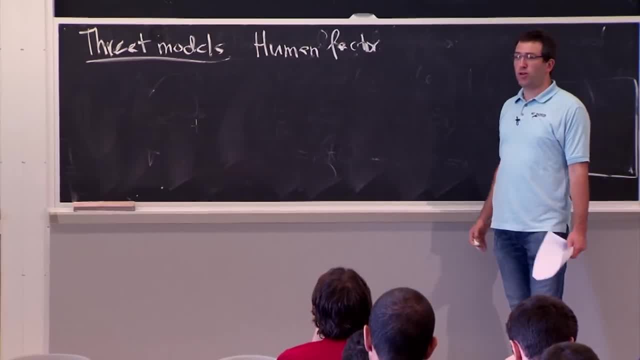 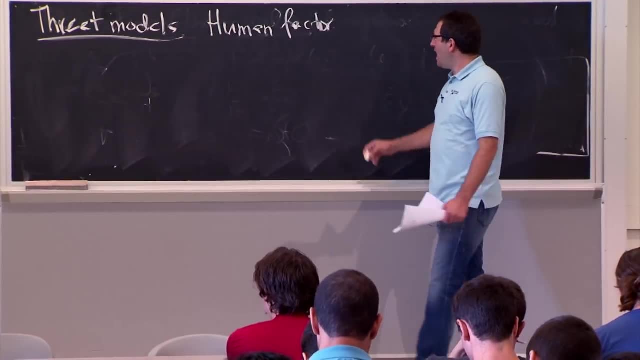 And people will click on random links And people will enter their passwords on sites that are actually not the right site at all And they will not be paying a lot of attention. So you probably don't want to have threat models that make very 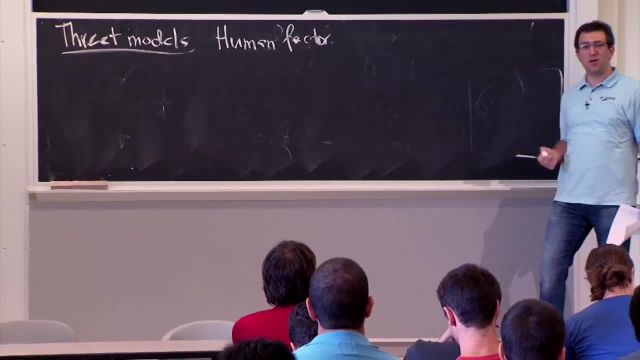 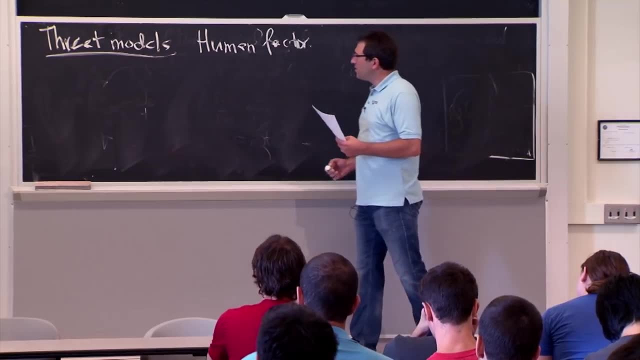 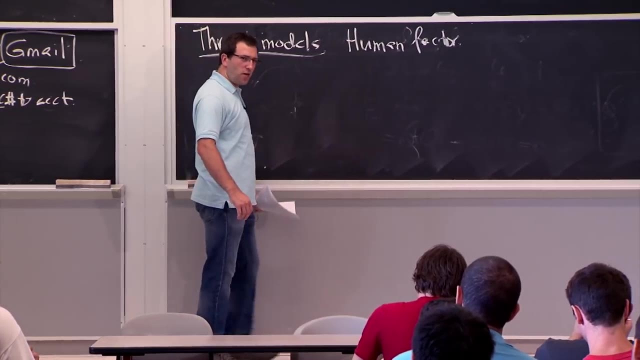 very strong assumptions about what humans will do, Because inevitably something will go wrong. Make sense Any questions, All right. Another sort of good thing to watch out in threat models is that they sometimes change over time, Or sort of whether something is a good assumption or not. 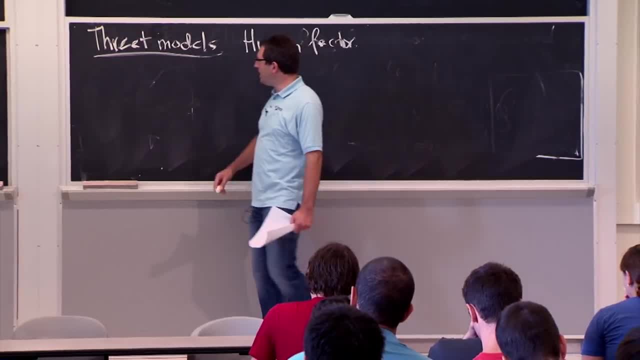 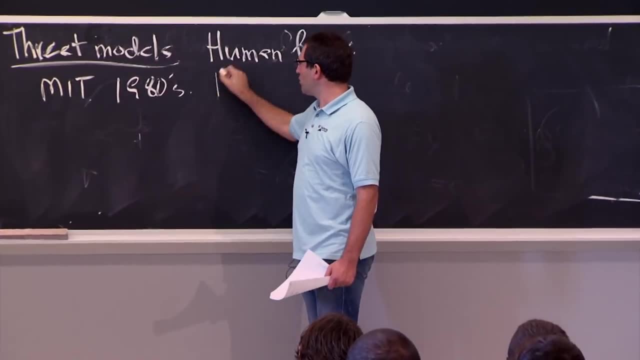 changes over time. One example of this is actually at MIT in the mid-90s, mid-80s actually, Project Athena developed this system called Kerberos, And we'll read about this. It's been a couple of weeks in this class. 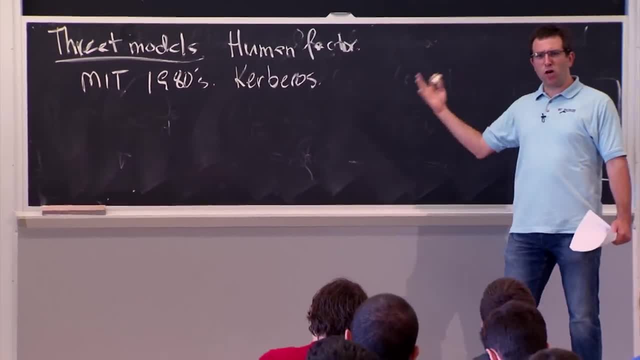 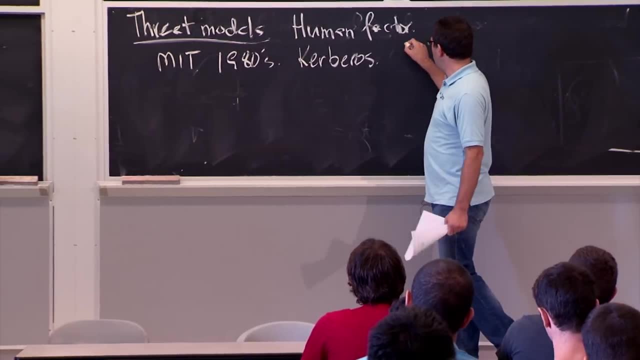 And at the time they were sort of figuring out: well, Kerberos is going to be based on cryptography, So we need to pick some size keys to make sure they're not going to be guessed by arbitrary people. And they said, OK, well, 56-bit keys. at the time, 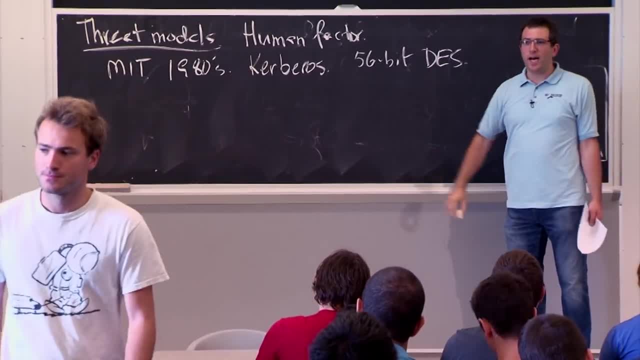 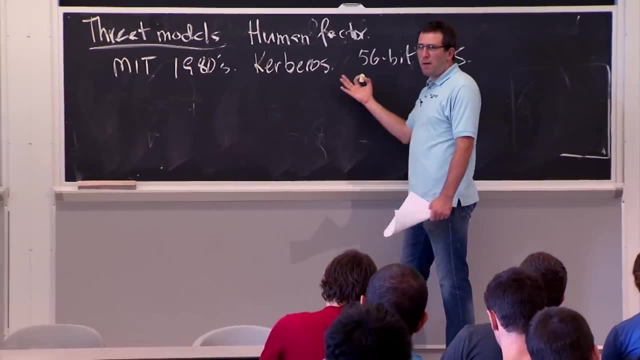 for this cipher called ds seemed like a plausible size, Maybe not great, but certainly not entirely unreasonable. And this was in the mid-80s. But then the system got popular, got used a lot- MIT still uses it- And they never really went back to seriously revisit. 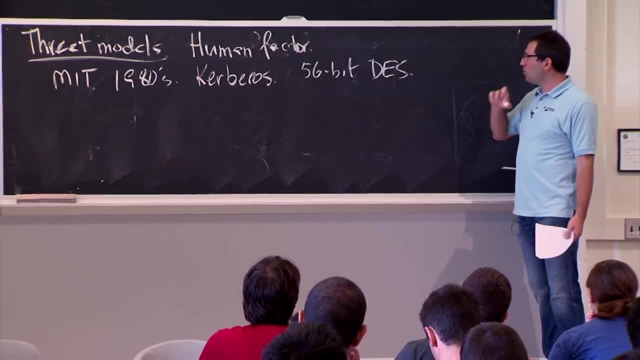 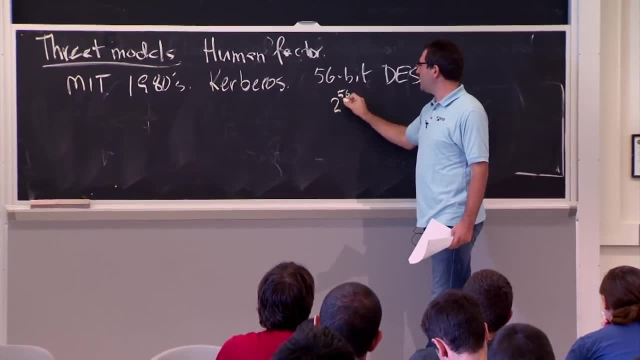 this assumption And then, a couple of years ago, a group of 6.858 students figured out that actually, yeah, you can just break this right. It's easy enough to enumerate all the 256 keys. these days, Computers are so fast, you can just do it. 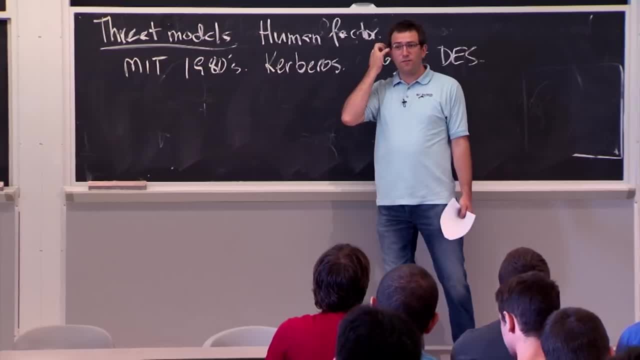 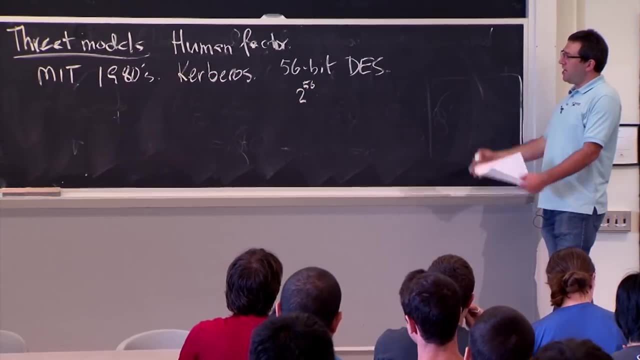 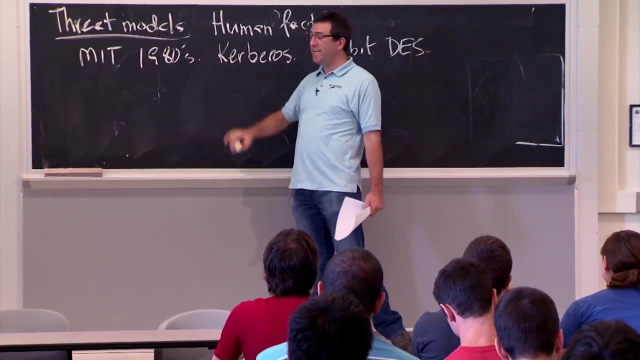 And as a result they were able to, with the help of some hardware from a particular web service- we'll have some links in the lecture notes- they were able to get basically anyone's Kerberos account key in roughly a day, And so this assumption was good in the mid-90s. 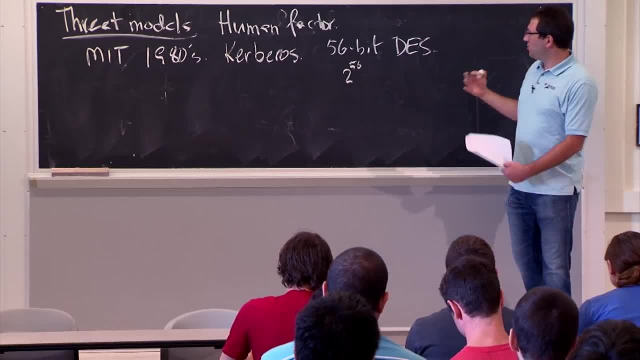 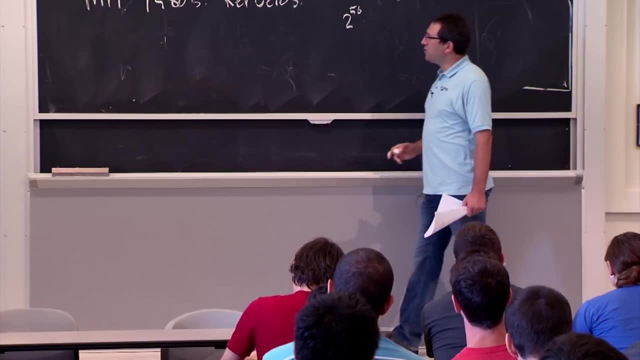 no longer a good assumption today. So you really have to make sure your assumptions sort of keep up with the times. Maybe a more timely example is if your adversary or if you're worried about government attacks, you might realize that you shouldn't trust hardware even. 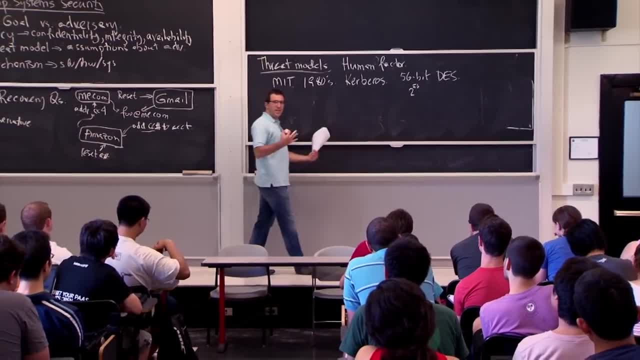 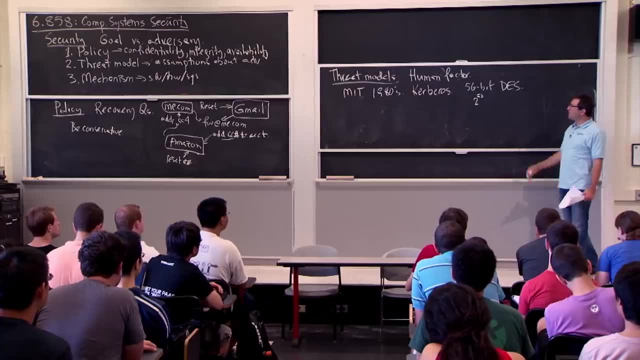 these days, right Like there's all these revelations about what the NSA is capable of doing, And they have hardware back doors that they can insert into, put into computers. Maybe up until a couple of years ago. well, who knows, I guess you didn't know about this stuff. 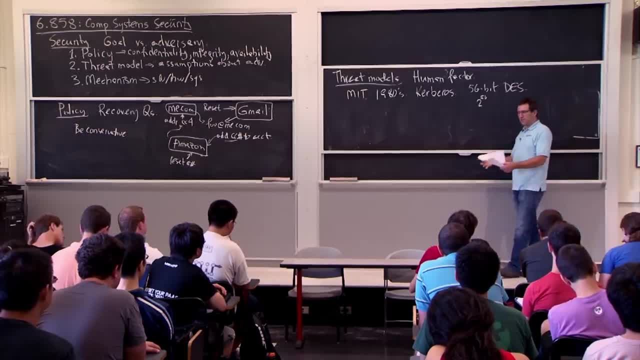 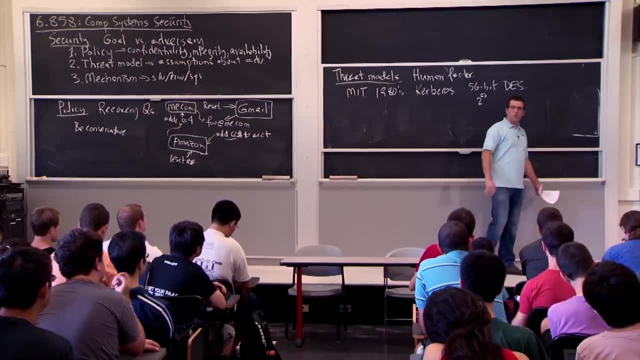 So maybe it was a reasonable assumption to assume your laptop is not going to be compromised physically like the hardware itself. But now you know, actually, if you're worried about the government being after you, you probably have a much harder problem to deal with. 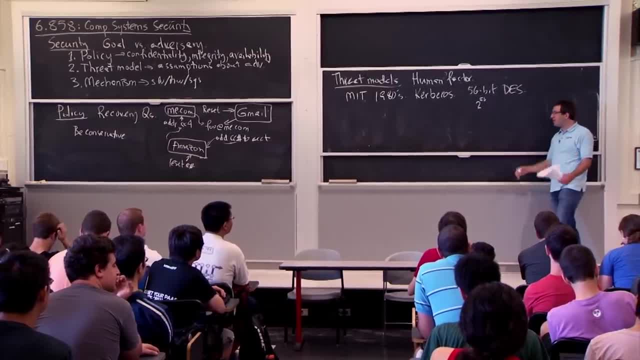 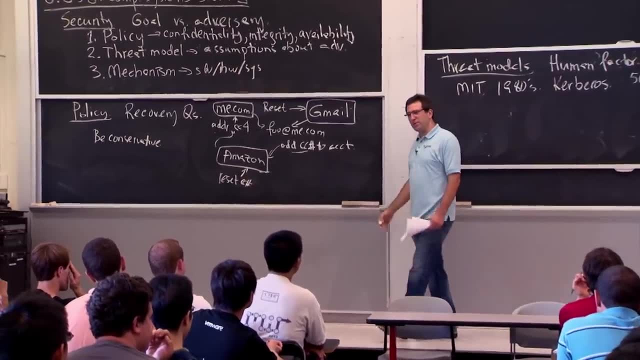 because your laptop might be compromised physically regardless of what you install on it. So you really have to be careful with your threat model and really sort of balance it against who you think is out to get you Like. I think it's going to be a very expensive proposition. 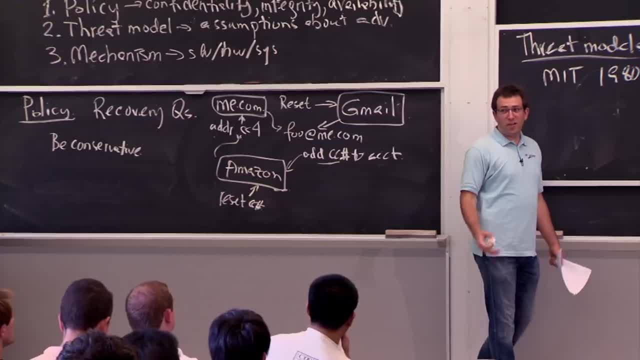 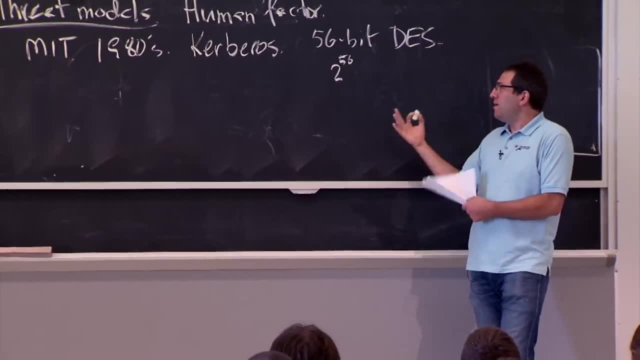 if you're going to try to protect yourself from the NSA really. On the other hand, if you're just protecting yourself from random other students that are, I don't know, snooping around in your Athena home directory or whatnot, maybe you don't have to worry about this stuff as much. 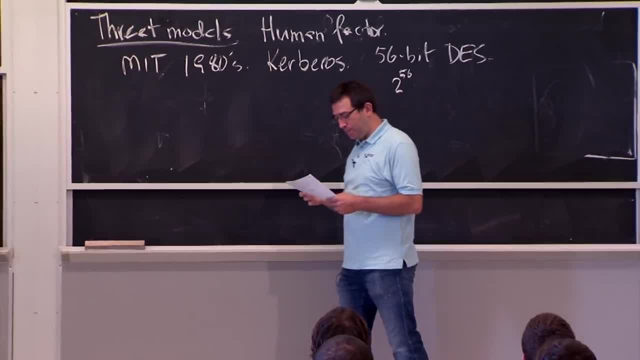 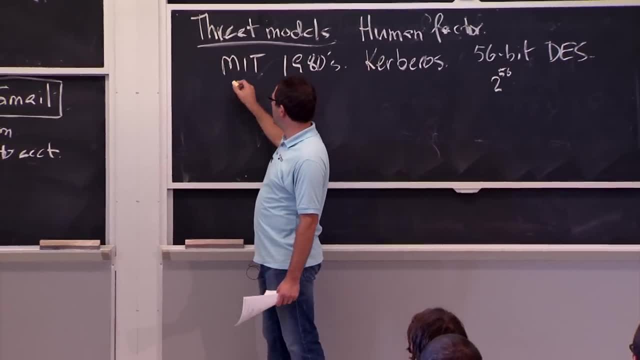 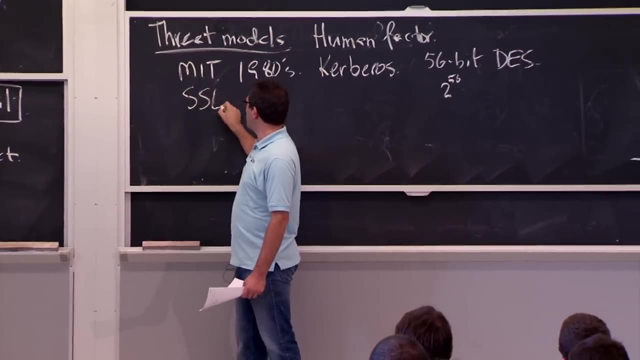 So it's really sort of a balancing game in picking the right threat model. Another sort of example of a bad threat model shows up in the way secure websites these days check certificates of a website that you're connecting to. So, in this SSL protocol or TLS, when you connect to a website, 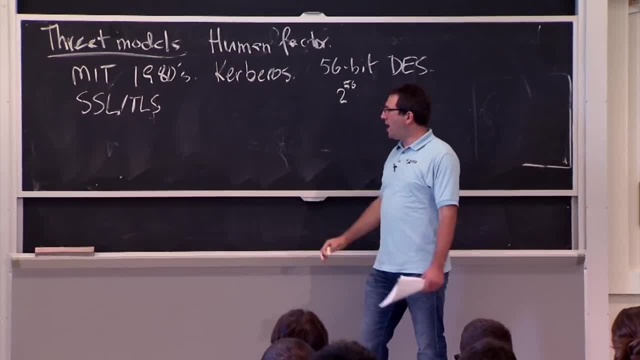 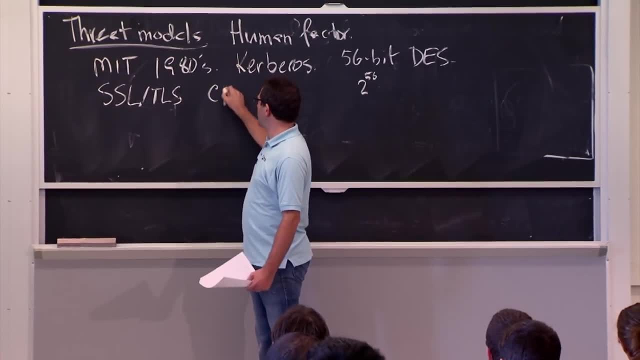 and it says HGPS. we'll talk much more about this in later lectures, But what happens is that the site you're connecting to presents you a certificate signed by one of the certificate authorities out there that asks that: yep, this key belongs to Amazoncom. 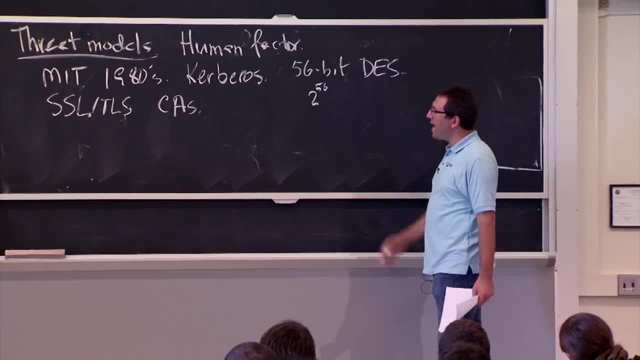 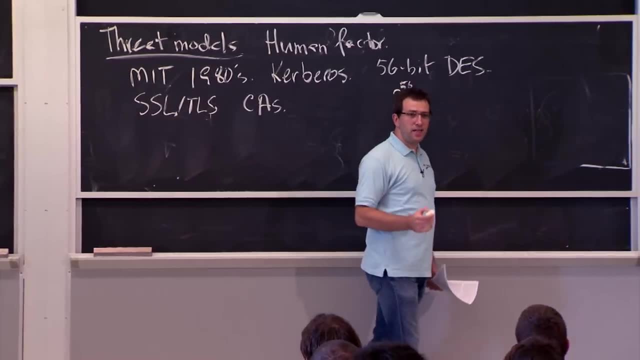 And architecturally, the sort of mistake that, or the bad threat model that these guys assumed, is that all these CAs are going to be trustworthy, they'll never make a mistake, And in fact, the way the system works is that there's hundreds of these CAs out there. 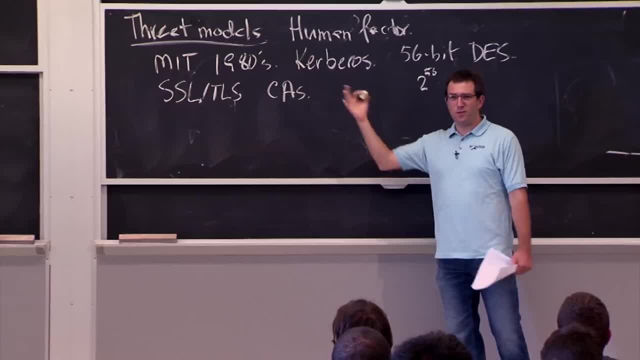 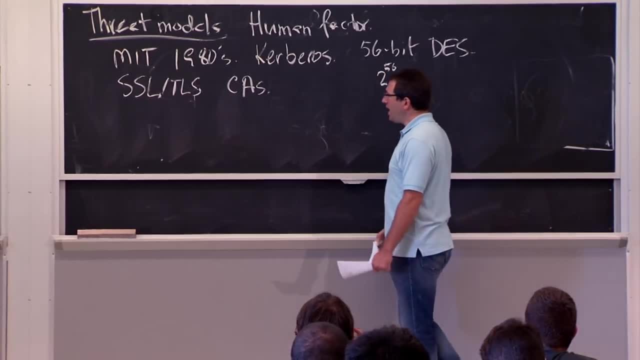 The Indian Postal Authority, I think, has a CA. The Chinese government has a CA, Lots of entities are certificate authorities in this design And any of them can make a certificate for any host name or any domain name. And, as a result, what happens if you're a bad guy? 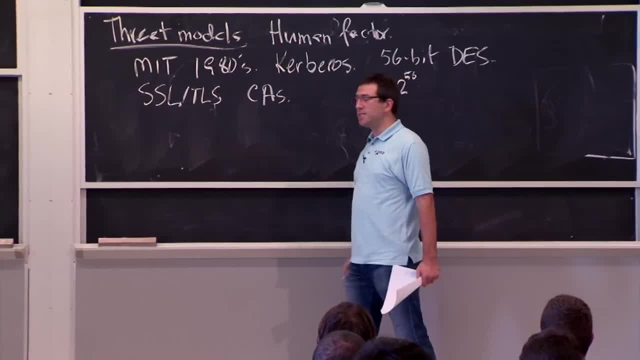 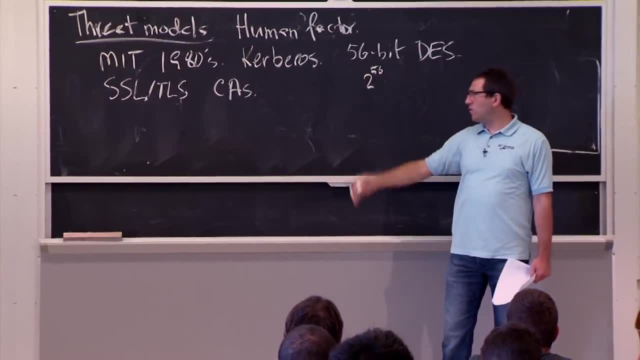 if you want to compromise Gmail, or if you want to impersonate Gmail's website, you just have to compromise one of these certificate authorities And it turns out the weakest link is probably some poorly run authority somewhere in some not particularly up-to-date country. Who knows right, And as a result, it's probably a bad assumption to build a system, or it's a bad idea to build a system around the assumption that you'll manage to keep all 300 certificate authorities spread out around the globe perfectly secure. 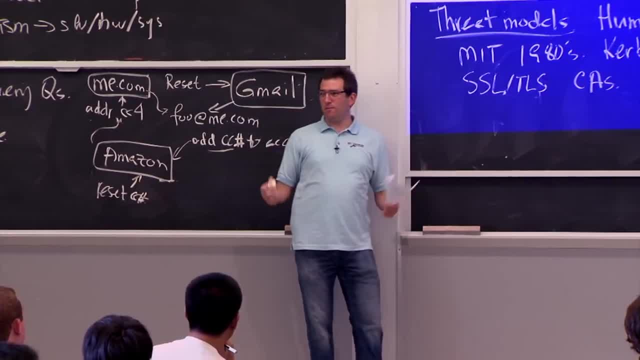 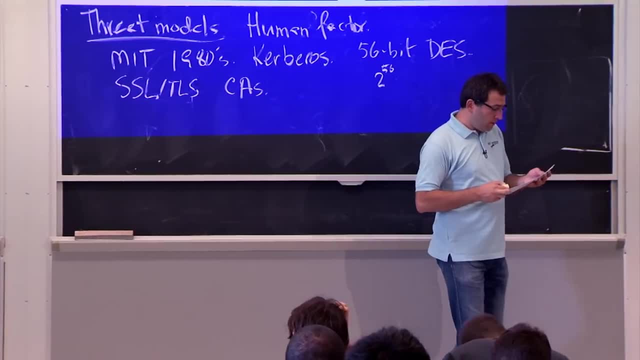 But yet that's the assumption underpinning the security mechanism of today's SSL. OK, So that's the protocol used by web browsers, And there's sort of many other, I guess, examples that are things you might not have thought of. 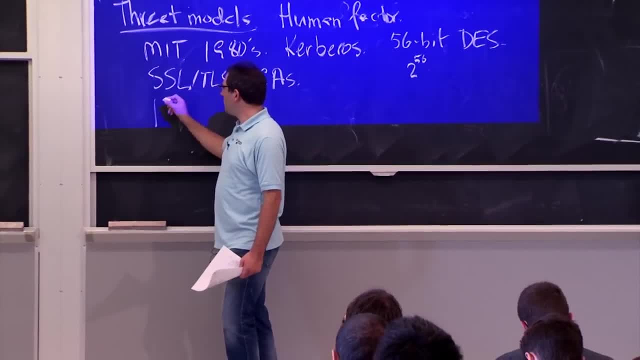 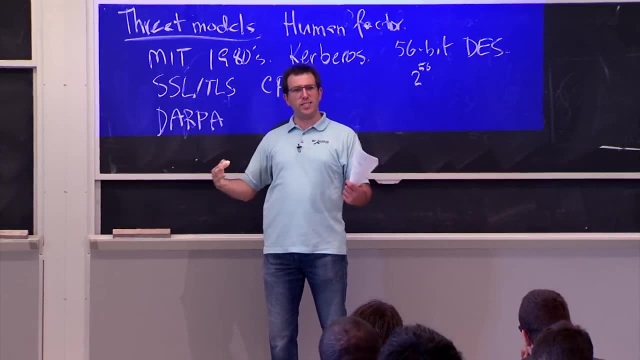 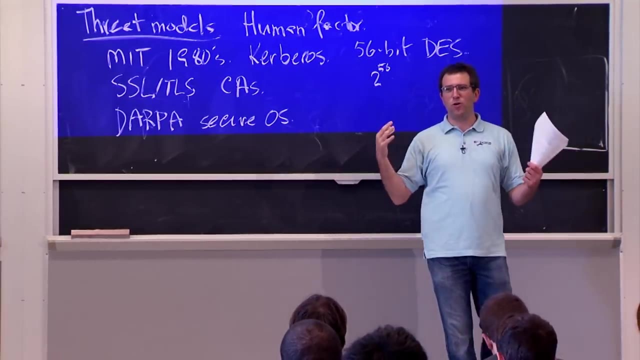 Another sort of amusing example from the 1980s was DARPA. this defense agency at the time really wanted to build secure operating systems And they actually went so far as to get a bunch of universities and researchers to build secure OS prototypes. 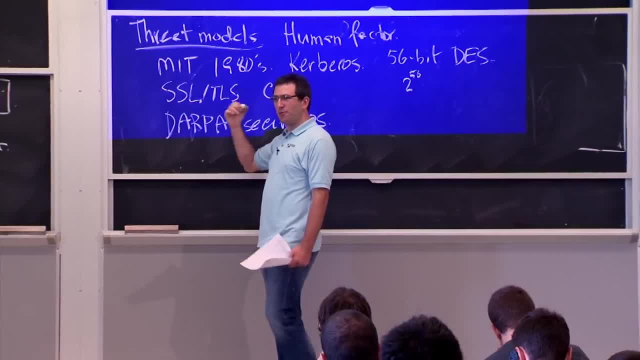 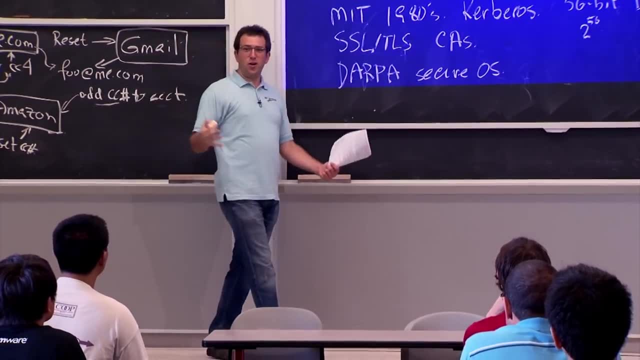 And then they actually got a red team, like a team of guys, pretending to be the attackers, and told them: well, go break into these secure operating systems any way you can. We actually want to know: is it secure? And it's kind of amusing. 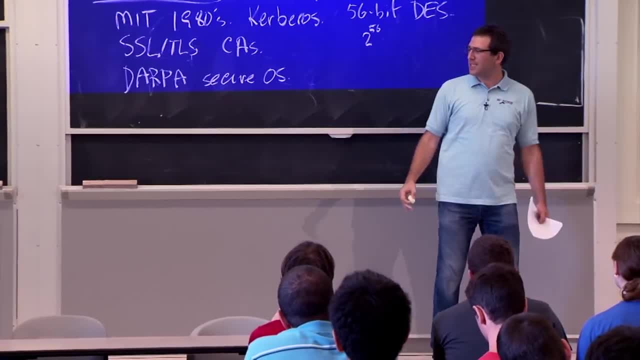 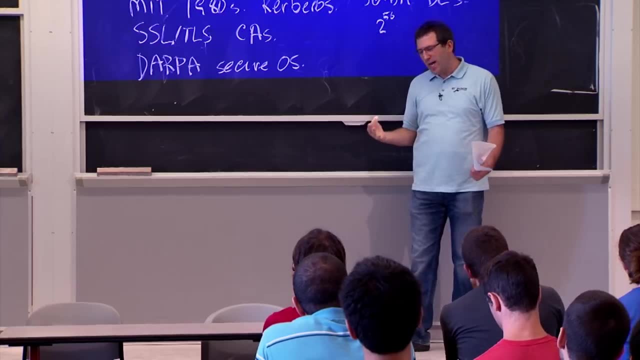 Some of the surprising ways they compromised the systems. One was that there was this OS research team that seemed to have a perfectly secure OS, but it got compromised, And the way it happened is that the server in which the source code of the operating system was stored. 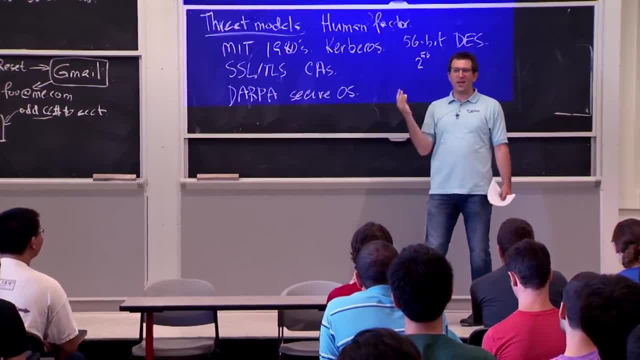 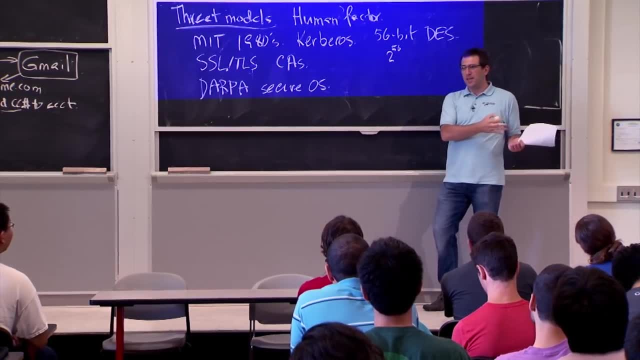 was some development machine in someone's office that wasn't secured at all But that had all the source code. So the bad guys broke into that server- It was not protected very well- changed the source code of the operating system to introduce a back door. 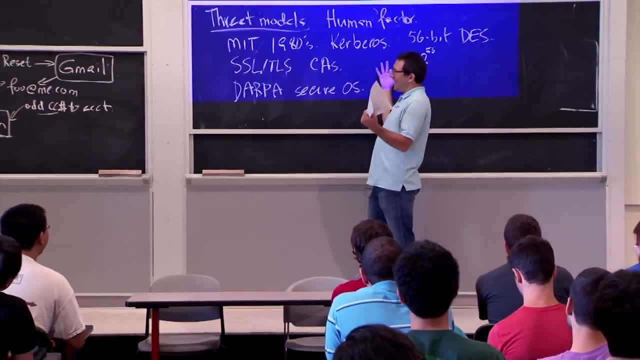 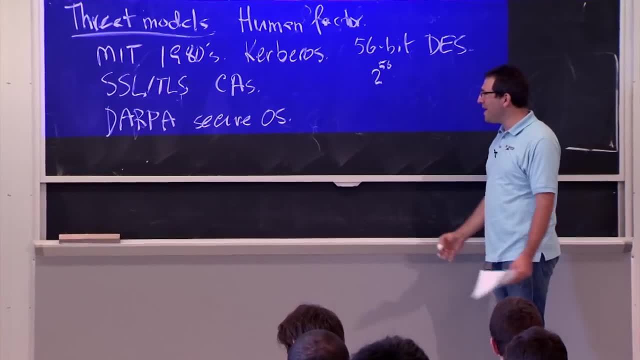 And then when the researchers built their operating systems, well, it had this back door and the bad guys were able to break in. So you really have to think about all the possible sort of assumptions you're making about where your software is coming from, about how the bad guy can get in in order. 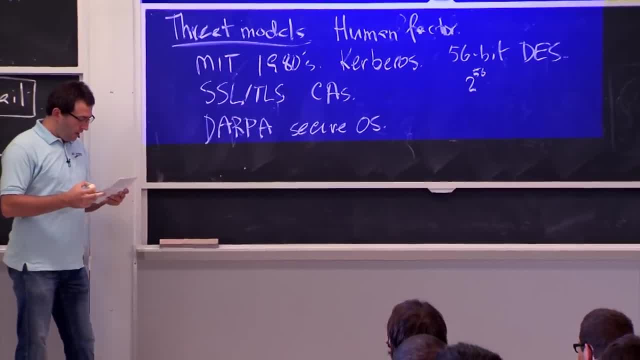 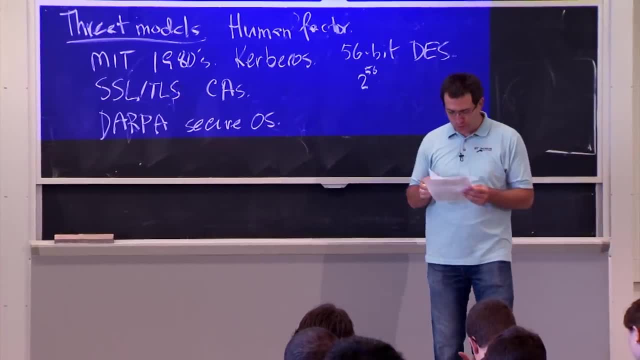 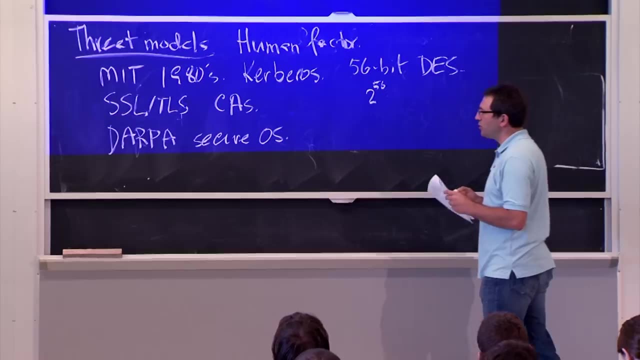 to make sure your system is really secure, And there's many other examples in lecture notes, but if you want sort of some using anecdotes, you can page through those. Probably the most pervasive problem that shows up, of course, is in mechanisms, though. 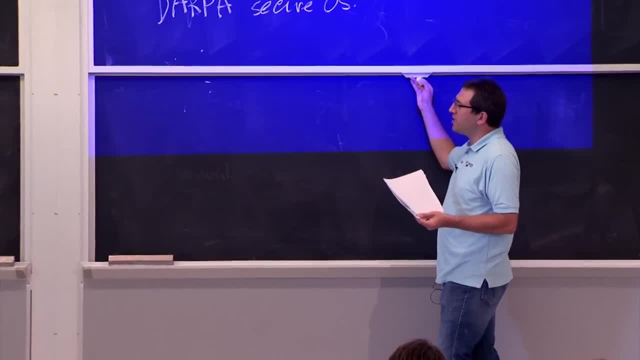 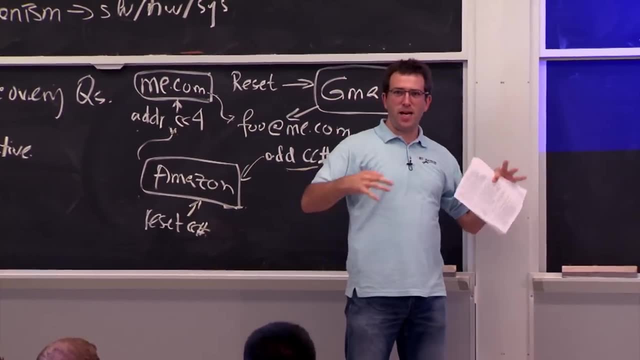 And in part it's because mechanisms are the most complicated part of the story. It's the entirety of all the software and hardware and all the sort of system components that make up what is trying to enforce your security policy. And there's not much. 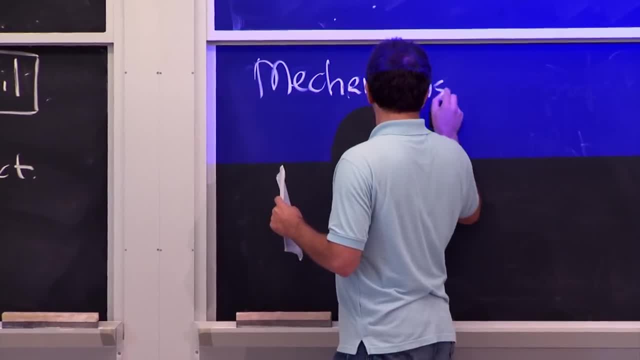 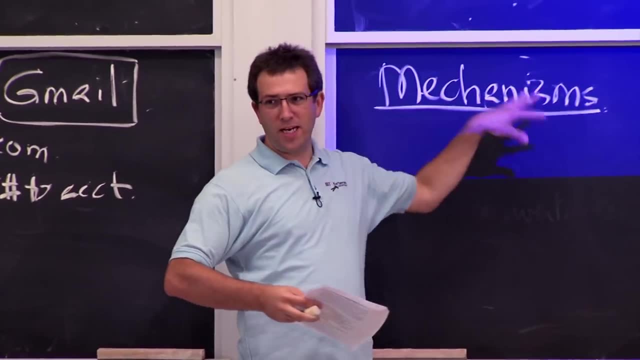 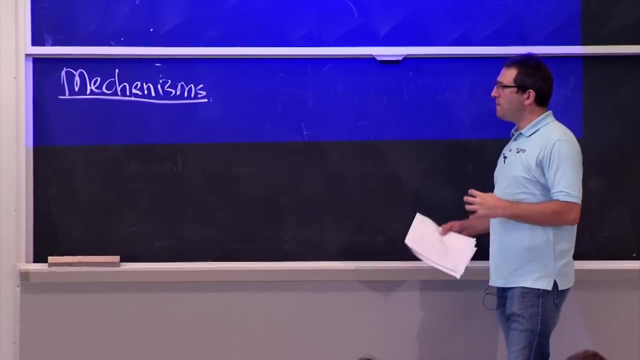 There's no end of ways in which mechanisms can fail And, partly as a result, much of this class will focus pretty heavily on mechanisms and how do you make mechanisms that are secure, that provide correct enforcement of security policies, And we'll talk about threat models and policies as well. 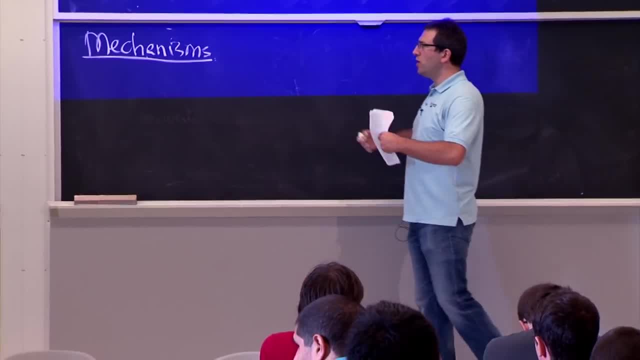 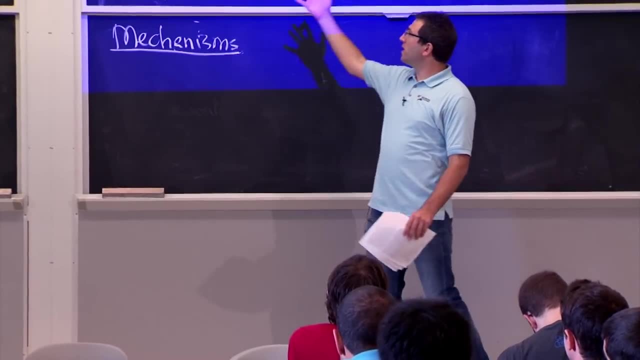 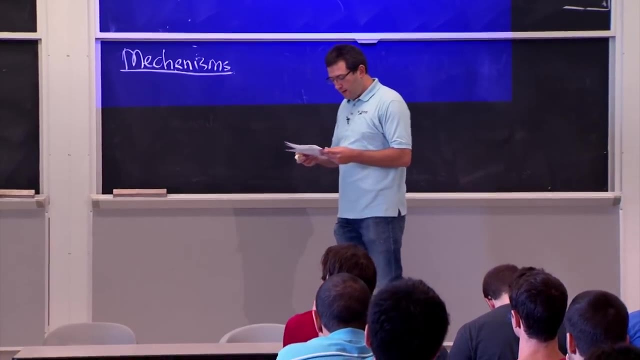 but turns out it's much easier to make clean sort of crisp statements about mechanisms and ways they work and don't work, As opposed to policies and threat models, which really you have to figure out how to fit them into a particular context where you're using a system. 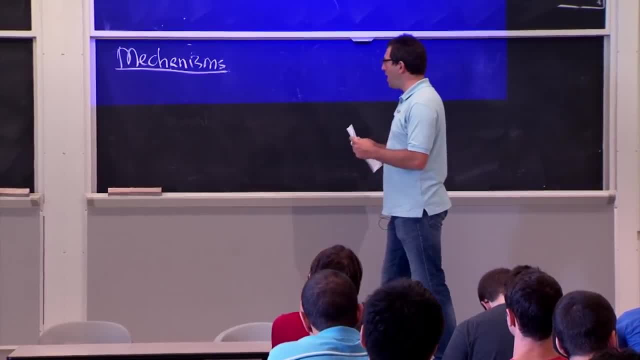 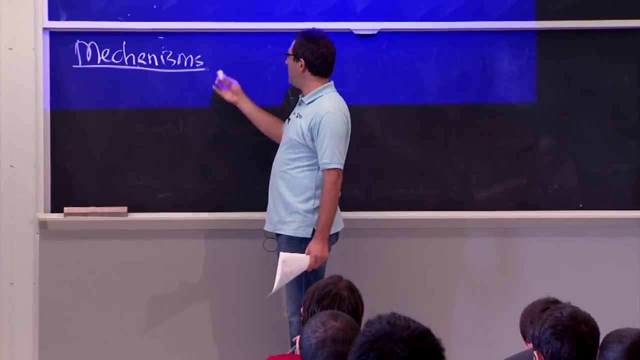 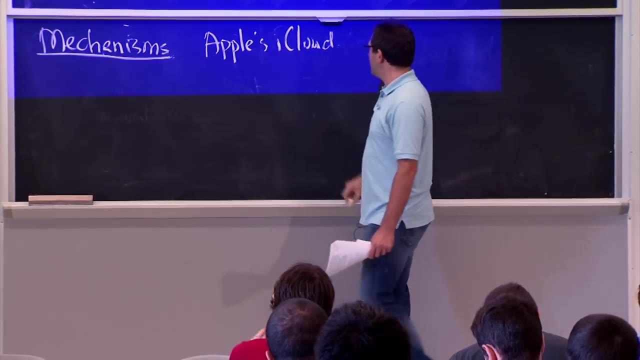 So let's look at some examples of, I guess, mechanism bugs. One that you might have heard in the last couple of days was a problem in the security mechanism in Apple's cloud infrastructure called iCloud. Actually, any one of you that has an iPhone might be using. 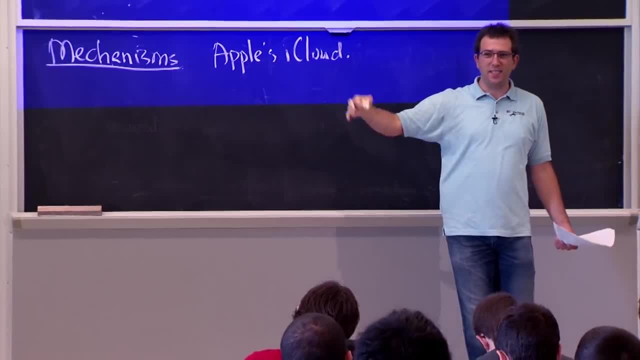 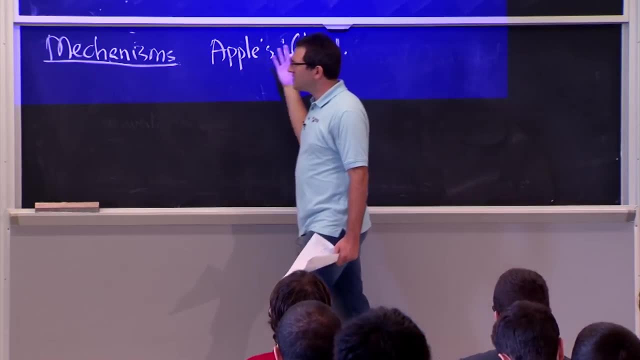 this iCloud service. They basically provide storage for your files and let you find your iPhone if you lose it, and probably lots of other useful features, And I think it's some relative of this mecom service that was implicated in this scheme a couple of years back. 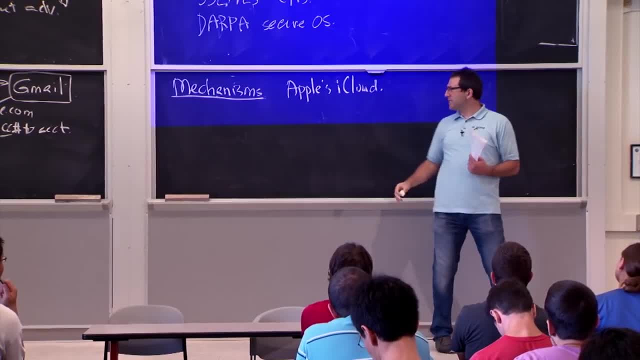 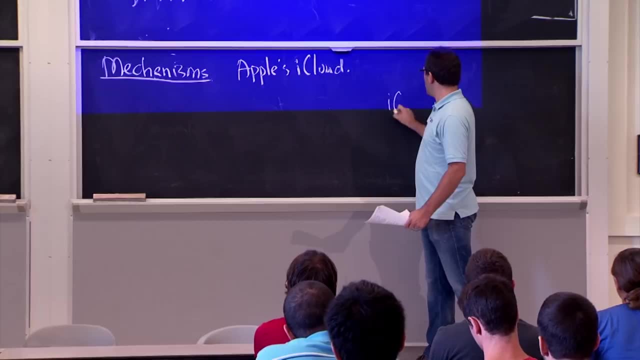 And the problem that someone discovered in this iCloud service is that they didn't enforce the same sort of mechanism at all interfaces. OK, so what does iCloud look like? Well, it basically provides lots of services because for the same sort of set of accounts, 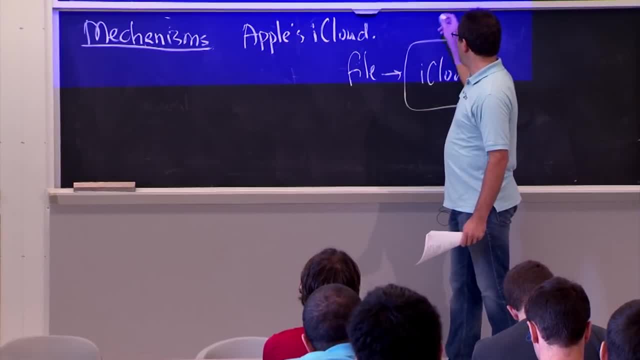 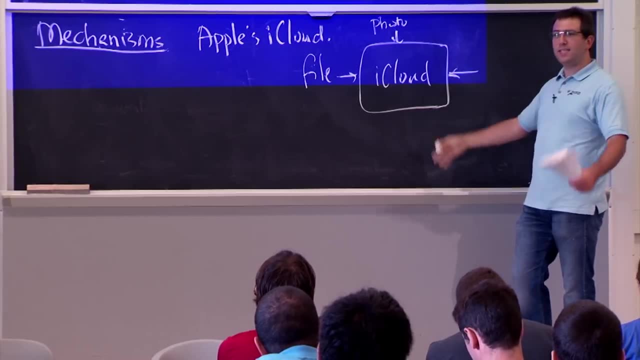 so maybe you have your file storage on iCloud, Maybe you have your photo sharing, Maybe you have other interfaces And one of the interfaces into iCloud- these are all sort of different APIs that they provide- was this feature to find my iPhone, I think. 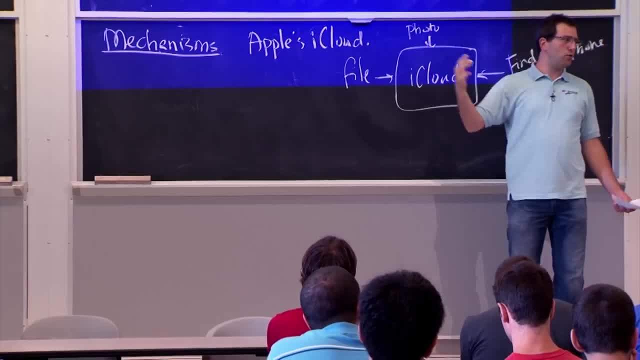 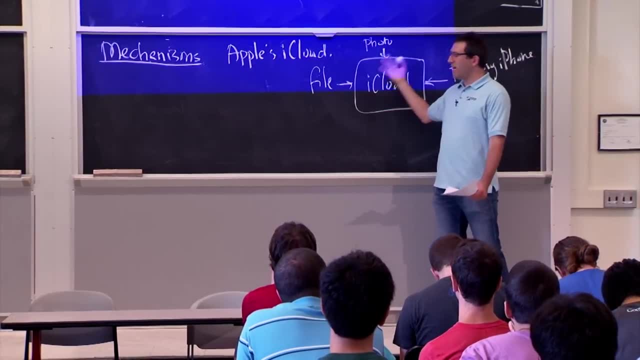 And all these interfaces want to make sure that you're the right user, you're authenticated correctly And, unfortunately, the developers of this iCloud system. it's a giant piece of software. I'm sure Lots of developers work on this, But on this particular interface. 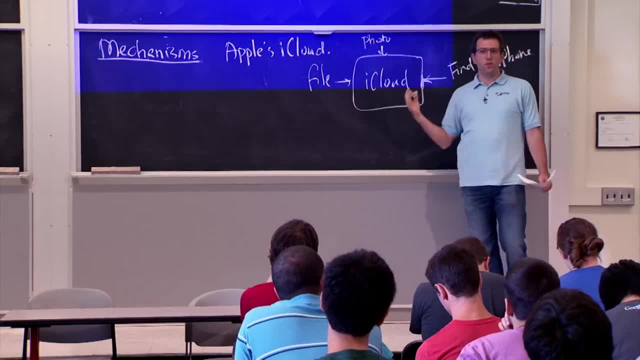 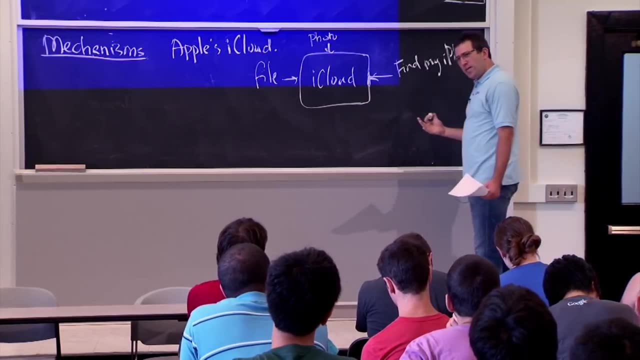 the find my iPhone interface when you try to log in with a username and password. they didn't keep track of how many times you try to log in, And the reason this is important is that, as I mentioned earlier, humans are not that great at picking good passwords. 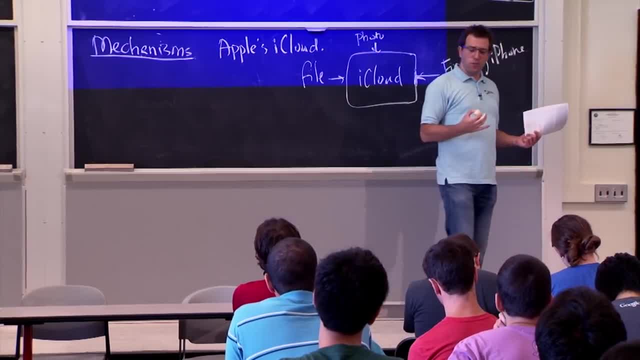 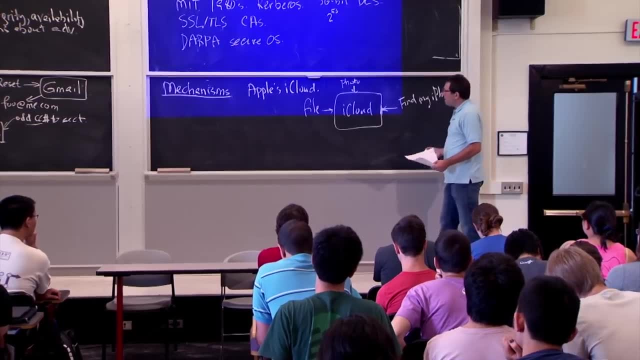 So actually building a system that authenticates users with passwords is pretty tricky- We'll actually read a whole paper about this later on- But one good strategy is: there's probably a million passwords out there that will account for 50% of the accounts. So if you can guess, make a million attempts at someone's account, then there's a good chance you'll get their password, Because people actually pick predictable passwords, And one way to try to defeat this is to make sure that your system doesn't. 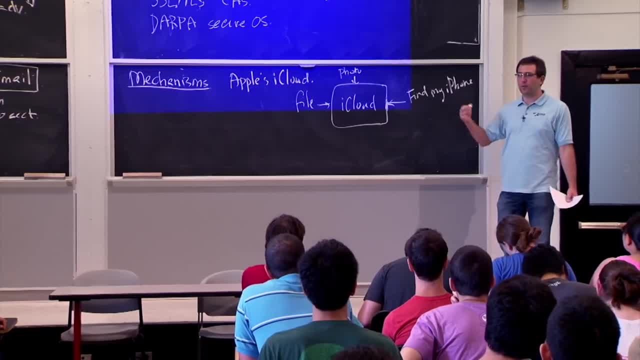 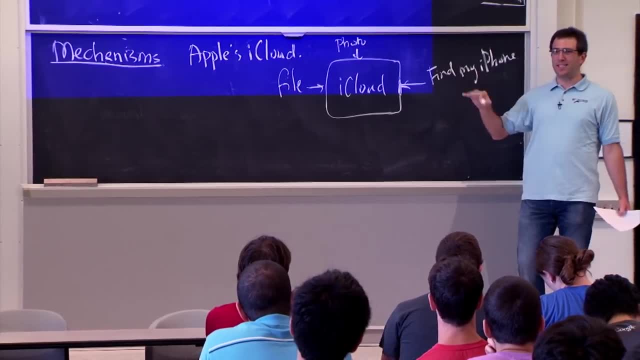 allow an arbitrary number of attempts to log into an account. Maybe after three or 10 tries you should say: well, you've had enough tries Time out. You can try again in 10 minutes or in an hour, And this way you really slow down the attacker. 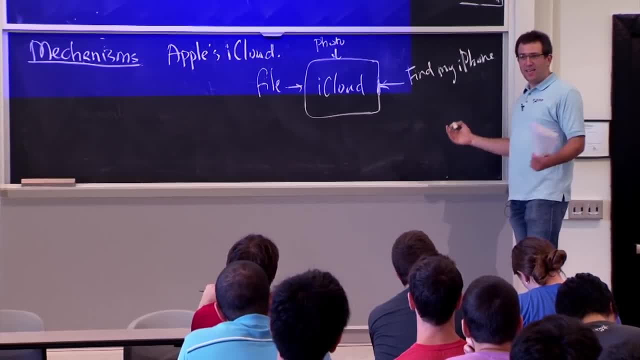 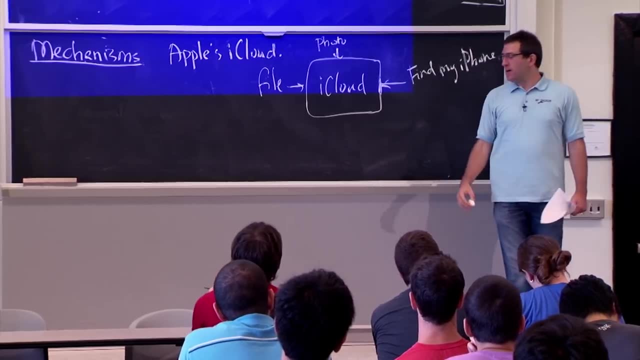 so they can only make a handful of guesses a day instead of millions of guesses And, as a result, even if you have not the greatest of passwords, it's going to be pretty hard for someone to guess it. But what happened is that iCloud had this password guessing. prevention, or basically back off on some interfaces, Like if you tried to log in through other interfaces and you failed 10 times, it would say: well, sorry, you have to wait until you try again, But on this, Find My iPhone interface. they forget this check. It's probably some guy just forgot to call this function on this API, But the result is that for the same set of accounts, a bad guy would be able to now guess your password through this interface at millions of attempts per day. easily, Because this is just limited at how fast they can send packets to this iCloud thing And they can probably guess your password with pretty good accuracy or with pretty good success rate, after You know making many guesses, And this led to some unfortunate break-ins. 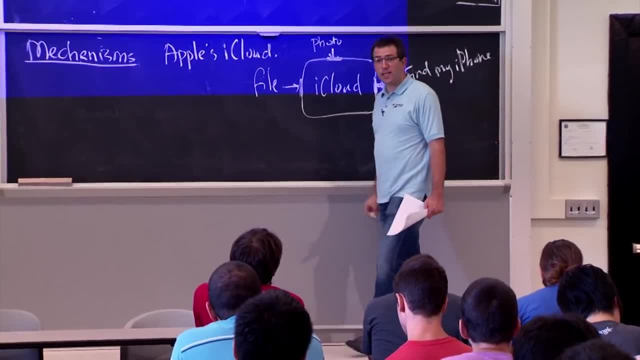 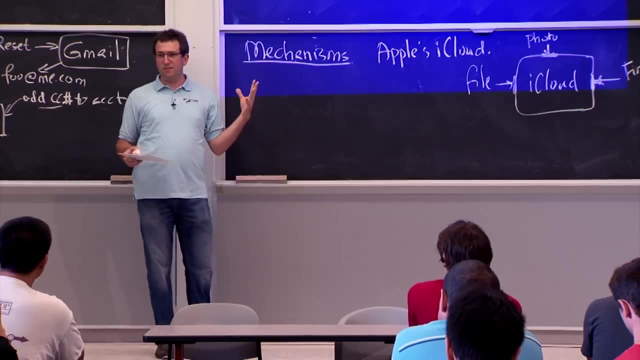 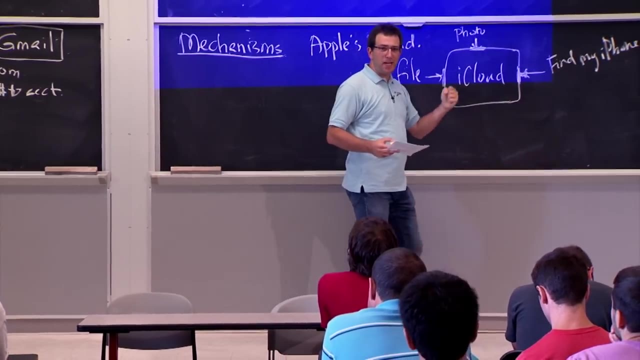 and people's confidential data got stolen from this iCloud service. So this is sort of an example of you had the right policy. Only the user and the right password would get you access to the files. You even had the right threat model that well the bad guy might be able to guess the password. 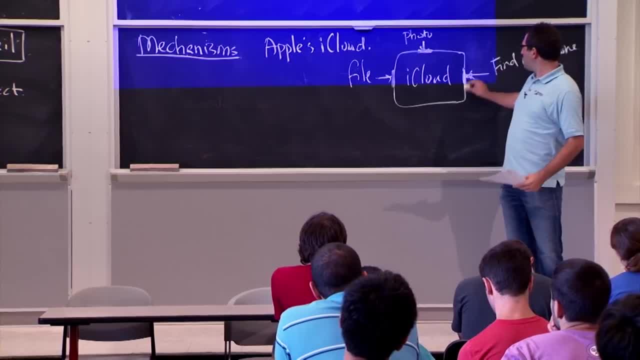 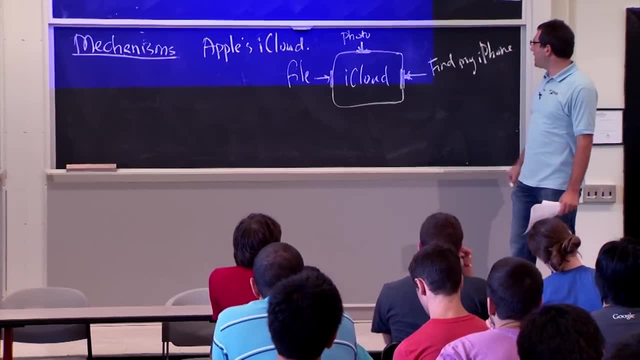 so we'll have to rate limit the number of guess attempts. But he just screwed up Like the mechanism had a bug in it. We just forgot to enforce this right policy and mechanism at some interface, And this shows up again and again in systems. 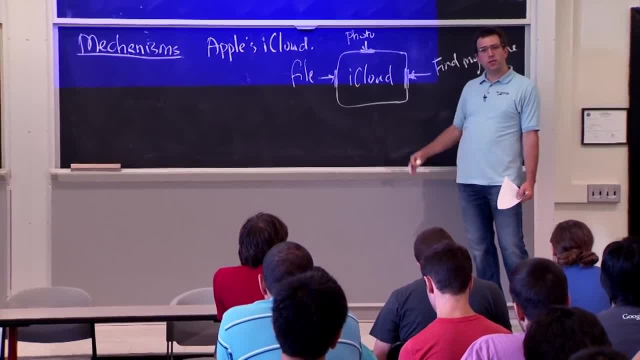 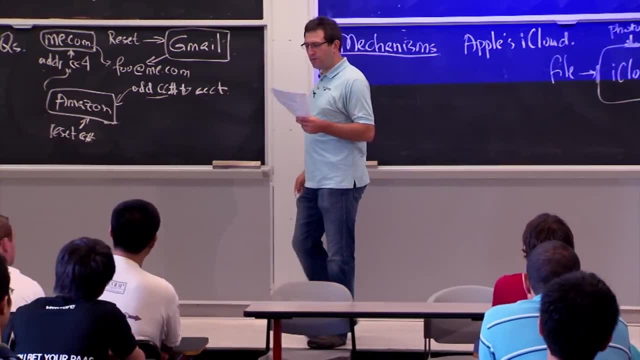 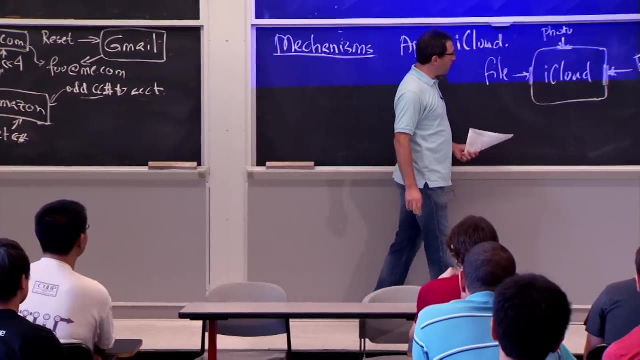 where you just made a mistake and it has pretty drastic effects on the security of the overall system. Does this make sense? Any questions? so far, All right, OK, So another example. This is sort of an example of you forget to check for password guessing attempts. 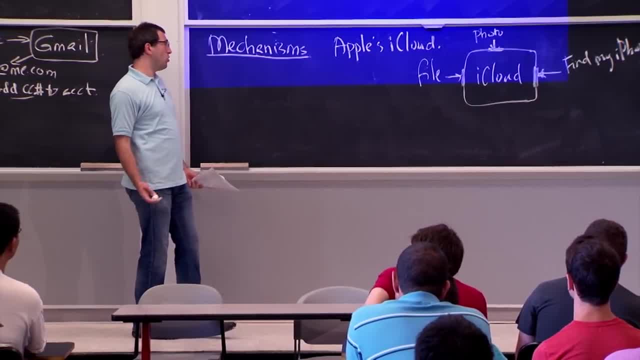 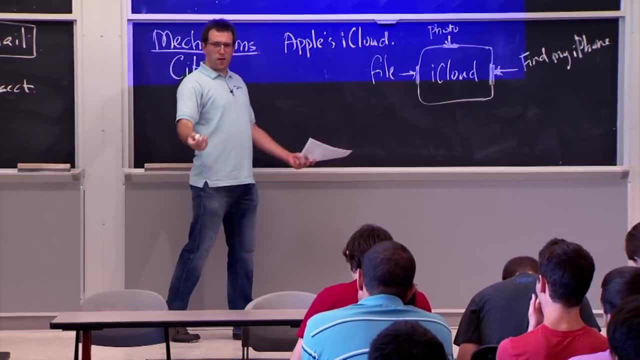 There's many other things you can forget. You could forget to check for access control altogether. So one example is Citibank had a website- actually still has a website that allows you to look at your credit card account information. So if you have a credit card with Citibank, 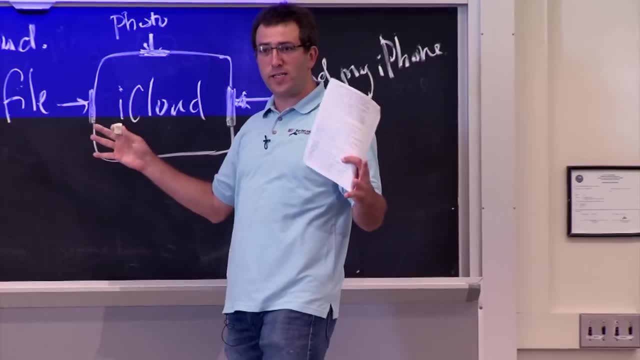 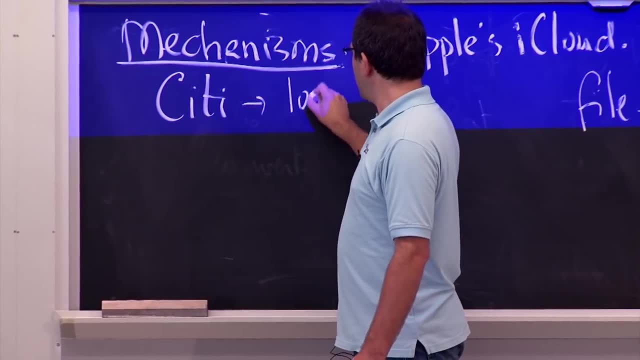 you go to this website, It tells you: yeah, you have this credit card, Here's all the charges, all this great stuff. And the workflow a couple of years ago was that you go to some site, You provide a login username and password. 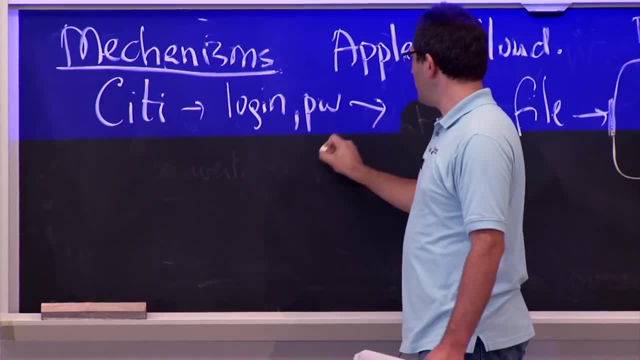 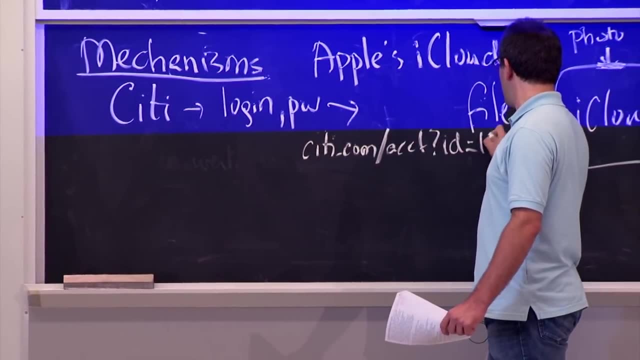 And you get redirected. You get redirected to another URL which is something like: I don't know I'm guessing, but basically like citycom slash account. question mark ID equals whatever: 1,, 2,, 3,, 4.. 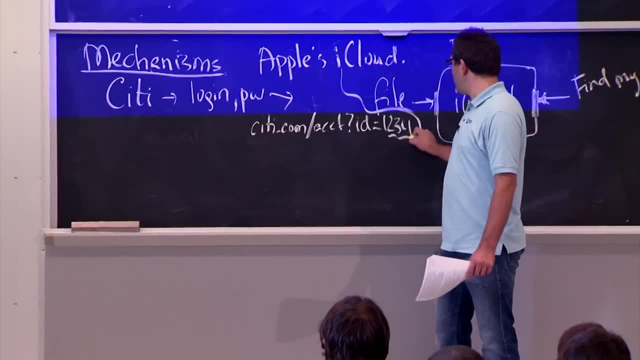 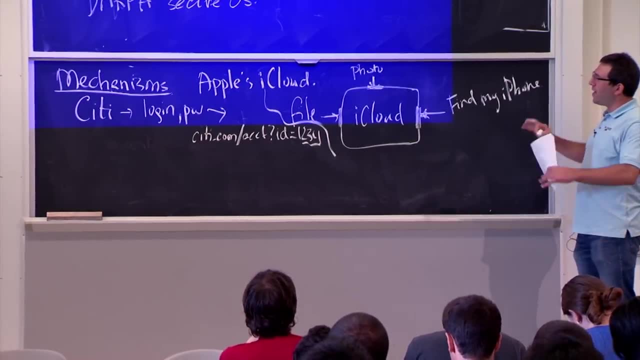 And it turns out that some guy figured out. well, if you change this number, you just get someone else's account, And it's not clear quite how to think of this. One possibility is that these guys were just thinking right, But they again forgot to check a function in this account page. 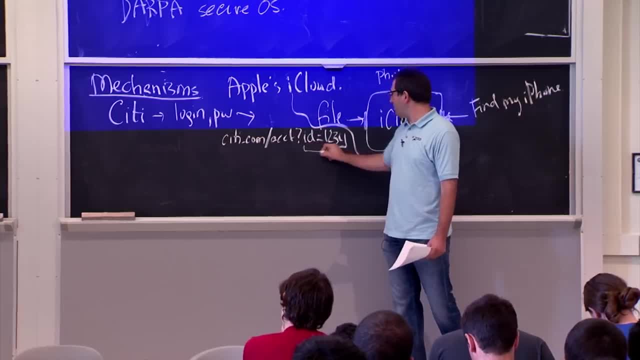 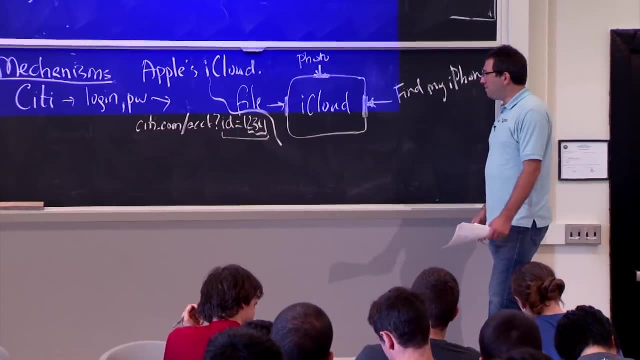 that you can't do that. But not only do I have a valid ID number, but it's also the ID number of the guy that's currently logged in. That's an important check to make, but it's easy to forget. Another thing is: maybe these guys were thinking 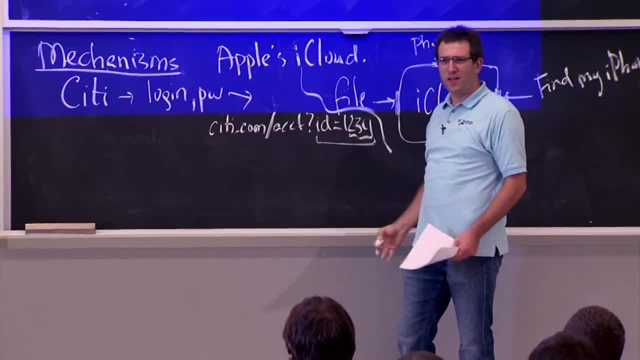 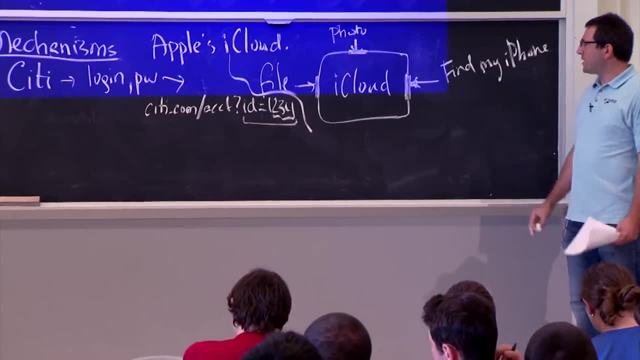 no, no one can have URLs. Maybe they had a bad threat model. Maybe they're thinking the URL. if I don't print this URL, no one can click on it. It's like a bad threat model. Well, it's hard to tell exactly what went wrong. 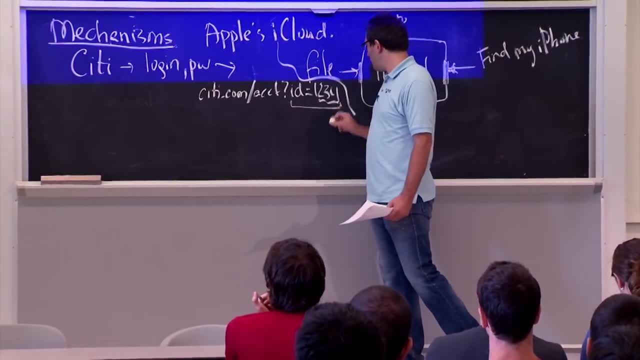 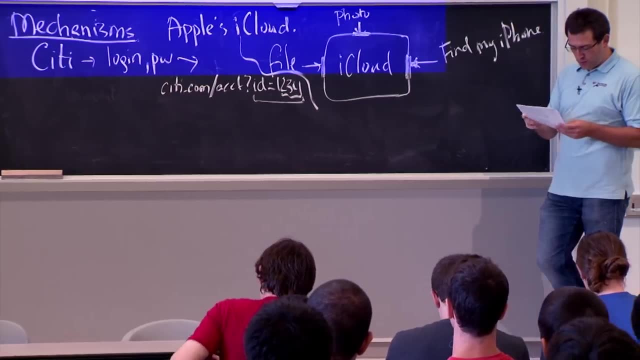 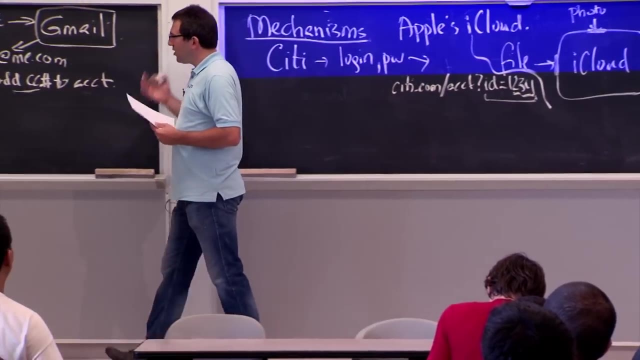 But anyway, these mistakes do happen And they show up. a lot Sort of easy to have. small, seemingly bugs in your mechanism lead to pretty unfortunate consequences. Another example that's not so much in missing checks is a problem that showed up on Android phones. 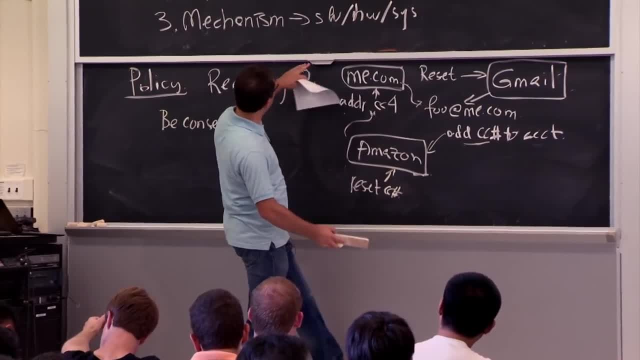 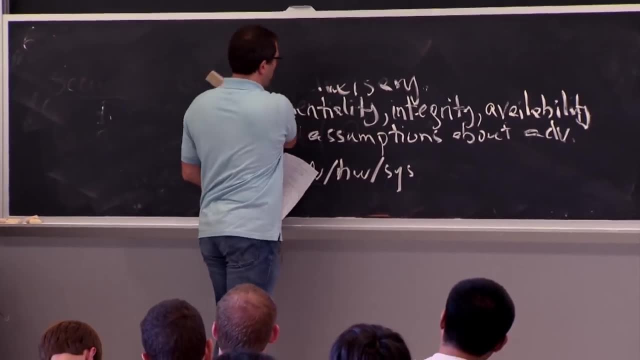 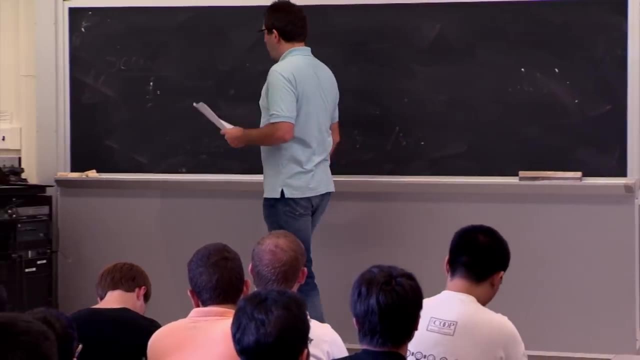 a couple of months ago. Maybe I'll use this board over here. So the problem was related to Bitcoin, which is this: well, I'm sure you've heard this. You know Electronic currency system that's pretty popular these days And the way that Bitcoin works at a very high level. 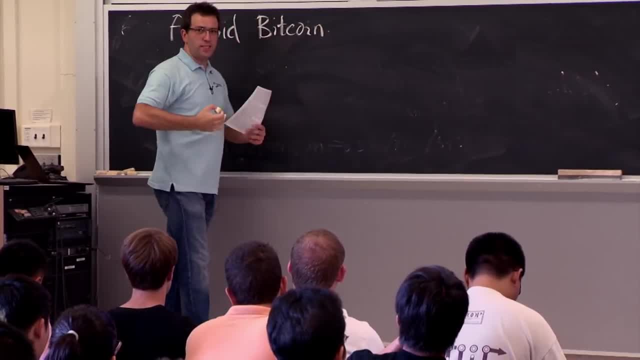 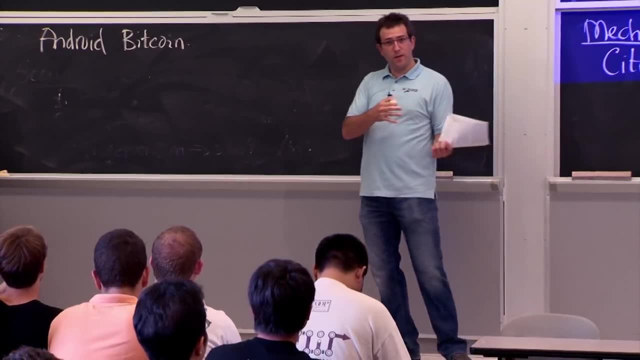 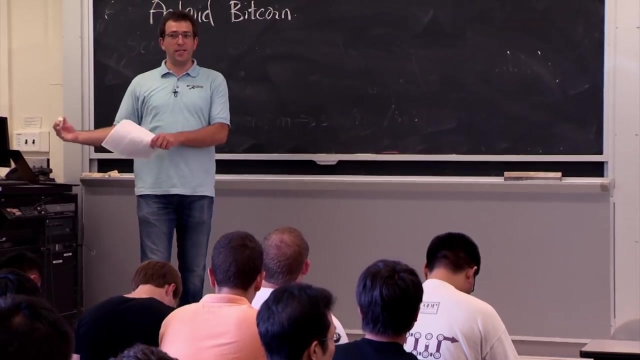 is that your balance of Bitcoins is associated with a private key, And if you have someone's private key, you can, of course, spend their Bitcoins. So the security of Bitcoin relies quite heavily on no one else knowing your private key. It's kind of like a password, except it's even more important. because people can probably make lots of guesses at your private key And there's no real server that's checking a key, It's just cryptography. So any machine can try to make lots of guesses at your private key And if they guess it, then they can transfer your Bitcoins. 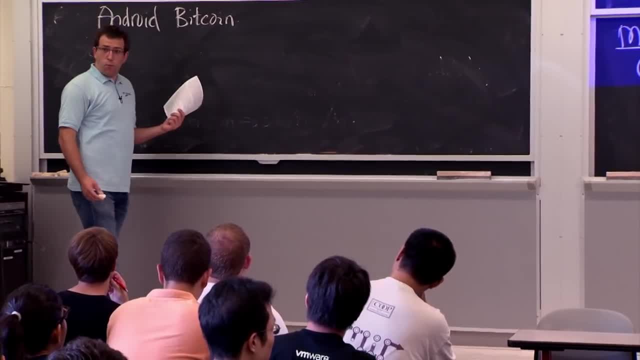 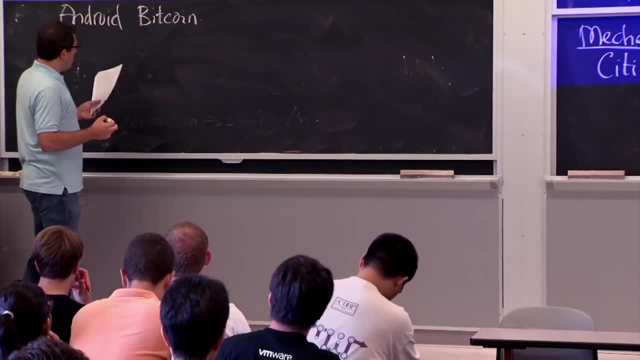 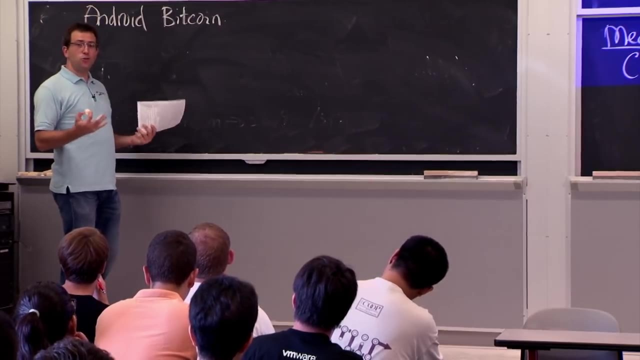 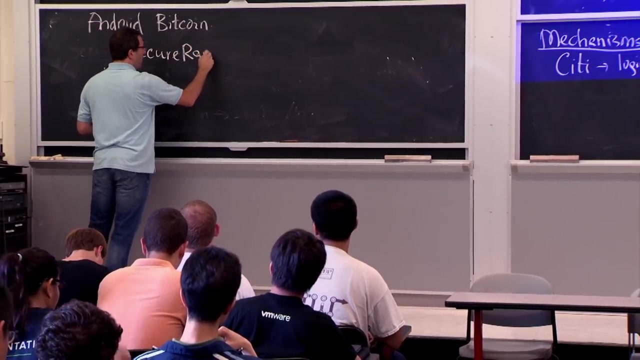 to someone else And, as a result, it's critically important that you generate good random keys that no one else can guess. And there are people using Bitcoin on Android And the Android applications for Bitcoin. we're getting random values for these keys using this Java API called Secure Random, which sounds great. 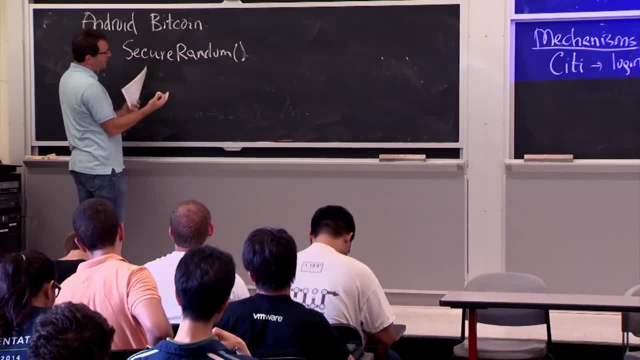 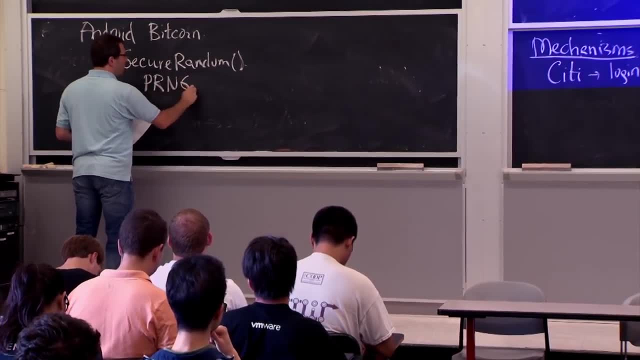 But as people figured out well, OK, so what it is, it doesn't really get real random numbers. Inside of it there's this construction called a pseudo-random number generator, or PRNG, that, given a particular seed value, like, you get maybe a couple of hundred bits of randomness. 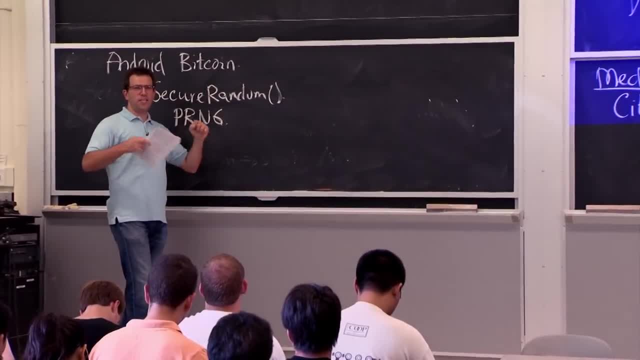 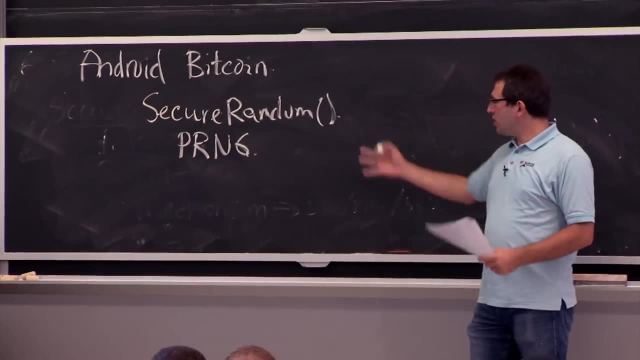 and you shove it into this PRNG and you can keep asking it for more randomness, And you can sort of stretch these random bits into as many random bits as you want. So you seed them initially and then you can generate as many random bits as you want. 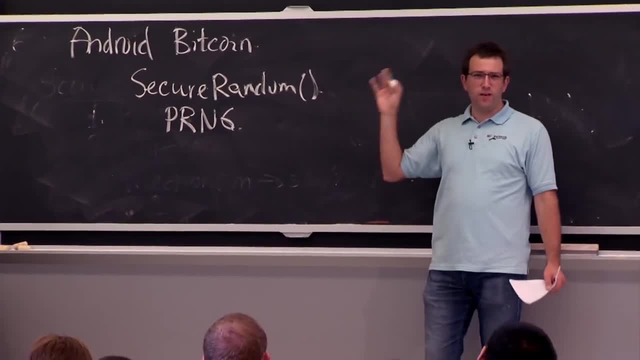 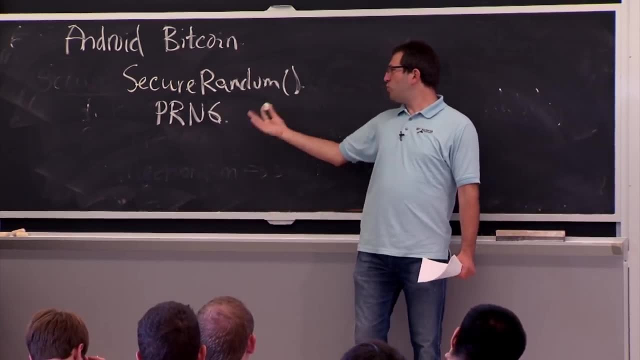 And for various cryptographic reasons I won't go into here, it actually works. If you give it a couple of hundred really good random bits. initially, it's going to be very hard for anyone to predict what the pseudo-random values generating are. But the problem is that this Java library had a small bug in it. In some set of circumstances it forgot to initialize the PRNG with a seed, So it was just all zeros, which means that everyone could just figure out what your random numbers were. If they start with zeros, they'll. 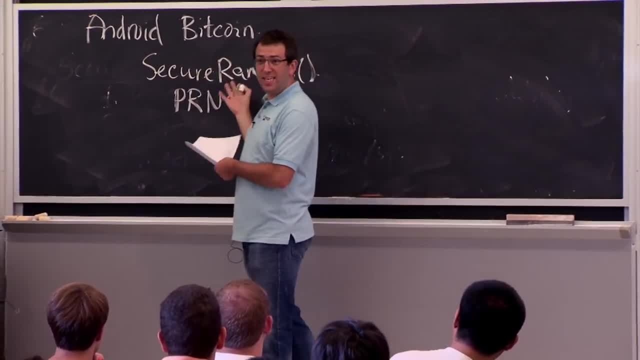 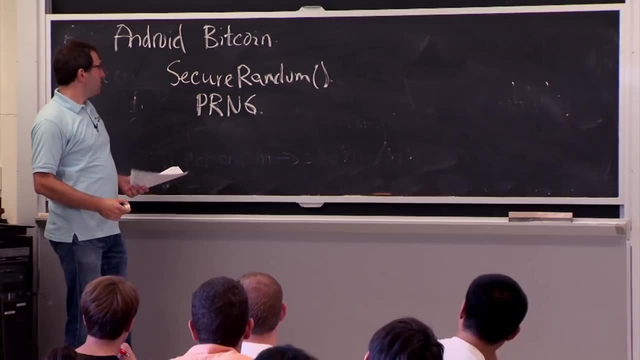 produce the same random numbers as you, which means they'll produce the same private key as you, So they can just generate the same private key and transfer your bitcoins. So this is again a small or not small bug, depending on, I guess, who is asking. 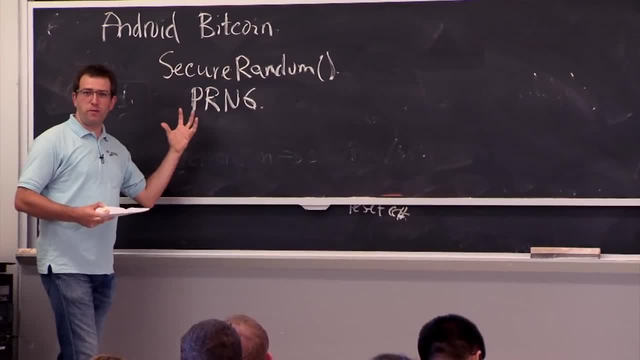 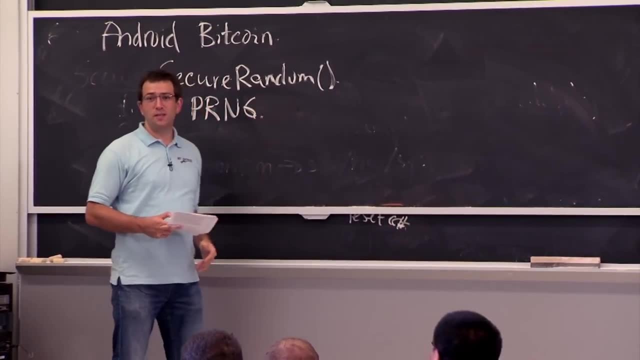 But nonetheless, another example of a small programming mistakes leading to pretty catastrophic results. You know lots of people got their Bitcoin balances stolen because of this weakness. Of course, the fix is pretty simple: at some level You change the Java implementation of secure random. 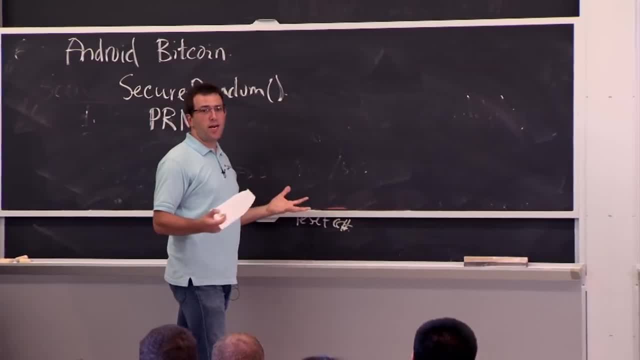 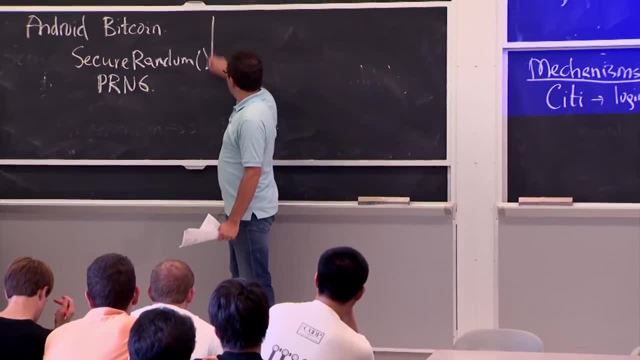 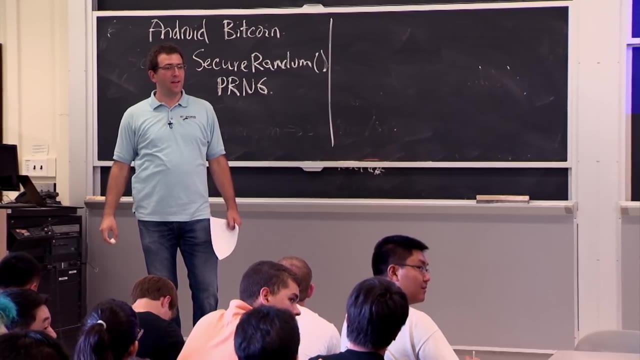 to always seed this PRNG with random input bits And then hopefully you're in good shape, But still it's a, you know, yet another example of mechanism failure. Yeah, Just to be clear, is this a different attack from the DSI signature randomness? 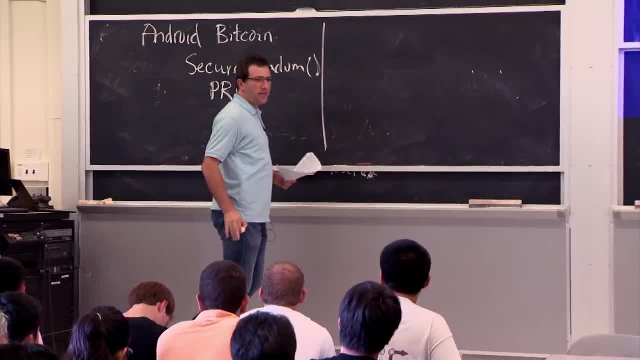 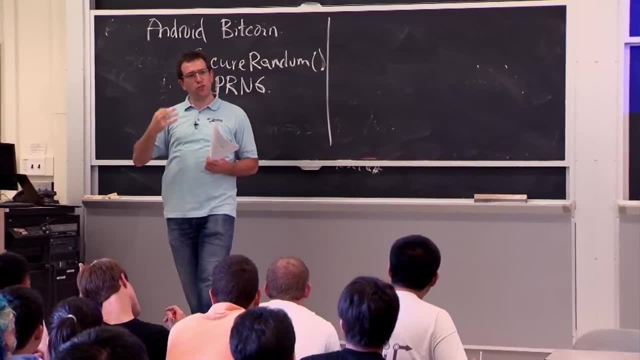 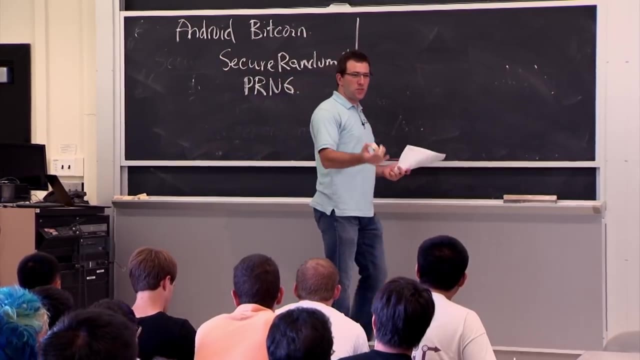 Well, yeah, So the actual problem is a little bit more complicated, as you were hinting at. The problem is, even if you didn't generate your key on the Android device in the first place, the particular signature scheme used by Bitcoin assumes that every time you generate a new signature. 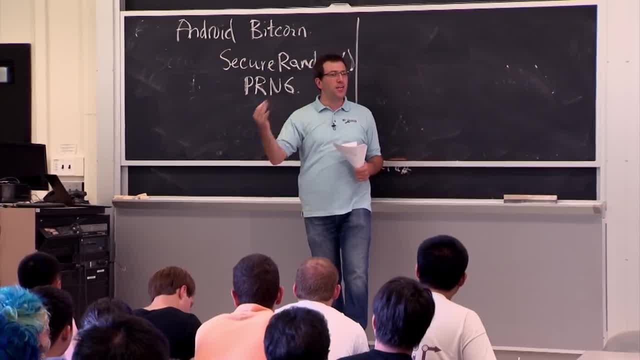 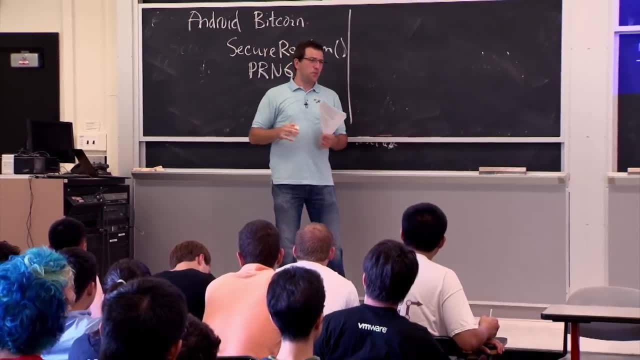 with that key, you use a fresh what's called a nonce for generating that signature, And if you ever generate two signatures with the same nonce, then someone can figure out what your key is. The story is pretty similar, but the details. 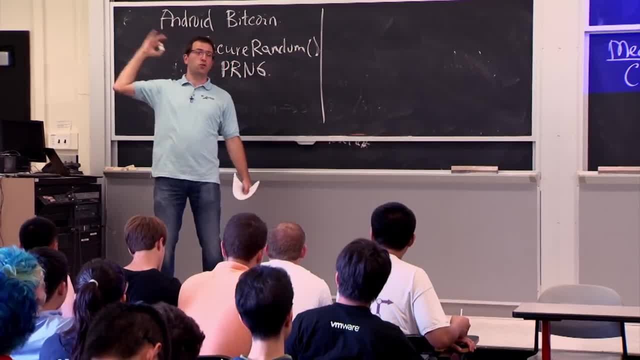 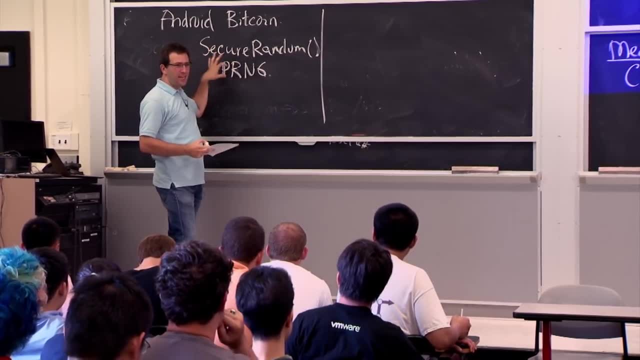 are a little different. So, yeah, so even if you actually generate your key somewhere else and your key was great, it's just that every time you generate a signature, you would- and you generated two signatures with exactly the same nonce or random value- someone. 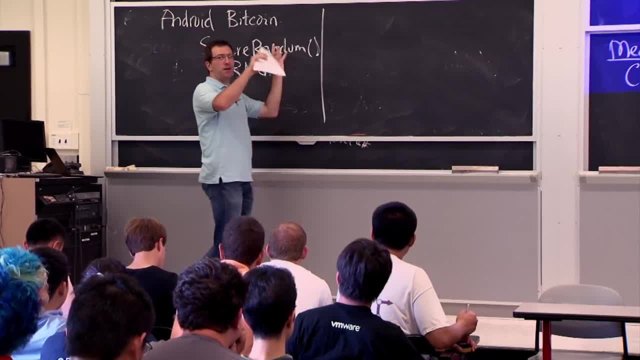 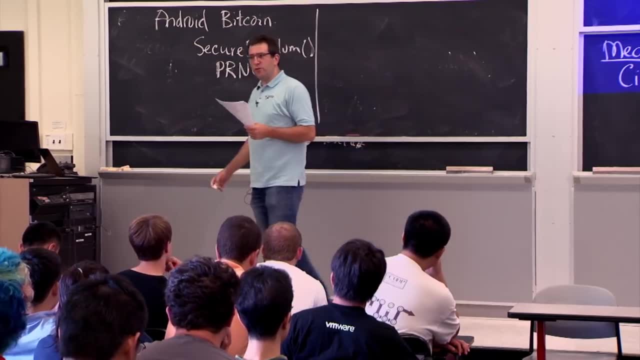 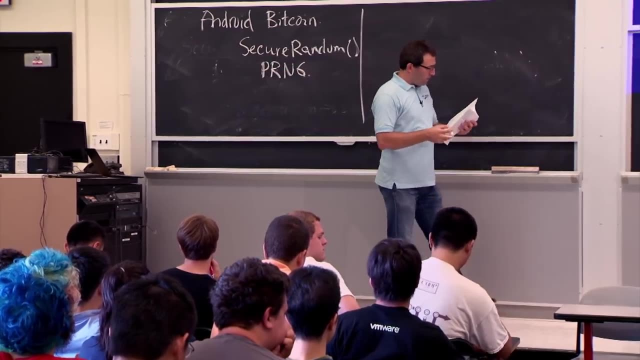 could apply some clever math to your signatures and sort of extract your public key out of it or private key more importantly. All right. Other questions about these problems, Examples, et cetera, All right, So I guess one thing I wanted to point out. 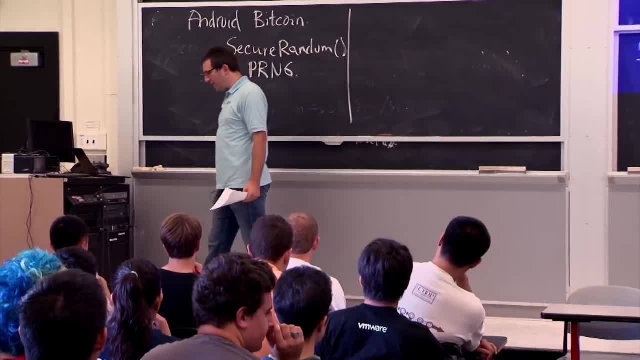 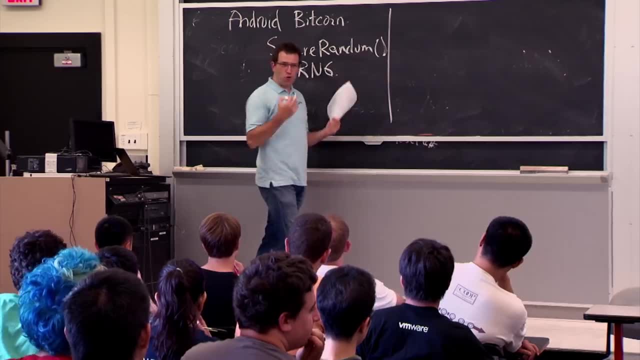 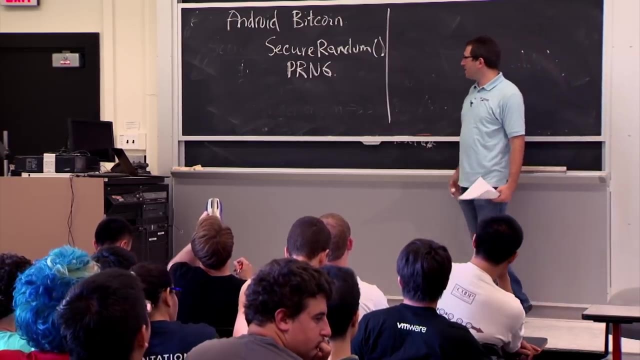 is that actually? well, as you're starting to appreciate, is that in computer security, almost every detail has a chance of really mattering, Like if you screw up almost something seemingly inconsequential, like forgetting to check something or this, or forgetting to initialize the random seed. 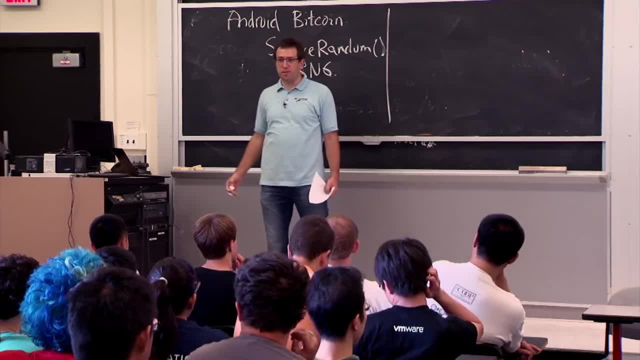 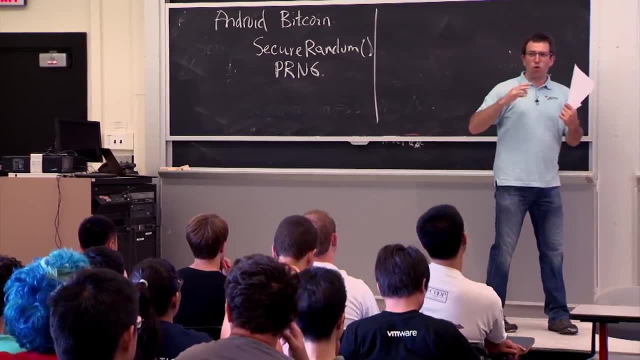 it can have pretty dramatic consequences for the overall system And you really have to be very clear about what is the specification of your system. what is it doing exactly? what are all the corner cases And a good way to think of breaking a system? 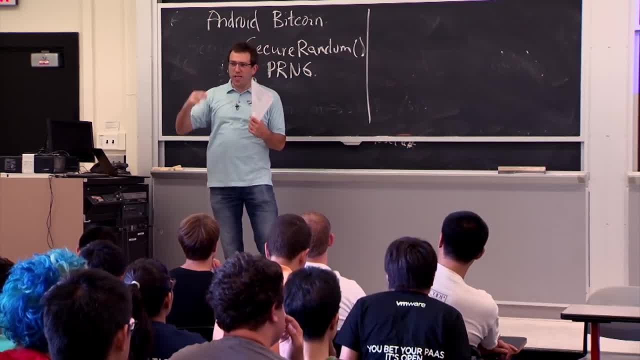 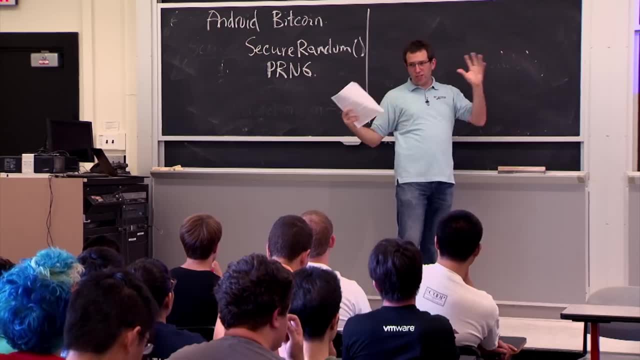 or, conversely, figuring out if your system is secure is to really push all the edge cases, Like what happens if my input is just large enough, Or what is the biggest or the smallest input, What is the strangest set of inputs I could provide to my program and push it. 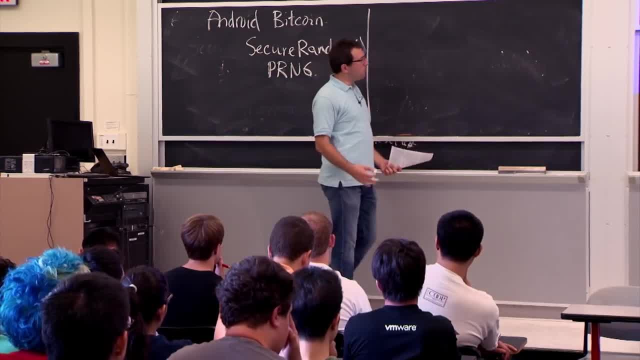 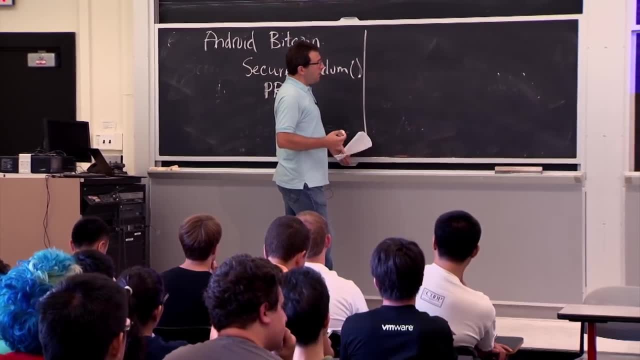 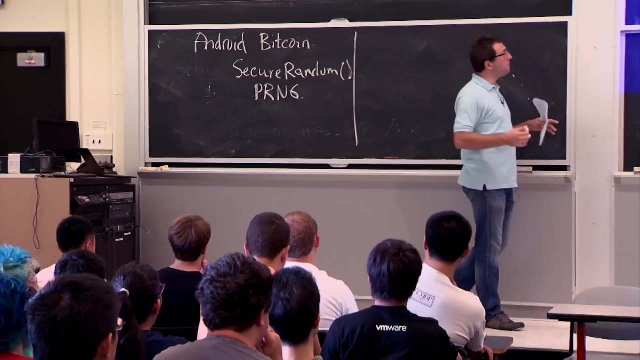 into all these corner cases. Maybe one example of this ambiguity- sort of a good example to keep in mind- is How SSL certificates again encode names into the certificate itself. So this is a different problem than the problem about the certificate authorities being trusted. 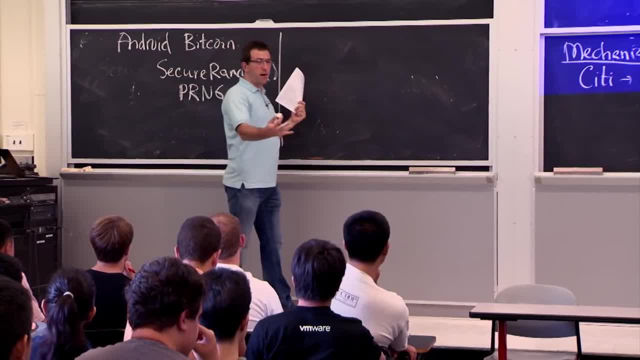 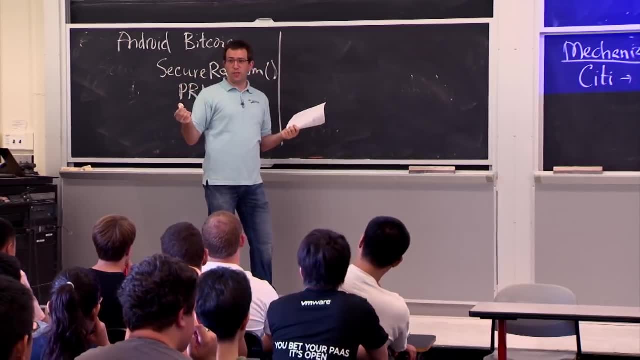 So these SSL certificates are just sequences of bytes that a web server sends to you, And inside of this SSL certificate is the name of the server you're connecting to, So something like Amazoncom. You can't just put down those bytes, You need to encode it somehow and specify: well it's. 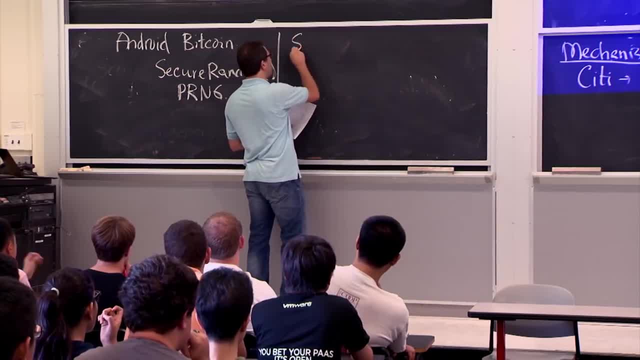 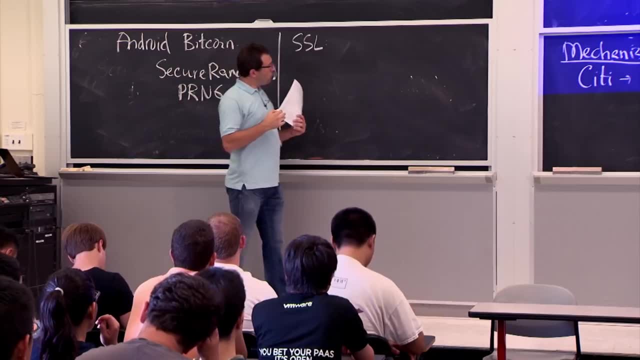 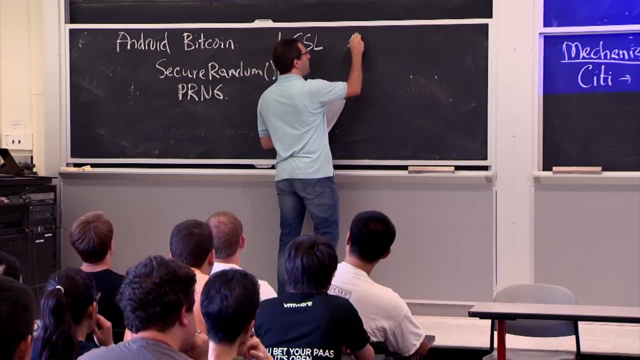 Amazoncom, And that's the end of the string. So in SSL certificates they use a particular encoding scheme that writes down Amazoncom, But by first writing down the number of bytes in the string. So you first write down. OK, well, 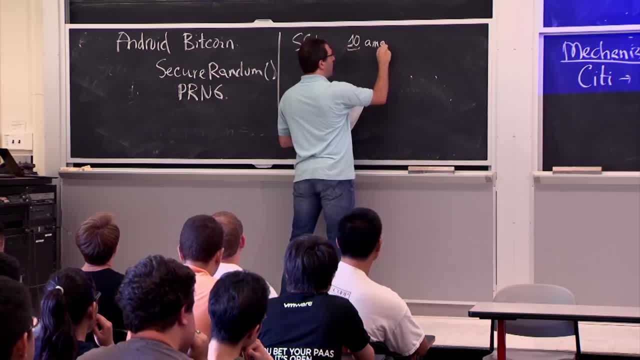 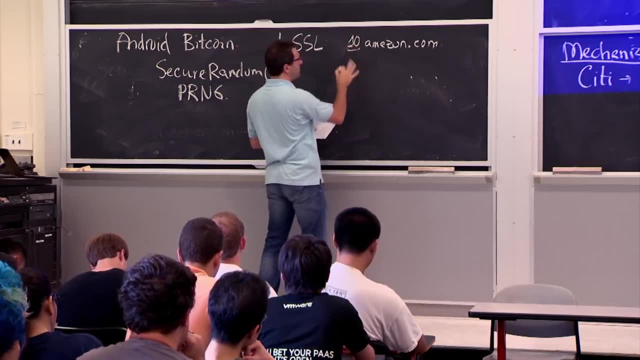 I'm going to have a 10-byte string called Amazoncom. It's actually 10 bytes, Great, OK. So this is like in the SSL certificate. somewhere in there there is this byte 10, followed by 10 bytes saying what the host name is. 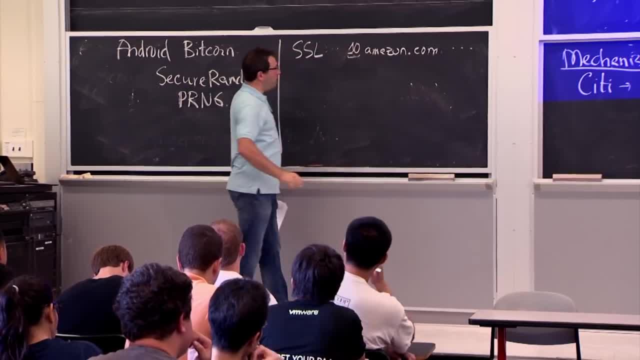 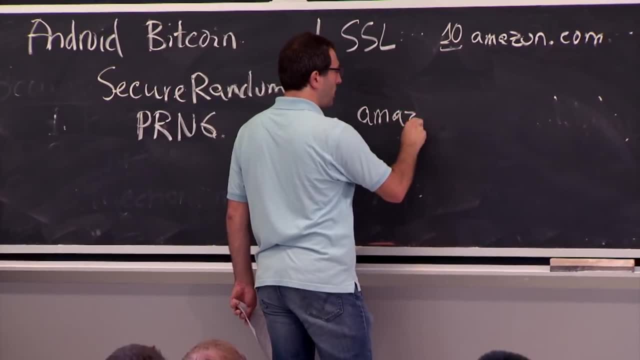 And there's other stuff afterwards and before And when a browser takes it. well, the browser is written in C, And the way C represents strings is by null, terminating them. So in C a string doesn't have a length count. Instead it has all the bytes. 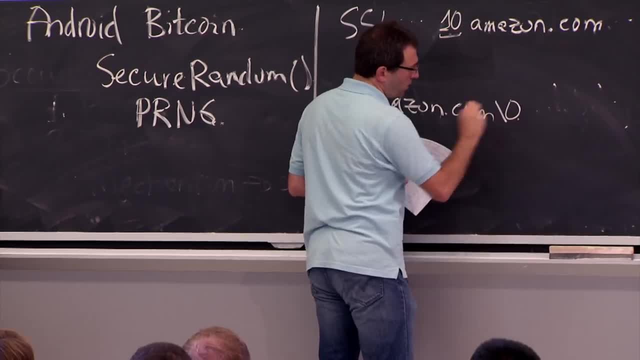 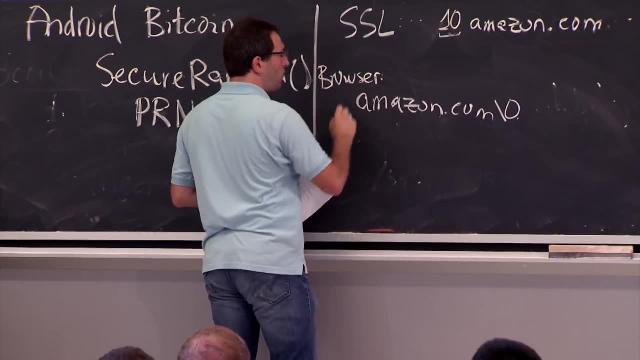 And the end of the string is just the byte 0. And in C you sort of write it with a backslash 0 character. So this is in memory in your browser. Somewhere in memory there's this string of 11 bytes now. 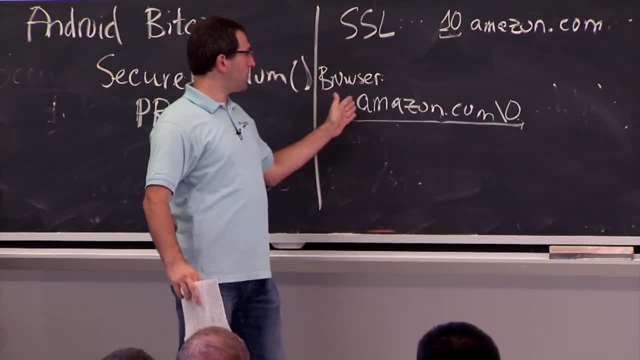 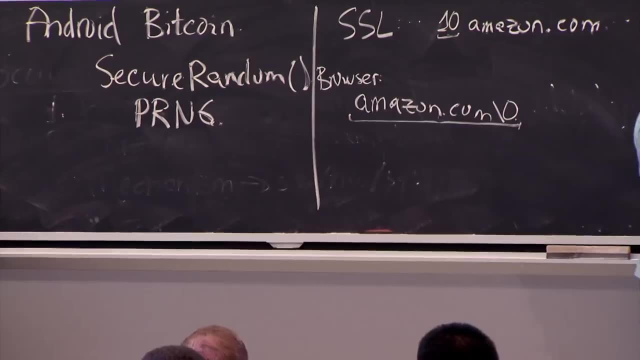 with an extra 0 at the end, And when a browser interprets the string, it just keeps going until it sees an end of string marker, which is the 0 byte. OK, So what can go wrong? Any guesses? Yeah? 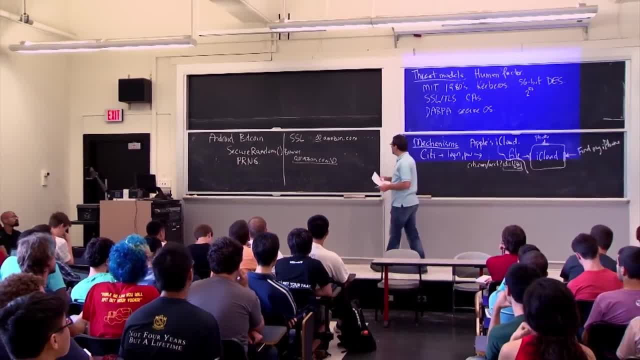 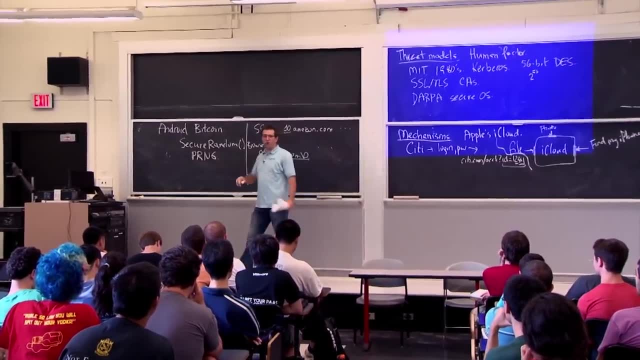 You can have a 0 in the middle of your string. Yeah, This is great. So this is actually like a bit of a discontinuity in terms of how this guy represents strings and this guy, So suppose that I own the domain Foocom. 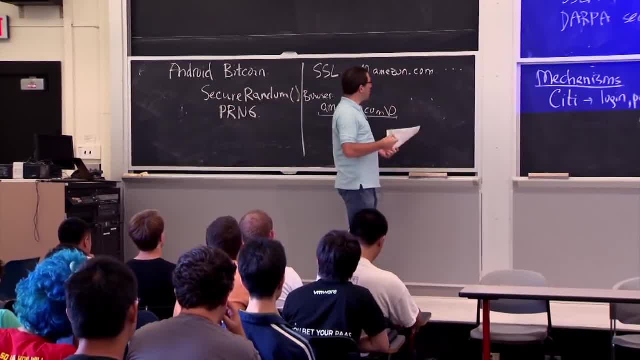 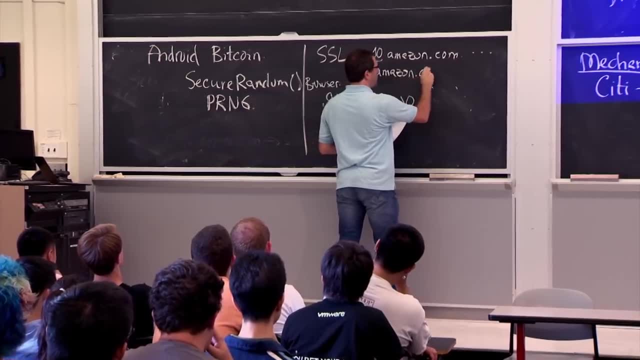 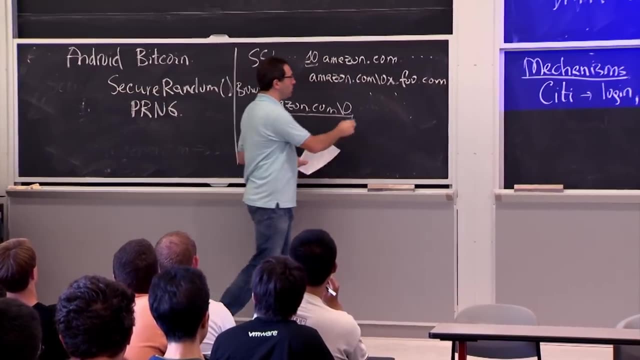 So I can get certificates for anythingfoocom. So what I could do is ask for a certificate for the name amazoncom0xfoocom. That's a perfectly valid string. It has a bunch of bytes. I guess it's 10,, 11,, 12,, 13,, 14,, 15,, 16, there's another 4,, 20.. 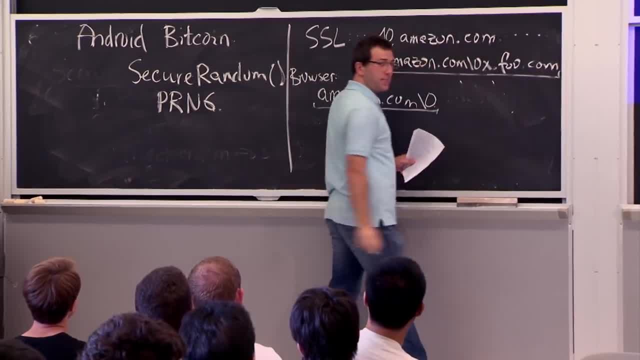 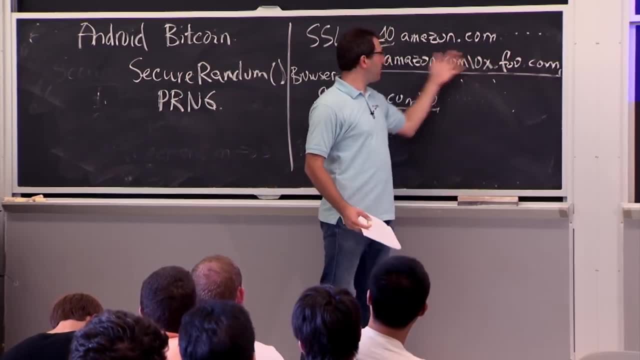 So this is a 20 byte name with these 20 bytes. So It used to be that if you go to a certificate authority, in many cases you could say: hey, I own foocom, Give me a certificate for this thing. 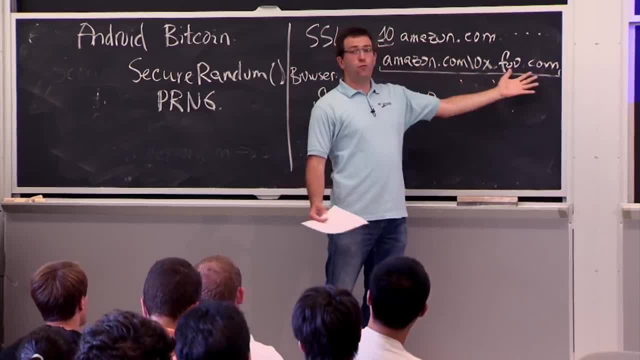 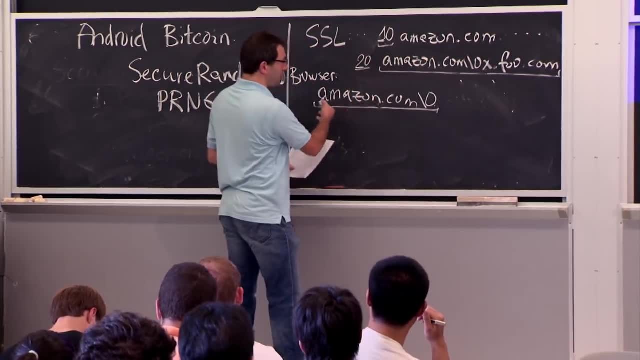 And they'd be perfectly willing to do it, because it's a subdomain of foocom, It's all yours. But then when a browser takes this string and loads it in memory, well, what it does is the same thing it did here. 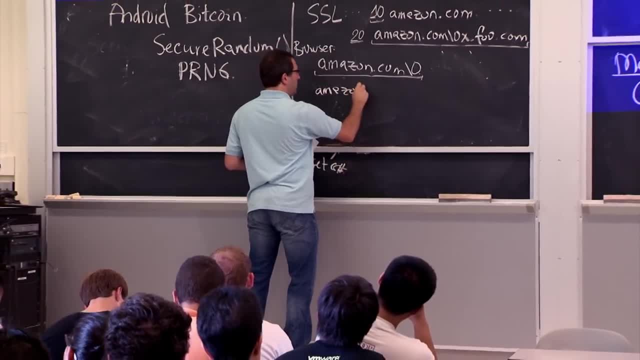 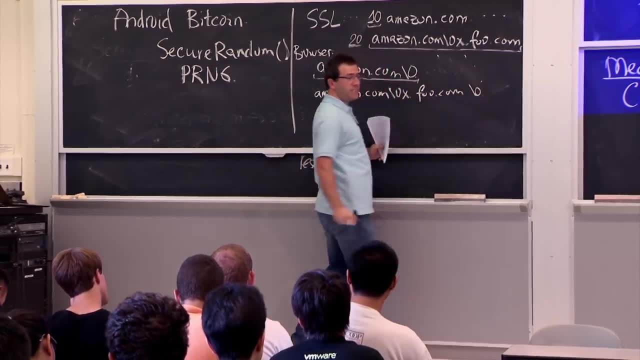 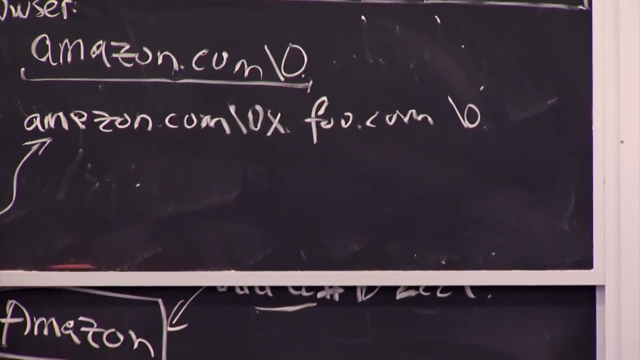 It copies the string amazoncom backslash- 0xfoocom, It'll dutifully add the terminating 0 at the end. But then when the rest of the browser software goes and tries to interpret the string at this memory location, it'll keep going up until it gets to 0 and say OK. well, 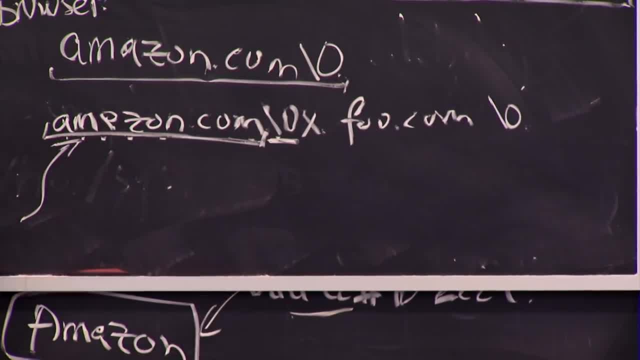 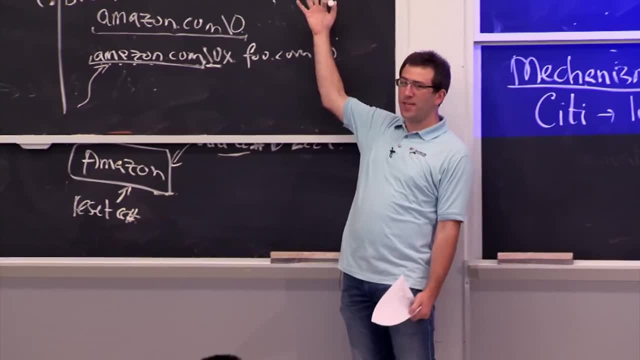 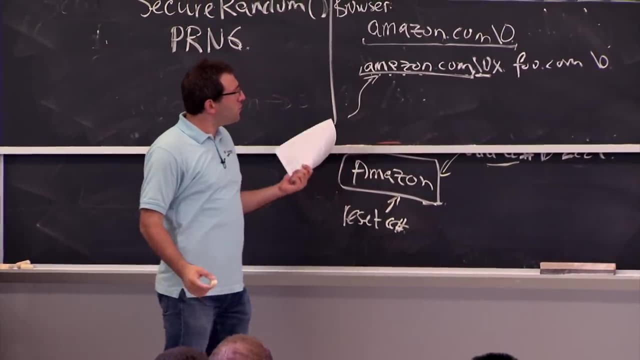 that's the end of the string. So this is amazoncom. That's it. So this sort of disconnect between how C software and how SSL certificates represent names led to some unfortunate security problems. This was actually discovered a number of years ago now by this guy, Moxie Marlinspike. 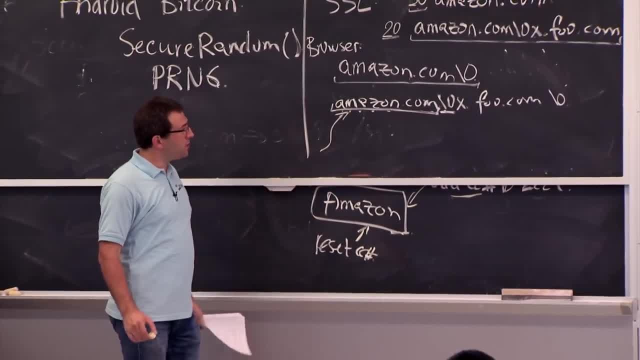 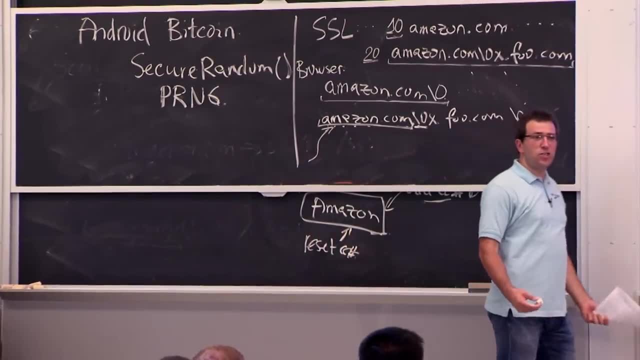 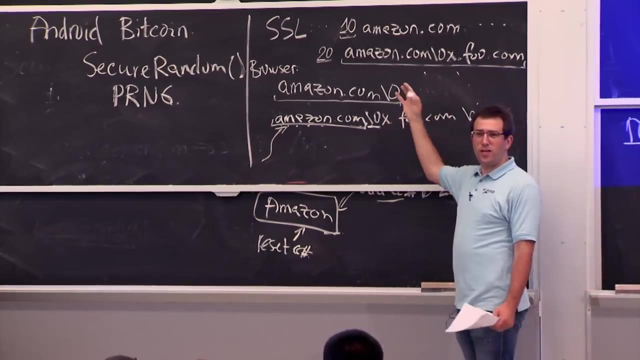 But it's a fairly clever observation And these kinds of encoding bugs are actually also pretty common in lots of software, because unless you're very diligent about exactly how you encode things, there might be different ways of encoding And whenever there's disagreement. 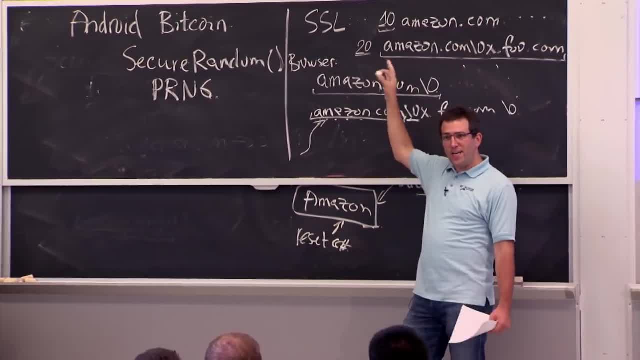 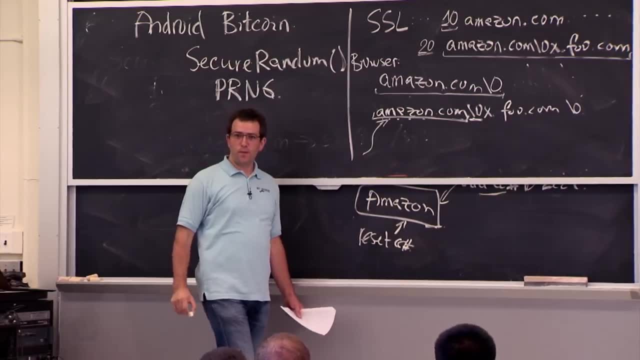 there's a chance the bad guy can take advantage of this. One system thinks that's a fine name, Another thinks that's something else. So these are good places to sort of push a system to see how it might break That make sense. 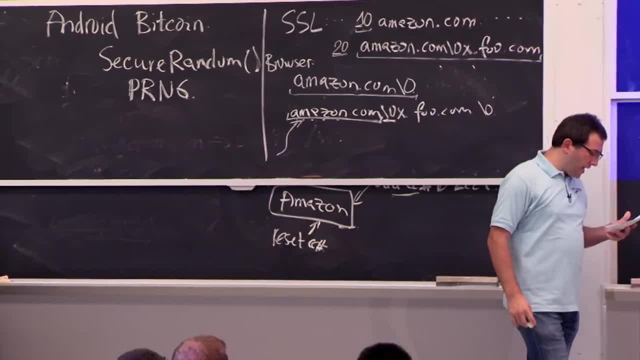 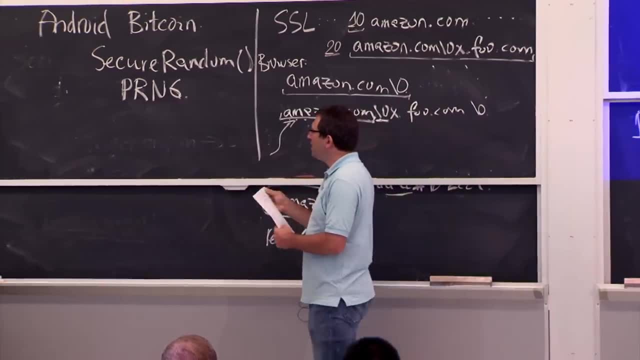 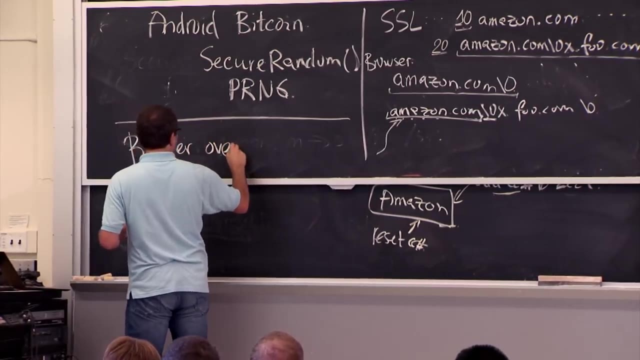 All right. so maybe the last example of mechanism failure I'm going to talk about today- it's a reasonably popular one- is this problem of buffer overflows. So some of you have seen this, or at least at some level in 6.033 if you did the undergrad course. 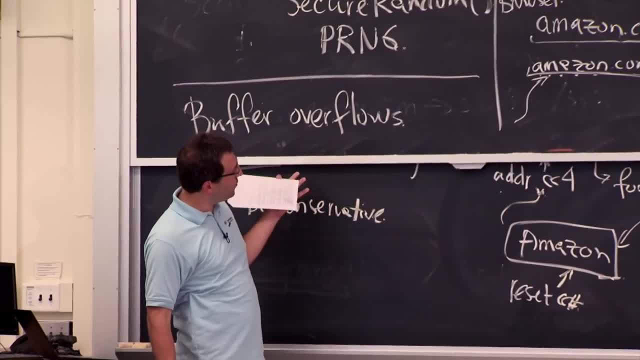 But for those of you that have forgotten or haven't taken 0.3.3,, we'll sort of go over buffer overflows in more detail And this will be actually a little bit more interesting. It's going to be quite critical for you guys. 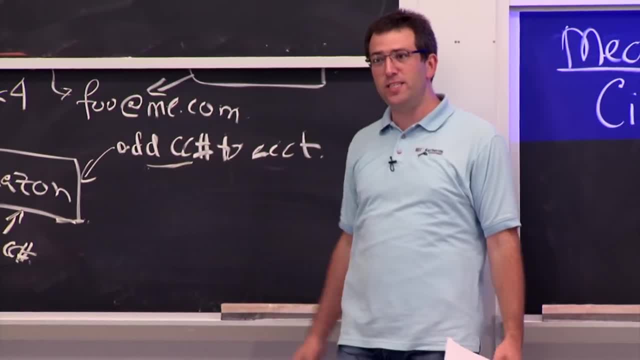 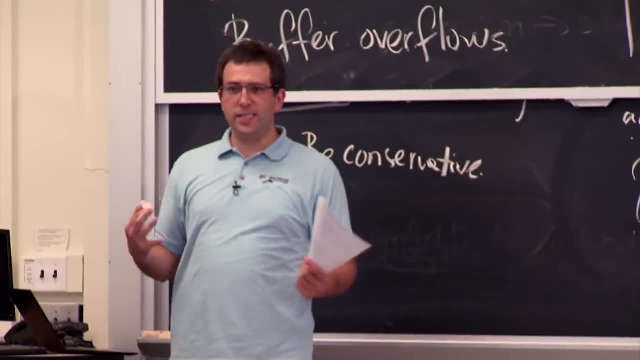 because Lab 1 is all about buffer overflows And you're going to be exploiting these vulnerabilities in a somewhat real web server. So let's figure out. what is the setting. What are we talking about here? So, a setting we're going to be considering. 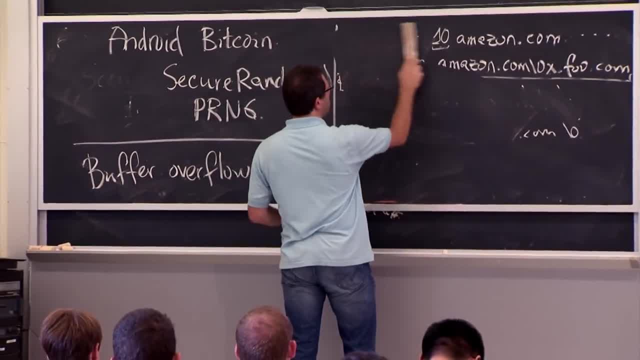 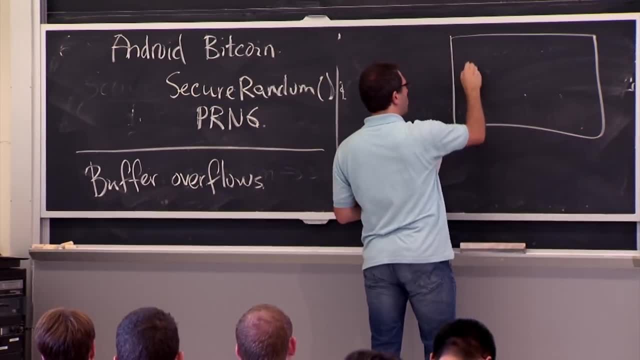 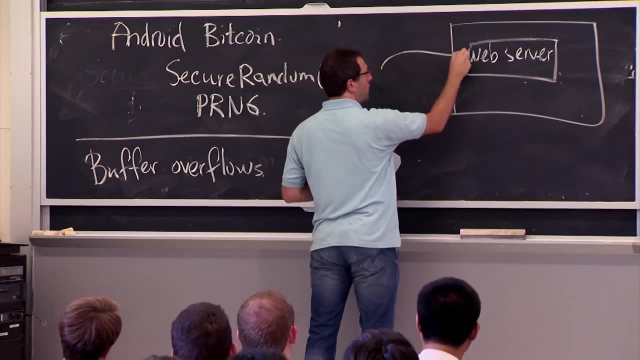 is a system which has, let's say, a web server. So what we have is we have some computer out there that has a web server on it And the web server is a program that is going to accept connections from the outside world. 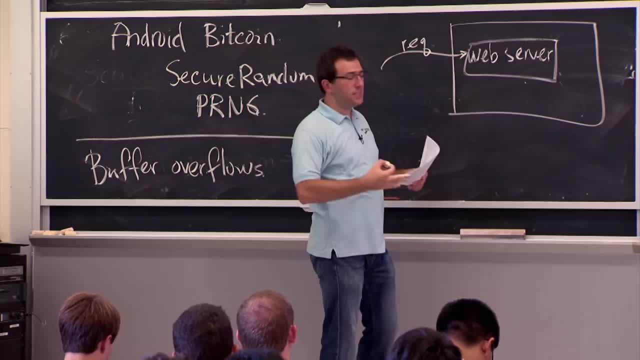 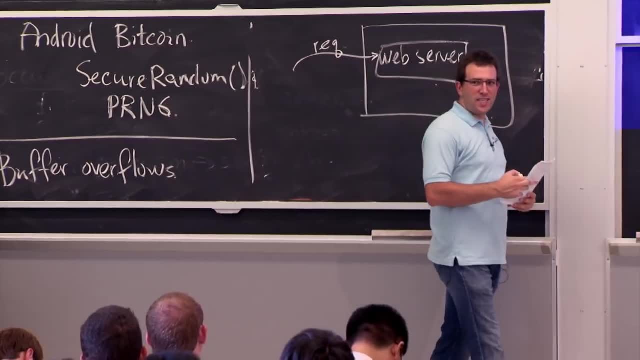 take requests which are basically just packets and somehow process them and do some checking, probably if it's an illegal URL or if they're trying to access a file they are not authorized to access. The web server is going to return an error. 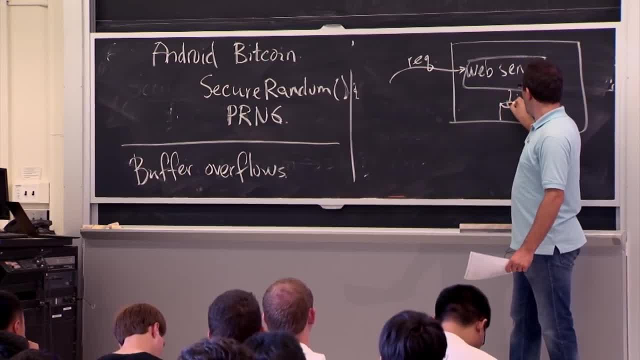 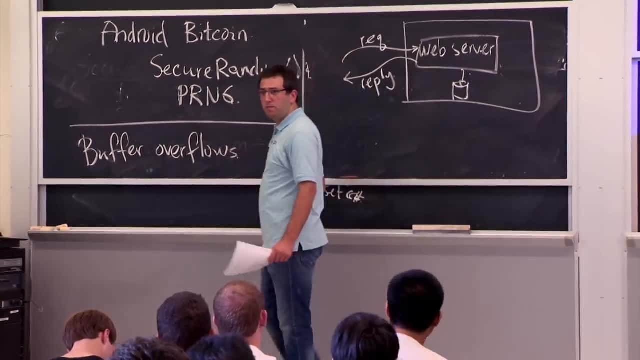 But otherwise it's going to access some files, maybe on disk, and send them back out in some sort of a reply. So this is a hugely common picture. OK, So let's figure out what is the system we're talking about here. 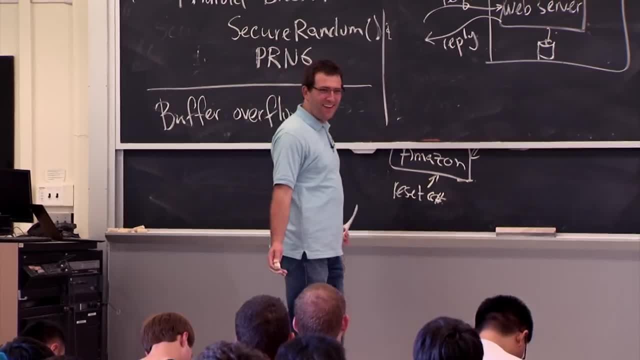 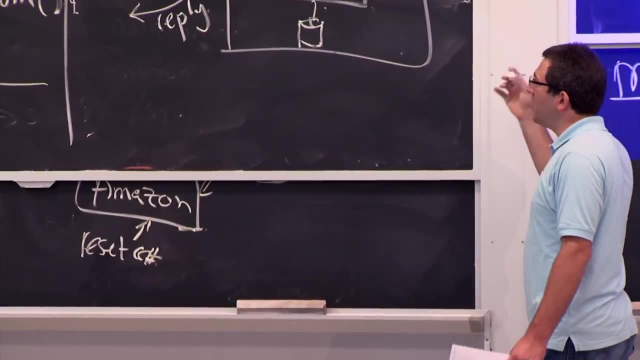 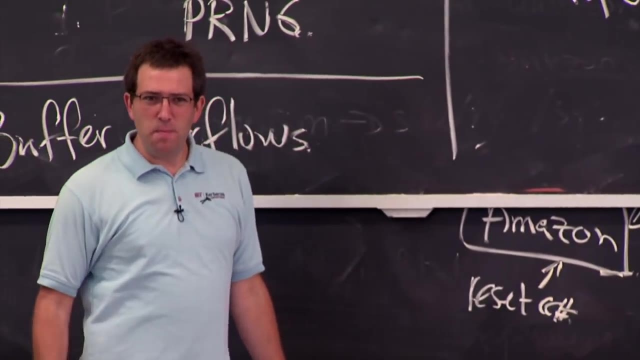 What's the policy Or what's the threat model. So this is a bit of a problem in many real world systems, namely that it's actually pretty hard to pin down what is the exact policy or threat model that we're talking about, And this sort of imprecision or ambiguity about policies. 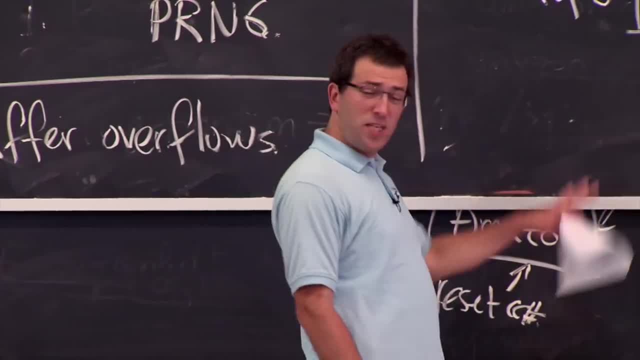 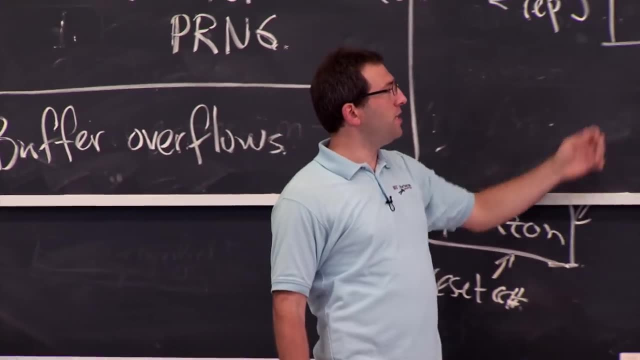 threat models et cetera, is what sometimes leads to security problems- Not in this particular case, but we'll see. But maybe just to give you a little bit of a sense of how to think of a typical web server in the context of this policy: threat model kind. 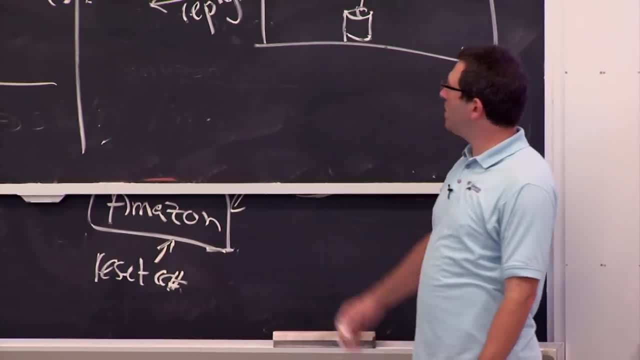 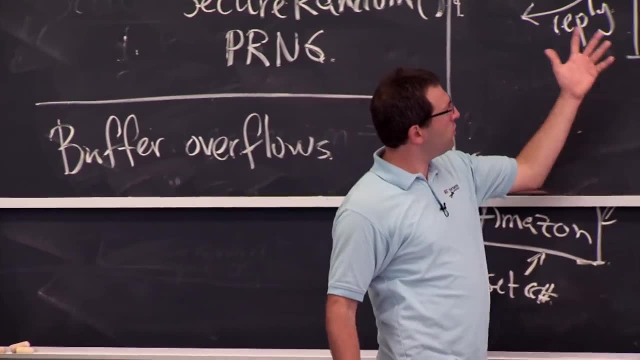 of stuff. is that? well, probably the policy is, the web server should do what the programmer intended it to do. It's all vague, but that's probably what's going on, Because anything more specific is well, the web server should do exactly what that code does. 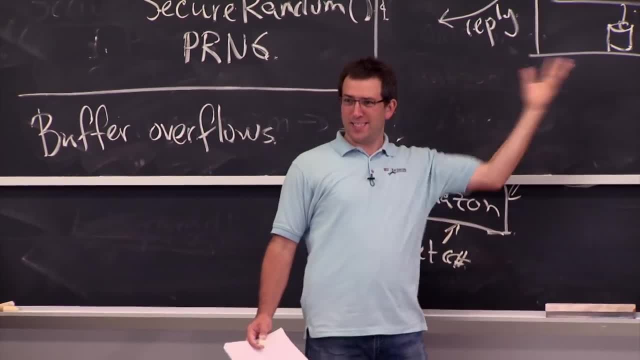 It's going to be a bit of an op, And if a code has a bug, well, your policy says: well, that's exactly what I should do. I should follow the bug. So it's a little hard to state a policy precisely. 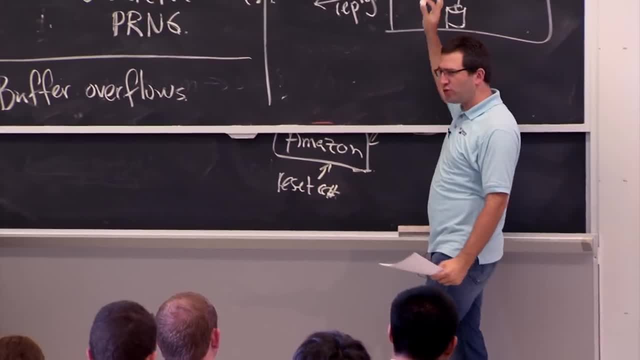 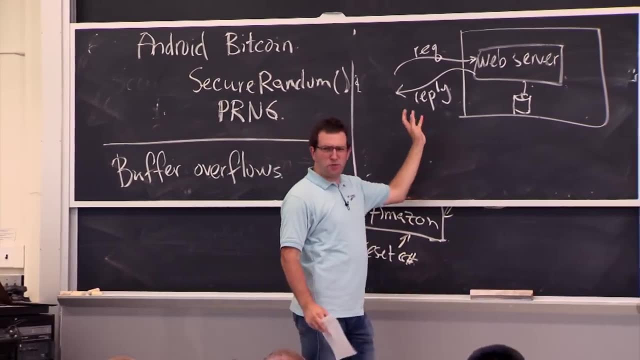 But in this case let's go with, you know, some intuitive version of: well, the web server should do what the programmer wanted it to do, And the threat model is probably that the attacker doesn't have access to this machine, can't log into it remotely. doesn't have physical access to it but can send any packet they want, So they're not restricted to certain kinds of packets. Anything it can shape and deliver to this web server, that's fair game. Seems like a reasonable threat model in practice to have. 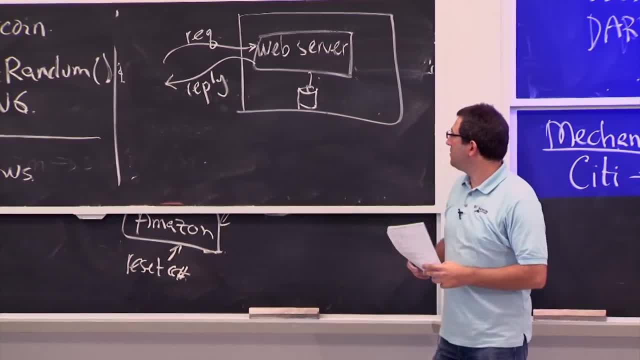 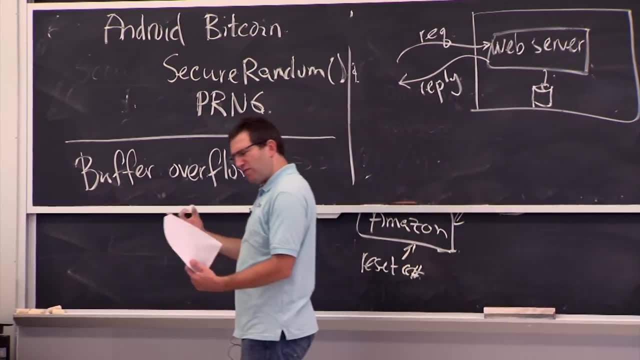 in mind, And I guess the goal is that this web server shouldn't allow arbitrary stuff to go wrong here. I guess it sort of goes along with what the programmer intended. The programmer probably didn't intend any request to be able to access anything on the server. 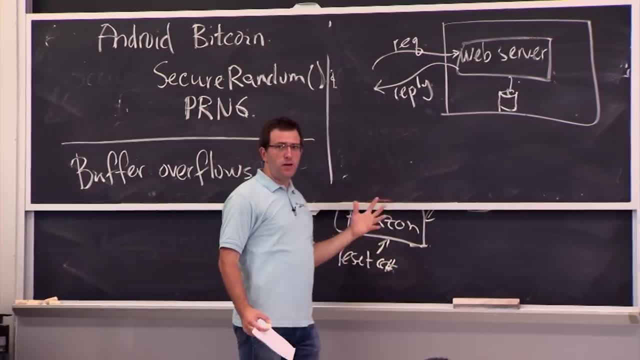 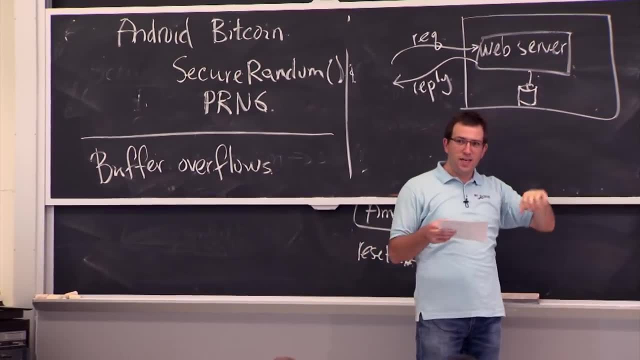 And yet it turns out, if you make certain kinds of mistakes in writing, the web server software, which is basically the mechanism here, the web server software is the thing that takes a request and looks at it and makes sure that it's not going to do something bad. 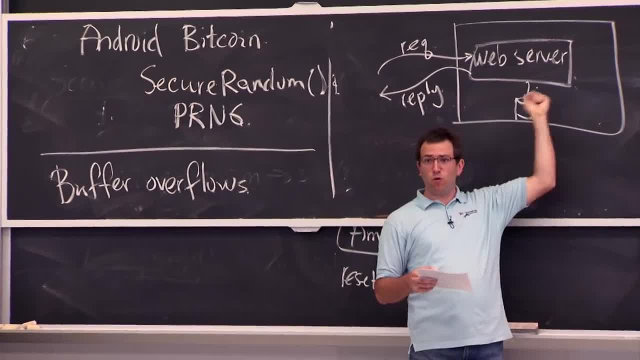 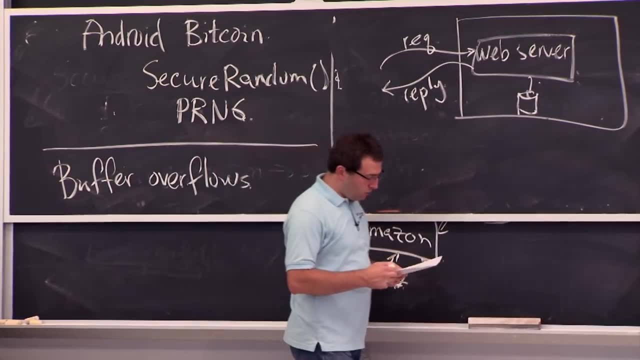 sends a response back if everything's OK. The web server is this mechanism. It's enforcing your policy And, as a result, if the web server software is buggy, then you're in trouble, And one sort of common problem if you're writing software. 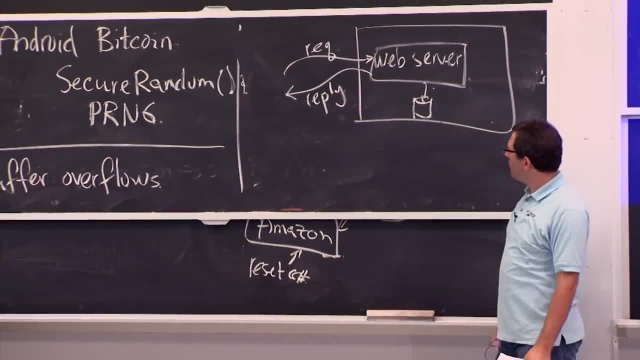 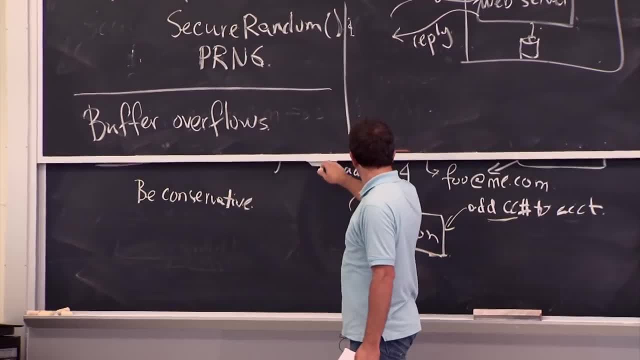 in C, which many things are still written in C and probably will continue to be written in C for a while. you can mismanage your memory allocations And, as we saw in this SSL certificate naming example, even sort of a single byte can really 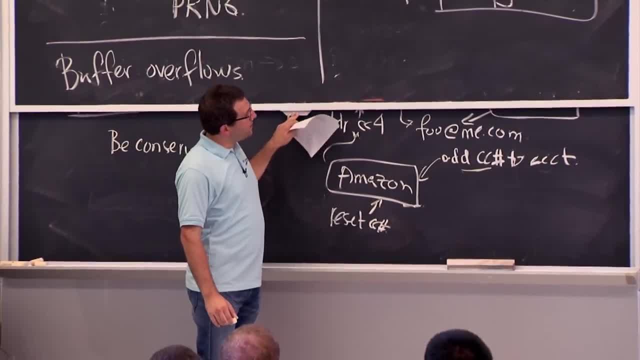 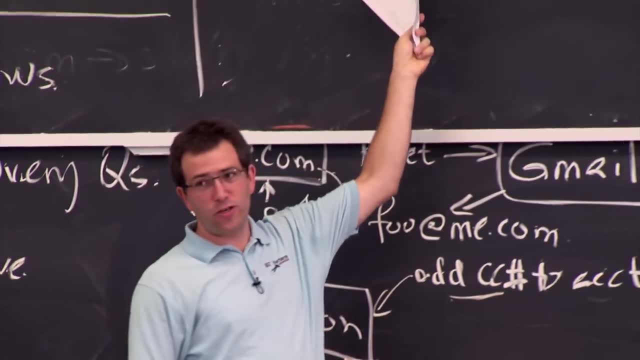 make a huge difference in terms of what goes on, And I guess for this example we'll look at a small piece of code that's not quite a real web server. In the lab you'll have this whole picture to play with, But for lecture I just want to give you a simplified example. 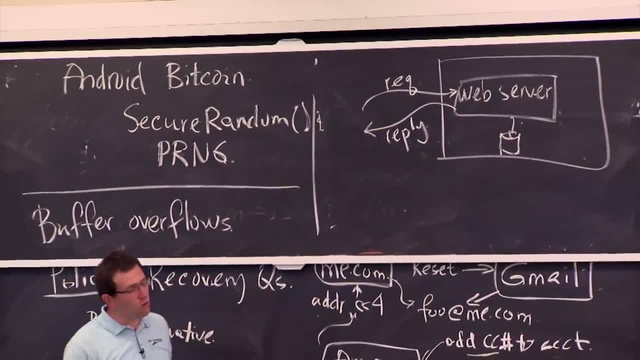 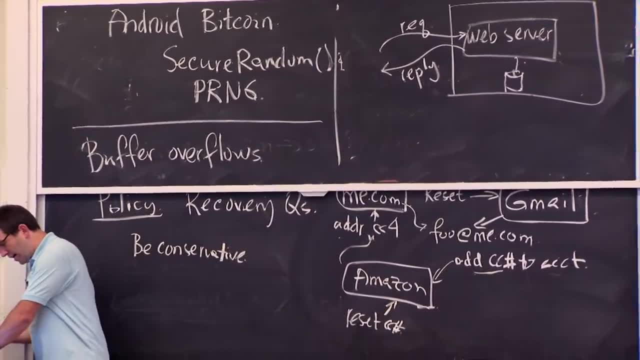 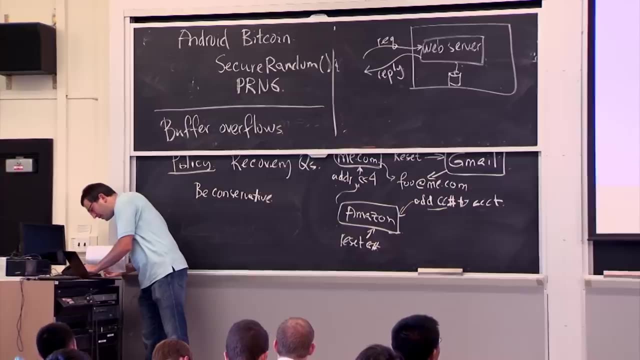 so we can talk about what's sort of at the core of what's going wrong. And in particular, if the system wakes up, I will show you sort of a very small C function And we can sort of see what goes wrong if you provide different inputs to that piece of code. 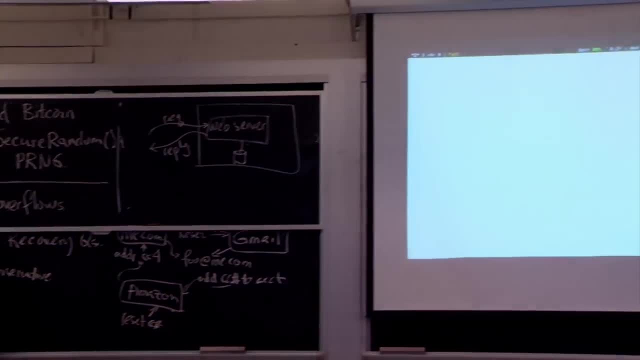 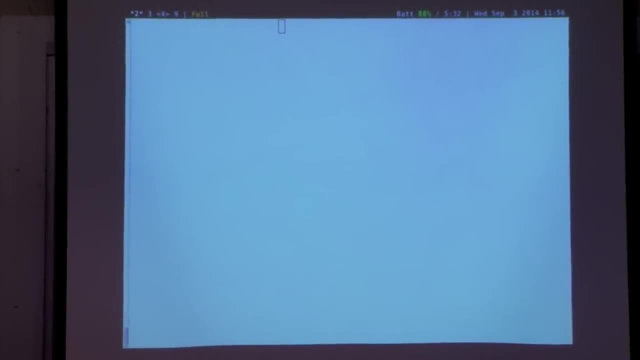 All right. So the C function that I have in mind is a This guy, let's see somewhere here I can. oh yeah, All right. So here's the sort of program I'm talking about, or I want to use as an example here. 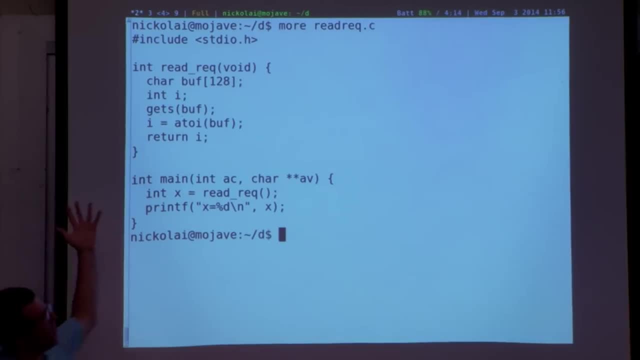 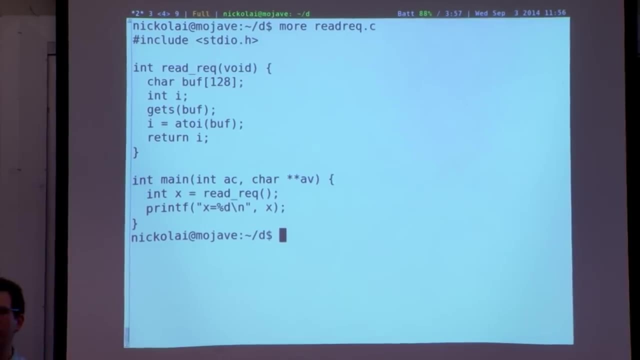 So this program is just going to read a request And you can sort of imagine it's going to read a request from the network. But for the purposes of this example, it's just going to read a request from whatever I'm typing in on the keyboard. 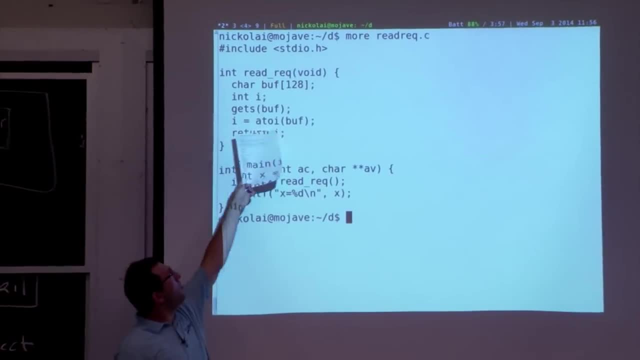 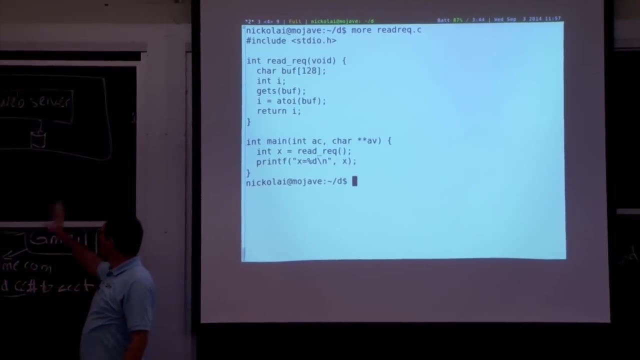 And it's going to store it in a buffer here And then it's going to parse it as an integer and return the integer And the program will then print whatever integer I get back. It's far from a web server, but we'll. 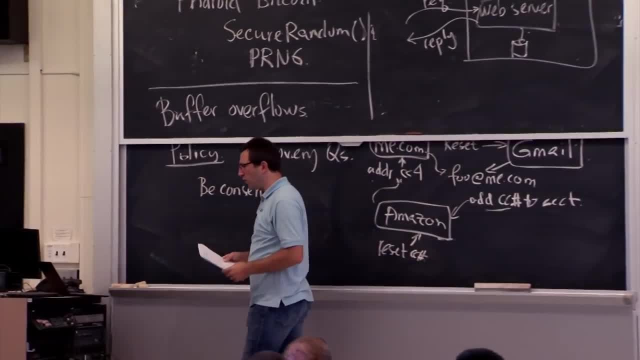 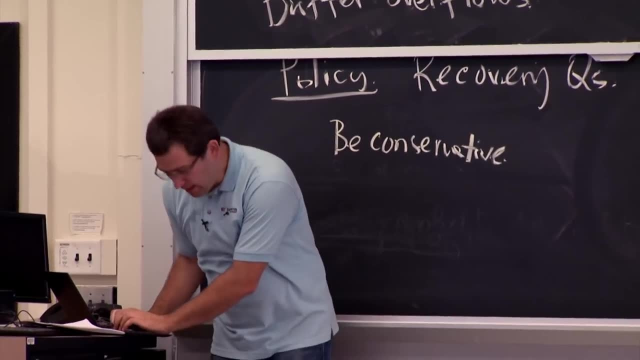 at least see some basics of how buffer flows work and what goes wrong. So let's see actually what happens if we run this program, So I can compile it here And actually you can sort of see the It's already telling me what I'm screwing up, right? 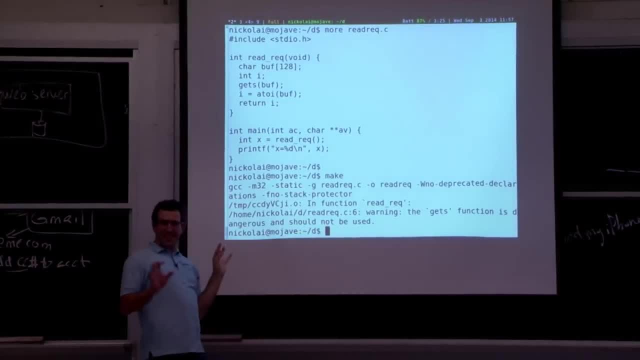 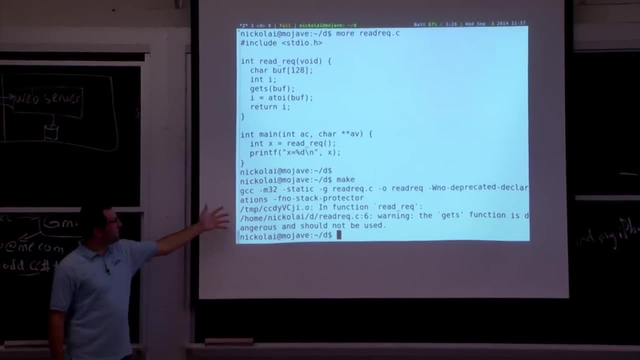 The get function is dangerous and should not be used, And we'll see in a second why the compiler is so intent on telling me this, And it actually is true. But for now, suppose we're a happy-go-lucky developer that is willing to ignore this warning. 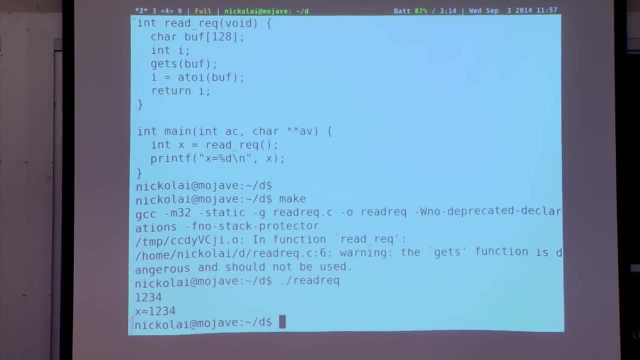 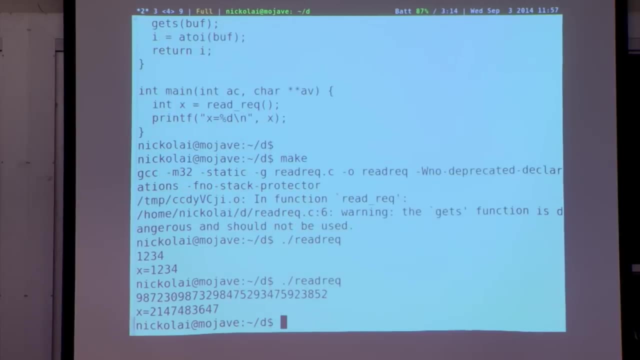 So OK, I run this redirect function, I provide some input And it works. Let's see if I provide large inputs. If I type in some large number, Well, At least it gives me some large number. It basically maxes out to 2 to the 31 and prints that. 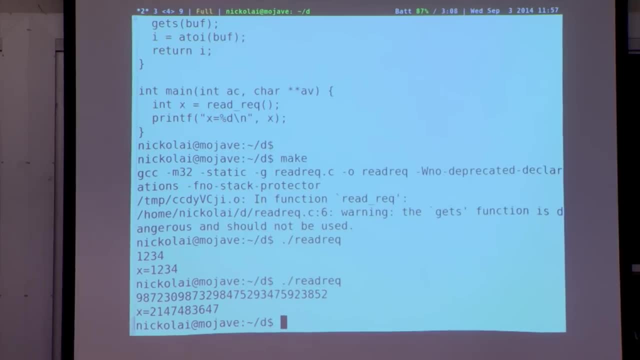 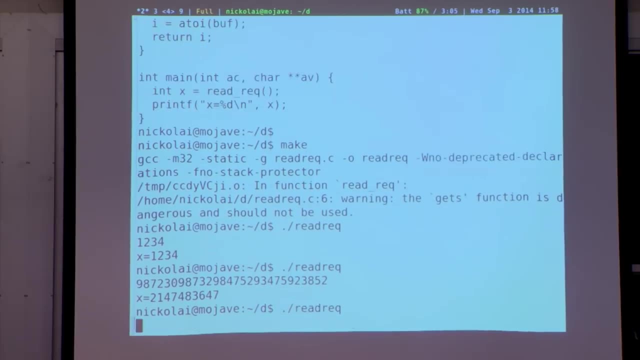 and doesn't go any higher, That's maybe not disastrous, right? Whatever You provided us this ridiculously large number, You got something that didn't quite work, So it's not quite a problem yet, But if we provide some really large input, 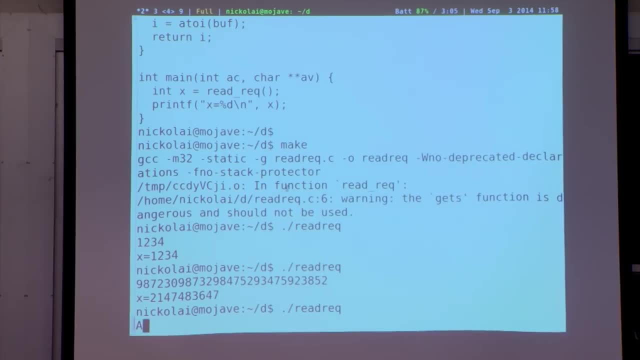 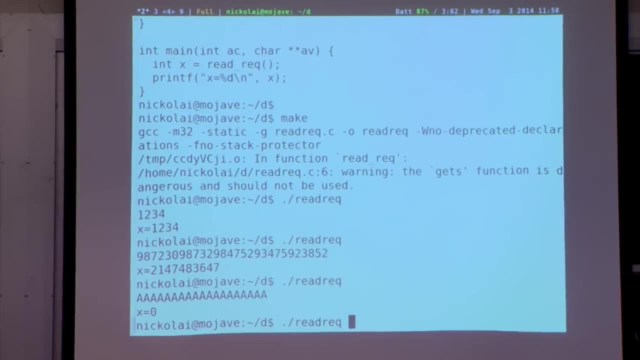 we might get some other problems right. So suppose I provided a lot of bytes. Well, if I just provided things that are not numbers, print 0. That's not so bad, But suppose I'm going to paste in a huge number of As. 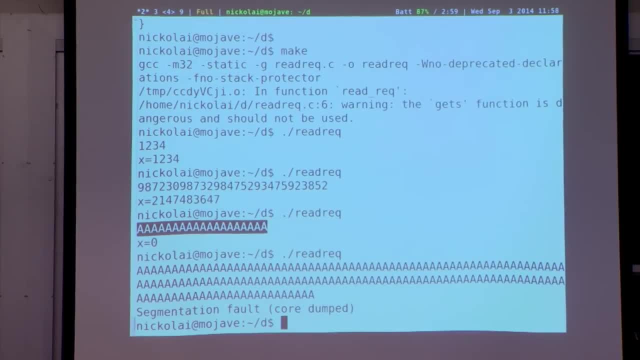 OK, so now the program crashes right. Maybe not too surprising. So if it was the case that if I sent a bad request to a web server, it just doesn't get back to me or doesn't send a reply, that would be fine. 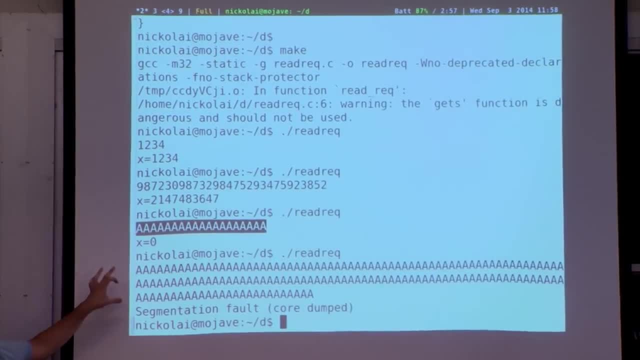 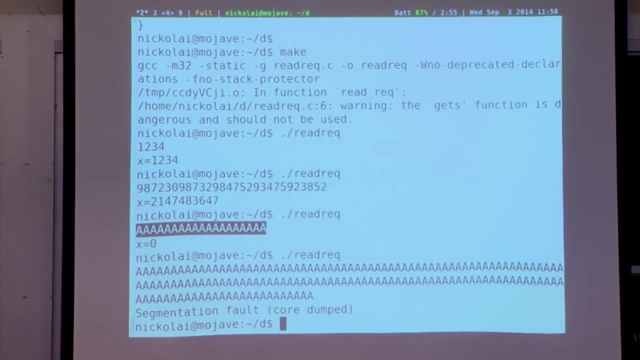 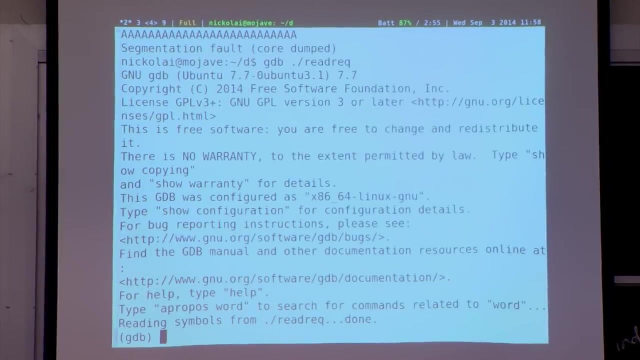 But we'll sort of look inside and see what happens and try to figure out how we can actually take advantage of this crash to maybe do something much more interesting or well, much more along what that attacker might be Interesting in doing. So to do this, we're going to run this program under a debugger. 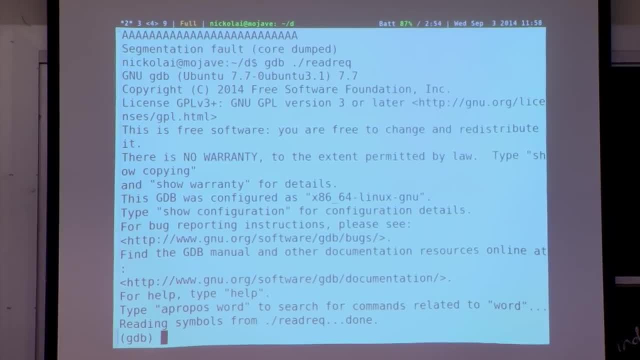 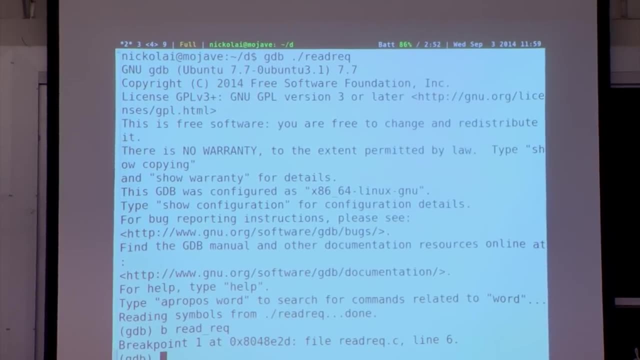 You'll get super familiar with this in lab one. But for now what we're going to do is set a break point in that redirect function And we're going to sort of run along and see what happens. So when I run the program it's going. 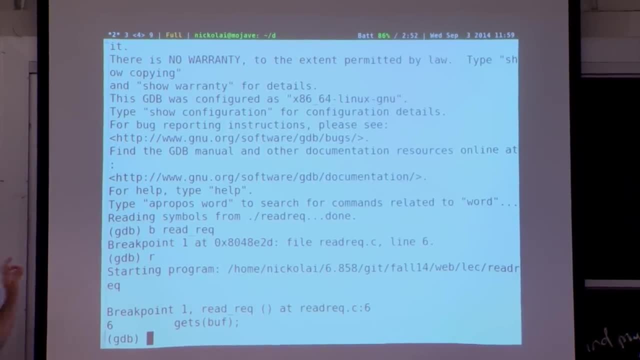 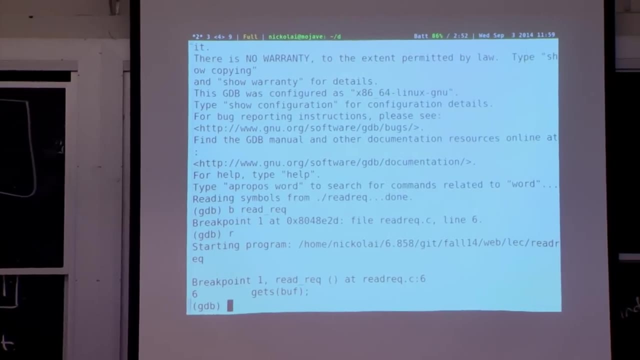 to start executing in the main function And pretty quickly it calls redirect And the debugger is now stopped at the beginning of redirect And we can actually see what's going on here. For example, we can ask it to print the current CPU registers. 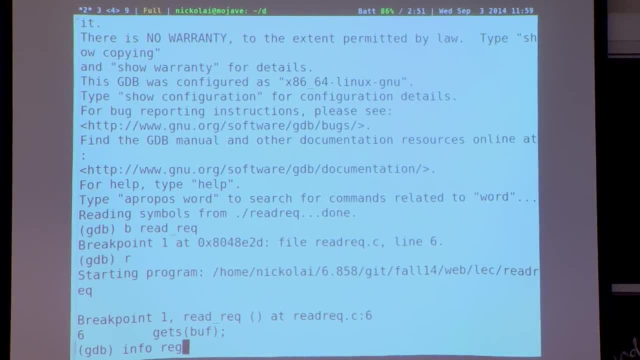 We're going to look at really low level stuff here, as opposed to at the level of C source code. We're going to look at the actual instructions that my machine is executing, Because that's what really is going on. The C is actually maybe hiding some things from us. 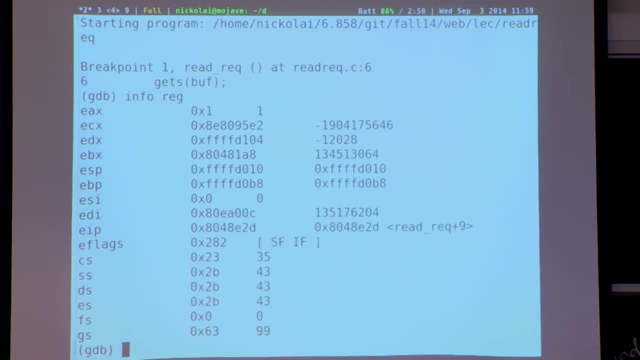 So you can actually print all the registers. So on x86,, as you might remember from well, on any architecture there's a stack pointer. So let me start maybe drawing this diagram on the board so we can try to reconstruct what's happening. 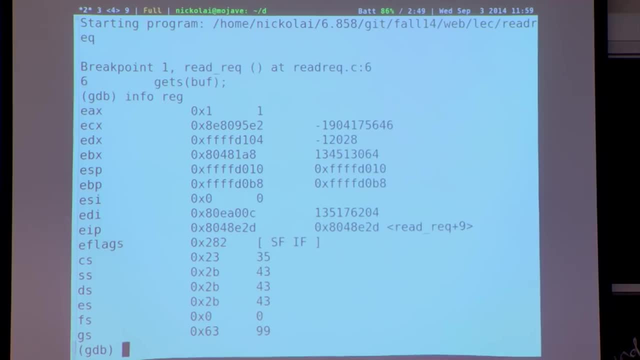 So what's going on is that my program, not surprisingly, has a stack On x86, the stack grows down, So it sort of is this stack like this And we can keep pushing stuff onto it. So right now the stack pointer points. 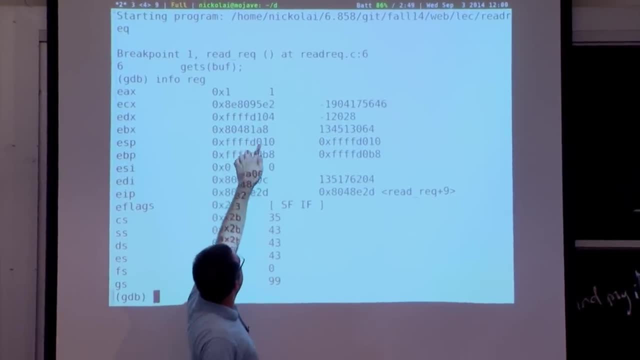 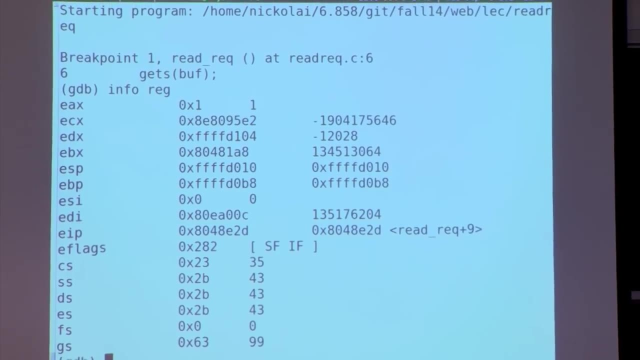 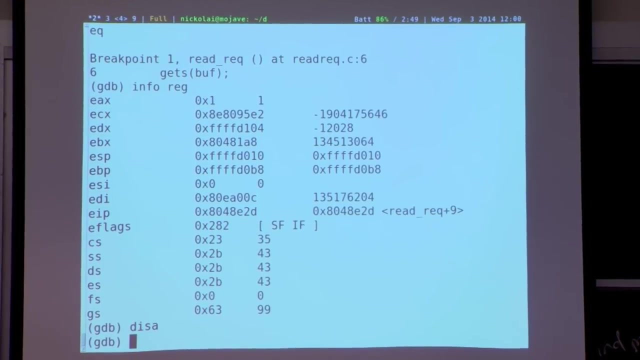 at this particular memory location, FFD010.. So some value, So we can try to figure out. how did it get there? One way to do it is to disassemble the code of this redirect function. Is that going to work better? 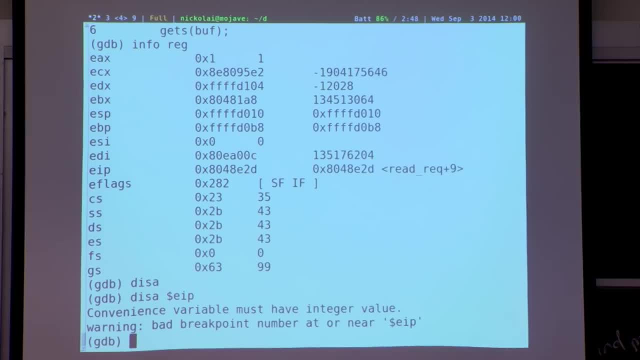 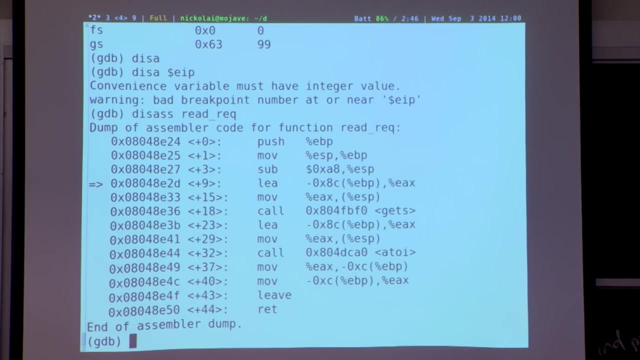 Really, Convenience variable must have integer value. Break my number, Man. What is going on with my debugger Redirect? Well, we can disassemble the function by name. So this is what the function is doing. So, first off, it starts by: you know. 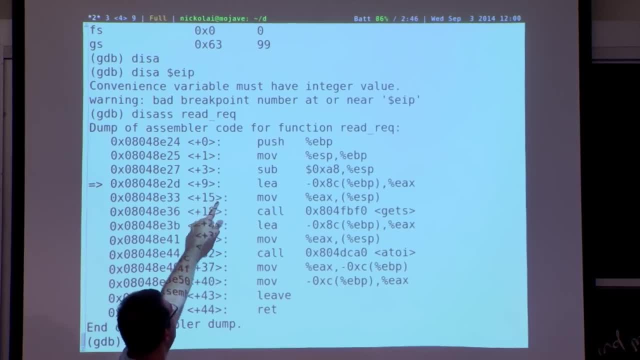 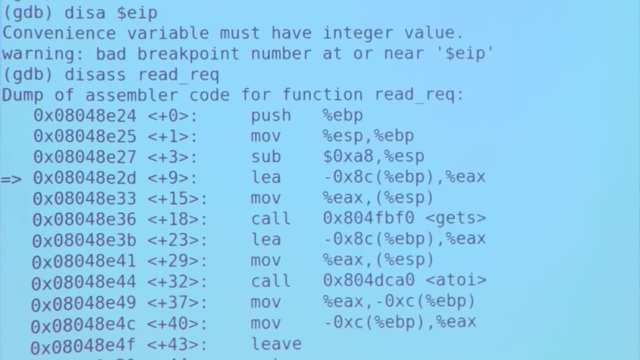 manipulating something with this EBP register. That's not super interesting, But the first thing it does after that is subtract a certain value from the stack pointer, And this is basically making space for all those variables like the buffer and the integer i we saw in the C source code. 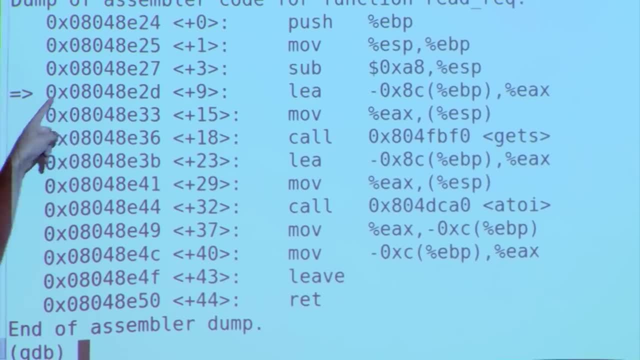 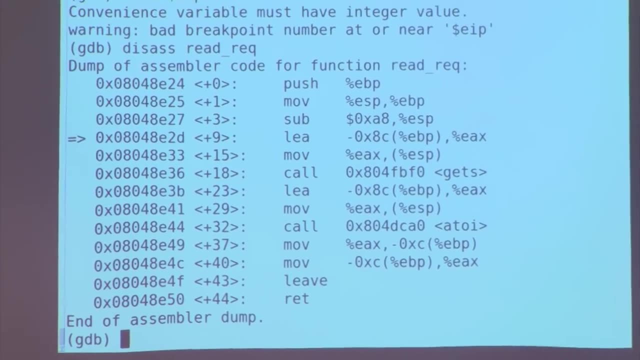 So we're actually now four instructions into the function here. So that stack pointer value that we saw before is actually already in the middle, so to say, of the stack, And currently there's a stack. There's stuff above it that is going. 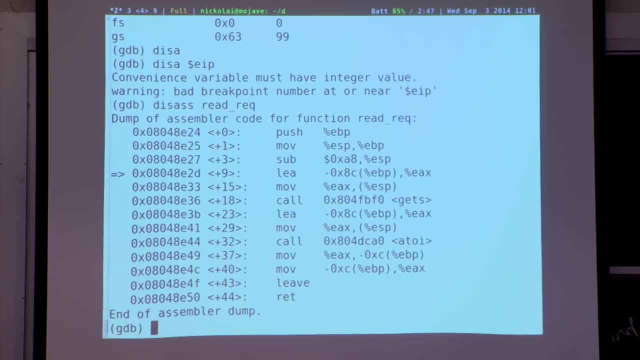 to be the buffer. that integer value and actually also the return address into the main function goes on the stack as well. So somewhere here we'll have the return address And we can actually try to figure out where are things on the stack. 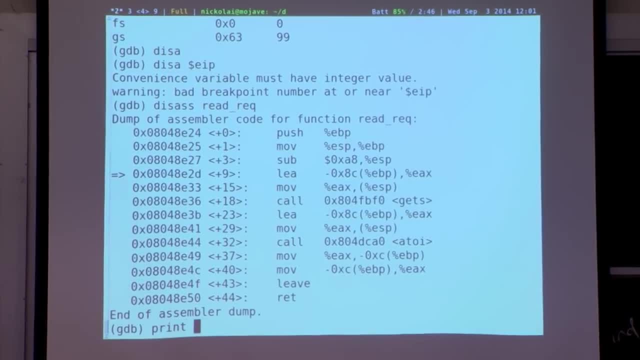 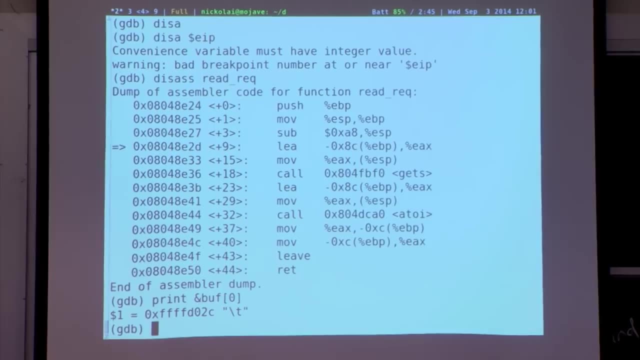 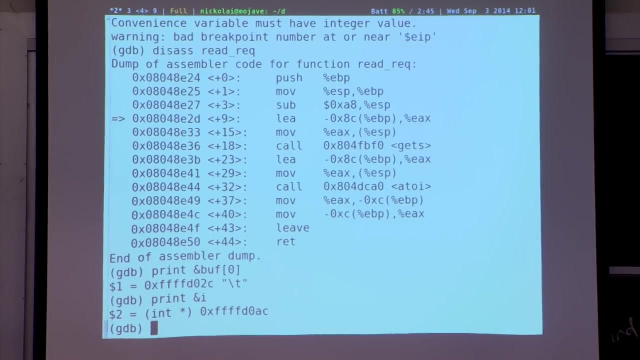 So we can print the address of that buffer variable. So the buffer variable is at address D02C. You can also print the value of that integer i. OK, So that guy is at D0AC. So the i is way up on the stack, but the buffer is a bit lower. 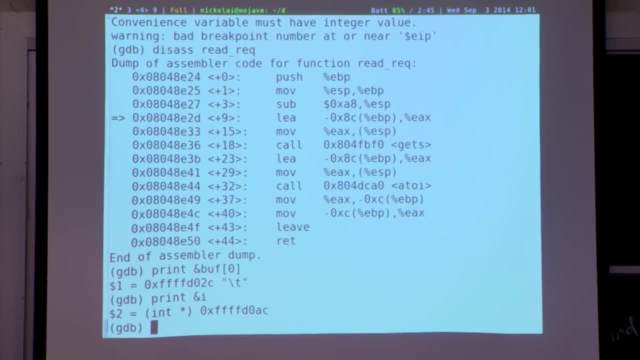 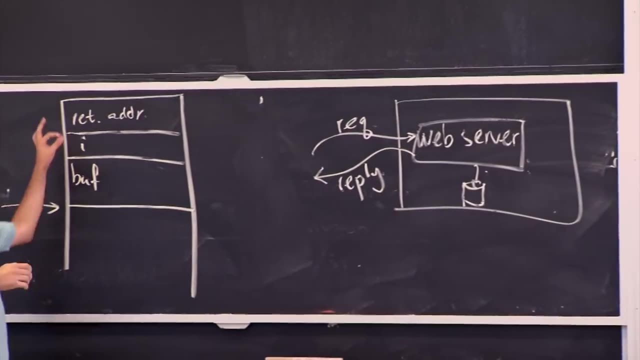 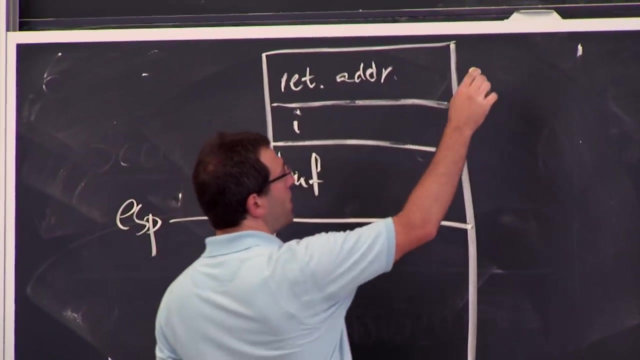 So what's going on is that we have our buffer here on the stack and then followed above by i and maybe some other stuff, and then finally the return address into the main function called redirect, And the buffer is going. the stack is growing down. 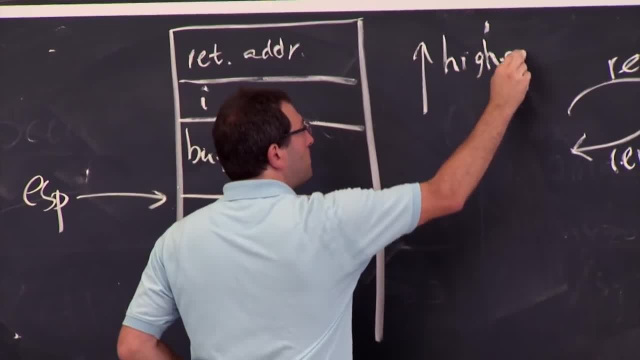 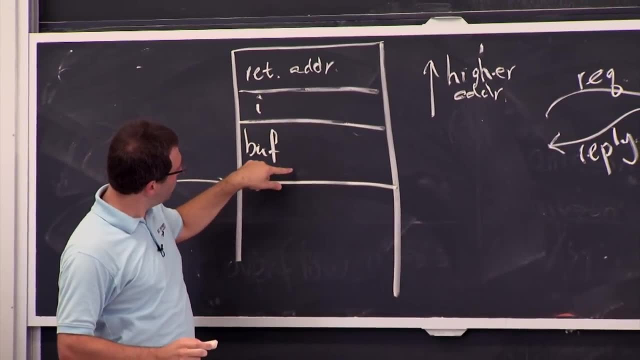 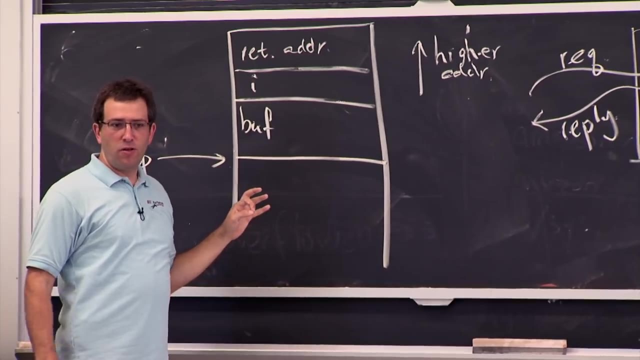 so these are higher addresses. So what this means is that the buffer we actually have to decide where is the 0-th element of the buffer and where is the 128-th element of this buffer. So where does the 0-th element of the buffer go? 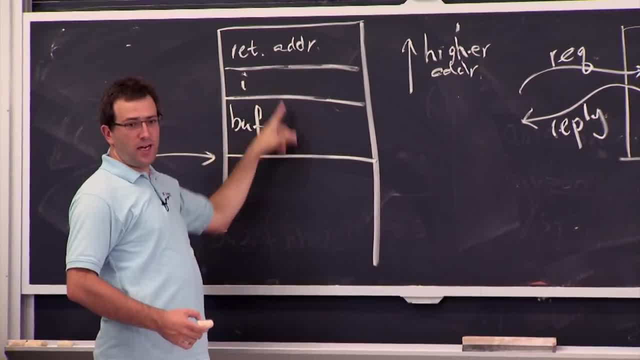 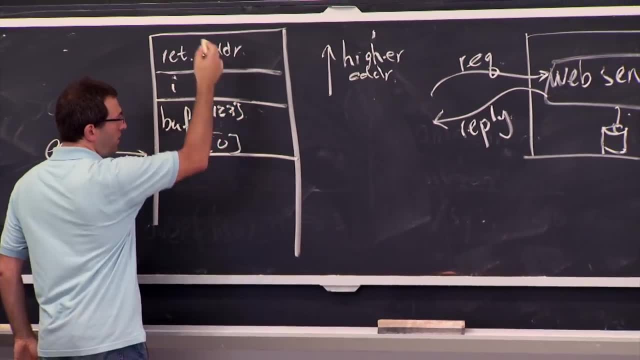 Yeah, It should be at the bottom right, Because higher elements just keep going up. Yeah, So buff of 0 is down here and just keeps going on, And buff of 127 is going to be up there. Then we'll have i and other stuff. 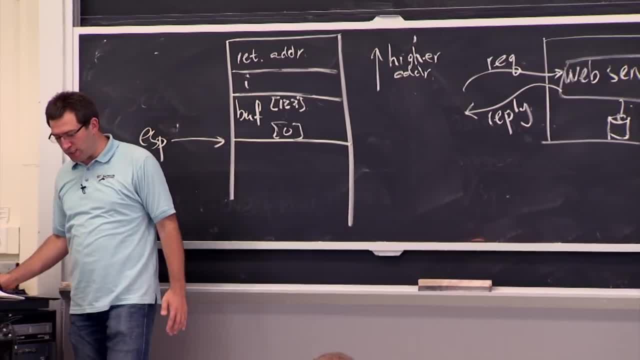 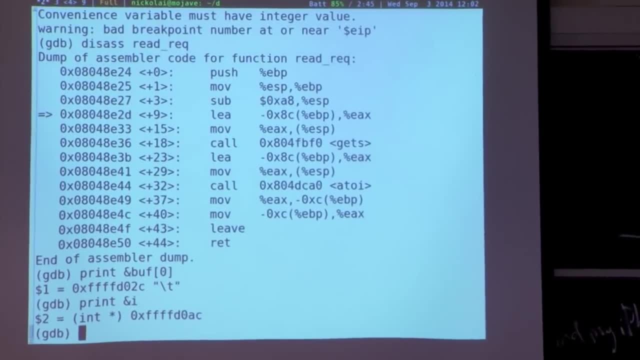 OK, Well, Let's see what happens now if we provide that input. that seemed to be crashing it before. So I guess one thing we can actually do before this is to see whether we can actually find this return address. Where it actually happens to live is at the EBP pointer. 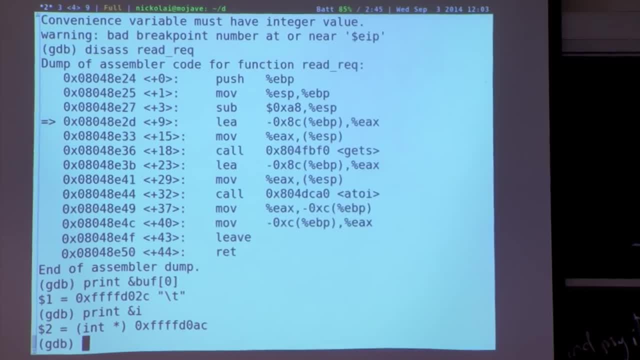 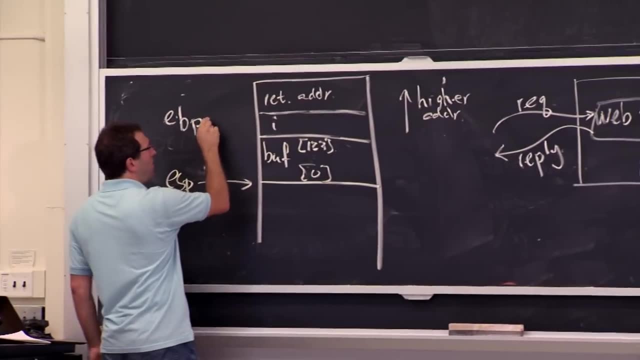 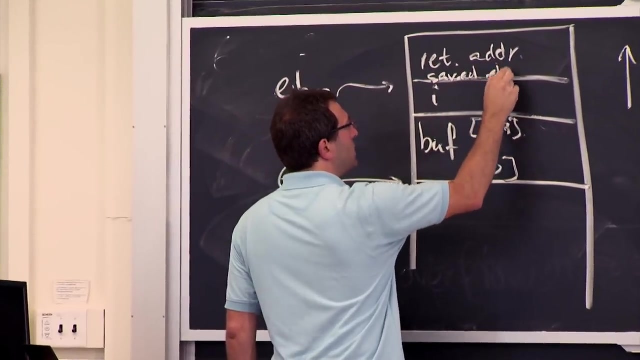 This is just a convenient thing in the x86 calling convention that the EBP pointer or register actually happens to point to something on the stack which is going to be called the saved EBP. It's a separate location sort of, after all the variables. 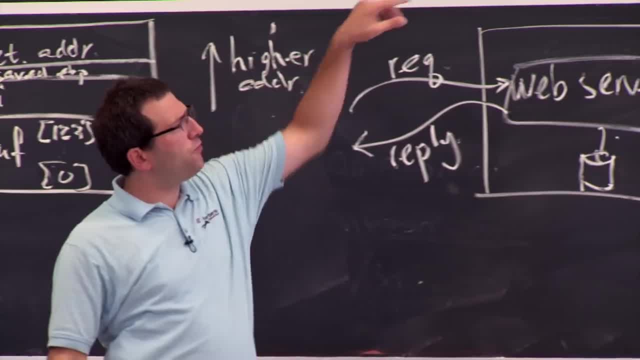 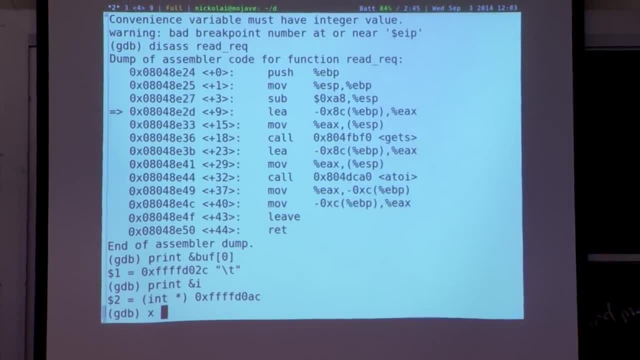 but before the return address. And this is the thing that's being saved by those first couple of instructions at the top And you can actually sort of examine it In GDB. you can say: examine x, some value. So the EBP pointer value. 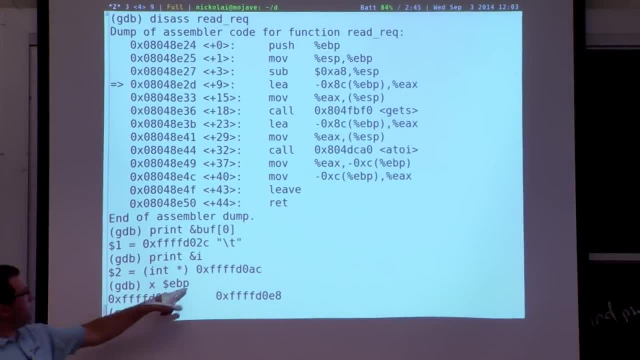 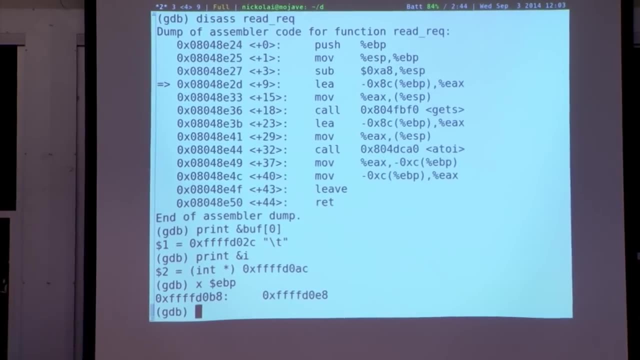 So that's the location of the stack d0, b8.. Indeed, it's actually above even the i variable, So it's great And it has some other value. that happens to be the EBP before this function was called, But then sort of one more sort of memory location up. 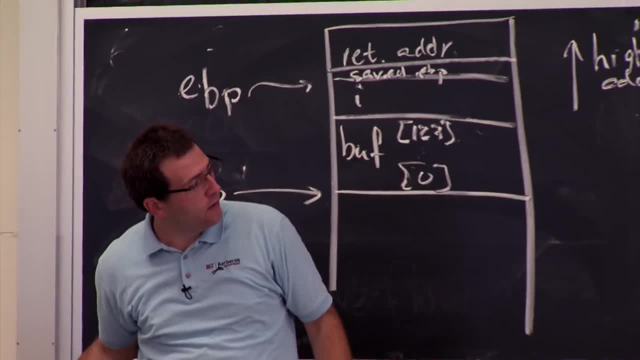 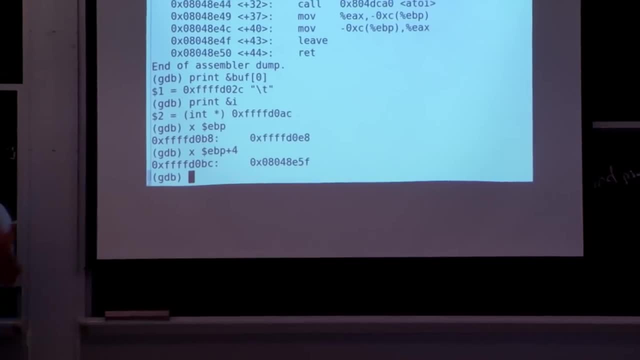 is going to be the return address. So if we print EBP plus 4, there's something else there, This 0x08048e5f, And let's actually see where that's pointing. This is something you're going to do a lot in the lab. 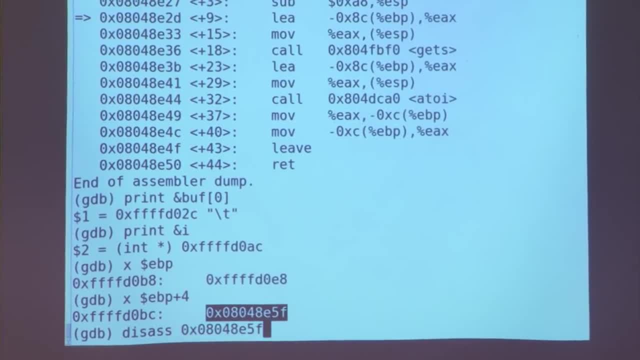 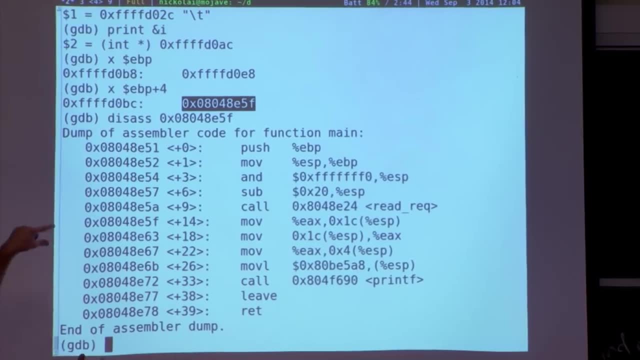 So you can take this address and you can try to disassemble it. So what is this guy? Where did we end up? So GDB actually helpfully figures out which function can contain that address. So 5f, this is the guy that our return address is pointing to. 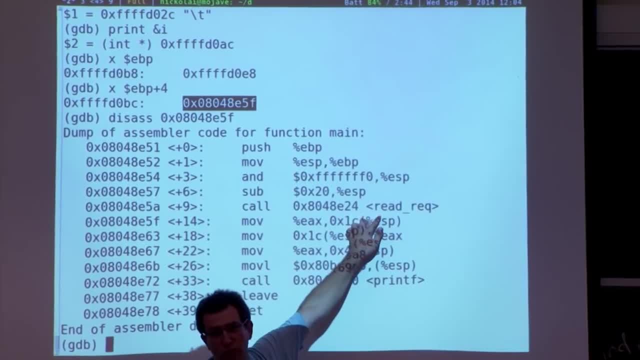 And, as you can see, this is the instruction right after the call to redirect. So when we return from redirect, this is exactly where we're going to jump and continue execution. This is hopefully fairly straightforward stuff from 004 or some standard OS class. 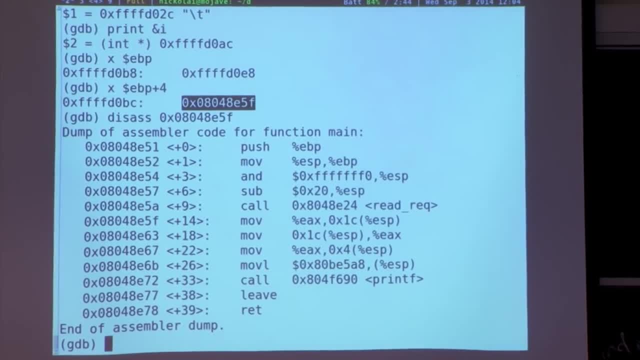 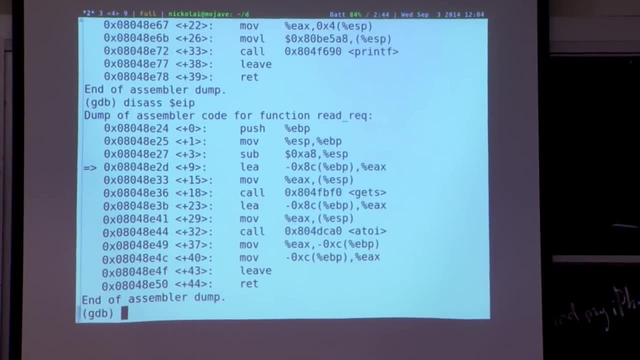 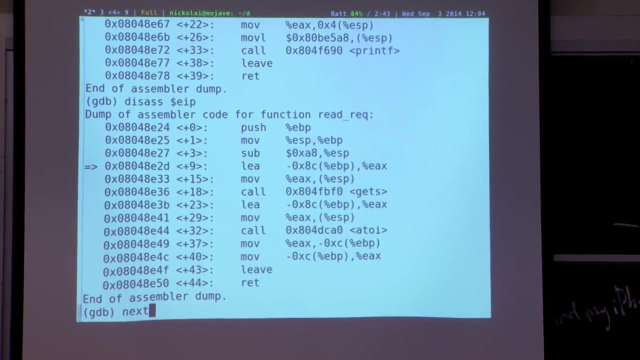 OK, so where are we now? Just to recap, we can try to disassemble our instruction pointer. So we're at the beginning. We're at the beginning of redirect right now And we can run for a bit and maybe run that get s function. 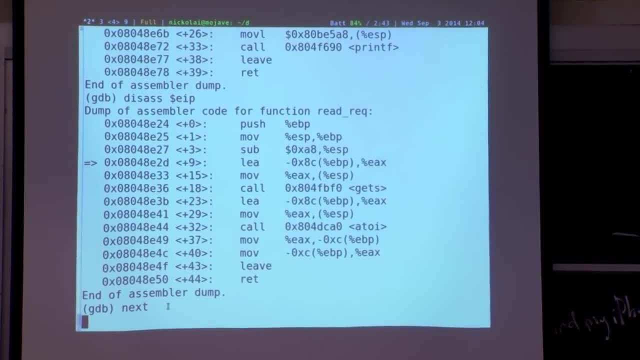 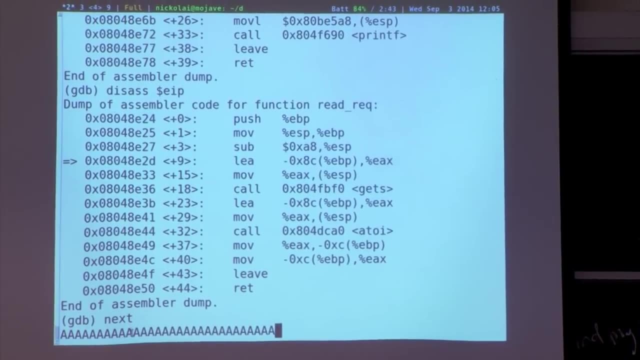 So OK, we run next. What this does is it runs get s and it's waiting for get s to return So we can provide our bad input to get s and try to get it to crash again and see what's going on really there. 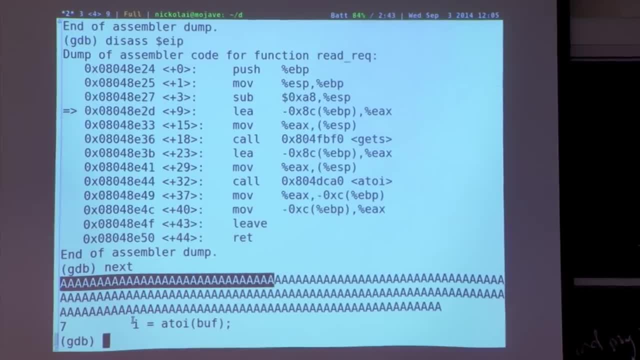 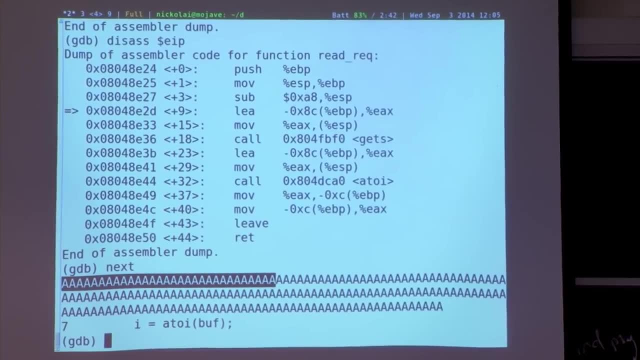 So we can paste a bunch of a's again. OK, so we got out of get s and things are actually still OK. The program is still running, But we can try to figure out what is in memory right now And why are things going to go wrong. 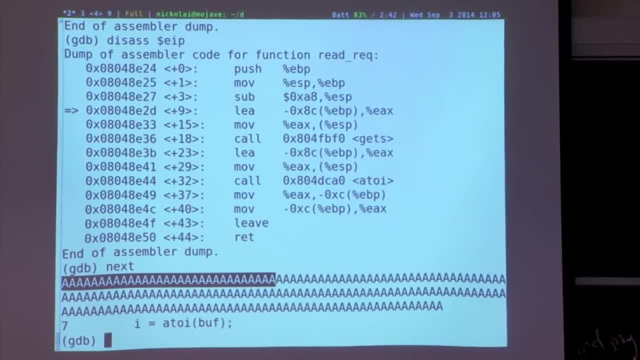 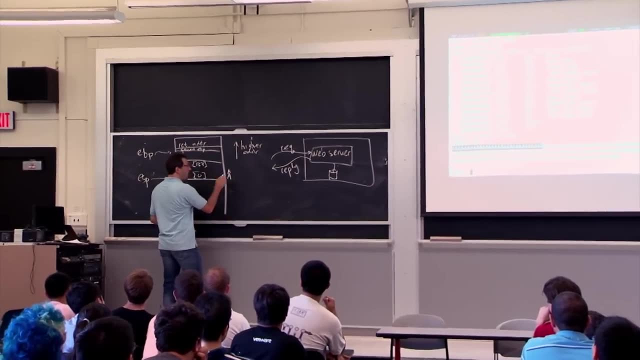 Actually, what do you guys think? What happened? So I printed out a bunch of a's. What did get s do to the memory? Write a: i, Yeah, yeah. so it just keeps writing a's here. All we actually passed to get s was a single pointer. 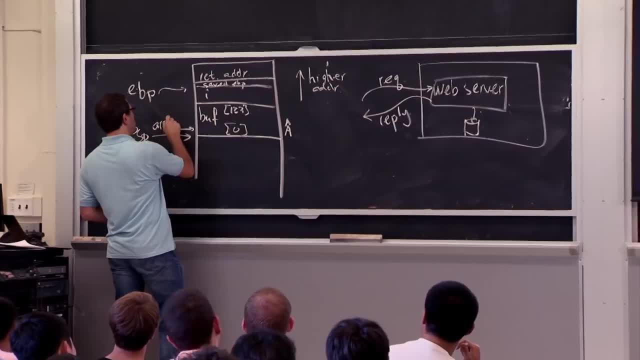 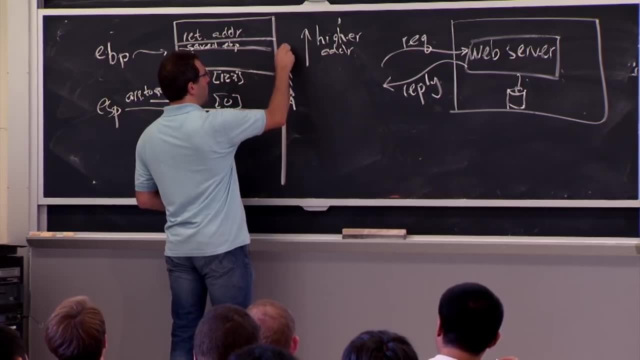 at the start of this address. So this is the argument to get. s is a pointer to this memory location on the stack. So it just kept writing a's And it doesn't actually know what the length is, so it just keeps going. 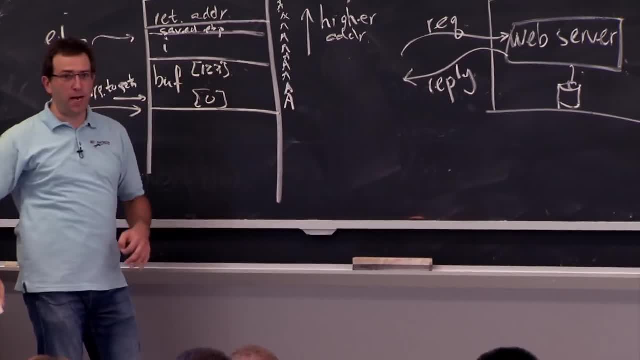 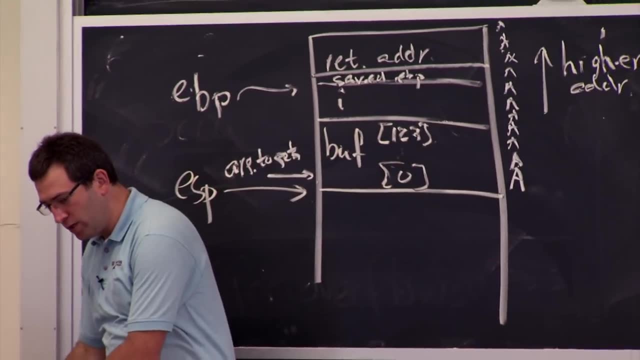 Right, It's going to overwrite a A's all the way up the stack, past the return address probably, and into whatever was up the stack above us. So we can check whether that's the case, So we can actually print the buffer. 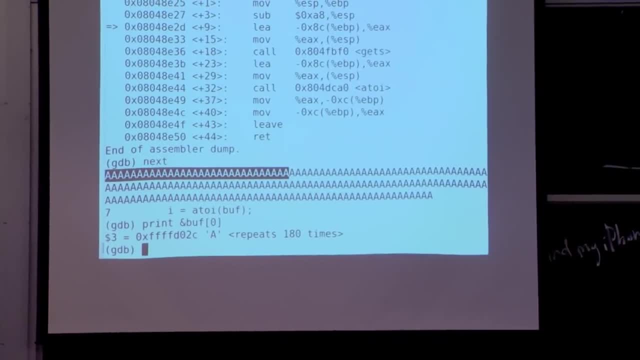 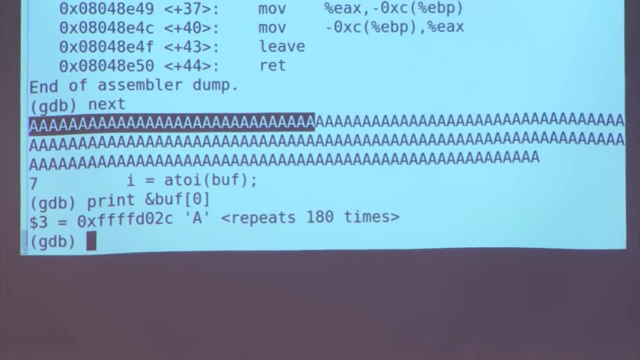 And in fact it tells us: yeah, we have 180 a's there, even though the buffer should be 128 elements large. So this is not so great And we can actually again examine what's going on in that EBP pointer. 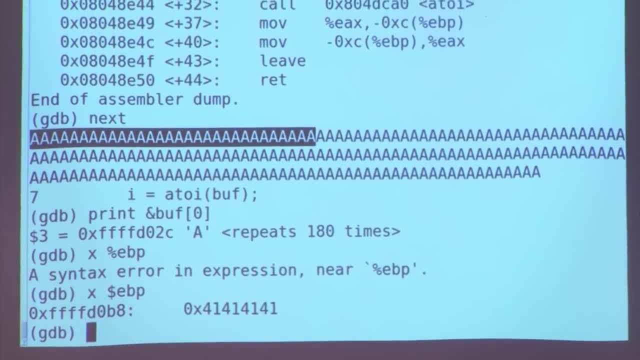 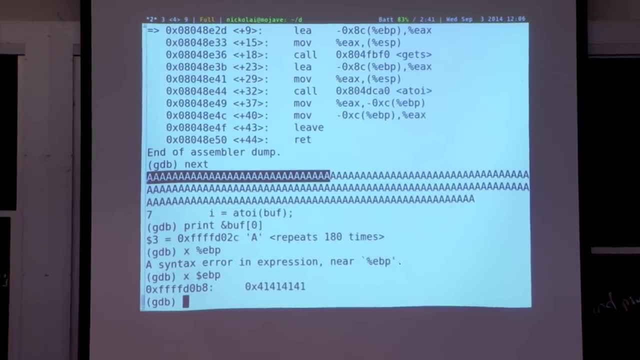 Dollar sign: EBP. So in fact, yeah, it's all 0x41,, which is the ASCII encoding of the letter a, And in fact, the return address is probably going to be the same way, right? Even if we print the return address, it's also all a's. 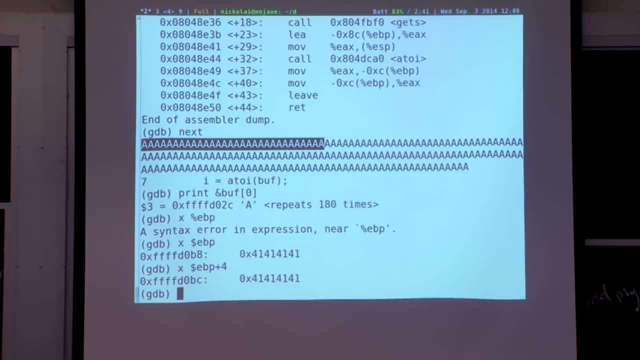 That's not so great. In fact. what's going to happen if we return now is the program will jump to that address 41414141, and there's nothing there, and it'll crash. That's the segmentation fault you're getting. 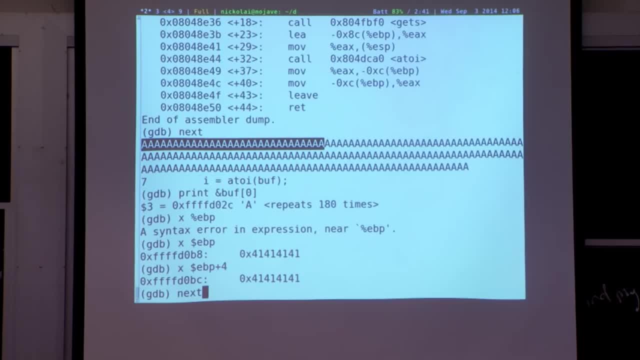 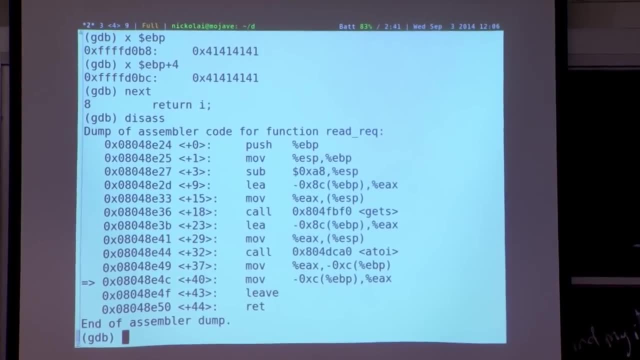 So well, let's just step up to it and see what happens, Right? So let's run next. So we keep stepping through the program And we can see where we are. OK, we're getting close to the end of the function. 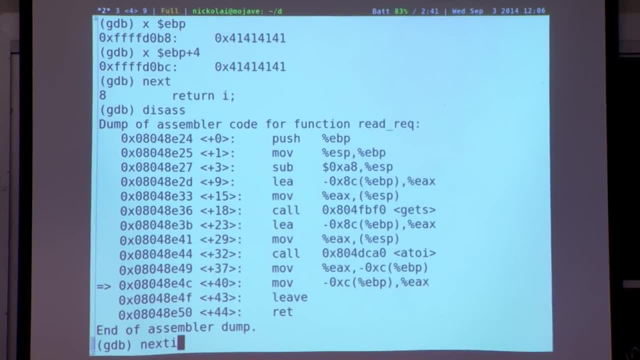 So we can step over two more instructions: Next i, next i, And now we can disassemble again. OK, we're now just at the return instruction from this function And we can actually figure out. So, as you can see at the end of the function, 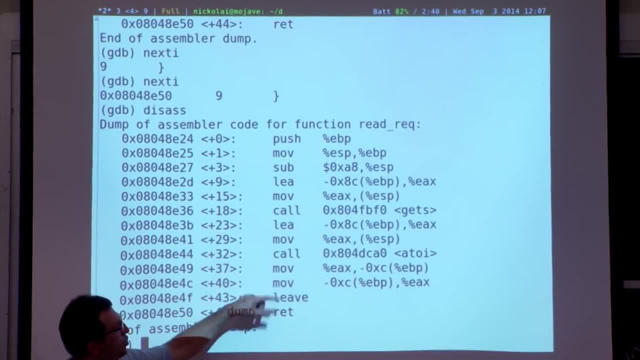 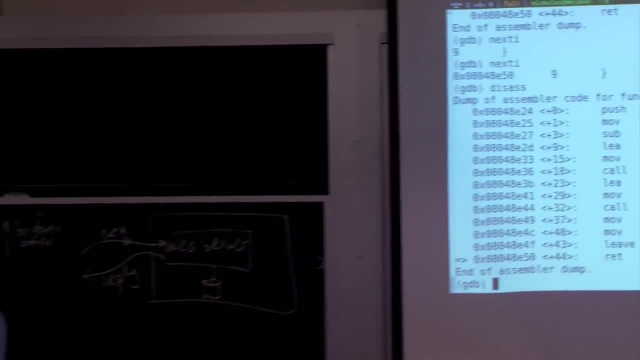 it runs this leave x86 instruction, which basically restores the stack Back to where it was. So it sort of pushes the stack pointer all the way back to the return address using the saved EBP. That's what it's basically for, And now the stack is pointing at the return address. 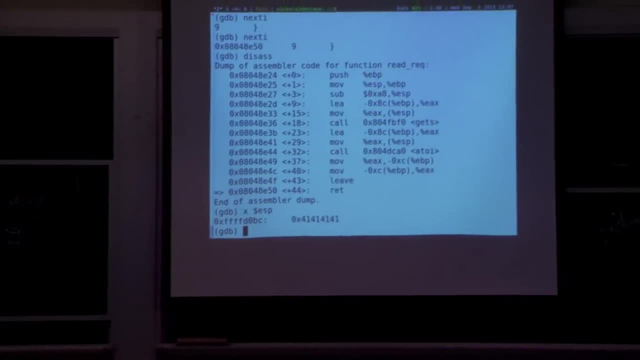 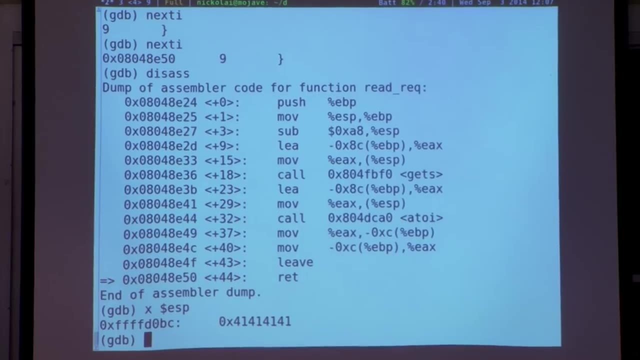 that we're going to use And in fact it's all a's- And if we run one more instruction, the CPU is going to jump to that exact memory address and start executing code there and crash because it's not a valid address. that's in the page table. 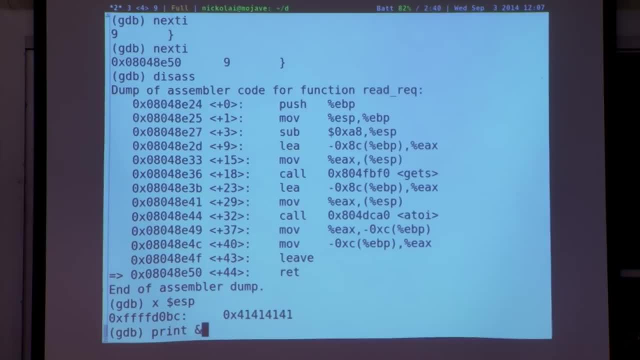 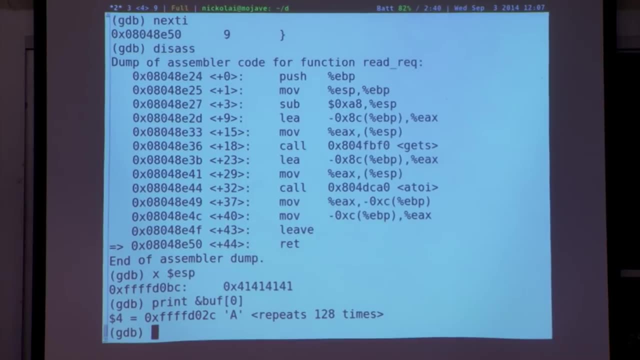 So let's actually see what's. just to double check what's going on, Let's print our buffer again, Our buffer. well, it's actually kind of interesting, right? So now buffer. for some reason it only says a, repeats 128 times. 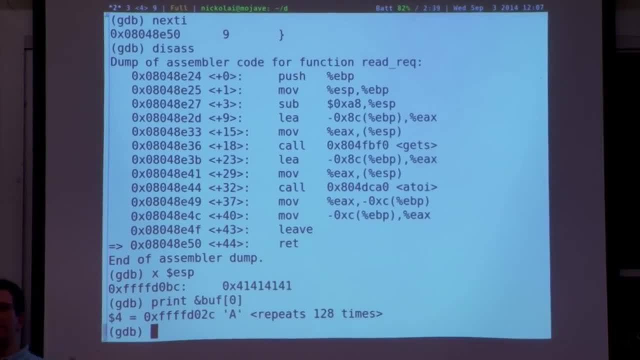 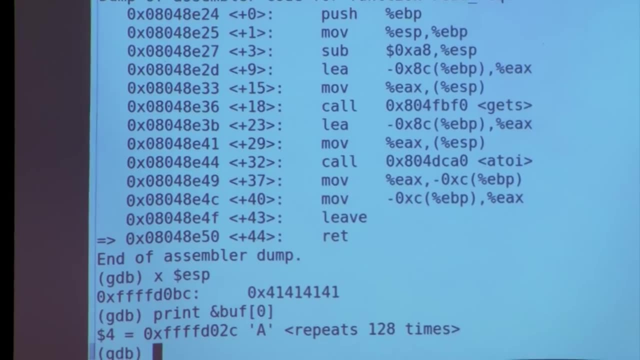 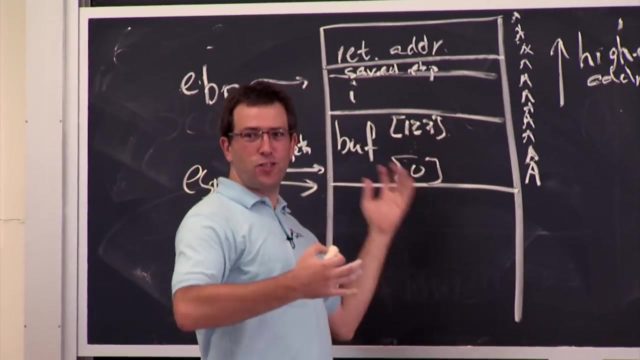 Whereas, if you remember, before it said a repeated 180 times in our buffer. So what happened? Yeah, Yeah, yeah, exactly. So there's actually something going on after the buffer overflow happens that changes what's going on. So, actually, if you remember, we do this a to i conversion. 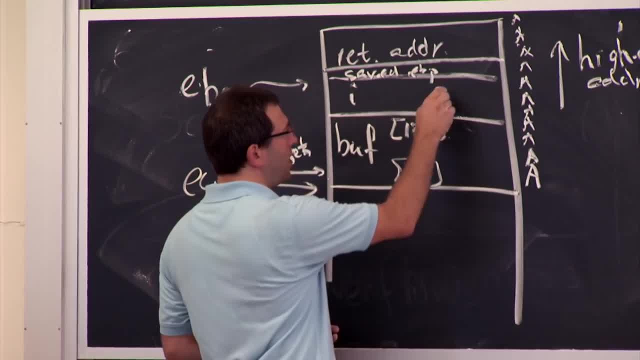 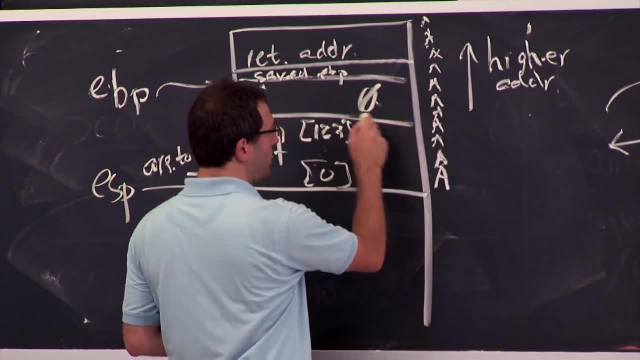 of the string to an integer. And if we provide all a's, it actually writes zero. So a zero, if you remember, terminates strings in C. So GDB now thinks: yep, we have a perfectly well terminated 128 byte string of all a's. 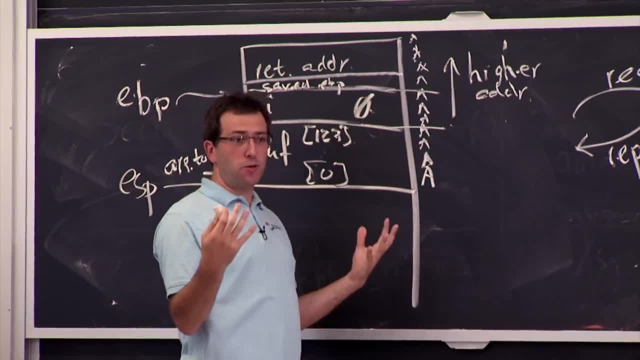 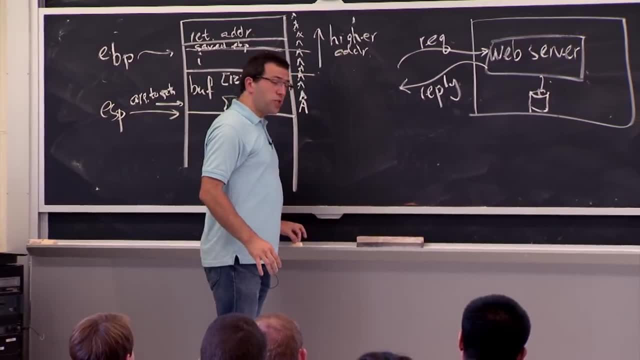 But it doesn't really matter, because we still have those a's up top that already corrupted our stack. OK, this is actually kind of an important lesson that it's actually a little bit tricky sometimes to exploit these buffer overflows, because even though you've already changed lots of stuff in the stack, you still have to get to the point where you use the value that you've somehow placed on the stack. So there's other code that's going to run after you've managed to overflow some buffer and corrupt memory. 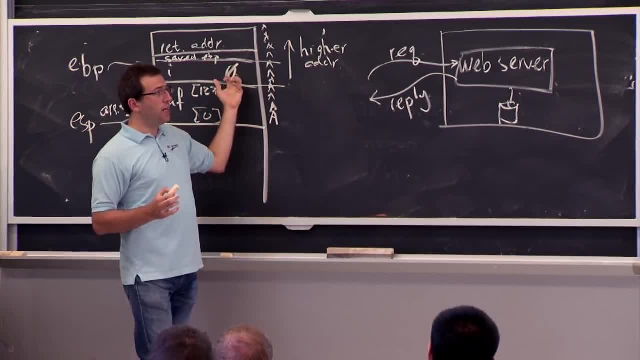 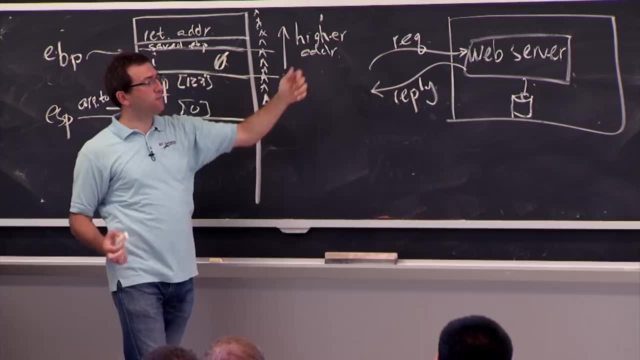 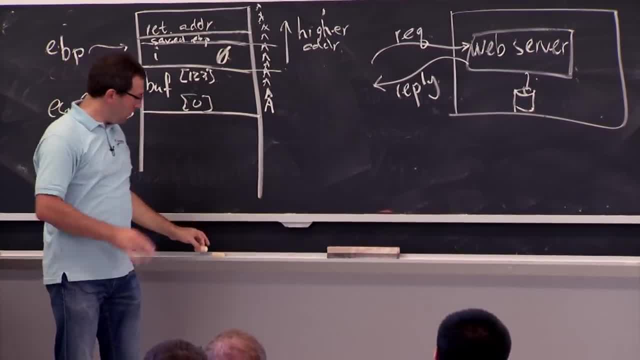 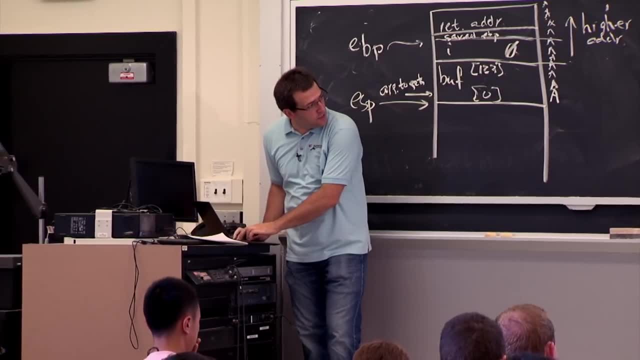 address. So you have to massage your input in some cases- Maybe not so much in this case, But in other situations you'll have to be careful in constructing this input. OK, so just to see what happens, we can jump One more time. 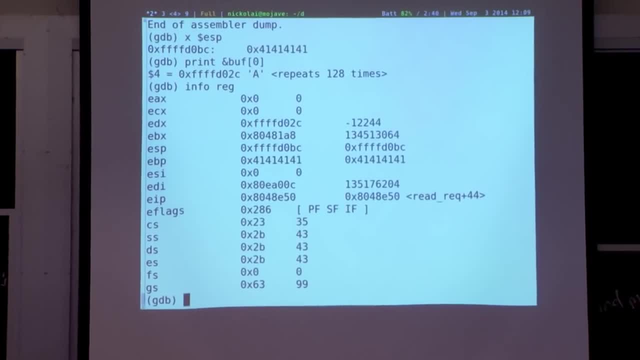 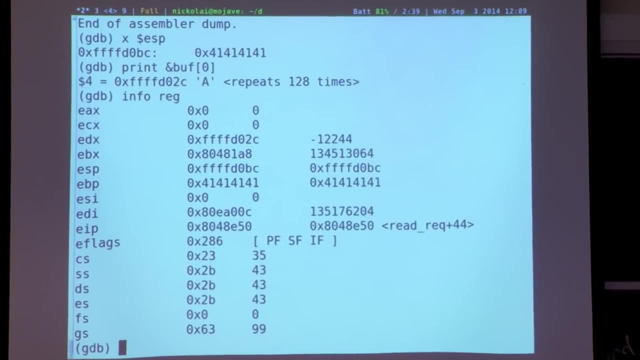 Well, let's look at our register. So right now, our EIP, the sort of instruction pointer, is pointing at the last thing in redirect And if we step one more time, hopefully we'll jump to finally that unfortunate for one, for one address. 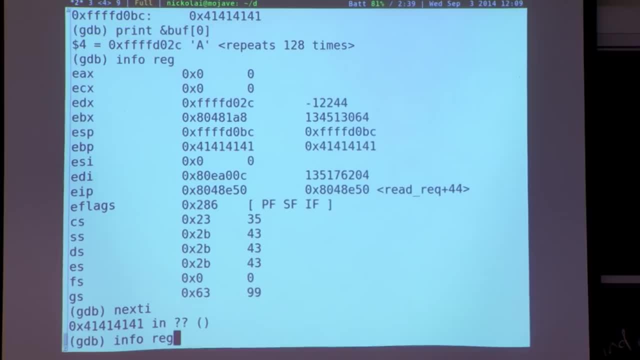 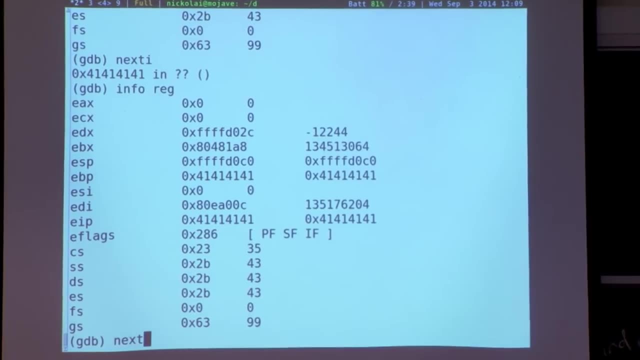 Over here in fact. yep, the program now seems to be executing there. If we ask GDB to print the current set of registers, yep, the current instruction pointer is this strange value. And if we execute one more instruction, 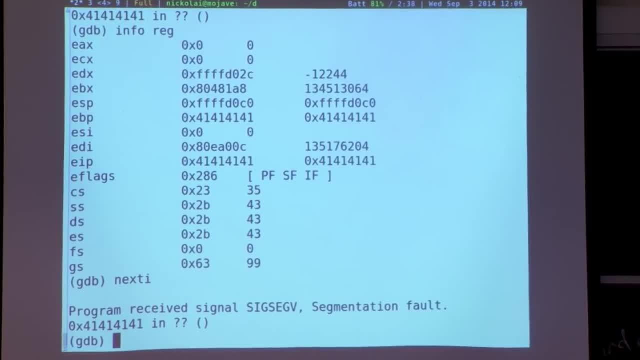 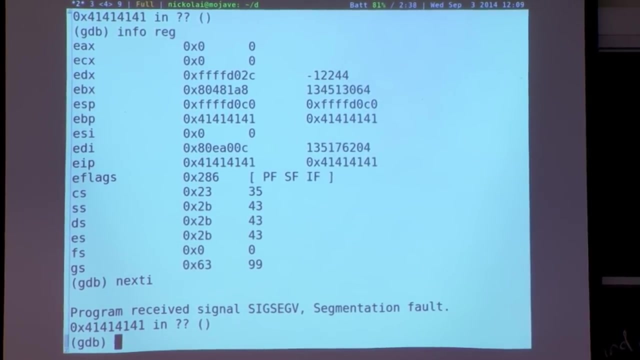 it's going to crash because that's finally trying to execute an instruction pointer that doesn't correspond to a valid page in the operating system's page table for this process. Make sense, Any questions? All right? well, I've got a question for you guys. 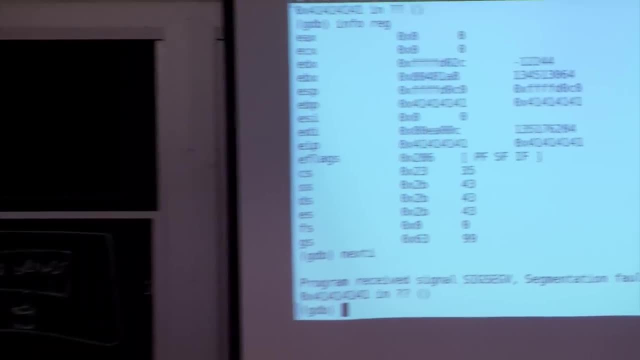 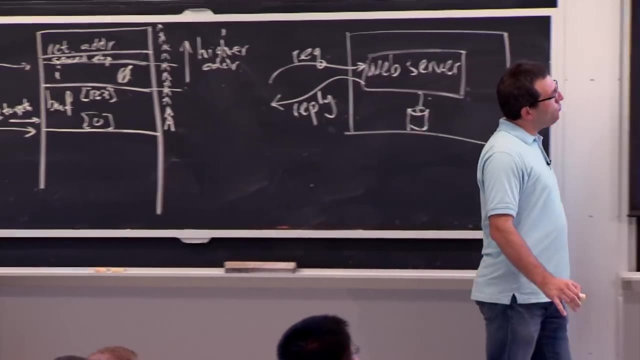 actually. So what happens? you know, this seems to be exploitable, Or well, OK, maybe let's first figure out why this is particularly bad, Right? So why? Why is this a problem? So not only does our program crash, 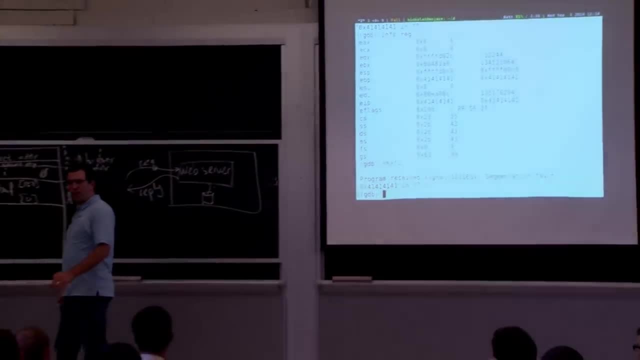 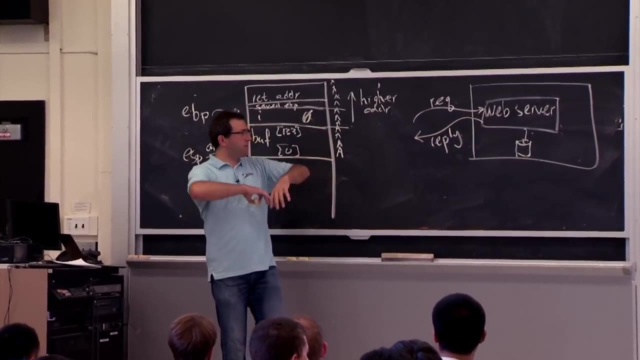 but presumably we're going to take it over. So I guess first simple question is OK. so what's the problem? What can you do? Yeah, Yeah, so I was actually pretty silly and just put in lots of As, But if you're careful about knowing, 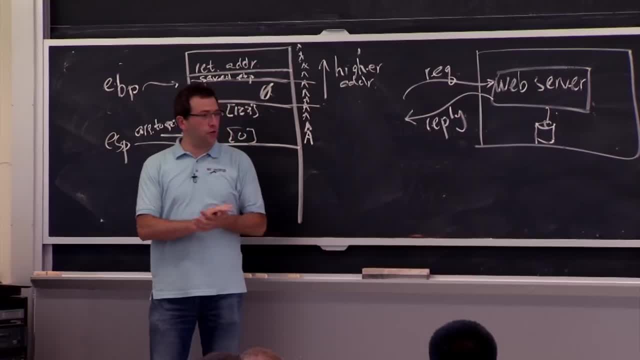 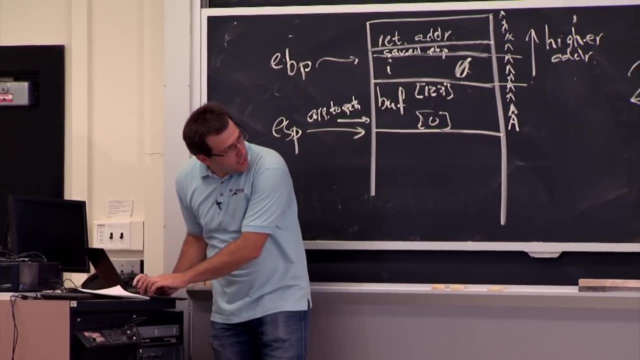 where to put what values you might be able to put in a different value and get it to jump somewhere else. So let's see if we can actually do this right. We can retrace this whole thing. OK, rerun the program again. 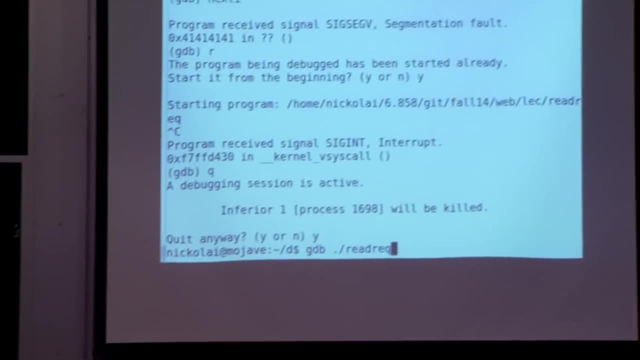 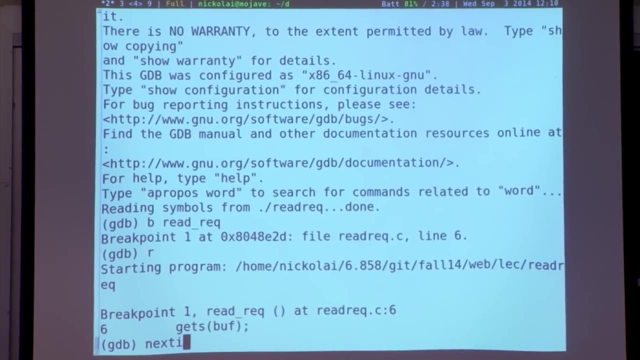 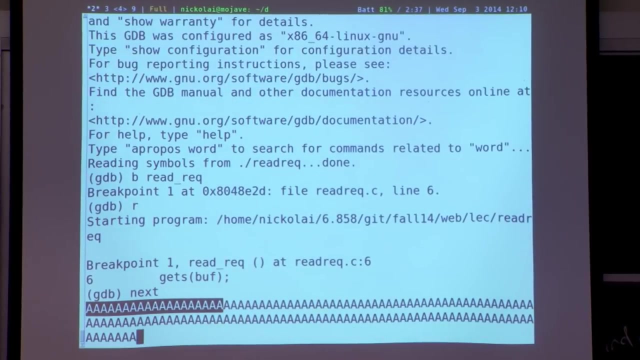 And I guess I have to reset the break point So I can break and redirect again and run, And this time I'll again supply lots of As and overflow things. But I'm not going to try to carefully construct, figure out which point in these As. 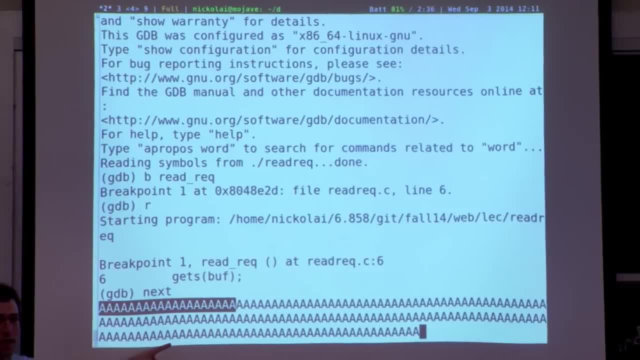 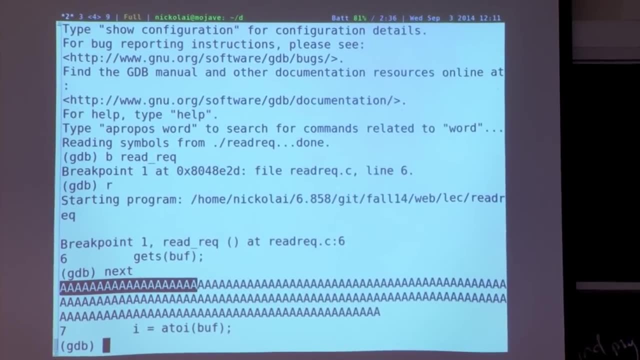 corresponds to the location of the stack. That's something you guys are going to have to do for lab 1.. But suppose that I overflow the stack here and then I'm going to manually try to change things on the stack to get it to jump to some point. I 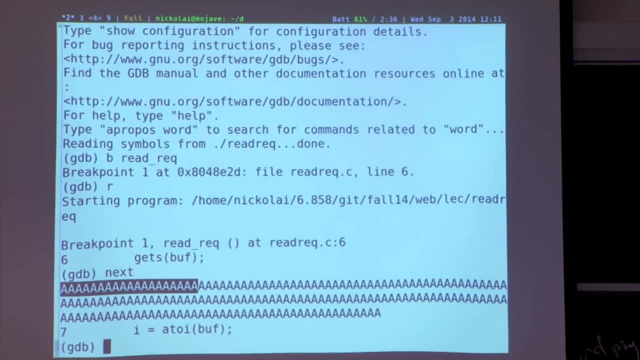 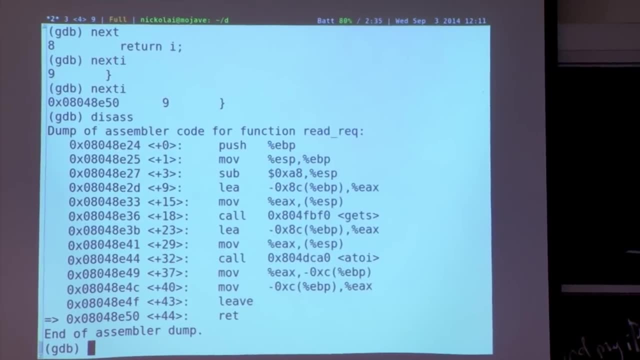 want to jump to And in this program. OK, so let's again. next i Where are we? We're again at the very end of redirect, And let's actually look at the stack, right? So if we examine ESP here, we see our corrupted pointer. 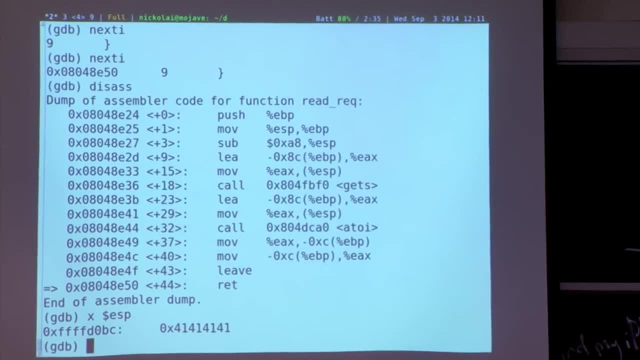 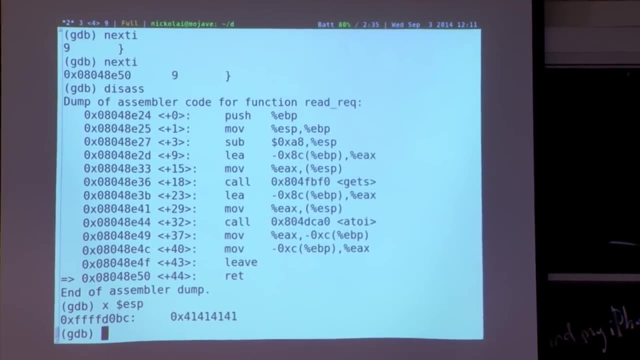 OK, where could we jump to? What interesting things could we do? Unfortunately, this program is pretty limited. There's almost nothing in the program's code where you could jump and do anything interesting, But maybe we can do a little bit of something interesting. 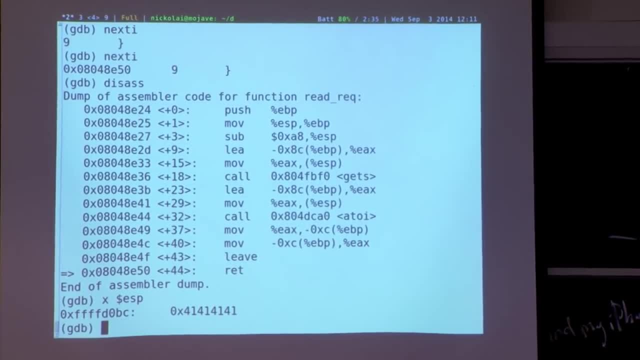 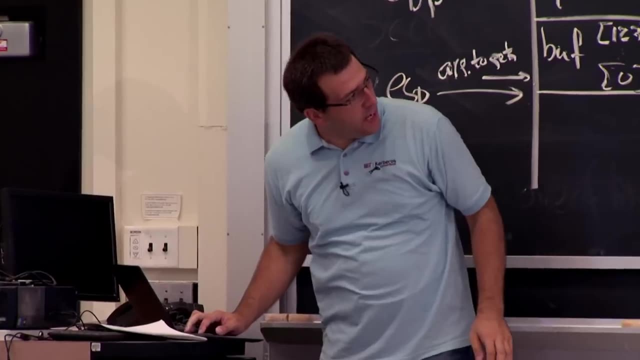 Maybe we'll find that Let's printf in main and jump directly there and get it to print. the x equals something. So we can do this. We can actually disassemble the main function And main does a bunch of stuff: initializes, calls, redirect. 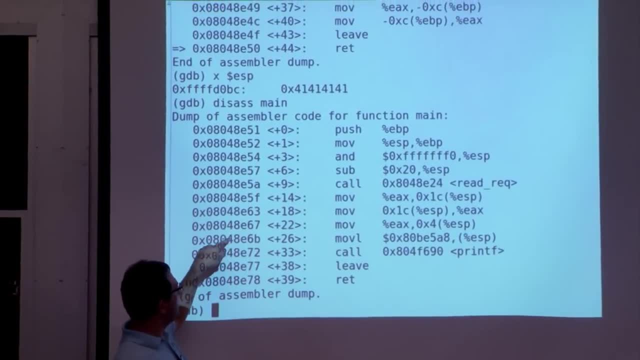 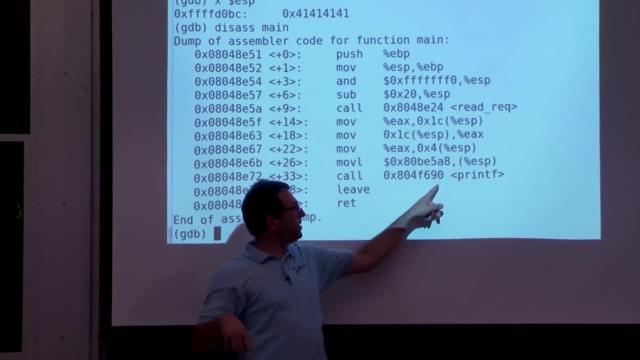 does some more stuff and then calls printf. So how about we jump to this point, which is it sets up the argument of printf, which is x equals percent d, and then actually calls printf, So we can actually take this value and try to stick it in the stack. 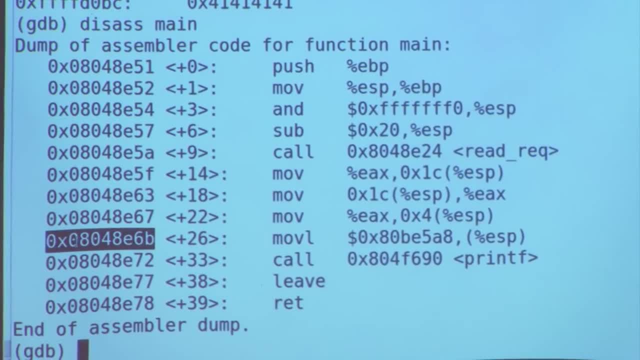 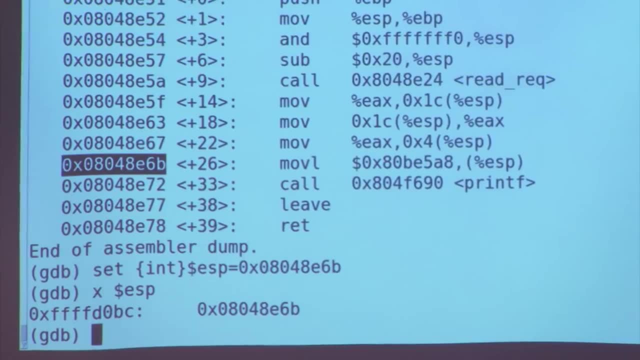 And we should be able to do this with the debugger pretty easily at least. So you can just do this. set int ESP equals this value, So we can examine ESP again And indeed it actually has this value. So if we continue now, well, it printed out. 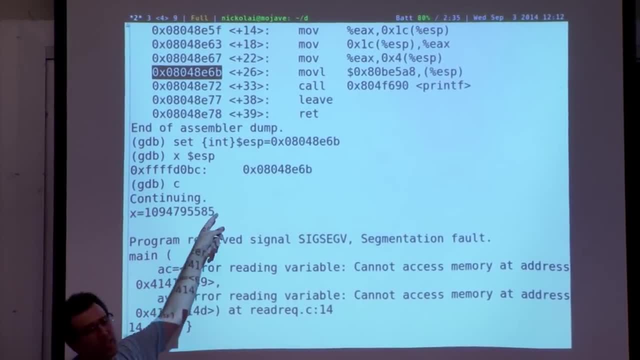 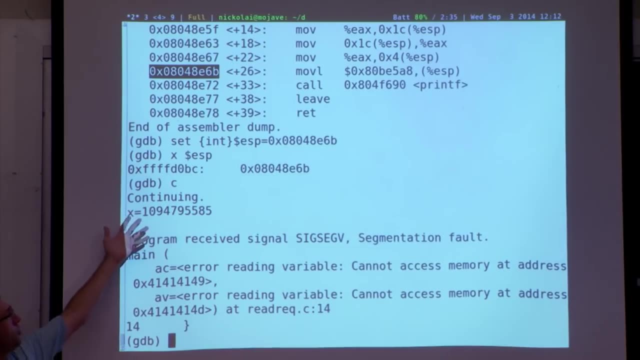 x equals some garbage, which I guess happens to be just whatever is on the stack that was passed to printf. We didn't correctly set up all the arguments because we jumped in the middle of this calling sequence. But yeah, we printed this value. 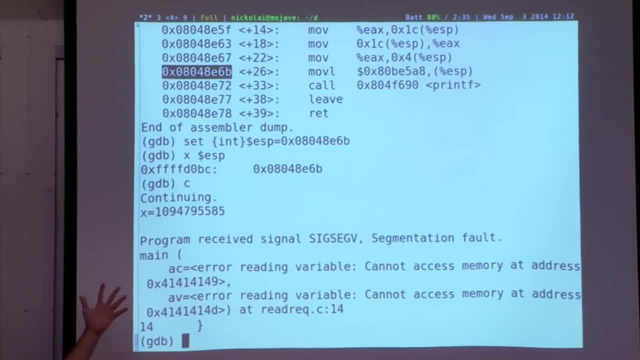 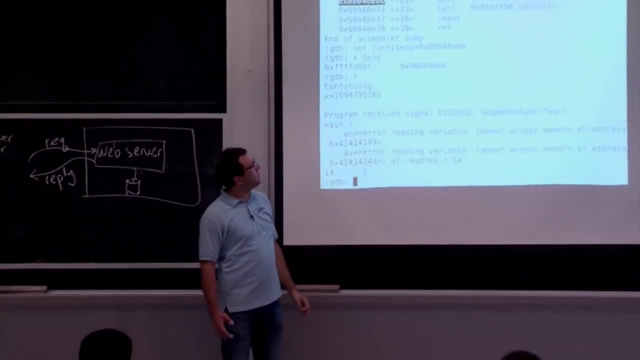 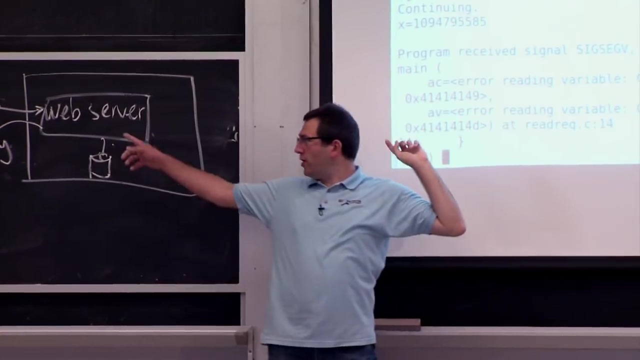 And then it crashed. Why did it crash? Why do you think What actually happens? So we jump to printf And then something went wrong. Yeah, When did the return address go? Well, we changed the return address so that when we return from redirect- 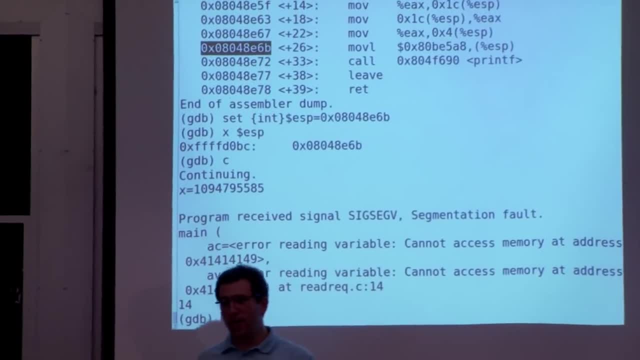 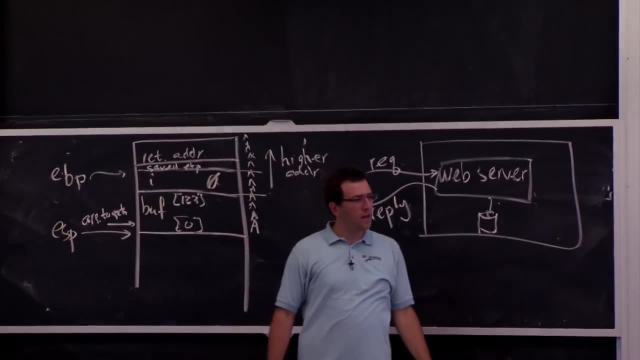 we now jump to this new address, which is that point up there right after printf. So where's this crash coming from? Yeah, Is it restricted? because your i is supposed to be some sort of. Yeah, well, the i is like. well, it's a 32-bit register. 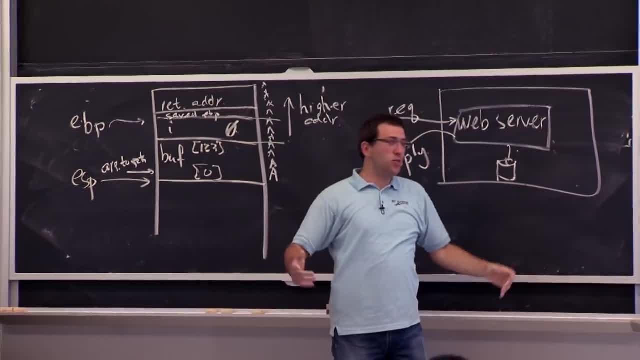 So whatever's in the register it'll print. In fact, that's the thing that's in the register, So that's OK. Yeah, It's simply doing main returns, Yeah, actually. yeah, What's going on is you have to sort of see here. 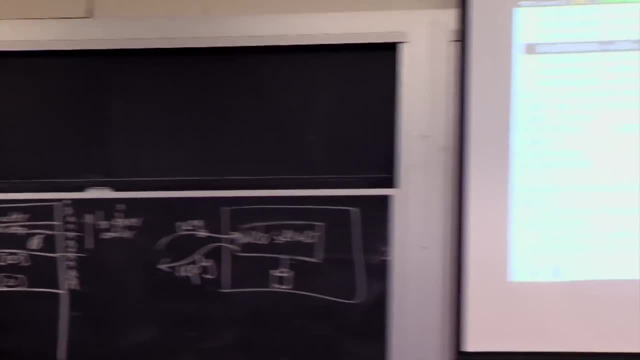 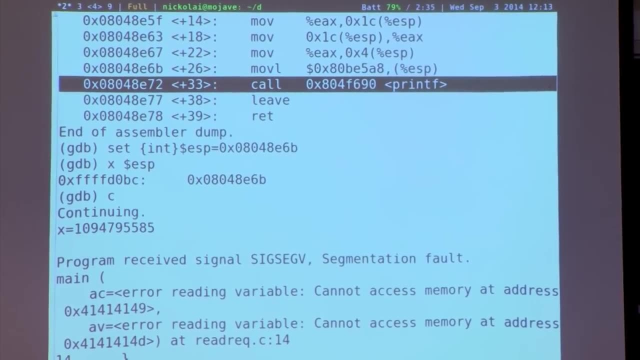 OK, so this is the point where we jumped. It set up some arguments. It actually calls printf. Printf seems to work. Printf is going to return. Actually, that's fine, because this call instruction put a return address on the stack for printf to use. 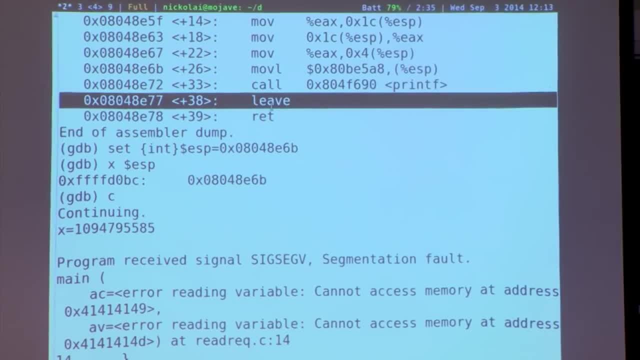 That's fine. Then main is going to continue running. It's going to run the sleeve instruction, which doesn't do anything interesting, And then it does another return, But the thing up in the stack doesn't actually have a valid return address. 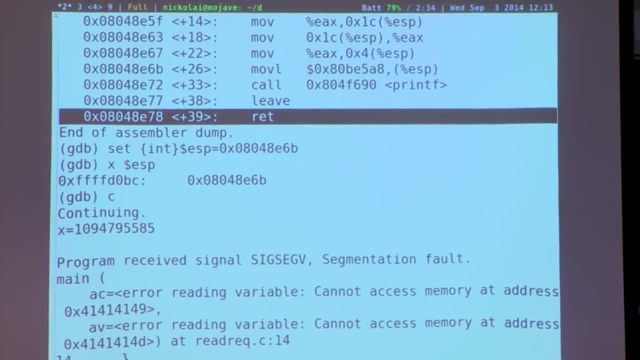 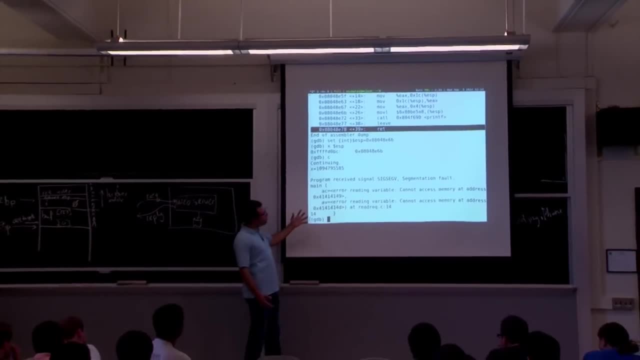 So presumably we returned to some other who knows what memory location that's up on the stack and jumped somewhere else. So unfortunately here our pseudo attack didn't really work at ransom code, But then it crashed. That's probably not something you want to do. 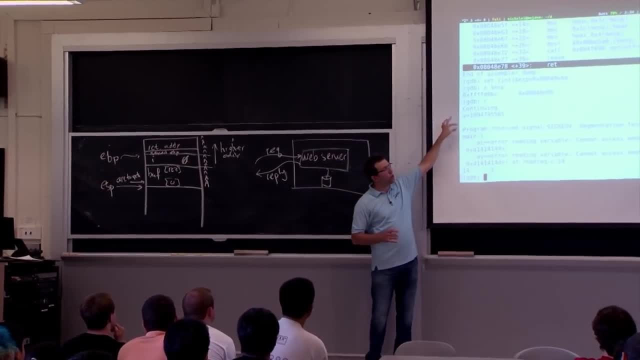 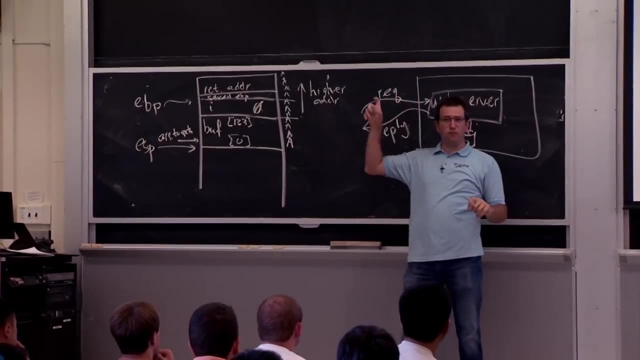 So if you really wanted to be careful, you would carefully plant not just this return address up on the stack, but maybe you'd figure out where is this second read going to get its return address from. Yeah, And try to carefully place something else. 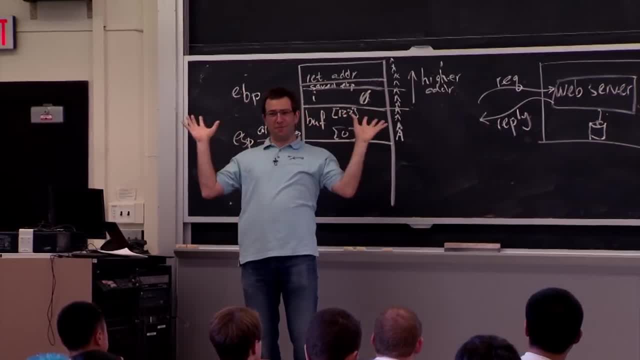 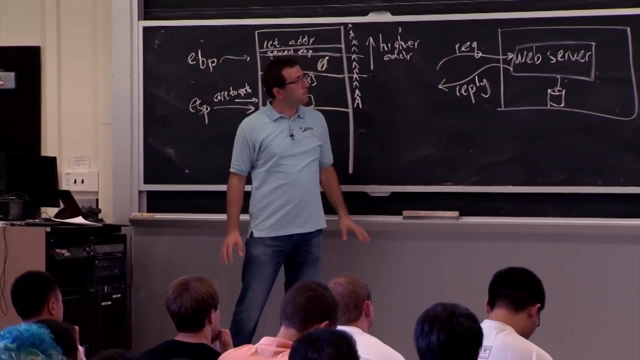 on the stack there. that will ensure that your program cleanly exits after it gets exploited so that no one notices. This is all stuff you'll sort of try to do in lab one in a little bit more detail, But I guess one thing we can try to think about now. 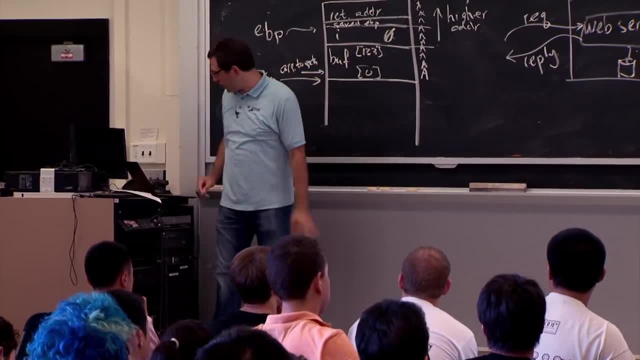 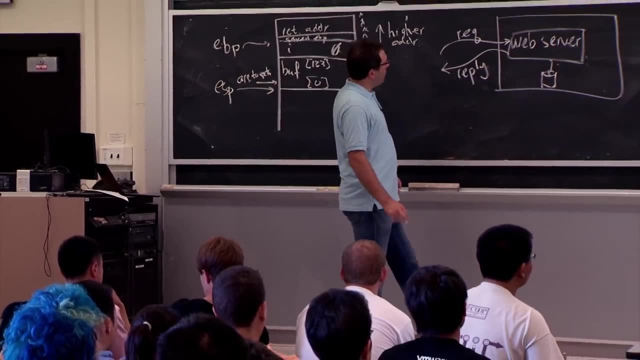 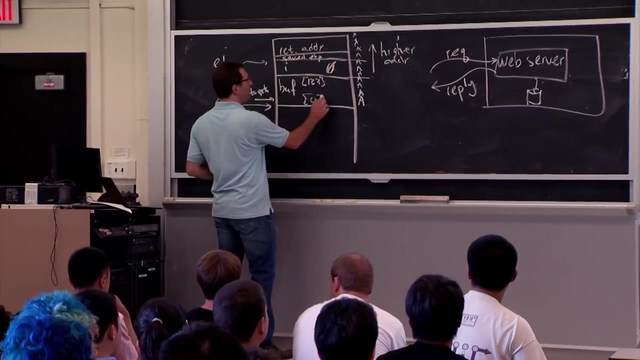 is we sort of understand why it's bad to have these buffer overflows. One problem, or one sort of way to think of this, is that the problem is just because the return address is up there, So the buffer keeps growing and eventually runs over the return address. 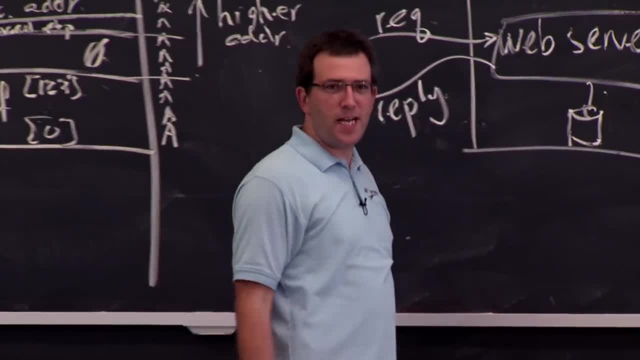 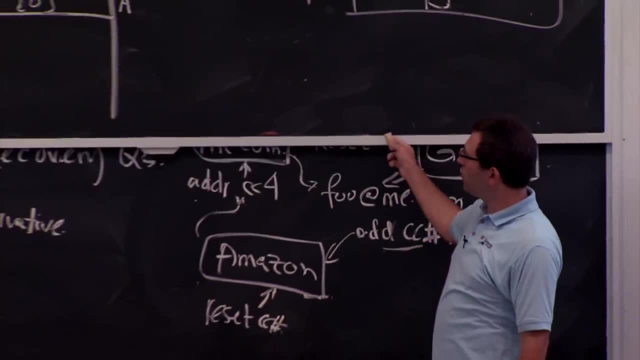 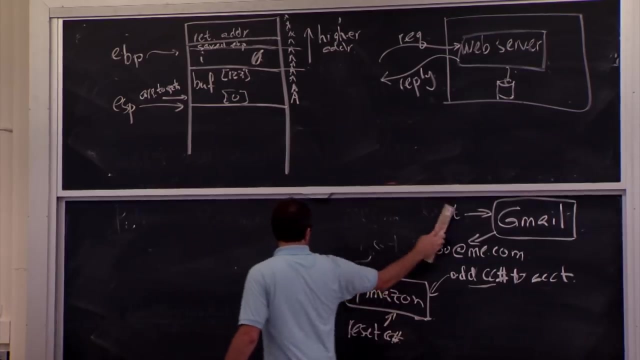 What if we flip the stack around? Some machines actually have stacks that grow up, So an alternative design we could sort of imagine is one where the stack starts at the bottom and keeps going up instead of growing down. So then, if you overflow this buffer, 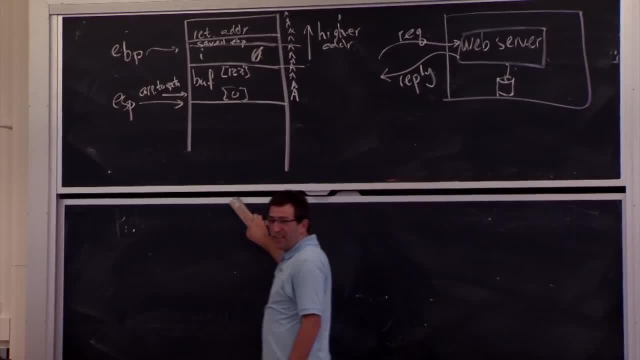 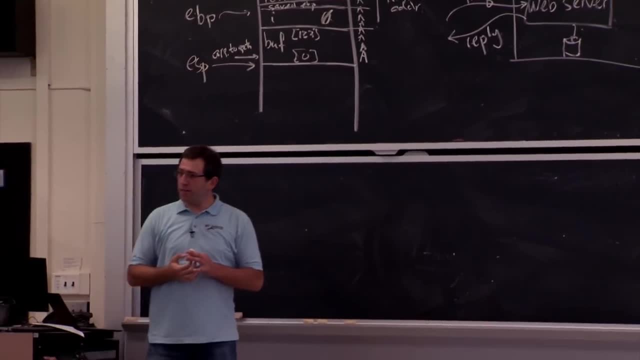 you'll just keep going up on the stack and maybe there's nothing bad that'll happen. Yeah, But that only applies to the most variable. So you're right, It might be that, if you have. well, so let me draw this new stack diagram and we'll. 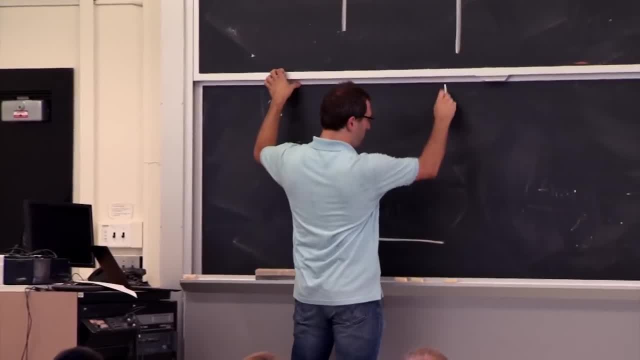 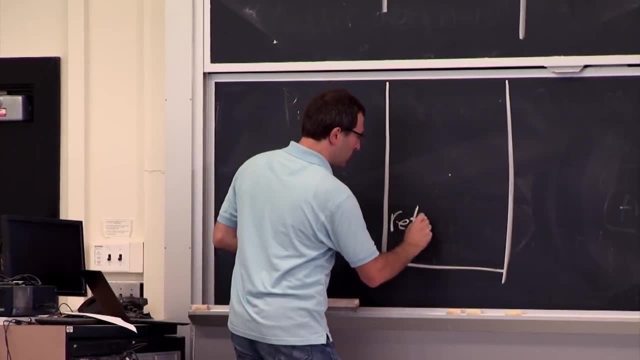 sort of try to figure out what it applies to and not. But OK, so we'll basically just invert the picture. So when you call redirect on this alternative architecture, what's going to happen is the return address is going to go here on the stack. 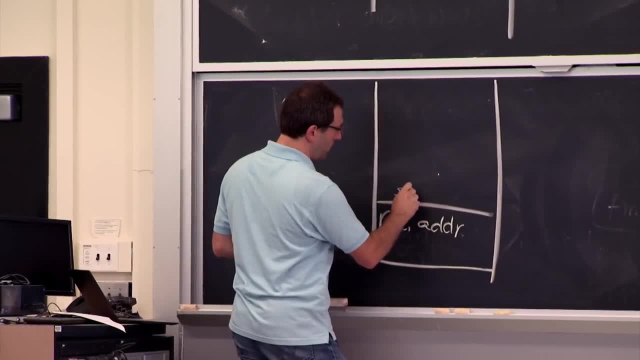 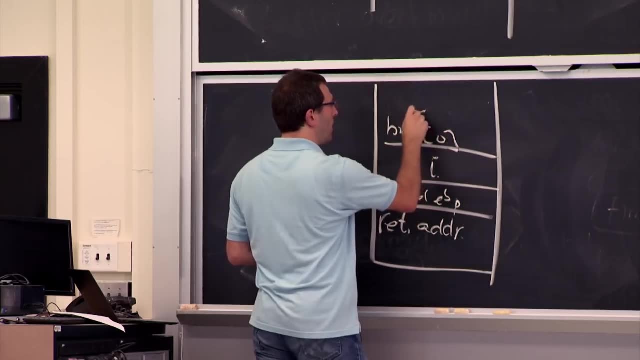 Then we'll have our i variable, or maybe the save dbp, Then we'll have our i variable, and then we'll have buff. So we'll have buff of 0, of 127, and so on. So then when we do the overflow, it overflows up there. 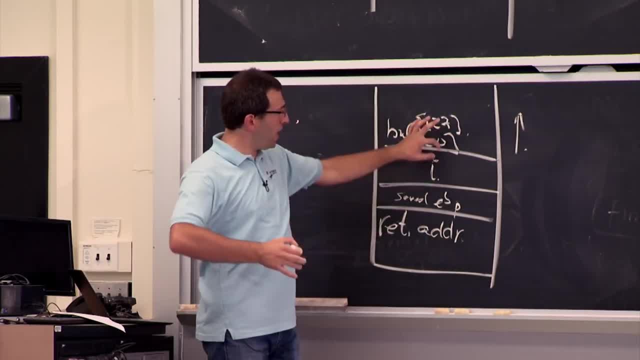 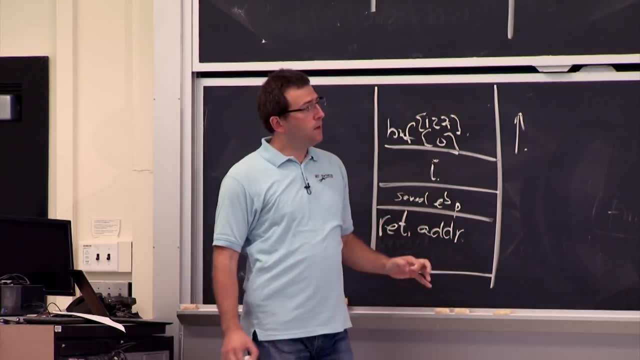 and maybe it doesn't hit anything bad. I guess what you're saying is that, well, maybe we had a buffer down there, And if we had a buffer down there, then yeah, that seems kind of unfortunate. It could overrun this return address. 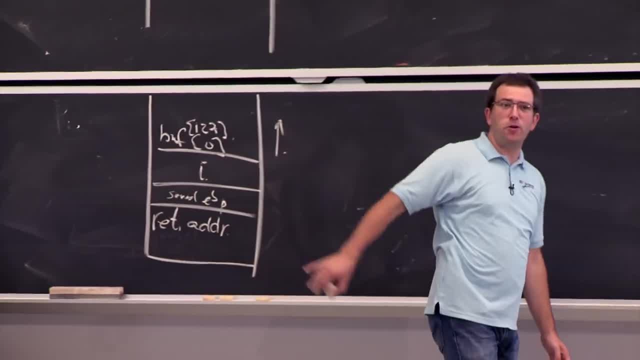 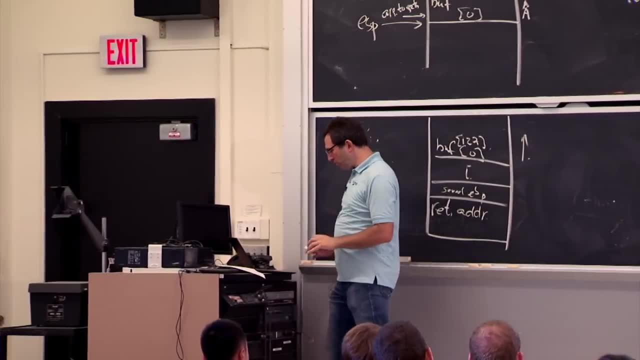 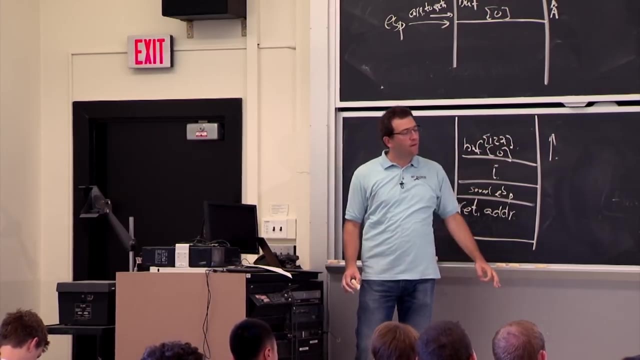 So you're right. So you could still run into problems on this stack growing up. But what about this exact program? Is this particular program safe on machines where the stack grows up? So just to recap what the program is: this guy, Yeah. 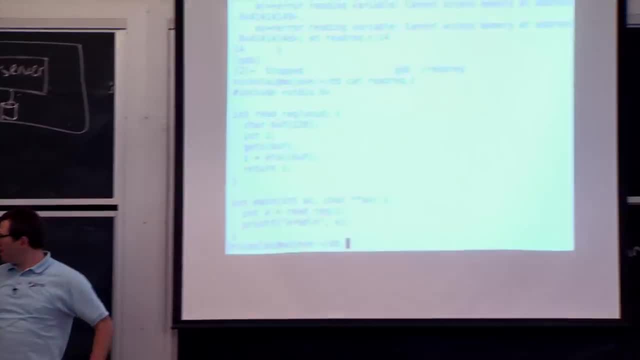 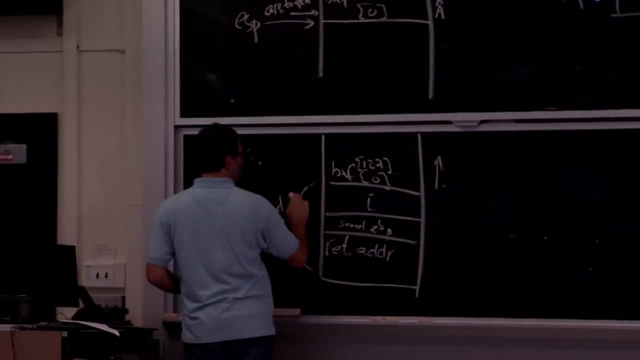 You're still going to overwrite. Yeah, so that's actually clever, right? So this is the stack frame. This is the stack frame for redirect. I guess it actually spans all the way up here. But what actually happens when you call get s? 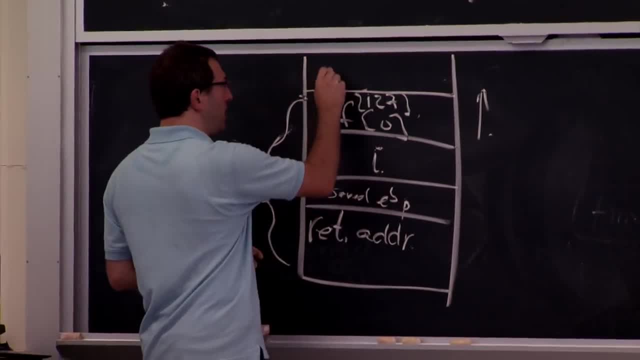 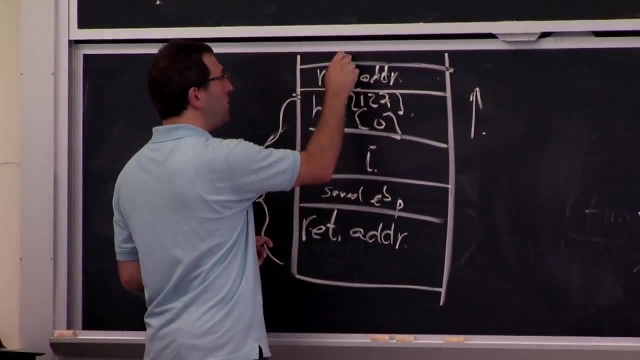 is that redirect makes a function call, It actually saves its return address up here on the stack And then get s starts running And get s puts its own save dbp up here And get s is going to put its own variables higher up. 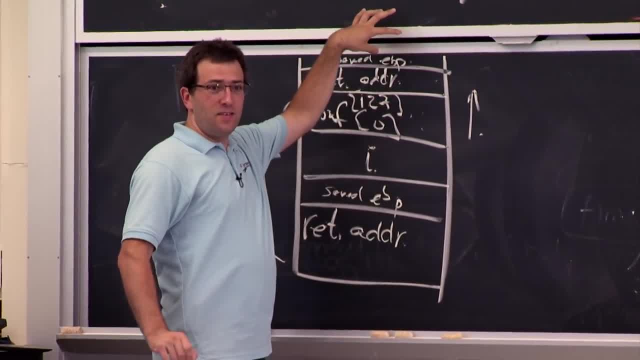 And then get s is going to fill in the buffer. So this is the same thing. It's going to put its own variables higher up And then get s is going to fill in the buffer. So this is the same thing, And get s is still problematic. 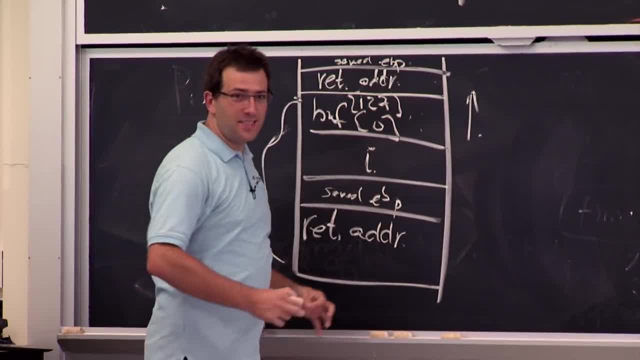 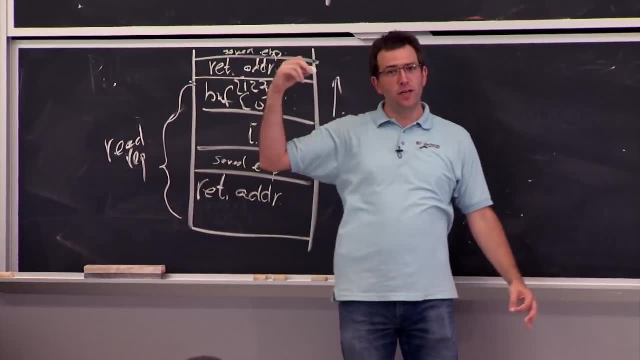 Basically, the buffer is surrounded by return addresses on all sides. Either way, you're going to be able to overflow something. So at what point suppose we had a stack growing up machine? At what point would you be able to take control of the program's execution then? 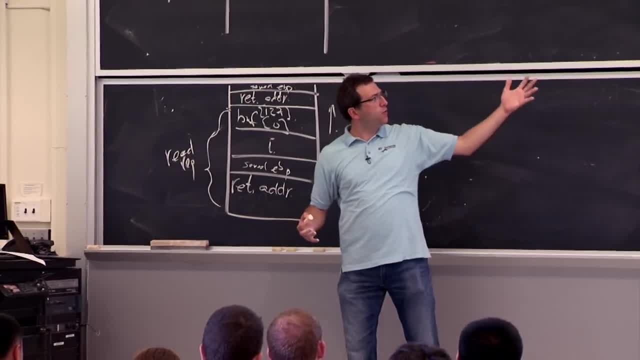 Yeah, so now it's actually even easier in some ways. You don't have to wait until redirect returns And maybe there's stuff that's going to mess you up, like this a to i. No, it's actually easier because get s is going to overflow. 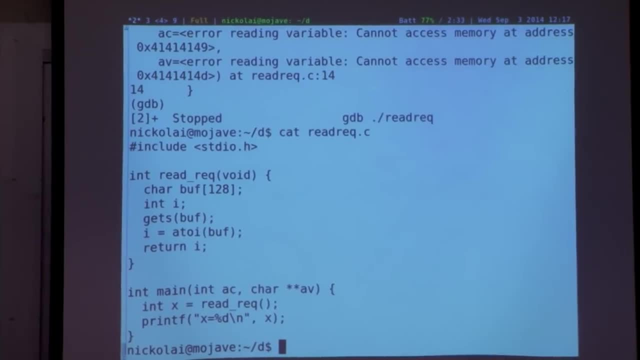 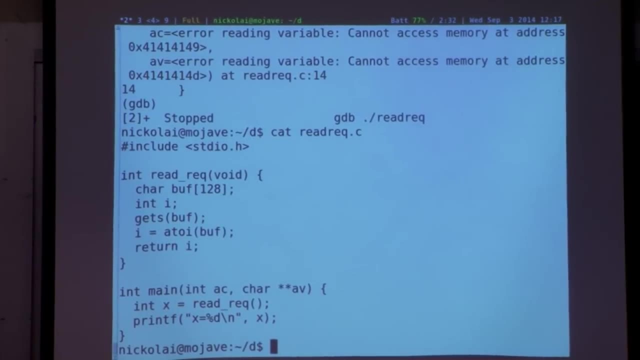 the buffer, It's going to change the return address And then immediately return and immediately jump to wherever you tried to construct Makes sense. So what happens if we have a program like this? that's pretty boring. There's no real interesting code to jump to. 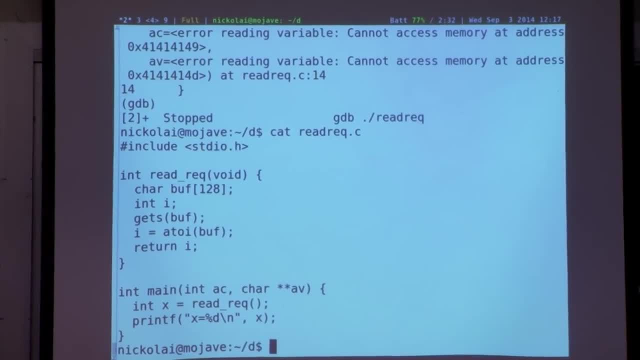 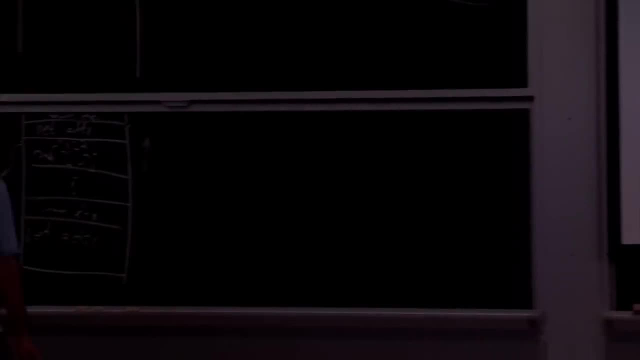 All you can do is get it to print different x values here. What if you want to do something interesting that you didn't? Yeah, I mean, if you have an executable stack, you could put arbitrary code That, for example, executes a shell. 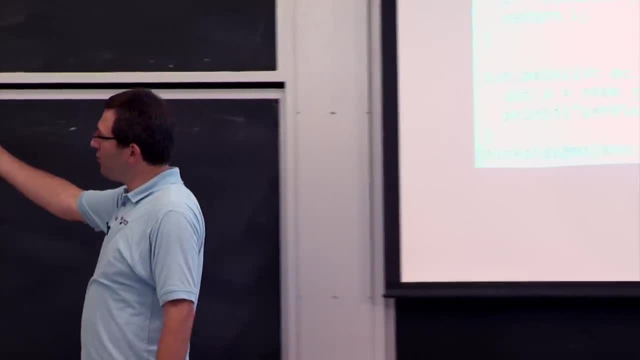 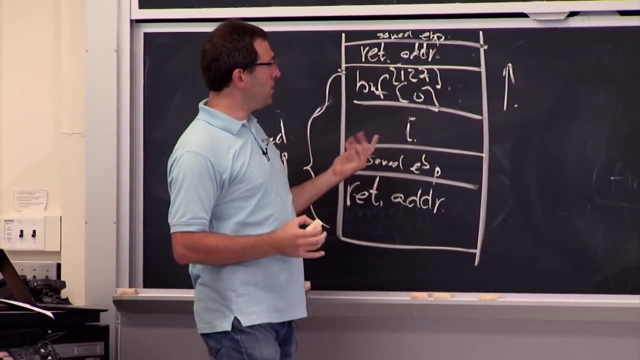 Yeah, so that's kind of clever, right, Because you actually can supply other inputs, right. So at least. well, there are some defenses against this And we'll go over these in subsequent lectures, But in principle, you could have the return address here. 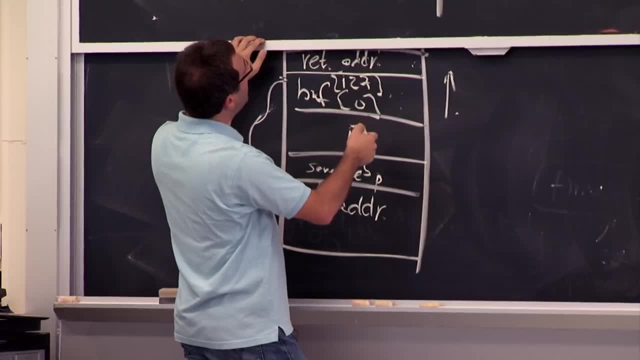 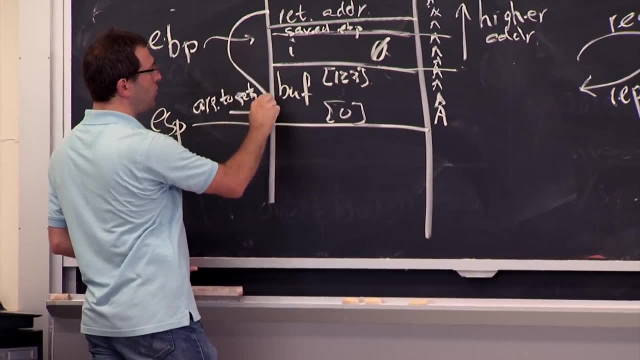 that you override on either the stack up or stack down machine And instead of pointing it to some existing code like the printf inside of main, we could actually have the return address point into the buffer. So it's previously just some location, But you could jump there and treat it as executable. 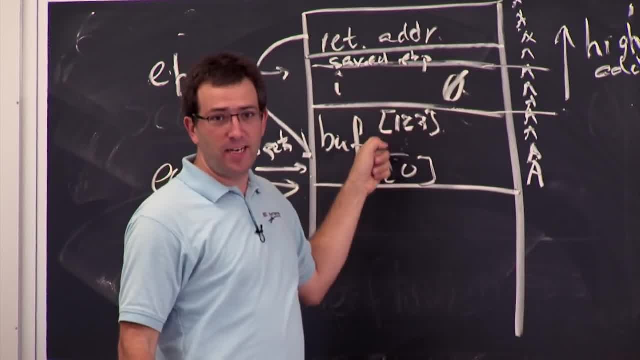 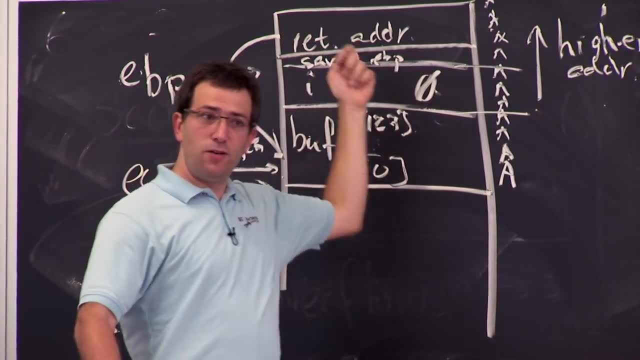 So, as part of your request, you'll actually send some bytes of data to the server and then have the return address or the thing you overwrite here point to the base of the buffer, And you'll just keep going from there. So then you'll be able to provide the code you want to run. 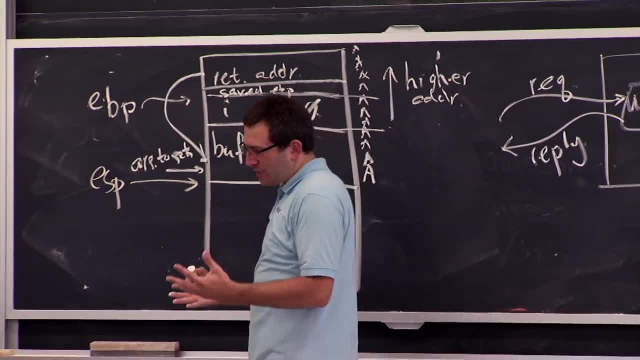 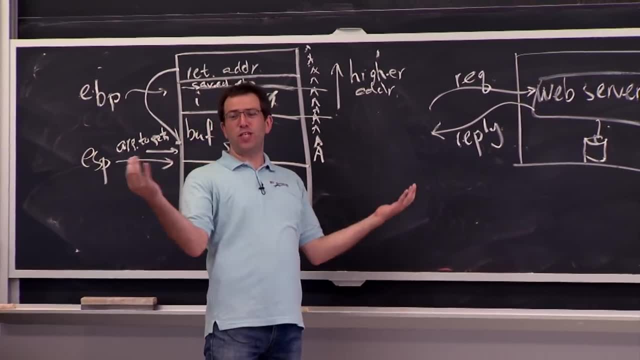 jump to it and get the server to run it, And in fact, traditionally in Unix systems, what adversaries would often do is just ask the operating system to execute the binsh command, which lets you type in arbitrary shell commands after that. 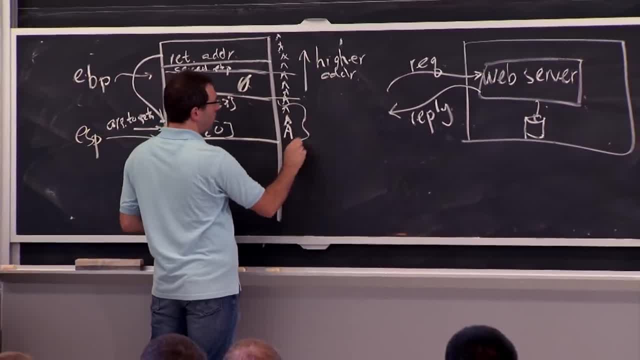 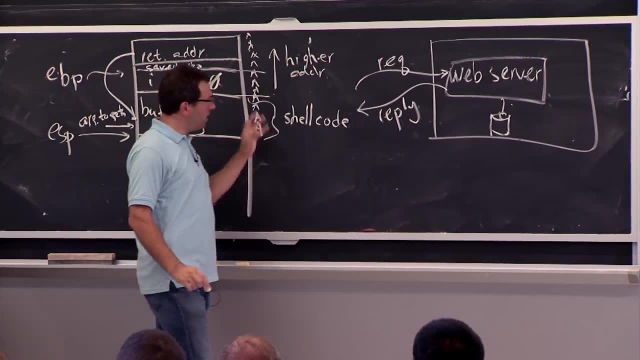 So, as a result, this thing, this sort of piece of code you inject into the buffer, was often called, for historical reasons, shell code, And you'll try to construct some in this lab one as well. All right, Make sense. 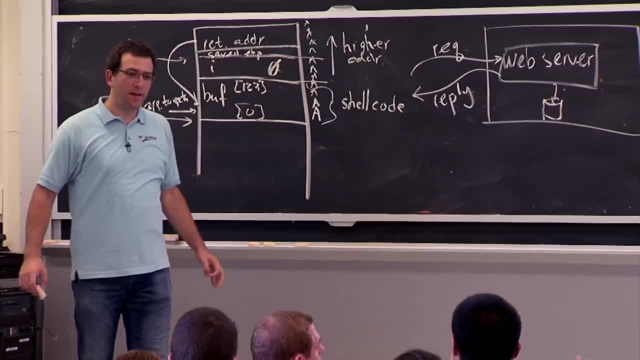 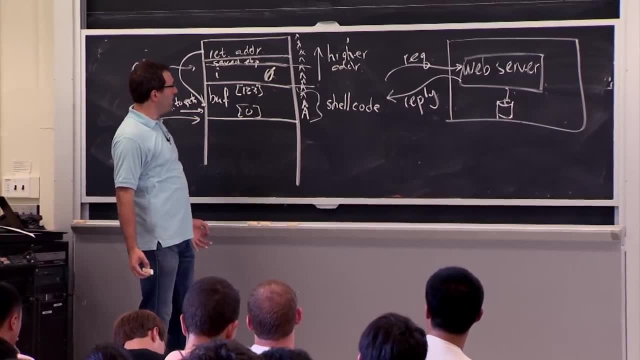 What you can do here. Yeah, Is there a separation between code and data? Right? So is there a separation between code and data here At least? well, historically, many machines didn't enforce any separation of code and data. You just have a flat memory address. 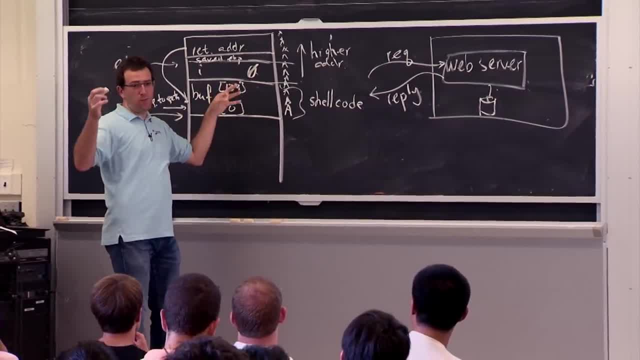 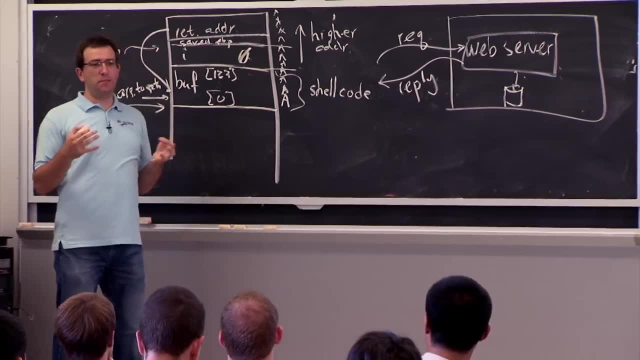 In the address space. the stack pointer points somewhere, The code pointer points somewhere else And you just execute wherever the code pointer or instruction pointer is pointing. Modern machines try to provide some defenses for these kinds of attacks. And what modern machines often do. 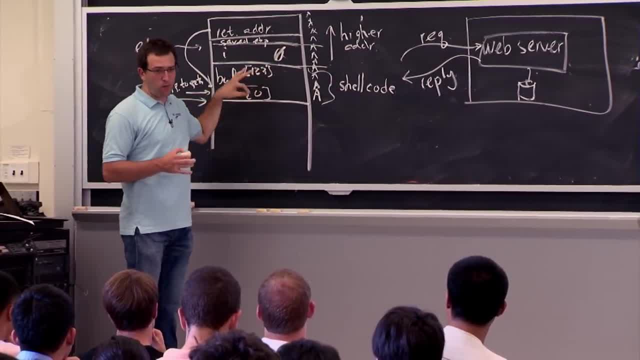 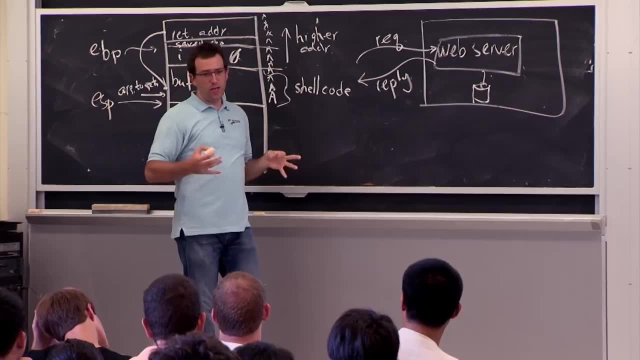 is they actually associate permissions with various memory regions And one of the permissions is execute. So the part of your 32-bit or 64-bit address space that contains code has the execute permission. So if your instruction pointer points there, the CPU will actually run those things. 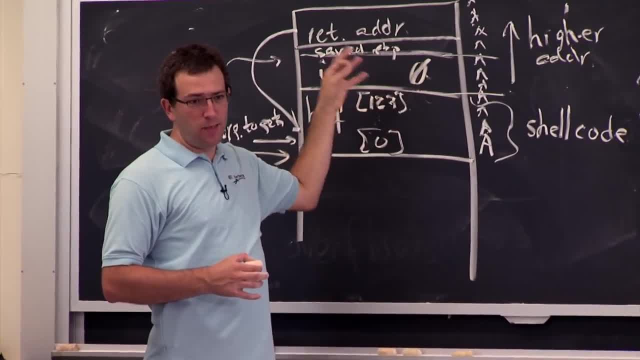 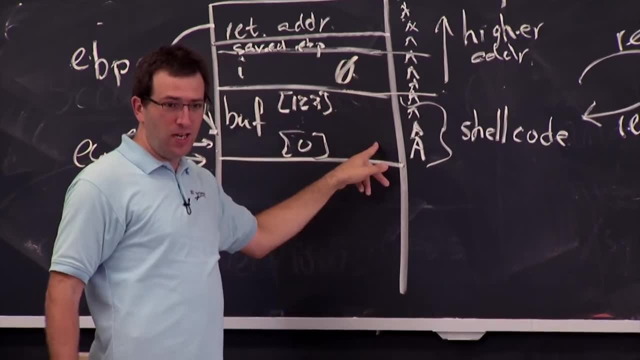 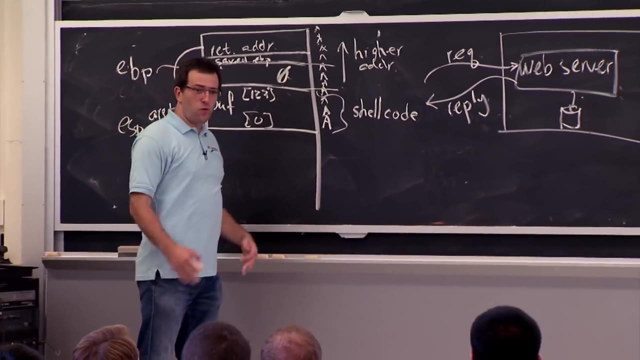 And the stack and other data portions of your address space typically don't have the execute permission. So if you happen to somehow set your instruction pointer to some non-code memory location, you can set it, But the CPU will refuse to execute it. So this is a reasonably nice way to defend. 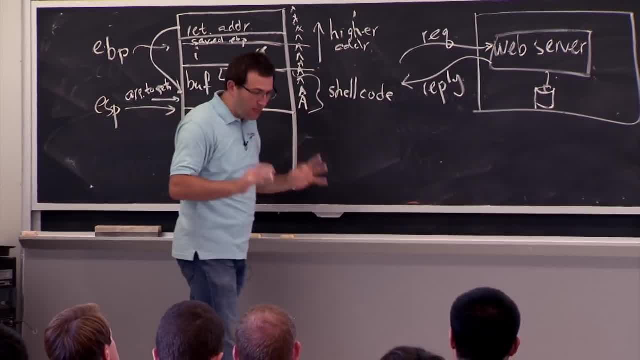 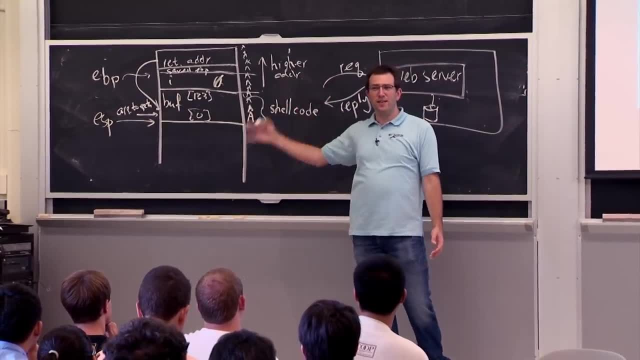 against these kinds of attacks, But it doesn't prevent anything, quite everything. So just a question: OK, so how would you bypass this if you had this non-execute? I guess we actually saw this example earlier, right When I actually jumped to the middle of main. 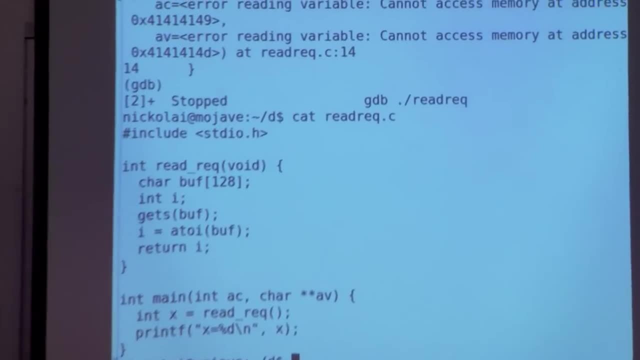 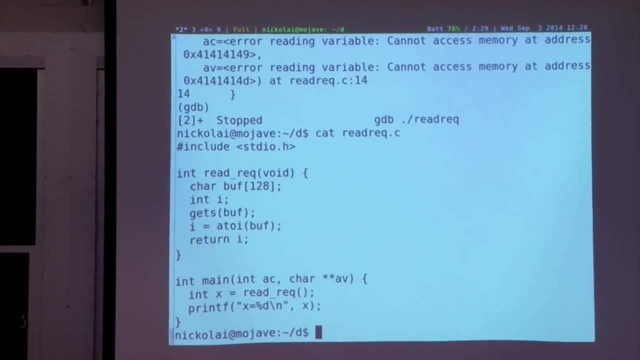 So that was a way of exploiting this buffer overflow without having to inject new code of my own. So even if the stack was non-executable, I would still be able to jump in the middle of main. In this particular case. it's kind of boring. 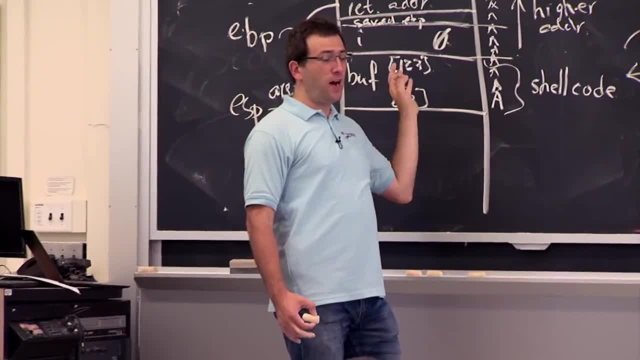 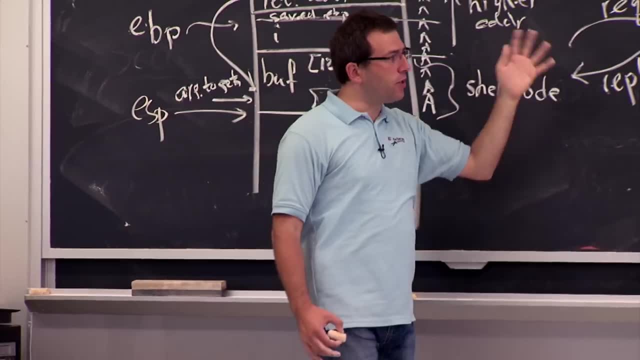 It just prints x and crashes. But in other situations you might have other pieces of code in your program that are doing interesting stuff that you really do want to execute And that's sort of called return to libsia. It's a way to bypass these security attacks for again. 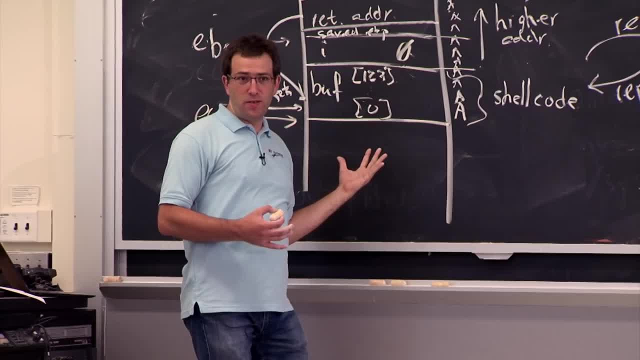 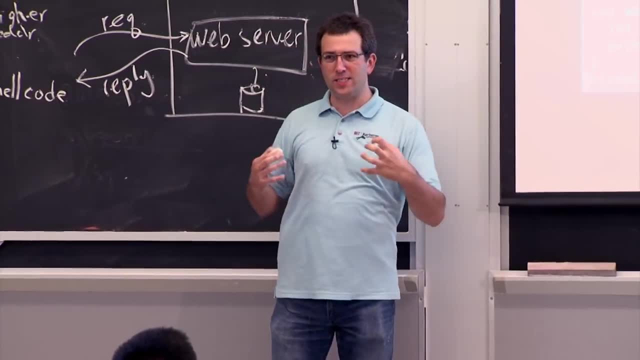 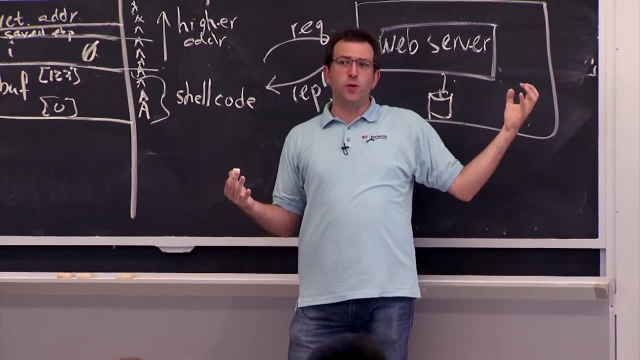 somewhat historical reasons, But it is a way to bypass these security measures. So, in the context of buffer overflows, there's not really a clear-cut solution that provides perfect protection against these mistakes, Because, at the end of the day, the programmer did make some mistake in writing a source code. 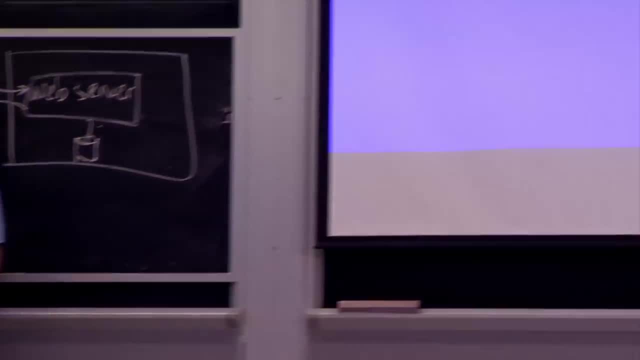 And the best way to fix it is probably just to change the source code and make sure you don't call get s. very much like the compiler warned you, And there's more subtle things that the compiler doesn't warn you about, It's just making those calls. 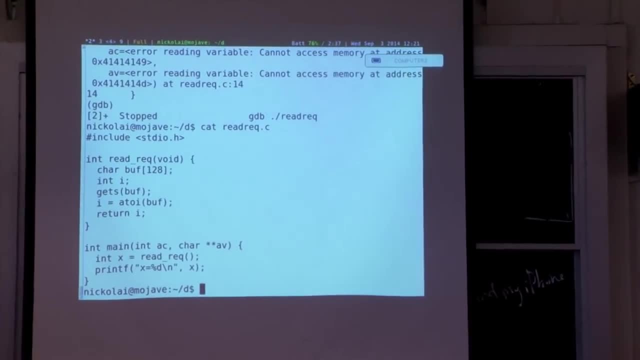 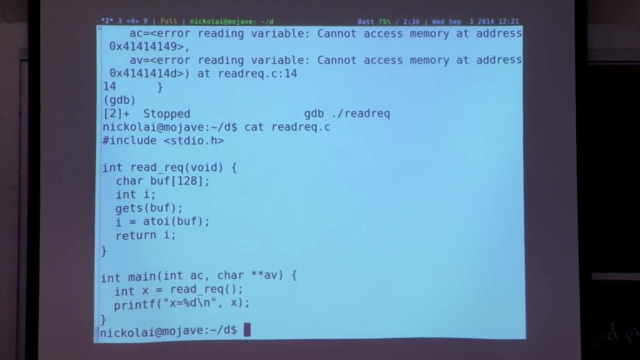 But because it's hard in practice to change all the software out there, many people try to devise techniques that make it more difficult to exploit these bugs, For example making the stack non-executable, So you can't inject the shell code onto the stack. 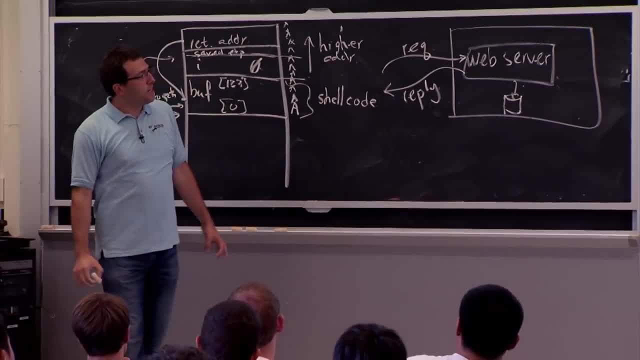 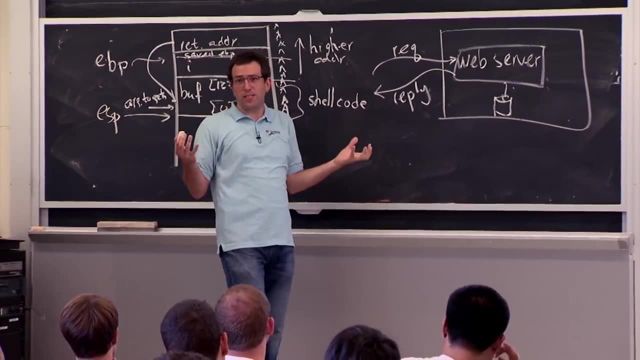 And you have to do something slightly more elaborate, And next two lectures, actually, we'll look at these defense techniques. They're not all perfect, But they do in practice make it much more difficult for that hacker to exploit things. Question. 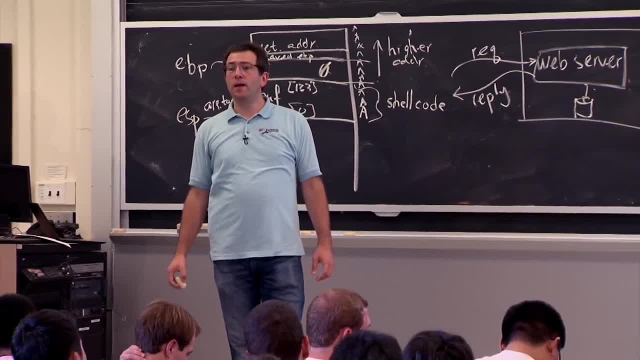 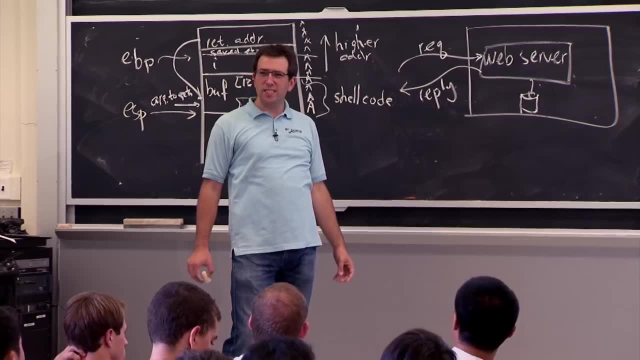 I was going to ask a general administrative question. I was wondering if there's a final and also if there are quizzes and what they are. Oh, yeah, Yeah, I think if you go to the schedule page there's two quizzes. 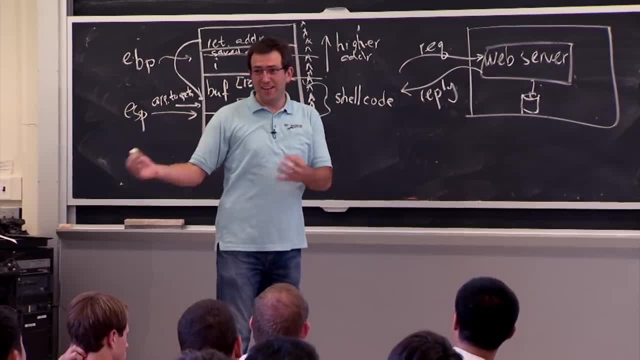 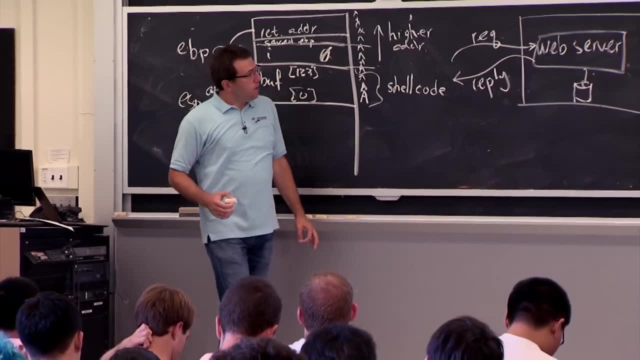 And there's no final during the final week, But there's a quiz right before it, So you're free for the final week, But there's still something at the end of the class. Yeah, All right, OK, so I think that's probably it for buffer overflows. 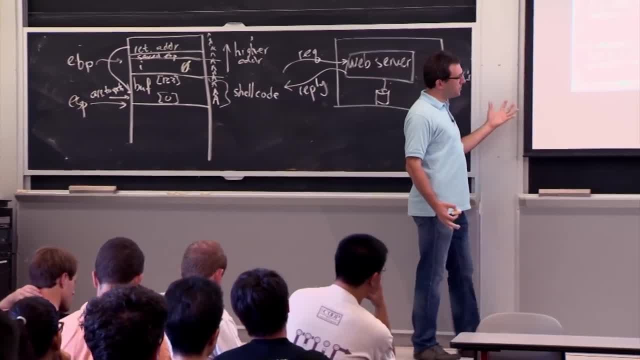 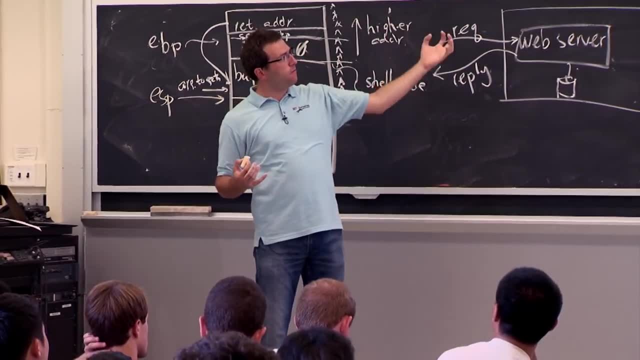 I guess the one question is OK. so what do you do about mechanism problems? And the general answer is to probably have fewer mechanisms. So, as we saw here, if you're relying on every piece of software to enforce your security policy, you'll inevitably have mistakes. that 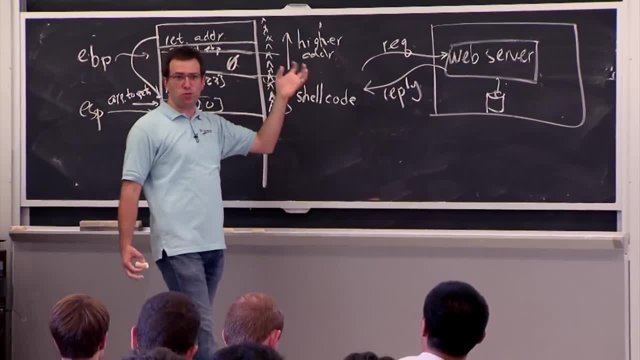 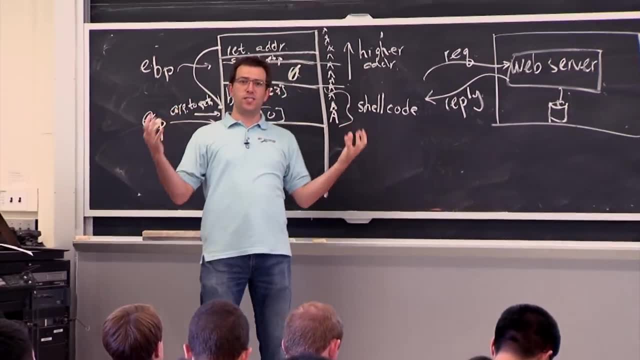 allow an adversary to bypass your mechanism to exploit some bug in the web server. And a much better design, and one that you'll explore in lab two, is one where you structure your whole system, so the security of the system doesn't depend on all the pieces of software. 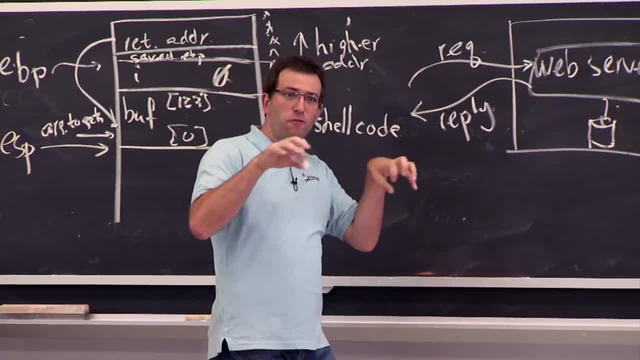 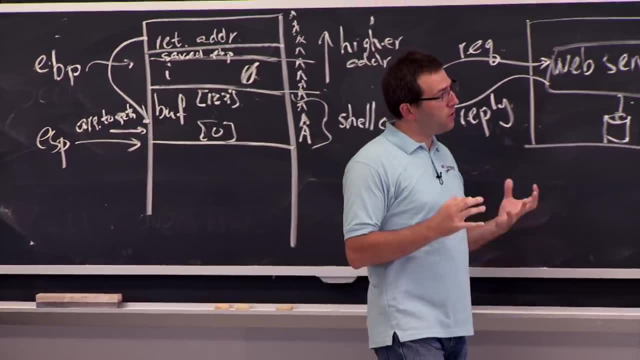 enforcing your security policy. The security policy is going to be enforced by a small number of components And the rest of the stuff actually doesn't matter for security purposes. if it's right or wrong, It's not going to violate your security policy at all. 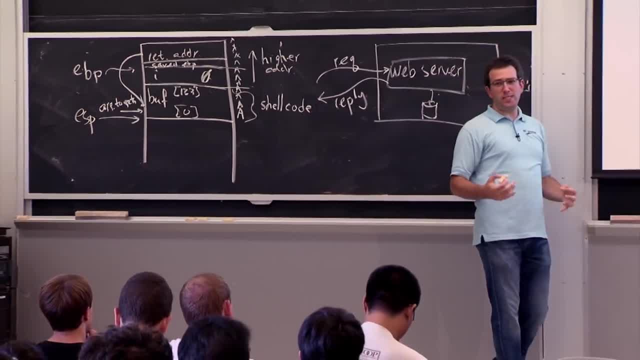 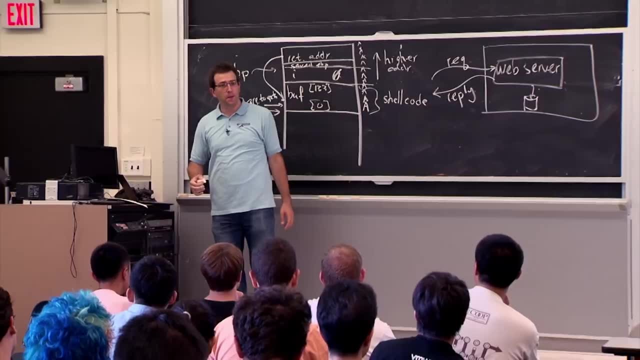 So this kind of minimizing your trusted computing base is a pretty powerful technique to get around these mechanism bugs and problems that we've looked at today, at least in a little bit of detail. All right, so read the paper for Monday and come to Monday's lecture and submit. the questions on the website. See you, guys then. 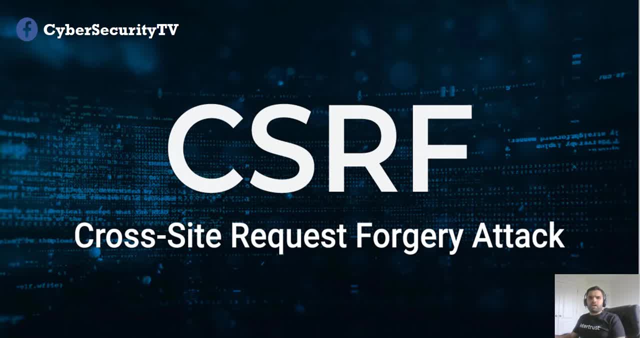 Hey everyone, welcome back to Cybersecurity Rehab. Today we're going to talk about the cross-site request forgery, or you can say CSRF. The reason I want to talk about this vulnerability is it's not very exciting, but recently I've been doing pen testing and I found this vulnerability in quite a few apps.